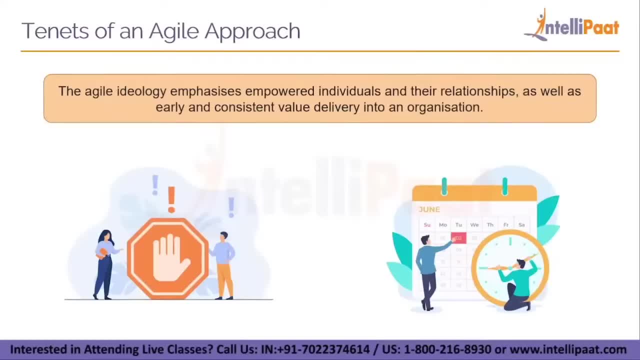 relationship, as well as early and consistent value delivery into an organization When the pressure to perform is greater than the risk. agile project management focuses on providing maximum value against business priorities in the time and money allotted. The following are some of the principles: The project divides the requirement into smaller chunks, which the team then 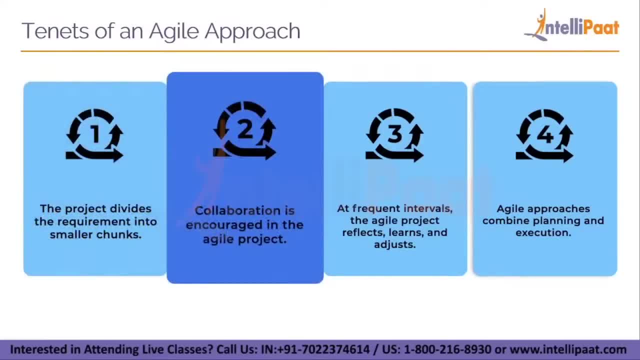 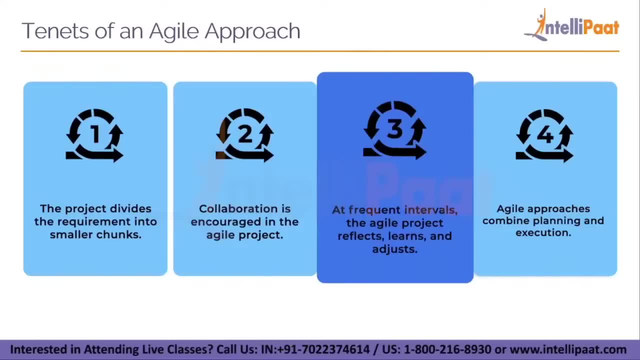 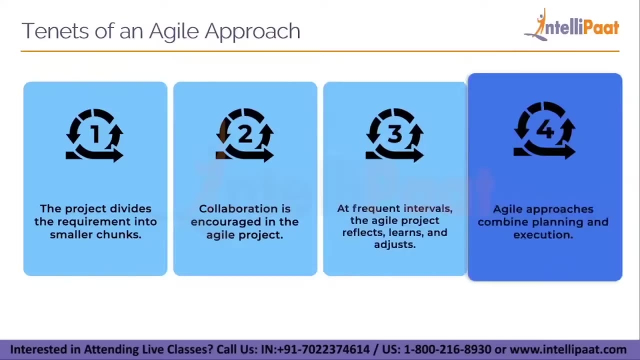 ranks in order of importance. Collaboration is encouraged in the agile project, especially with the customer. At frequent intervals, the agile project reflects, learns and adjusts to guarantee that the customer is always satisfied and that the benefits are delivered. Agile approaches combine planning and execution, allowing a company to develop a working attitude. 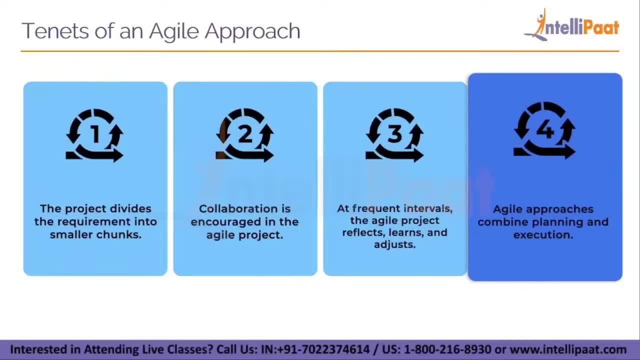 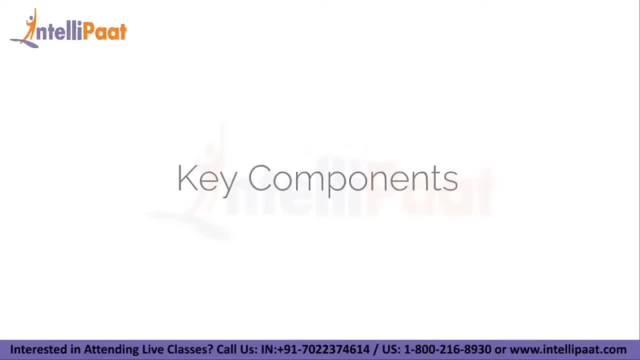 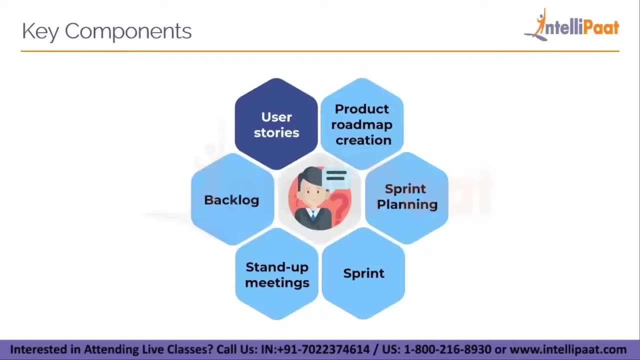 that enables a team to adjust quickly to changing needs. Now let's take a look at the key components of an agile approach. Agile project management primarily has six key components, and they are user stories. Simply put, a user story is a high-level description of a task It gives. 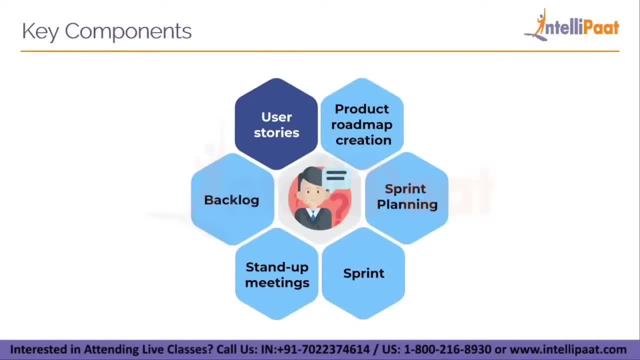 just enough information for the team to come up with a credible estimate of the time it will take to complete the request. This brief, straightforward explanation is written from the user's point of view and focuses on describing what your client wants and why they need it. 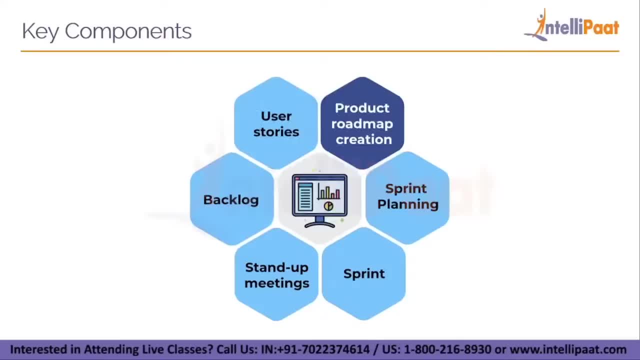 Do they want so? Next, we have product roadmap creation. A roadmap is a list of features that will be included in the final product, Because your team will construct these specific features throughout each sprint. this is an important part of an agile planning cycle. 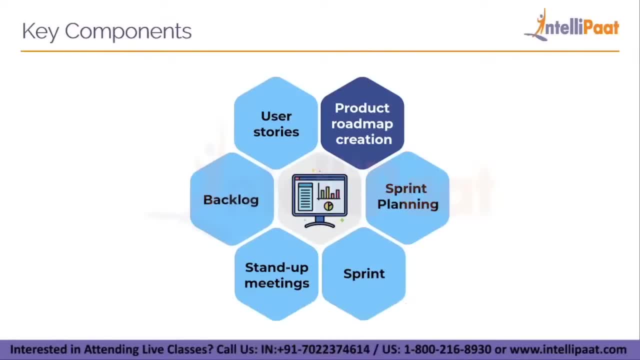 You will also create a product backlog at this time, which is a list of all the features and deliverables that will go into the final product. Your team will extract tasks from this backlog when planning sprints later. Next, we have sprint planning. Before each sprint begins, the stakeholders must attend. 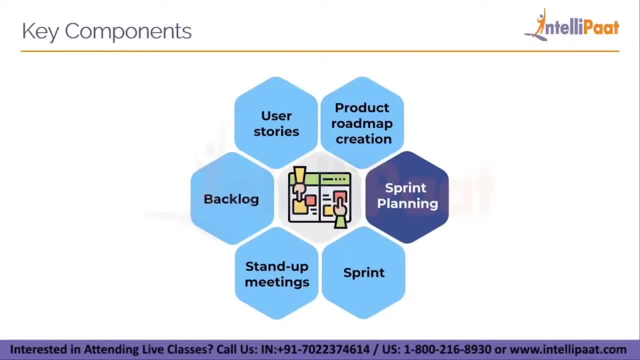 a sprint planning meeting to identify what each individual will do during the sprint, how it will be accomplished, and assess the task load. It's critical to equally distribute the workload among team members so that they can complete their assigned duties during the sprint, For team openness, shared understanding and detecting and reducing bottlenecks. you 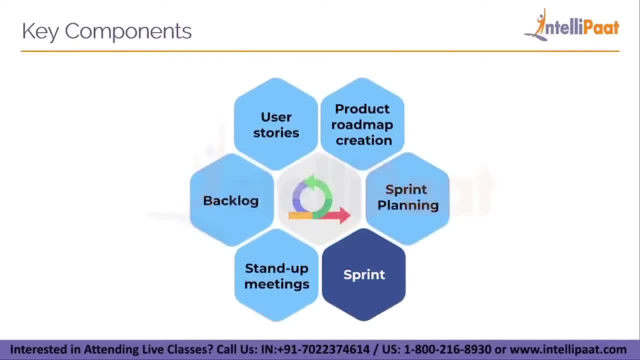 can easily describe your workflow. Next, we have sprint. Sprints are short iterations of 1-3 weeks in length, during which teams focus on tasks set out at the sprint planning meeting. As time goes on, the goal is to keep repeating these sprints until your product is future ready. After the sprint, you analyze. 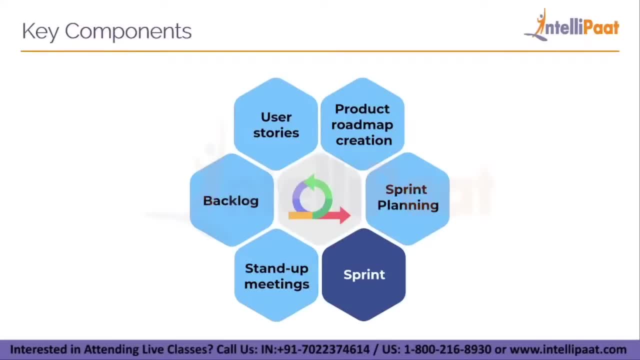 the product to see what is working and what is not, make improvements and start a new sprint to improve the product or service. Next, we have sprint planning. Sprint planning is a process that involves the startup meetings. Daily startup meetings, often known as daily scrum meetings, are an 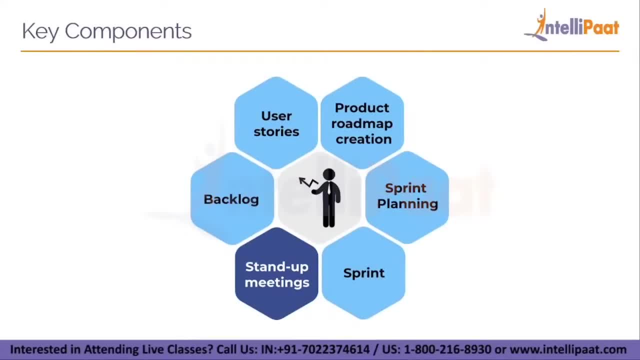 excellent approach to keep everyone on track and informed. These meetings are usually short and to the point. Last component that we have here is backlog. Project requests become outstanding stories in the backlog as they are added through your intake mechanism. Your team will estimate narrative points for each task during agile planning meetings. Stories from the backlog. 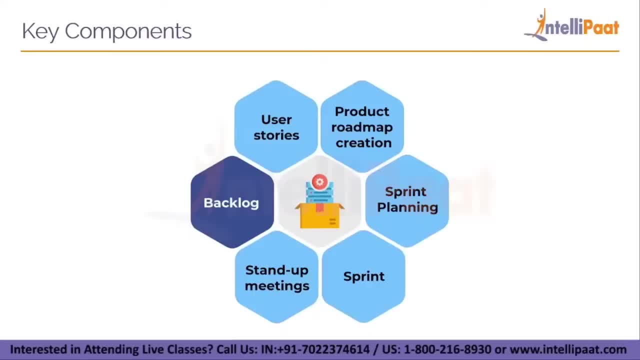 are added into the sprint to be prepared for the sprint. Next we have sprint planning. Sprint planning is a process that involves developing a sprint which is performed during the iteration. that is done during sprint preparation In an agile context. managing your backlog is critical for project managers With that. 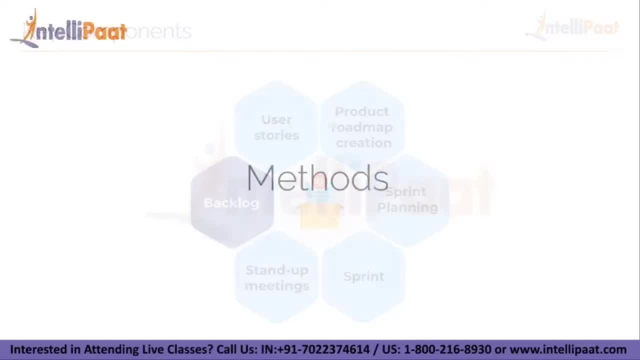 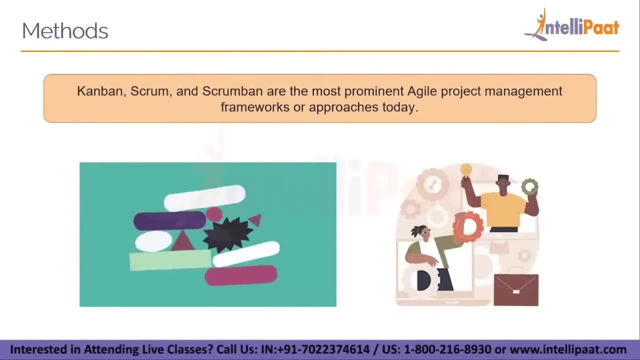 being the last component, let's move on to our next agenda, that is, the methods involved. As agile became a popular topic at the turn of the century, numerous frameworks jumped on the bandwagon and quickly rose to prominence, like scrum, etc. Many firms pursuing true business. 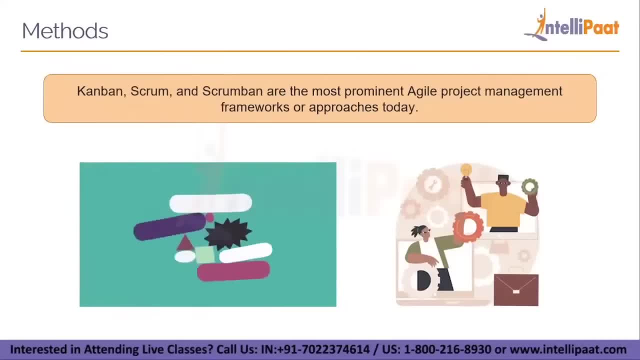 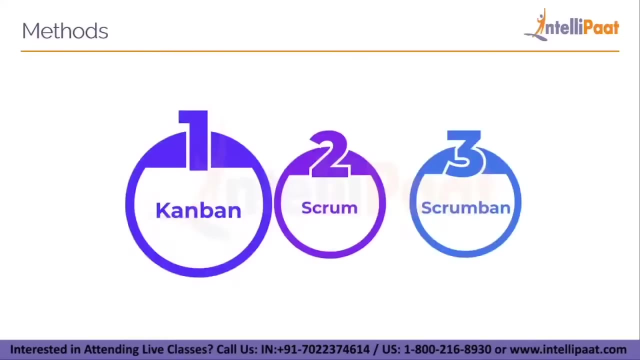 agility, on the other hand, discovered that overly prescriptive frameworks and agility are diametrically opposed. Kanban, Scrum and Scrumban are the most prominent agile project management frameworks or approaches that are present today. Let's start with Kanban. It is a method that was developed over a decade ago. It focuses 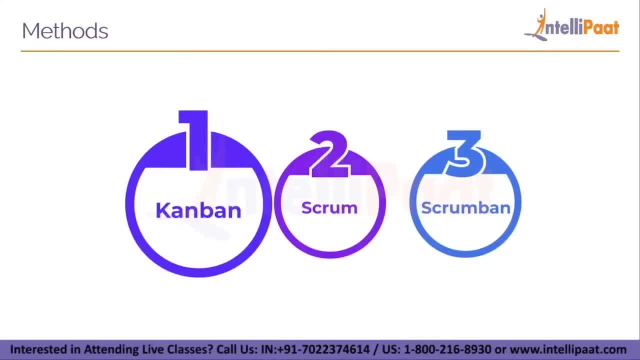 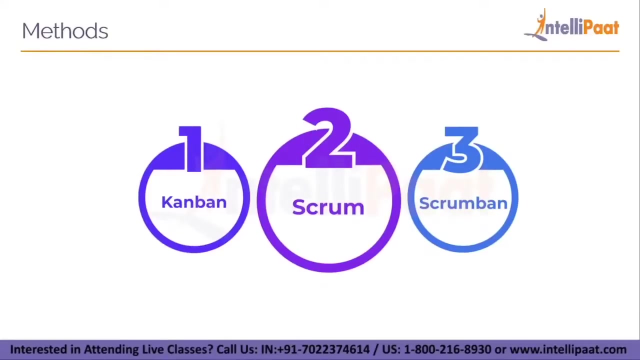 on ongoing process improvement and evolutionary development. The six key practices of the technique follows: Improve cooperation by visualizing work, limiting work in progress, managing flow, making process policies explicit, implementing feedback loops and improving collaboratively. Next up, we have scrum. Many people mistake scrum for an agile methodology, although it 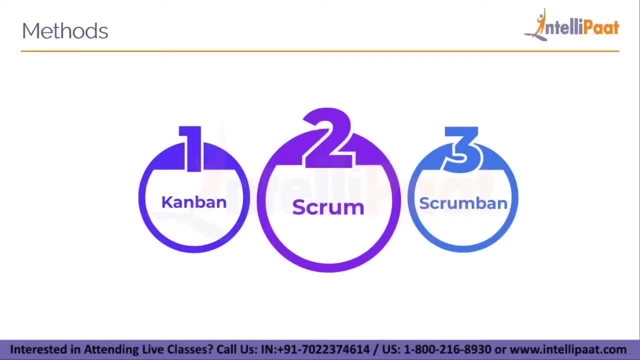 is essentially a prescriptive framework. It is an iterative approach that divides projects into set periods, called sprints, and uses time-boxed intervals. The primary goal is to assist teams in delivering high-value products in a productive and creative manner. There are three roles that cannot be changed in a scrum: Owner of the product. 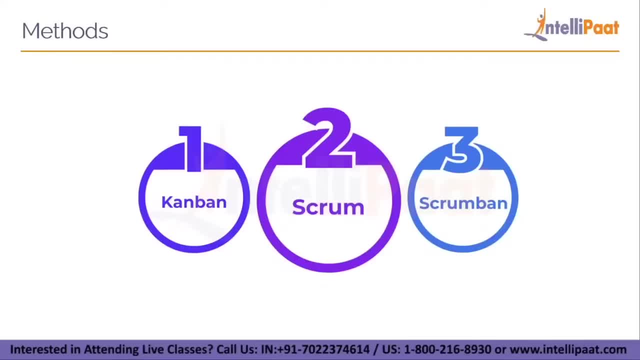 the scrum master and the team, Customers and other stakeholders are represented by the product owner. He or she organizes and manages the product backlog, which is a priority task list of all the product's work items. The scrum master, on the other hand, is a: 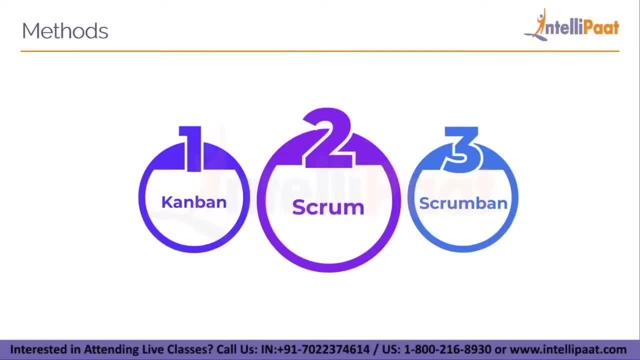 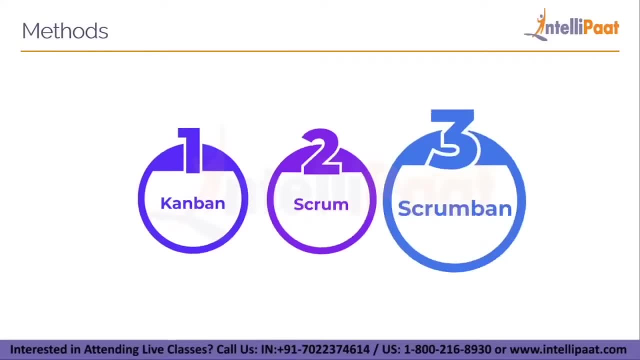 servant leader of the team. He or she is a leader of the team. The scrum master, on the other hand, is a person who is focused on leadership and assists everyone in understanding and applying the rules appropriately. And, lastly, we have scrum ban. A scrum ban became increasingly popular for individuals. 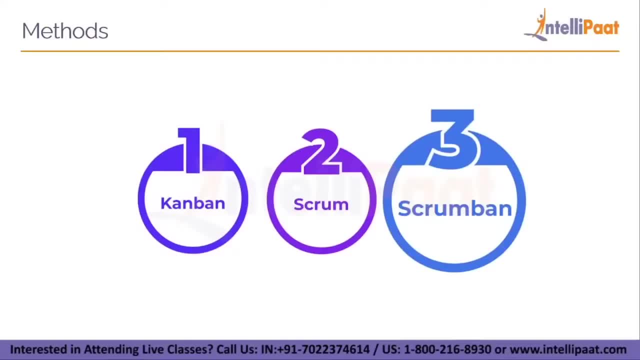 in the Agile community. This requires an opportunity to create a system that allows scrum teams to focus on continuous improvement and evolutionary change while moving forward. Scrum ban was born as a result of this. It's worth noting that 81% of scrum masters use 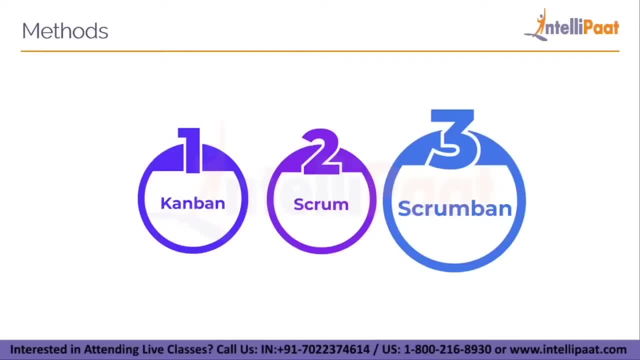 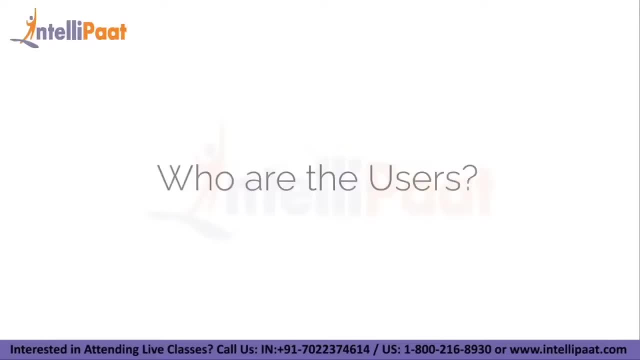 Kanban, in addition to Scrum. Scrum ban applies Kanban's concepts and practices to Scrum, while also removing some rules. Now let's move on to our next agenda. that who are the users or who uses agile project management, The agile project. 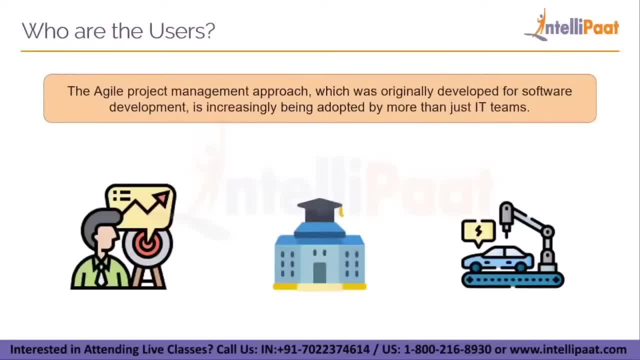 management approach, which was originally developed for software development, is increasingly being adopted by more than just ID teams. marketers, universities, the military and even the automobile industry are using it Agile methodologies and frameworks to develop creative products in difficult circumstances. Agile project management may help a wide range of enterprises and 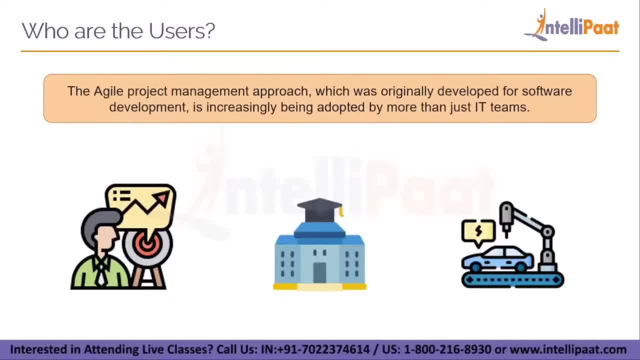 it's simple to set up and use. When deciding to establish or improve as existing technology in the software sector, the ultimate product can be difficult to describe. Agile allows for this ambiguity, since it enables project direction to alter as work goes on. Agile allows for this ambiguity, since it enables project direction to alter as work. 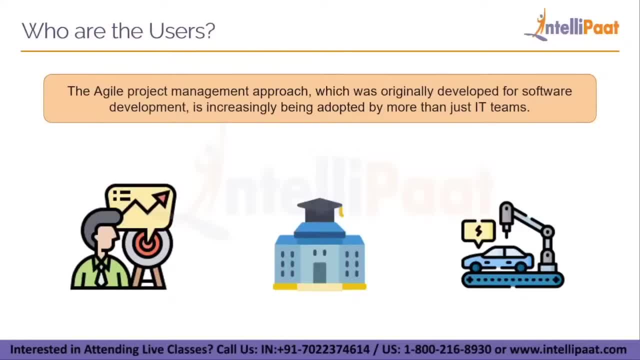 progresses into the future, While agile software, books and coaches can help you put together an agile methodology that works for you and your team, Each agile team is unique, and understanding the basics can help you build together an agile methodology that works for you and your team. Now let's move on to the 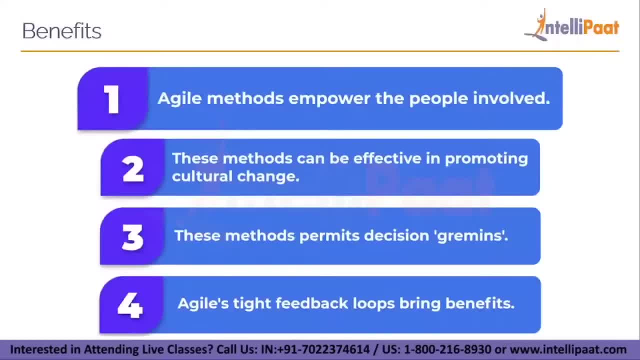 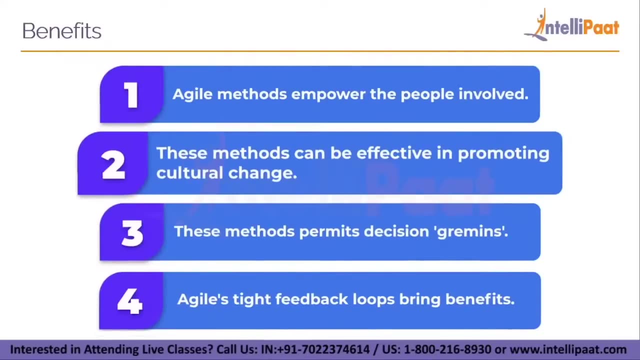 benefits of agile working. The first benefit that we have here is agile methods empower people involved, hence increasing accountability, promoting a variety of ideas, allowing early benefits release and promoting ongoing improvement. Second benefit is agile can be effective in promoting cultural change, which is important to the success of most. 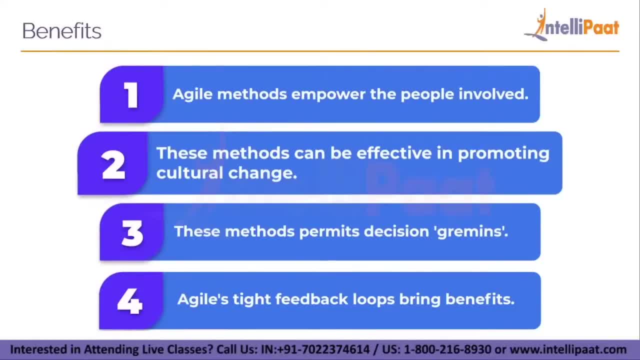 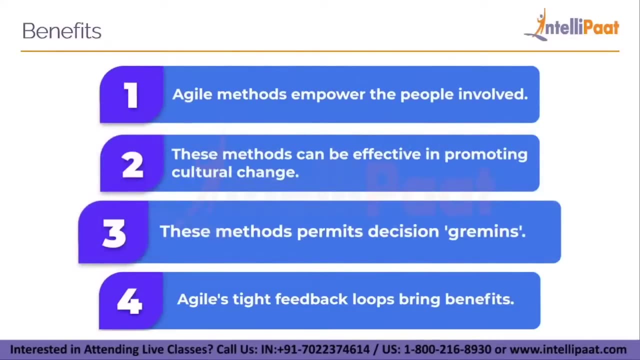 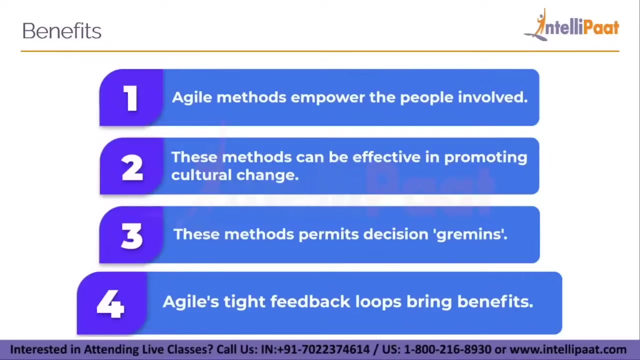 transformation projects because changes are progressive and evolutionary rather than revolutionary. As a result, it can assist in creating client and user involvement. Agile permits decision gremlins to be tried and rejected early, whereas the waterfall model does not. Agile's tight feedback loops bring benefits that, again, the waterfall model does not. 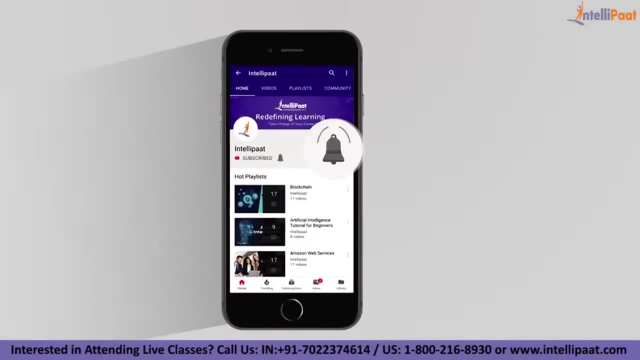 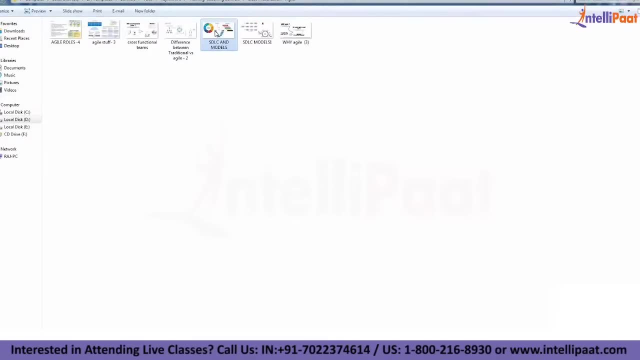 But before we begin the session, make sure to subscribe to our channel and press the bell icon so that you'll never miss any update from us. So understanding and identifying the right development lifecycle model is essentially important for any application development Successful. it's not only about how technically are we strong, but it is 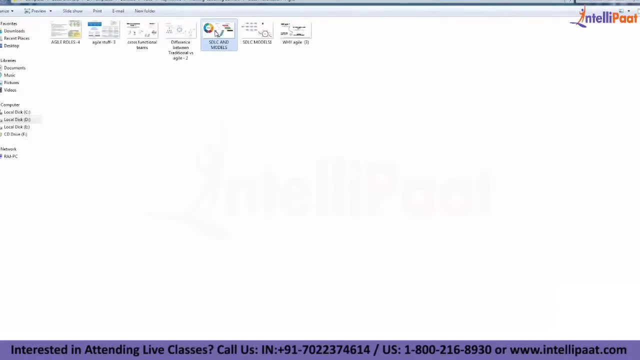 equally important to understand the right development lifecycle models. So, whatever are we going to discuss about agile and all everything is connecting to that, So let me explain you in a high-level note about the different, different models which are available, wherein you can see on the screen here: 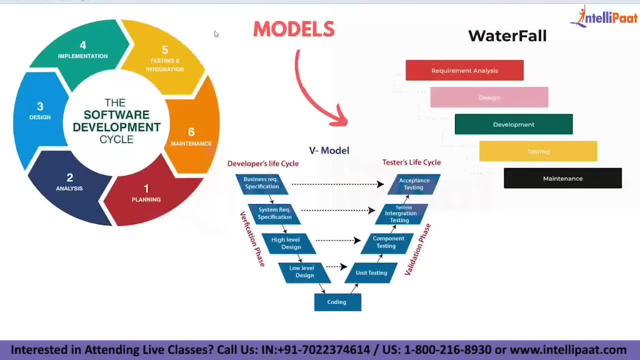 So there are different, different models of software development lifecycle. I'm just naming few, I'm not going in detail. So one, the first model we call it, is waterfall model. Waterfall is a kind of model which is also called as linear sequential model. So where we have 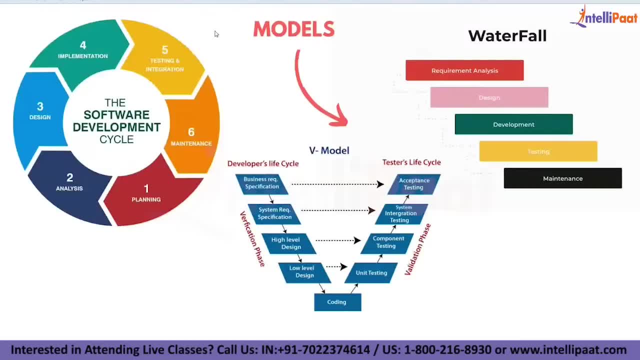 whatever the analysis, planning, design, implementation, testing or whatever we have, everything will happen one after another, so that there will be of no deviation, nothing. so once the analysis is completed, we go for a planning and design, followed by this we go for implementation of the project, testing, all that stuff, one after another. this is a kind of model, which is a traditional. 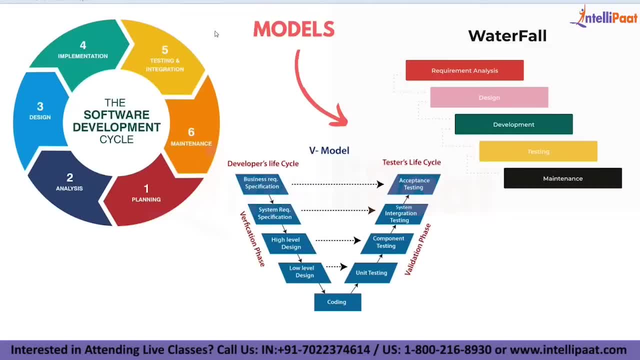 on its approach using BIOS for a very long time. at the same time, this is a kind of model which is call as linear sequential model. This is a model which having its own success rate in application development, but make sure the requirements, whatever customer has given, should not have any kind of 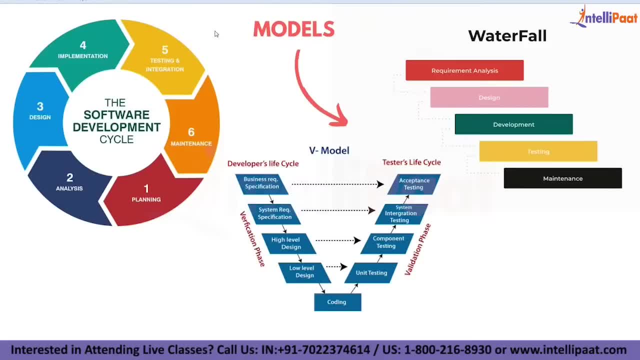 changes in between, and so when there is an assurance given by the client that no changes in requirements taken place, this waterfall model is highly useful. this is the first model, so this model, of course, even nowadays, even waterfall model underline, we use because when someone are new to agile or someone are new to 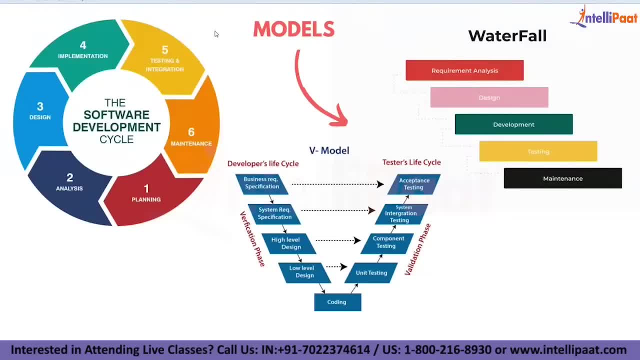 application development. this is the model which is rightly useful for everyone. the next model: we call it as V model. this V model will also called as verification and validation model. here both verification and validation happen. sequentially means whenever we have limited time- because in the first model of V model we don't have any- when there is no time restriction, no duration. 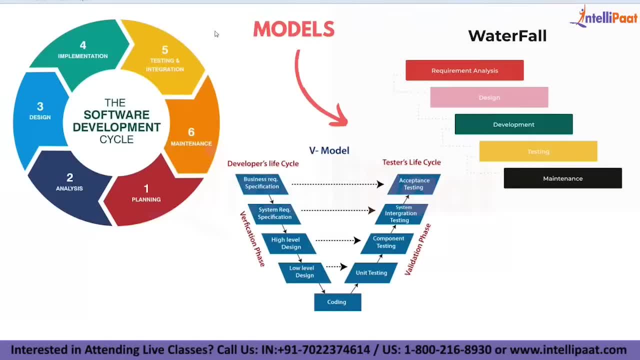 restriction. that model is highly useful. which one waterfall or sometimes customer has approached us to develop the project, to complete and provide the whole project? assume that it is taking eight months to one year. assume that right roughly. I'm saying when customer is accepting you at the same time when customer is accepting you that. 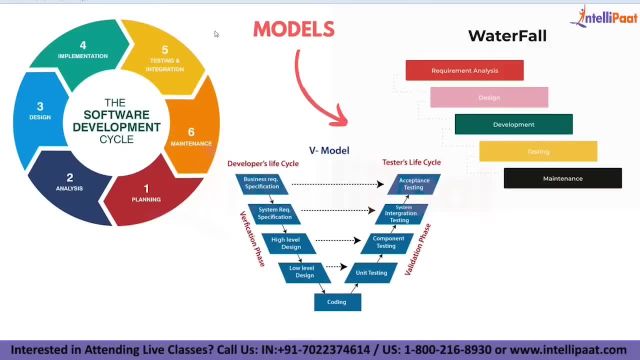 that no changes will be taken place in between waterfall is the best one. the second model is called as V model. V model means verification, validation, where whatever the development activity followed by the testing activity happens parallelly means testing team will start working right from the requirement analysis phase itself. usually right, because whenever we have taken the 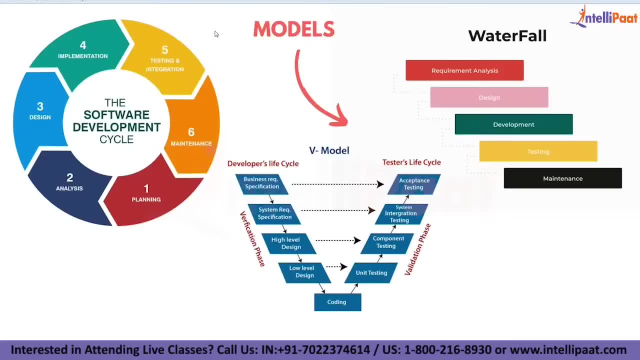 requirements from the BA. BA will take all the requirements right. so we try to analyze the requirements. we try to identify why are these requirements are important, how to understand the requirement- so whenever in this process even testing team will also work parallelly- means what requirements we have taken and what must be the output. that is what generally testing team will. 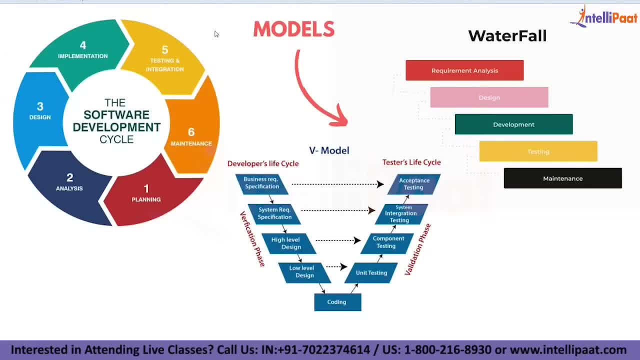 prepare. this is all happens through manual process because in testing there will be two different things. one is manual, second is automation. manual testing means they prepare different, different test cases, test plans, test scripts, all that, whereas automation testing means using different, different tools, something like selenium and all everything. code will be tested. 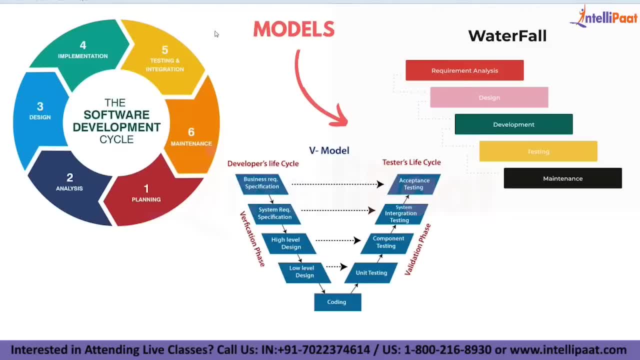 accordingly. so, based on the code, whatever they are tested, if they have identified bugs, that will be prepared as a report again on the document. again, this will be submitted to the implementation team so that they will do the corrections accordingly. this is how generally the process will go on, so this: 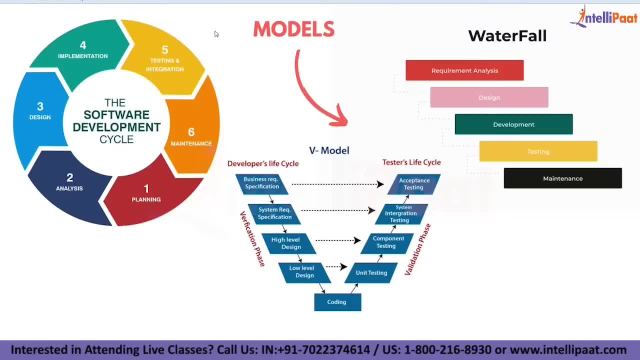 V is a model, verification and validation model majorly used when we have a limited time means when we have a limited amount of time we have. whenever we want to complete is complete it as a list. spray model is highly useful where both development team development as less. 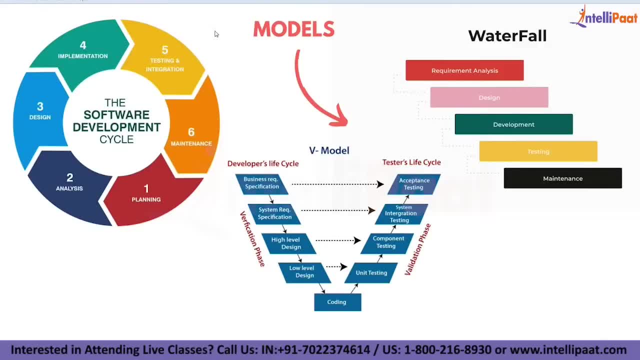 testing happens parallelly means whatever the work we do in the development phase, even before coding starts, even because before coding start there are a lot many things right, so we need to understand the requirements. once we have understood the requirements, we have to classify them. we have to 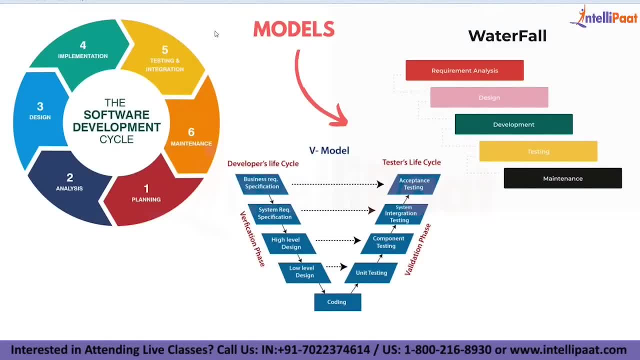 prioritize the record. after prioritization, we have to understand the requirements. whatever the prioritization we have, we need to understand whether these requirements were right or not right. so is this required? requirements were sufficient. so once the requirements we have identified, everything was finalized. then requirements communication. this is where 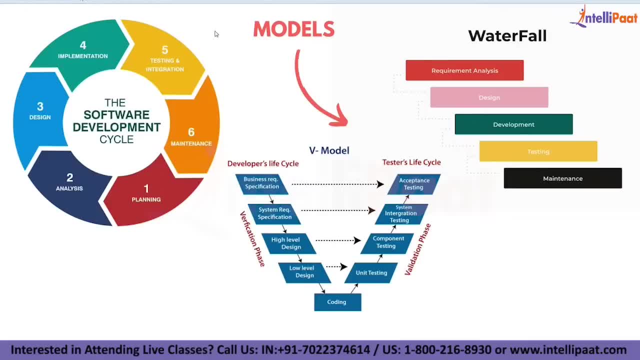 generally this BRD, SRS, all these things comes into picture. so after that we do the designing part, followed by the design, coding will be done. so whatever the activity from the development perspective as well as the testing perspective happens sequentially. this is what we call it as V model. so whenever 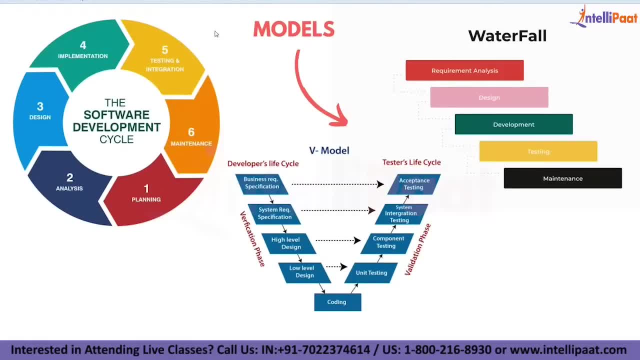 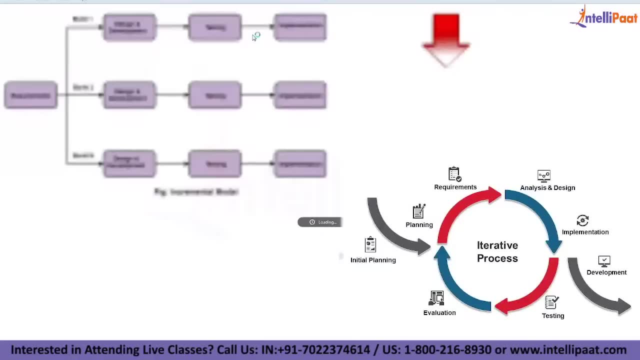 we have a limited time. V model is something highly useful and desirable. this is the second model, the third model, rather than the model. third and fourth are considered as incremental, iterative approaches rather than the model. the best part of the thing I tell you is that incremental and as less iterative are the approaches because- underline- 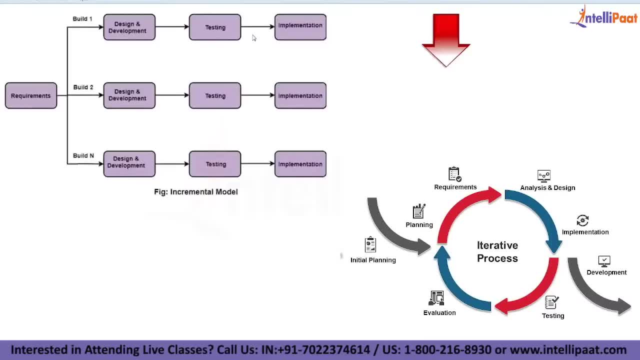 whenever we are working on agile environment. this incrementally iterative will be used because these are the approaches, the best part of saying these two things are approaches. so what is incremental model? incremental model means in each and every phase, each and every build of the application we do, we 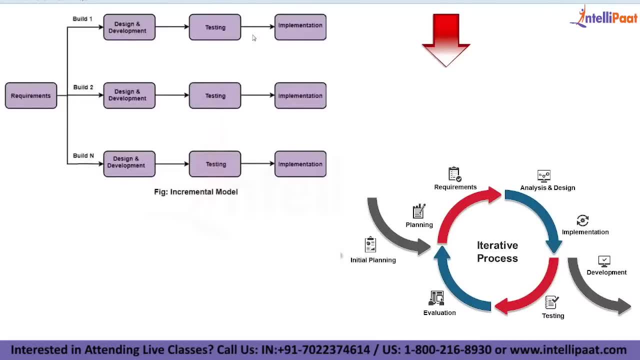 are adding new things into that. i'll give you best example. i think last time i have given. i hope let me repeat the same. if not, let's say there is a customer page, a login page which was created. whatever we have created, whatever the login page we have created so far, login page was created. we have given all the 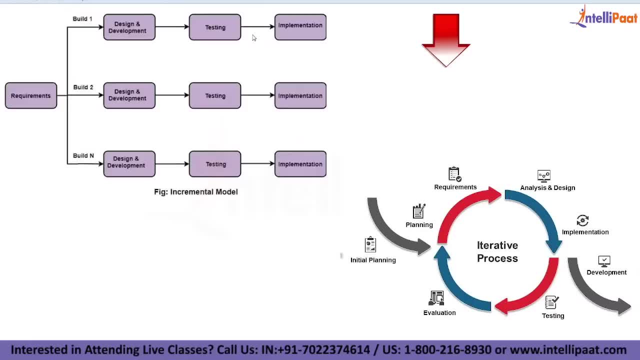 user id password. all the details is given now in between. customer wants you to add some second level verification. means second level verification process is what customer is expecting. means first level verification process. then login id password was given. customer wants to have an additional security. for that reason they want a two-step verification process. again the second step. 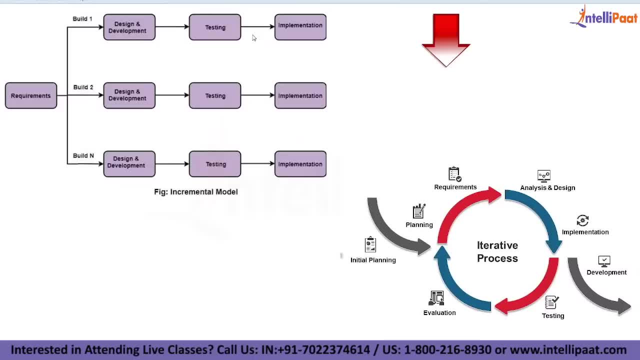 verification process: either we get a password, otp number to our registered mobile number so that we have to give so that it will be logged in right. so assume that this is the second way of second step of verification. in terms of the security, this is what generally the customer is playing. 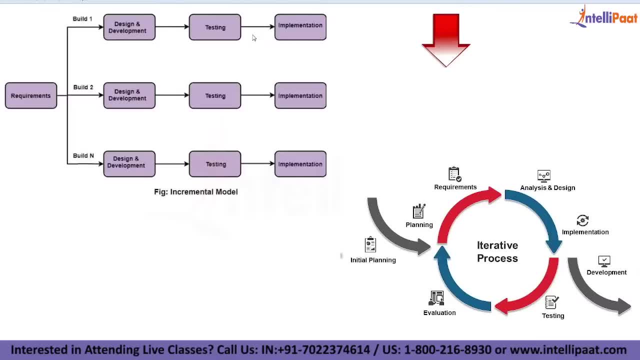 so where are we doing these add-ons, this? we are doing these add-ons and all everything on the second way. it means each and every phase of development phase means, once the implementation, everything done, wherever in the second build, we are adding new, more things into that. this is what generally. 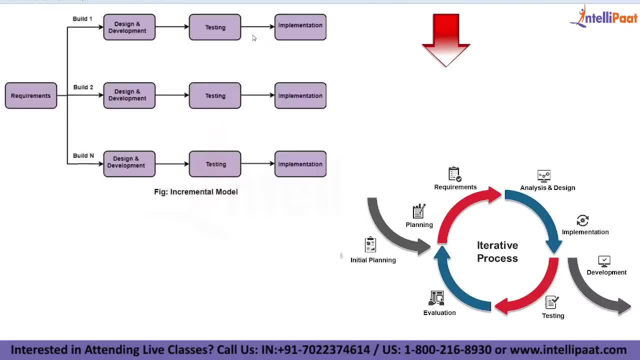 incremental stands for means each and every phase of implementation. we are adding new increments into the existing ones. this is what we call it as incremental model stands for, followed by incremental model. the next is iterative model or iterative process or approach. i can see iterative approach where we are working on something, giving it to the customer as long as customer is not accepting. 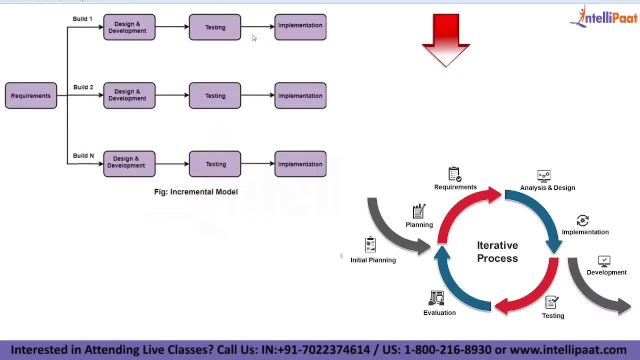 it, we don't go to the next level. this is what iterative process means. we are providing more value services to the customer by adding some new things, doing some changes and all everything into that right. so this is how generally iterative processes. so these are the traditional ones. 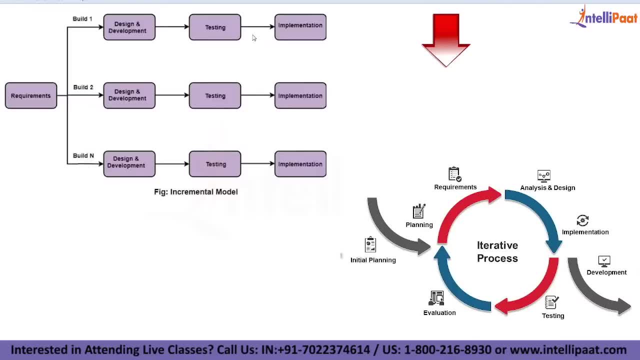 whatever we have discussed so far, either it is a waterfall model, or it may be a v model, or it is incremental or iterative. all these processes are the traditional ones. traditional ones which we are using for a very long time now, due to the changes in volatility and requirement. 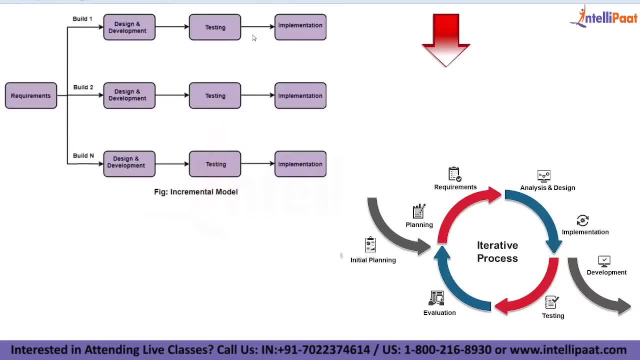 taken place nowadays, because nowadays, as you know, any enterprise, especially everything, is competitive, right. so, whatever the services they are providing today may not be by tomorrow, right. so tomorrow they have to come up with a new thing. this is how the market and industry has changed, evolved, so we have to run along with that right. so then, then, only existency will be there, for 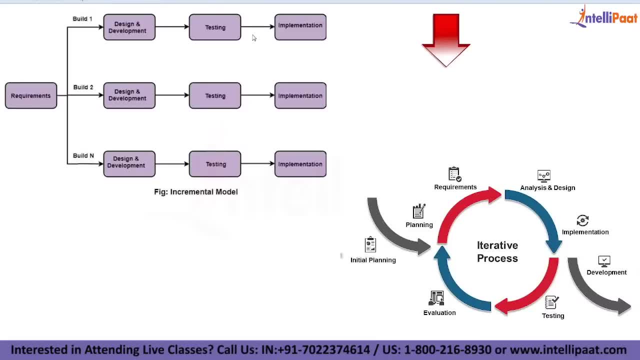 any enterprise- so customer- requires lot of changes to be made into the existing one sometimes, or else they may require to add some new things and all everything into the existing ones, or else to develop a new application or a new technology they want to implement. so this is a continuous process for any enterprise. nowadays they are expecting, means they are. 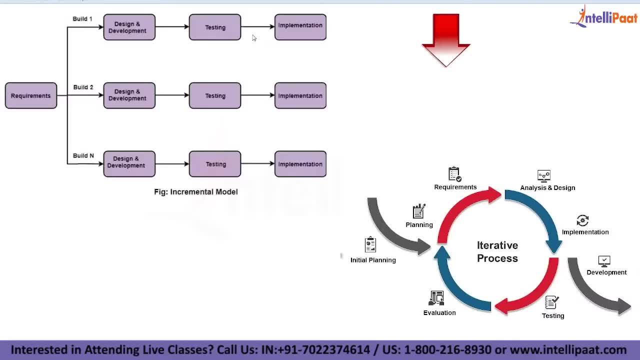 expecting an application to be completed in very less time. that to a quality out, because quality they don't want to compromise, but they want things to be completed within less time. but the practical difficulty is, as it's, a human intervention because, end of the day, whatever the coding we do, whatever the testing that design part diagrams, we prepare architecture. 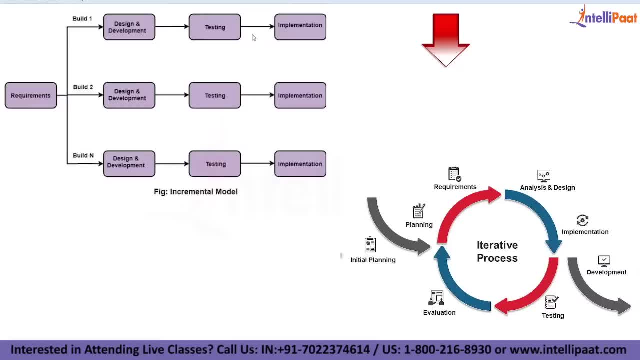 everything is being connecting with human right. manpower. people has to do it, it's not by robots, remember. so human intervention is involved. more so, there will be some desired timelines which are essentially required for us to complete, but unfortunately, some people- customers- doesn't have the time to wait due to multiple reasons. maybe they have their own reasons for that. so there are. 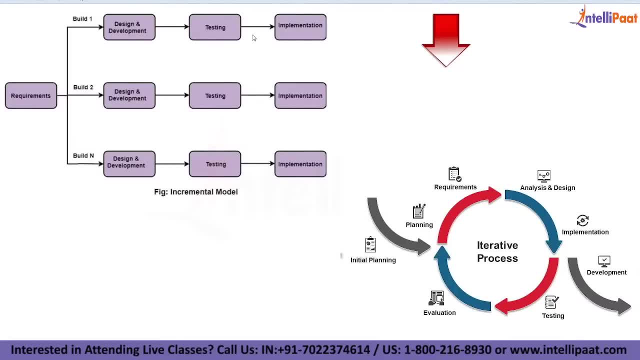 possibilities that they may not have that much time to wait, that extent possible. so they require several booking forms through Protigein. so once you have that procedure through Protigein, people smoothly go for it. once you have that single food that you announced, as always lifting off with many проблемatizing things and the audience just keeps well. 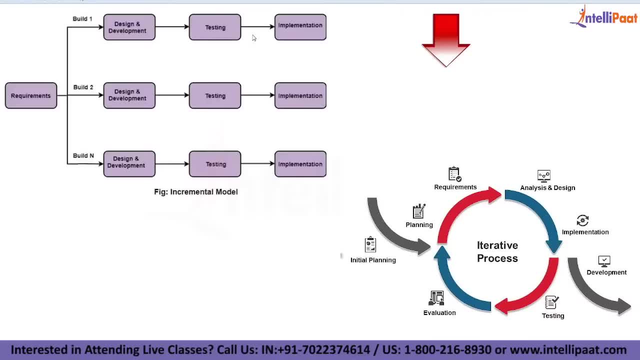 they are already getting some certifications and if there were any artisans going to complete an application in less time, then they are totally going to need to have a production on time. since they are going to report and again, maybe there is an issue- less time remaining- you have to make the distribution firm just in a regular meeting. 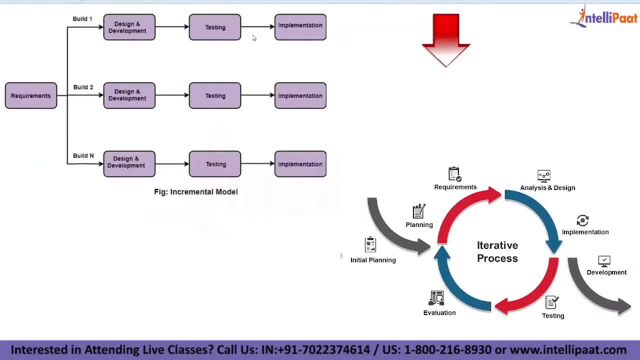 from past eight to ten years, agile was there, of course, in very limited in percentage, not more aggressively, but nowadays, of course, everybody were understood the importance of agile and slowly adoption in their processes is taking place. that's a different story. name anyway, right. so slowly the implementation and as well as the importance of agile has increased. agile is 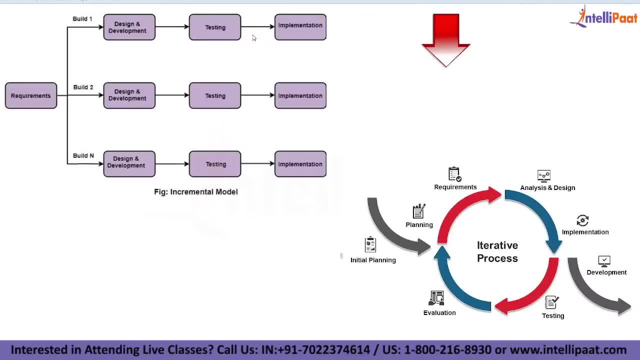 something suitable for the present condition which customers are expecting. that's the reason why importance of agile is more nowadays right. so i'm going to discuss about agile, because whatever we have completed so far about the waterfall v model, incremental iterative- all that we have completed, and now i'm going to discuss about agile. so what is agile is all about? why agile? 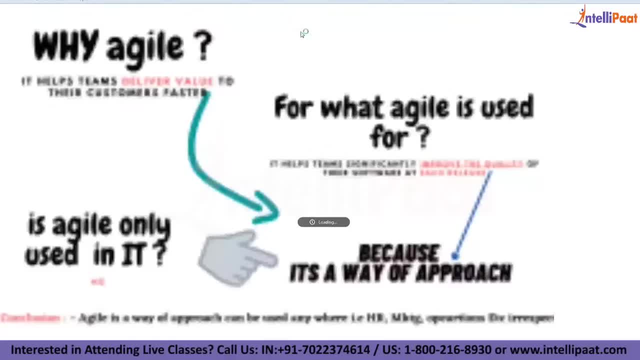 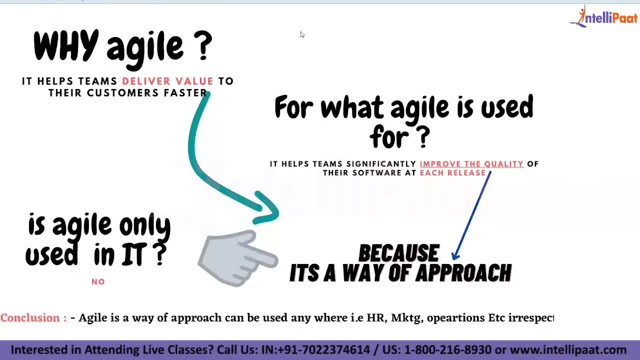 for what reason we are using agile all that? so this is: these are the three different points we need to discuss here. the first point is: why agile, for what reason agile is. second point: for what agile is being used for? and the third: is it agile agile is being used for? and the third, is it agile is being used for? and the third: is it agile? 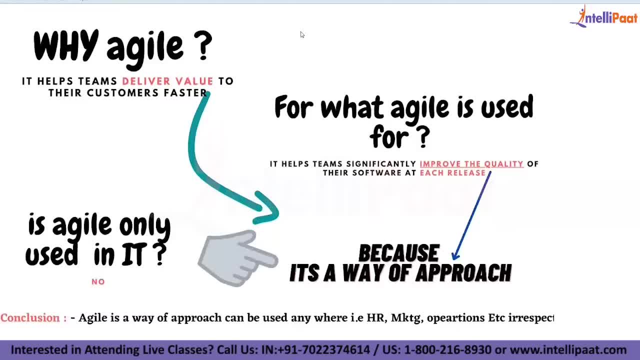 confined only to IT companies, or not, right? these are the three points we need to discuss first. then we go for: what are the different, different values and principles of agile we have followed by this? why Scrum, right. so what is the difference between Scrum and XP? Scrum and Kanban: right, so all that will be. 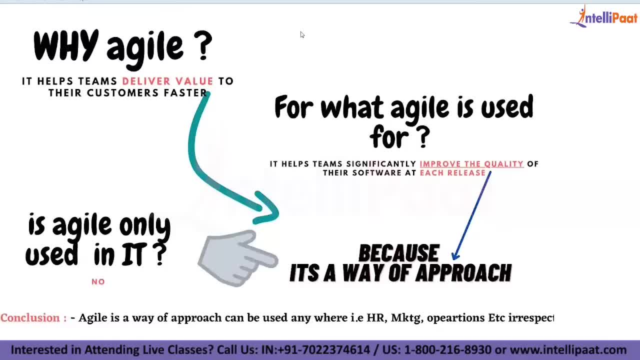 discussed in the later on screen. now let us discuss about why agile- as I told you earlier, customer wants. the project has to be. whatever the solution- let us understand from the perspective of a solution- has to be completed in very less time. that to delivery should have a value. quality delivery has to be done. 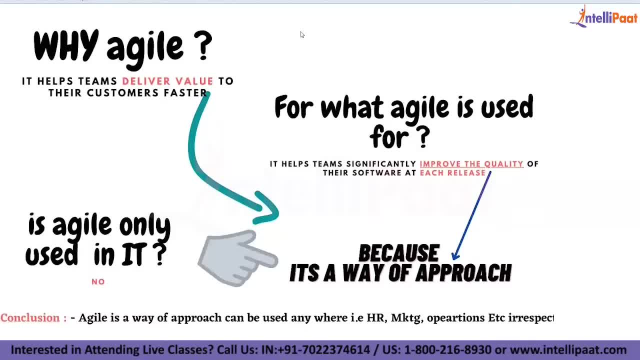 for that reason, agile is being used in application development. nowadays means whatever the requirement customer is having, whatever customer is expecting us to complete, we are completing in very less time and we are delivering it to the extent possible, whatever the quality we can provide to the client. but the 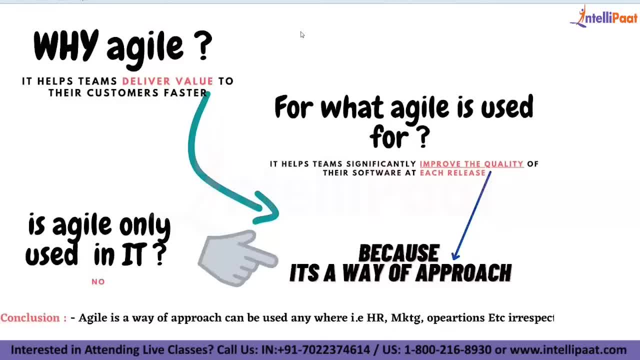 advantage in agile is: whatever the implementation we do, whatever the release we do, everything is under small iterations. because in agile we do small iterations assume that, for example, to have a clear and simple understanding and then to complete a project called a core banking. let us understand: a core banking is an application we are developing right from 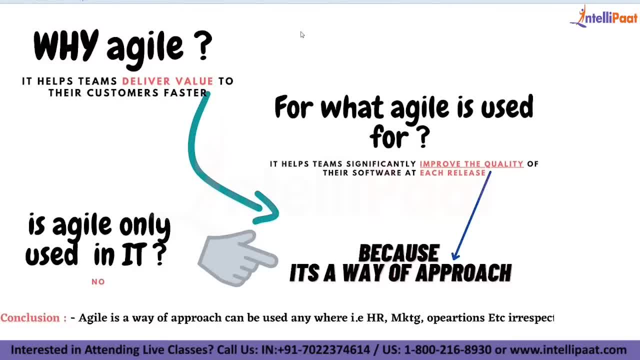 analysis to deployment, delivery, followed by followed till delivery. assume that it takes to 12 months time for you to complete. now, what is that we are doing? we are dividing it is to make you simple and giving this example making it more simple. so what is that we can do? we can divide into three different parts every. 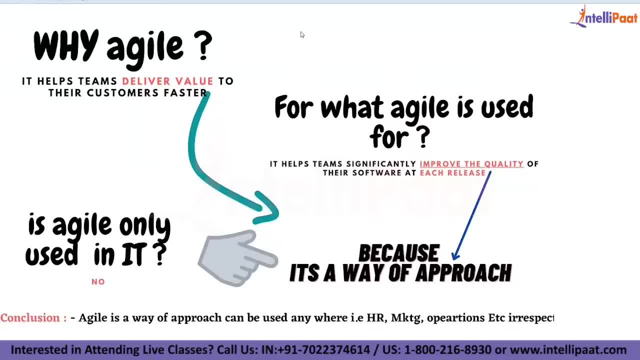 three months there is a release, or every three months there is a release. hence there will be four different releases. so four threes are twelve, or three into four, twelve, right, this is how it is. so every three months there is a release we are planning, or every four months we are planning a release, whatever. 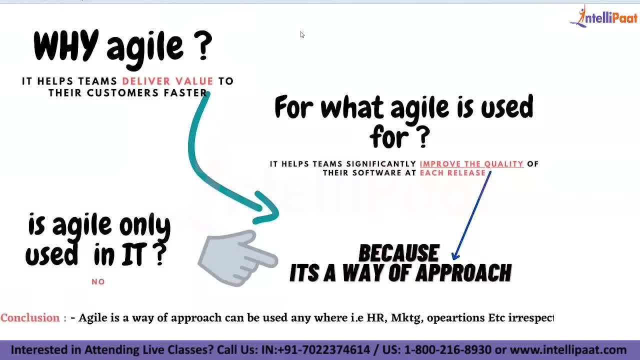 is required for the particular release is what the parameter. hence we are not focusing on the whole application. the advantage in agile is especially in reference to the team. I am saying whoever is involving in agile. they need not be focusing on the whole application, so their focus must be only for the particular 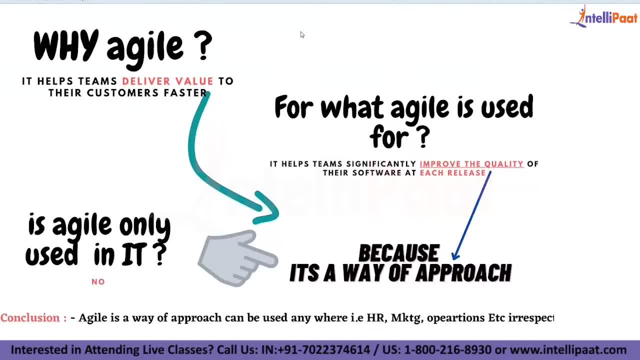 type timeline which is somewhere around near to about three to four months of time. let's assume that if it is three months time of release, whatever is required in the first coming three months is what the plan of action team will be focused more on. so once it is done, then, and next again, we plan for the 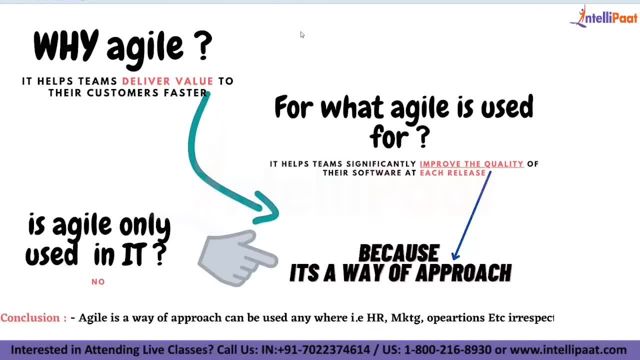 second release. third release for reason right. this is how generally, the process will happen, so this is possible. then we want to implement agile because the structure, as well as the value system which vigil is having whatever the principle and as well as the structure, of agile is something suitable to that. 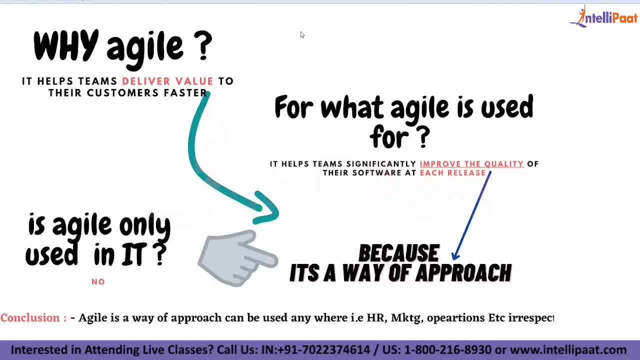 one advantage at the same time. the other advantage is that if there is any kind of changes to be made in between- because in the beginning itself i told you, volatility requirements will be more, because whatever the offer, whatever the changes and whatever the process they were implementing or whatever the strategy they were implementing today may be outdated for the next couple of days. 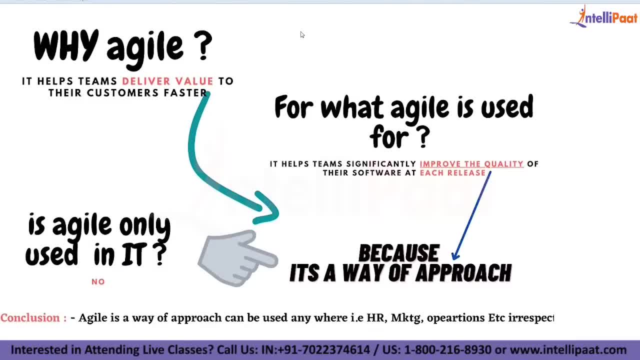 sometimes, due to the different, different domains, it varies, so there is a constant changes on the existing requirements which might be taken required in between. this is not possible- something in the traditional way of approach- because every requirement is being: whatever the functional and non-functional requirements we are developing, everything was interconnected. 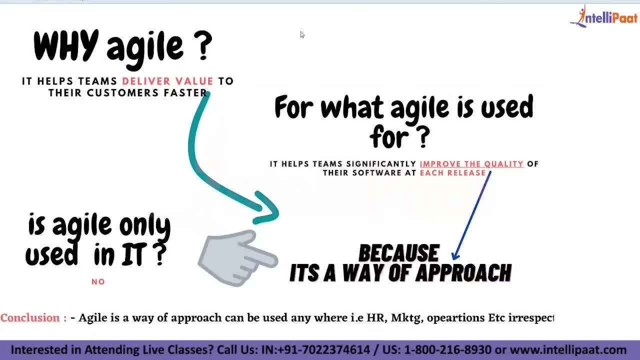 at the same time, whatever the requirements we are writing, everything will be written in a documentation format and we are implementing the same, the same way as this, but whereas in agile the approach of writing down the requirements and all everything in a different format. that is how generally user story- we call it as user story format it is. 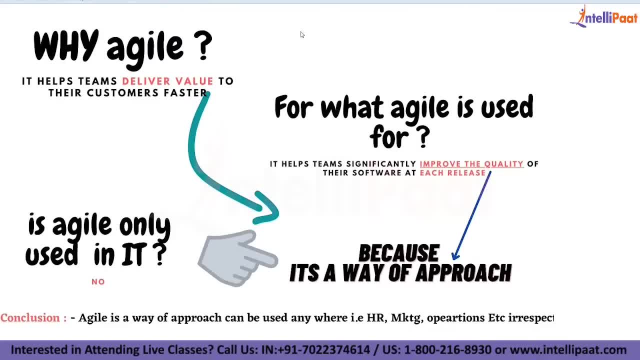 means each in every user story is having independent on its nature, so that there is no connect with other user story, so that whatever the implementation, whatever the changes we want to make out of it, can be changed accordingly, so that this is how generally, one example- i'm saying so. these are the ways where 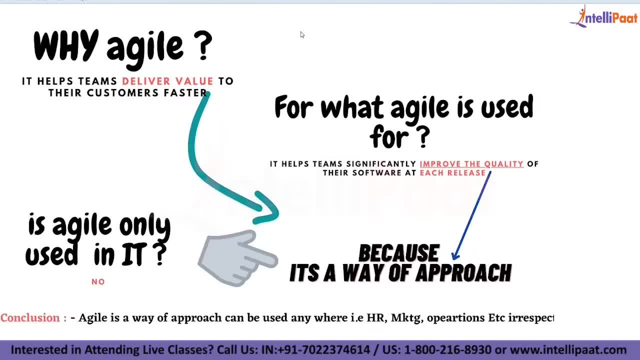 agile is more extensively using nowadays in implementation of the projects. so this explanation i am giving you, irrespective of technology in the domain. i am saying this in reference to the it projects. now the third question, important question for most of the people who are from non-it should. 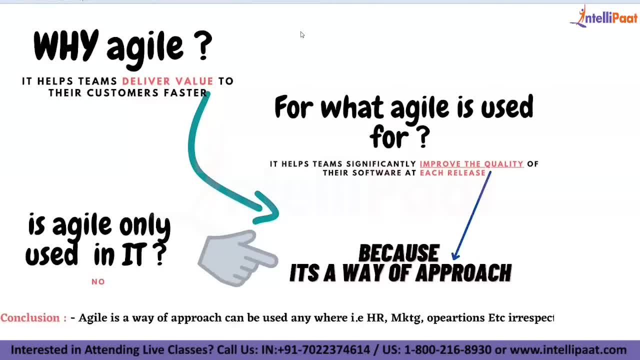 understand this. is this agile way of approach or agile methodology or a process? whatever we say, is it something relating only for it organizations, or is it relating to other? as see, agile provides you delivery for the value, value for the delivery, right. so whatever the delivery we are delivery of, 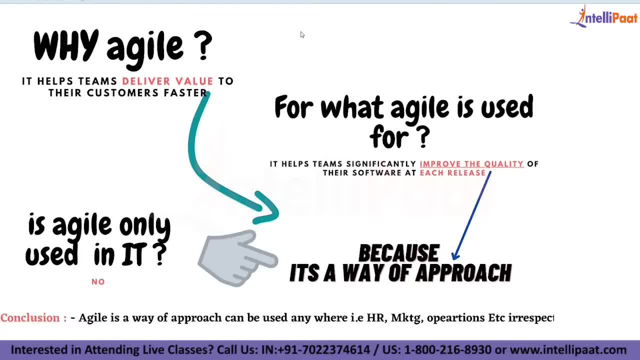 work we are providing, we are giving it to the client. it should have a value, should have a quality. that is what generally the aim of agile, so this can be incorporated anywhere. this is need not be for it, because the whereas we are working on it, projects, development- we are talking about agile for. 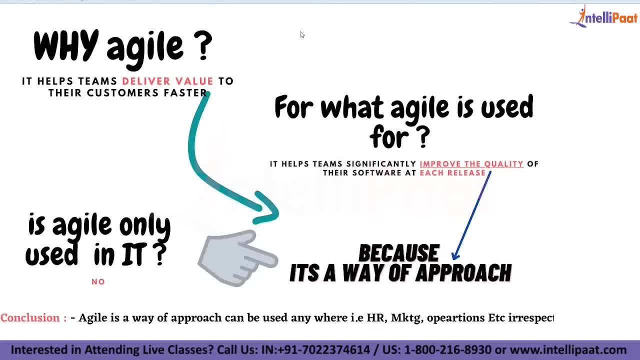 example, when you are working on operation, sector right, operations to mine cooperation side for any of the organization in order to streamline our processes and all agile agile can be incorporated now, for example, healthcare: in process of healthcare, agile can be incorporated. even in hr, agile can be incorporated. even in sales and marketing agile can be incorporated. so agile can be incorporated. 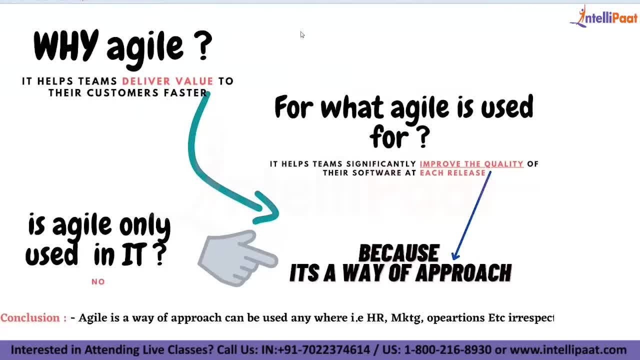 is a way of approach where you can provide a quality of services to the customer in phase wise, within the limited time. that is what the approach of agile is. so agile is not something confined only for it: project development. agile is useful everywhere because there is a connect here. 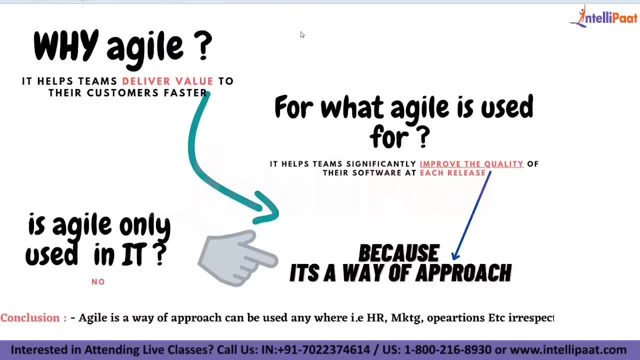 because every process, whatever process we follow, for any organization, everything is connecting to it. without technology, nothing right. so, for example, if you want to manage your customers and all, we have an application called crm customer relationship management we are using. you want to integrate all the departments, all the processes, all that, we have an application called 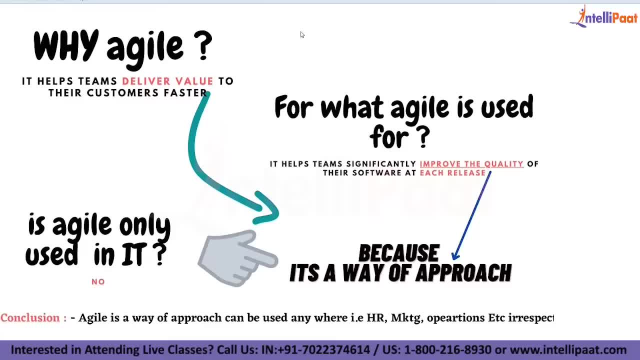 erp, where you are connecting with different, different departments to streamline your business process. all that stuff right, so even production, all that can be incorporated if you want to manage your employees, their payroll and all that payroll management system to manage back-end operations of a bank. they're using core banking, so every organization to manage their. 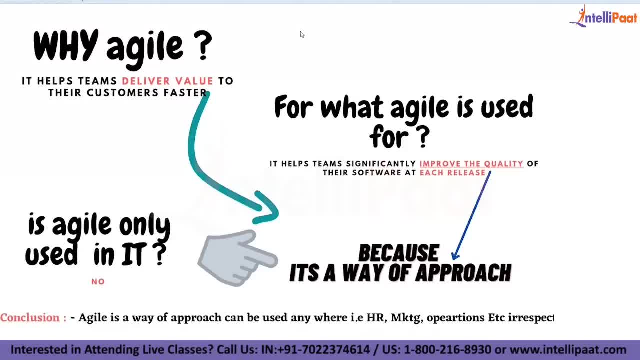 operations, business operations. technology has became an integral part of it. so understanding it, incorporating it has became has became inevitable in every organization and every process, even hr marketing operations everywhere. so agile has a connect to that extent. so agile is not something relating to it companies because it process is involved even in non-it also. right even, you can take any. 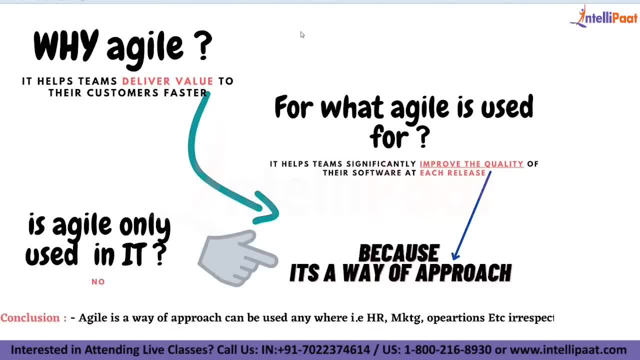 healthcare organization or a retail or a banking insurance, all that stuff. everywhere it is involved in the process they were following. everything is connecting to the machine, technology, it all that, hence agile, can be used anyway. right, this is the introduction about agile. so why is it? for what? 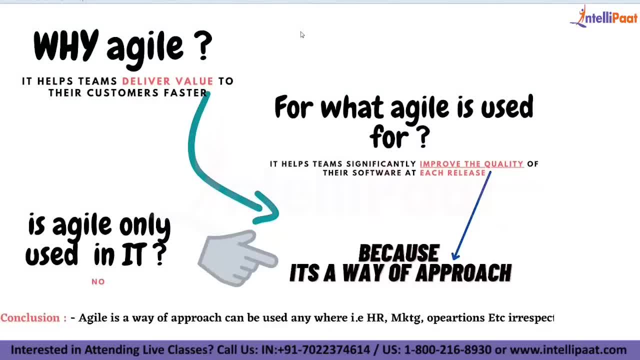 reason agile being used for. so is it agile is only used only for it or not? yes, it's not. no, it is no because agile is not completely to it: organizations, companies, even agile can be incorporated, even in non-80 also. so this is all about the introduction about agile at the same time comparing this with 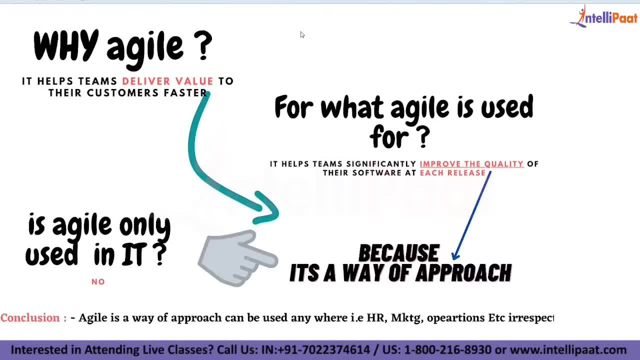 the traditional models we are using for the process they were following. everything is connecting to the role development, so the focus is on the apk events and we were referring to no-it. so we are using this to think of, to develop the project. we are now exploring the future we're well aware of. 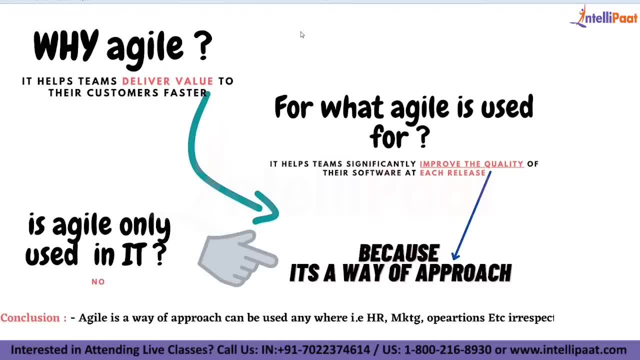 how agile can be developed for all time. so whatever the focus we do now is completely into it. project development not relating to non-it, subject to terms and conditions. this is what generally we have to, so our focus will be majorly to agile, towards it. this is what generally our focus is. 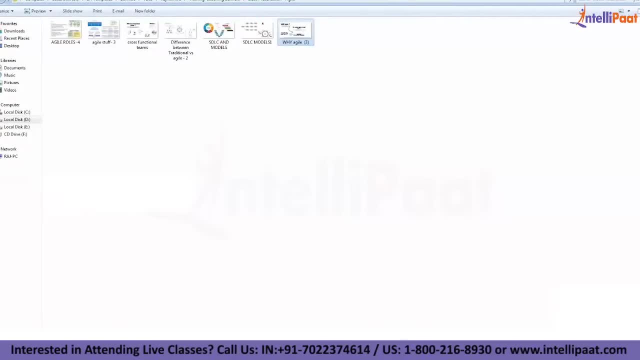 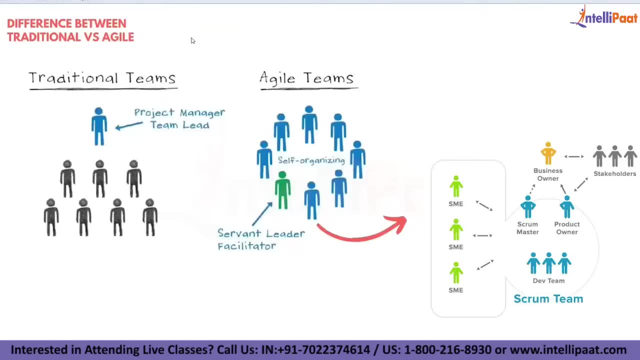 so this is what, whatever i have given so far about the introduction, about hr, it now, right now, i'm going- This is what you must be knowing first, before I'm going for AJR, values, principles, or else before I'm going for Scrum- 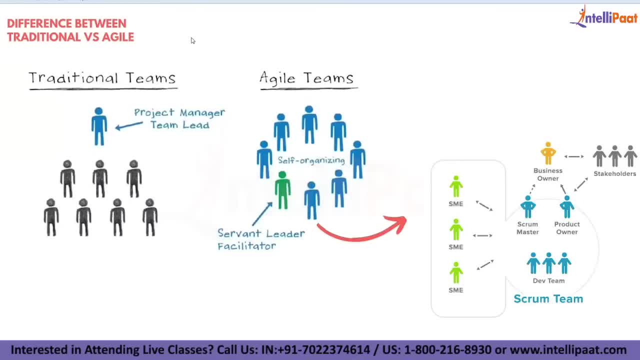 So if you'd like to know about all that. So, first of all, let us understand the difference between the teams. when we are comparing from traditional to AJR, This is what the comparison is. One more difference which you need to understand is this: 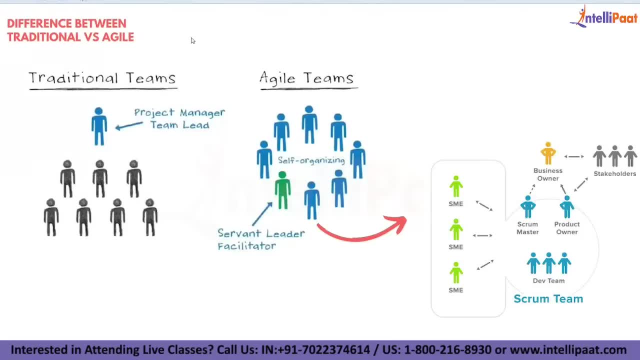 Because if you take a traditional team, let's say we are using waterfall model or V model, whichever the model are we using- When you take traditional teams into consideration, there are a lot of people will be involved. The major difference between traditional to AJR. 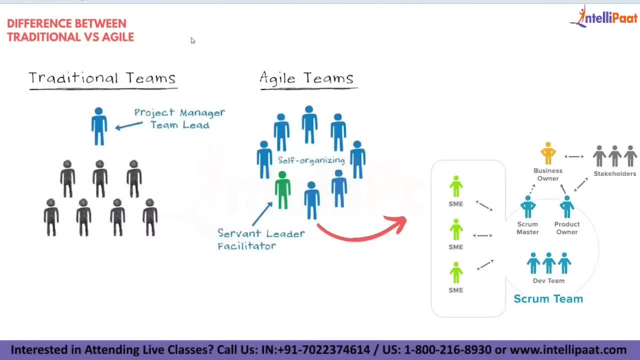 A lot of people will be involved in it, right, You'll be having a project manager who will be taking care of project planning, budgeting, all that stuff. You have architects. These people will be involved in developing architecture for the project. 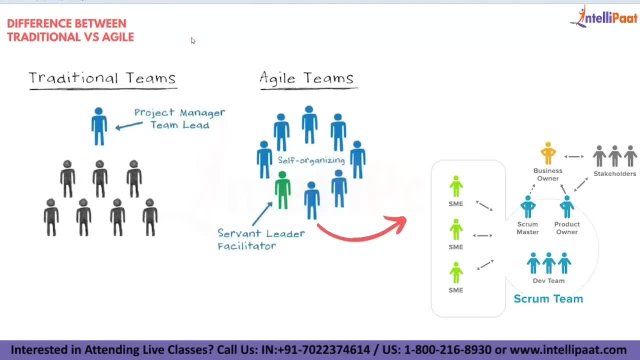 At the same time, you have development team, technical testing team, user interface designers, documentation team, business analyst. So these many people. So, if you want to Develop an application or if you are providing solutions for one customer, at least minimum to minimum 20 to 30 people required for you to complete the whole thing. 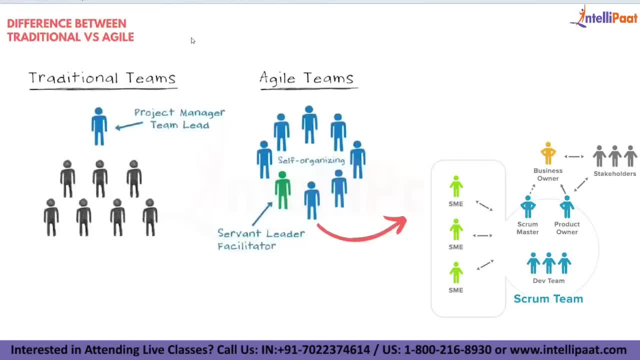 Why? Because project manager is the one who is exclusively focusing more on project planning. Business analyst takes care of business requirements. Architect takes care of architecture of the project. Remaining implementation teams take care of coding testing. all that. This is how generally the traditional teams are. 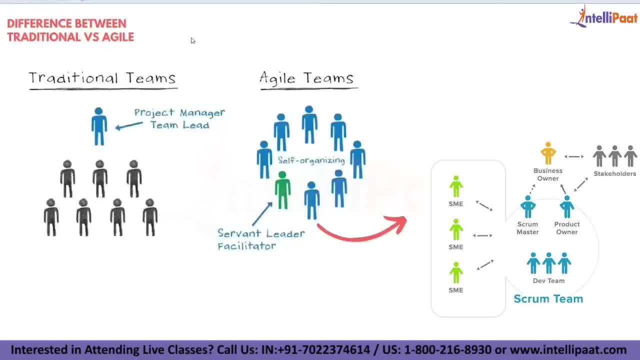 So the team size is very, very big. At the same time, everybody have their own individual responsibilities, So the focus is Only on the responsibility which was given to them. This is what generally traditional teams work. If you are a developer, your responsibilities in whatever the work you do, everything is confined only to your coding part. 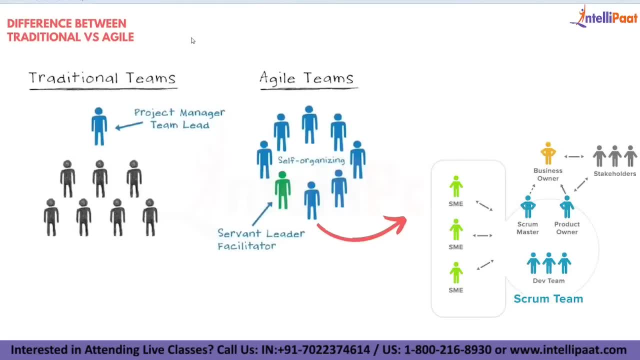 So you don't take care of other things, unless if it is assigned to you, which is compulsory, you do it. Otherwise, end of the day, we don't do it Right. So we are only for the particular work we are belongs to. 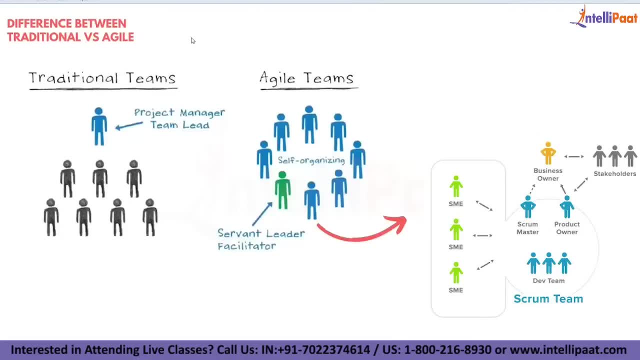 So we do only that part. We don't do anything else apart. That is what generally traditional teams works, But whereas when you're comparing traditional teams- Traditional to Agile- Agile has a different approach. Agile is a self-organizing team. 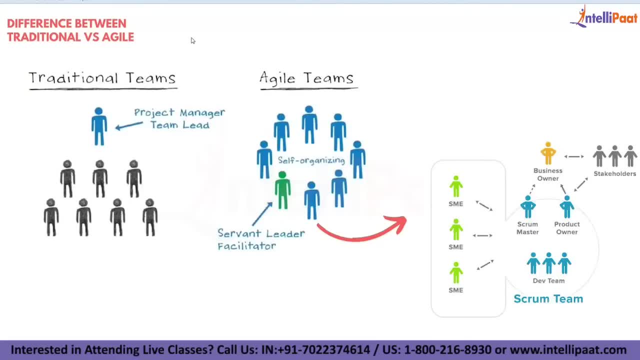 Self-organizing team means: whatever the decision, whatever the implementation they are doing, what are the decisions they are taking? Everything is self-organized means companies and organizations making everyone accountable on the deeds or the work, what they are working on. Because in traditional way, if you are taking project manager, project manager is the responsible to complete the project on time. 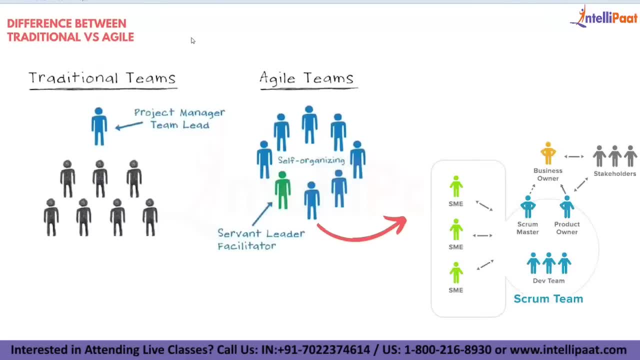 Right, Normally project manager is The responsibility only for the whole project, whereas the same responsibility- you don't see that- to the developer, because developer is only responsible for the work which was assigned to them. So once the coding is complete enough, so they don't go for anything else apart. 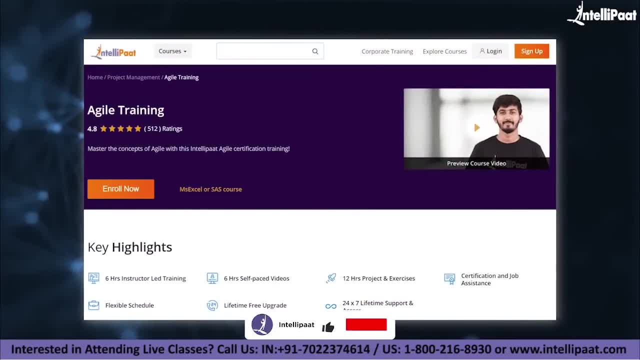 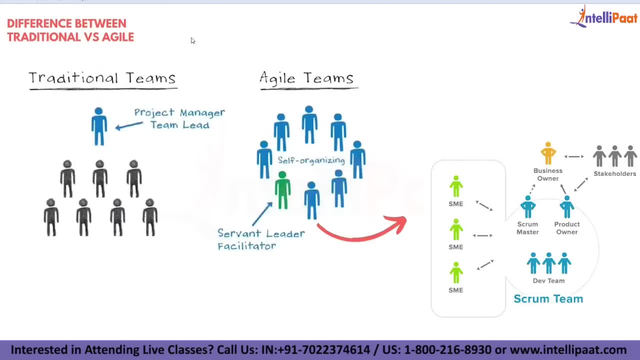 Just a quick info, guys. Intellipaat provides Agile training mentored by industry experts, the course link of which is given in the description below. Now let's continue with the session. But whereas when it comes to Agile environment, that is not something, because the major difference is this: because in Agile, the advantage in Agile- underline point- because, being in this organization industry for a very long time, as I could see closely, I could see and I'm interacting with a lot of entrepreneurs, business owners, when I'm transforming the teams, all that. 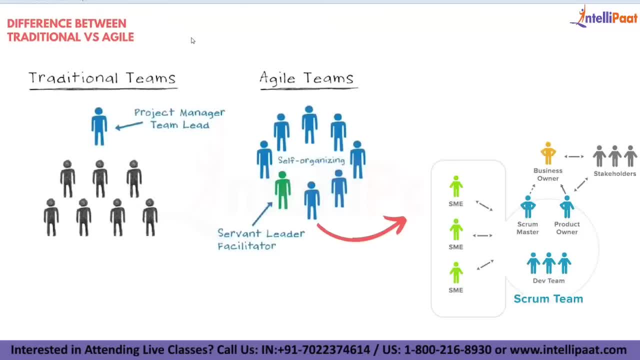 So what I closely observed is Agile implementation, not only for quality of services, providing all that stuff, we should also. They want to make each and everybody accountable for the deeds, what they are doing, so they are making everybody accountable. So when there is an accountability, there is a responsibility will be there right. 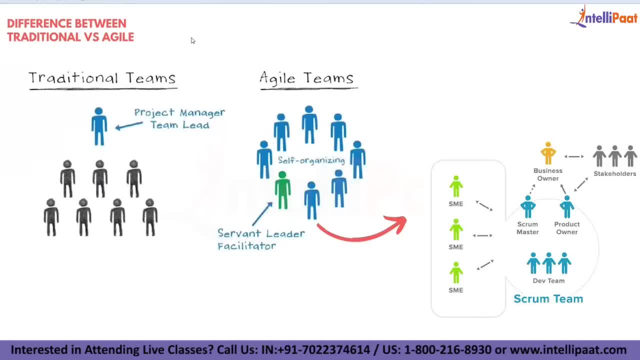 So responsibility and accountability were interconnected. so they want to make each and everyone interconnected and responsible to one another. That's the reason why this is all a self-organizing team. This is what we call it: a self-organizing team, where it is being connected, interconnected, self-organizing, nothing but interconnected. 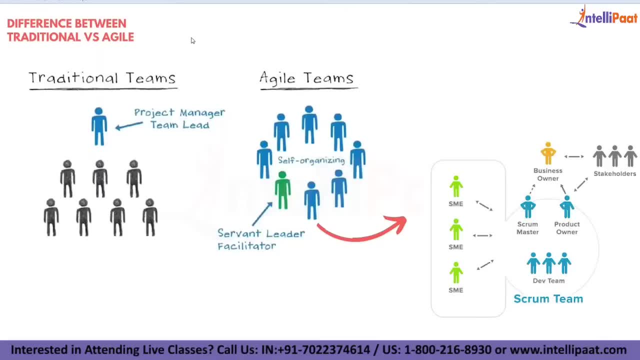 So it is all interconnected. So, whatever the work we do, everything was interconnected. Self-organizing teams are interconnected, So each and every person who is working in Agile environment is responsible for each and every deed which is happening Means if you are a developer, you cannot claim yourself that you will be only for developing. 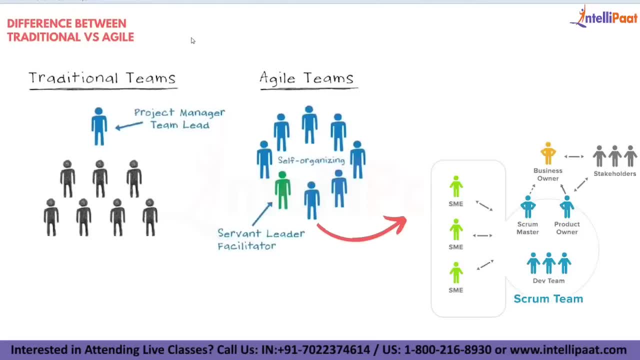 Even though work allotment, when given to you, if there is someone is absent, the other team members has to complete that work within the limited timelines, because Agile is completely into short iterations and specific timeline, So there must be. If one motor is working for Agile, then team effort right. 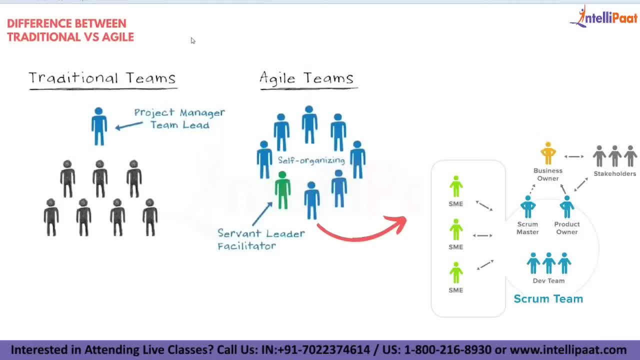 Team management, team coordination, team effectiveness is important, Then only that agile way of approaches successful, otherwise not. That's the reason why there is a difference between that. We are working in Agile environment. that and as well as working effectively in agile. 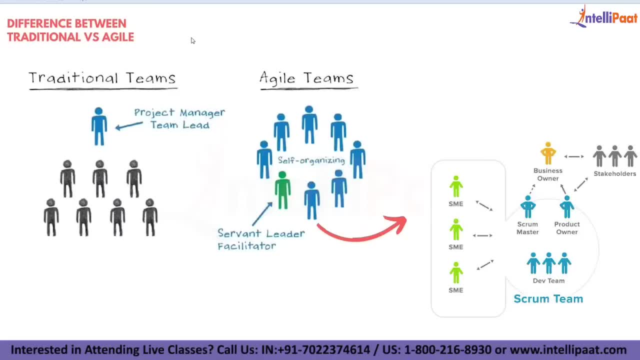 Because there is. there are two differences, because most of the people say that we are working for Agile environment. People say that we are working on Agile environment But, practically speaking, when we talk about this, When we talk about this 100%, are they implementing? agile is a million-dollar question. 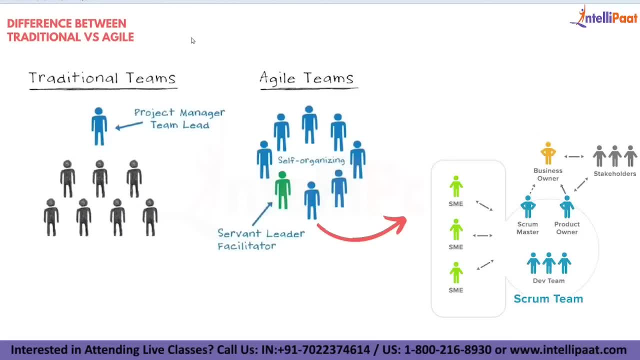 because there are a lot of parameters to take into consideration. One: they must be having prior experience to implement agile right. If not, they need to hire someone or they have to provide some training to someone and they need to start implementing. But when there is an implementation taking place, 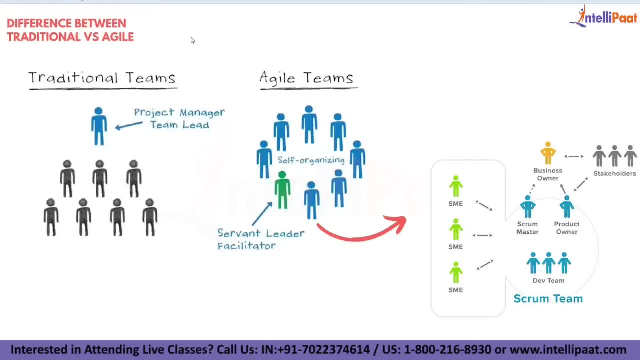 majorly, especially in agile. based on, out of my experience, what I have seen is what they have understood, is what we call it as agile. This is how generally few people- of course I am not generalizing this point- for every organization, every team on that. 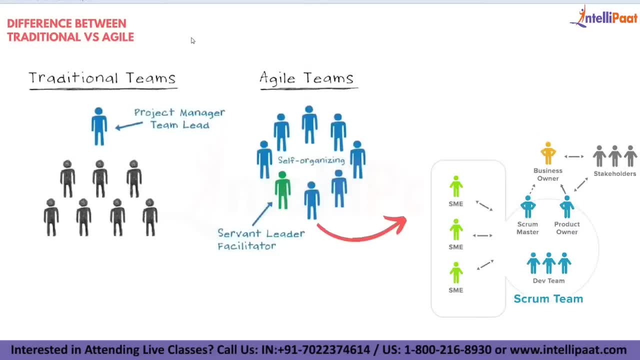 But most of the teams feel whatever they have understood is what the mod approaches. right. This is how generally they are. This is because of ignorance, not by intention. This is because of ignorance. Whatever they understood, the way how they understood, this is what generally agile. 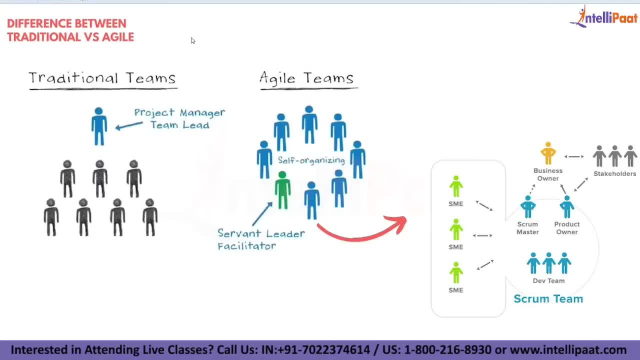 So this is how people, most of the people, feel. That's the reason why 100% agile implementation is not happening for a long time: All the projects. the reason why, even though we say agile 100%, they don't go for agile way, because agile way of approach have different. 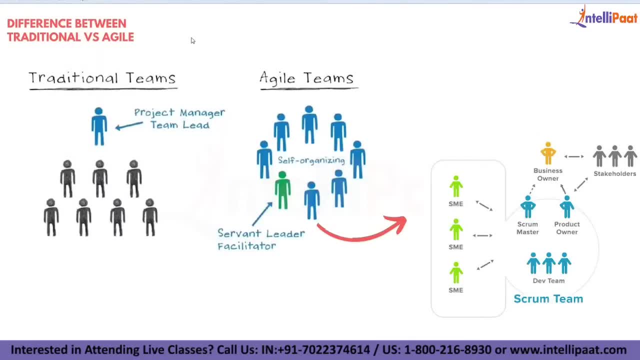 different values, principles which everybody must be a bite to. that That's it Underline. what they do is that they say agile, practical. these are the practical things. because, on a note of understanding about agile, we say so many, but in 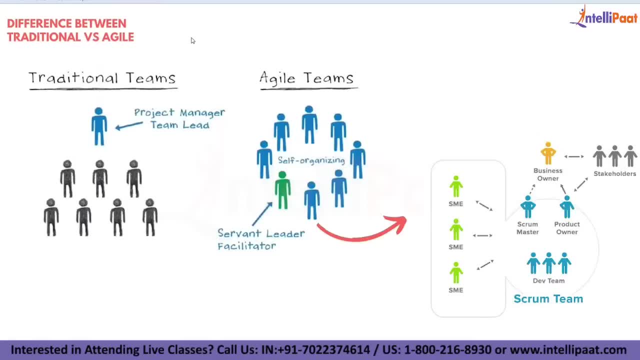 practical reality. a hundred percent agile are they implementing? No, because agile combination of traditional models will also be incorporated. because, due to the comfort, Because they are the kids First off, it's kind they're implementing. They want to make. they don't want to make it so confused, right? 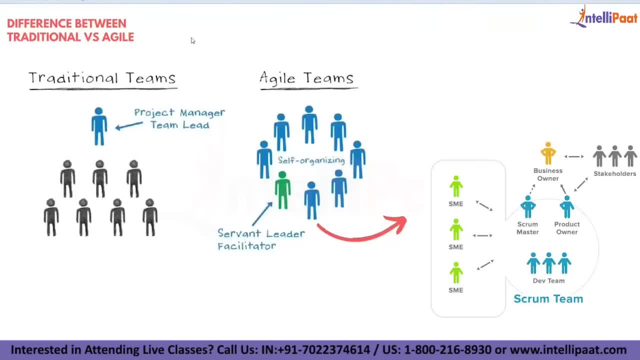 So they don't want to make it more troublesome when they're implementing. So what is that? they do A hundred percent. they don't follow a giant agile. They follow to some extent when there is a difficulty they have understood So far, they go for traditional model and the traditional approaches will be used. 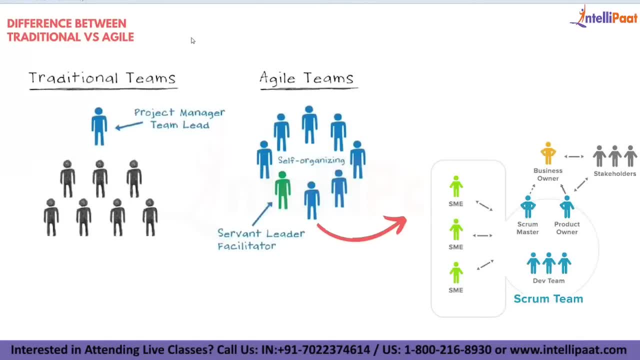 End of the day, What is important? We need to deliver according to the timelines, what customer has given right. So that is the ultimate model. but they have Started with the intention of implementing agile, but a hundred percent is agile implementation. 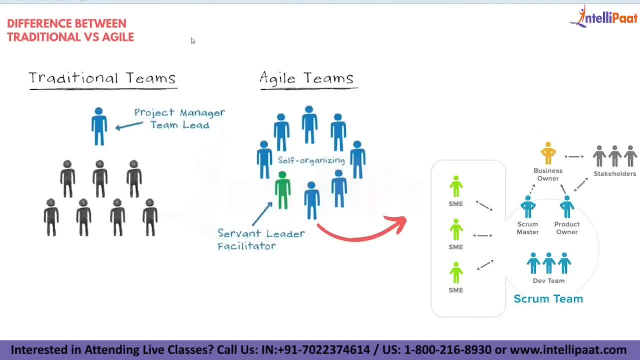 I don't say it is not possible. It is difficult because we have to travel. All the people should adopt. All the people has to understand what is that we are doing, How are we doing? And agent, everybody has to understand the value systems, principles and they have to. 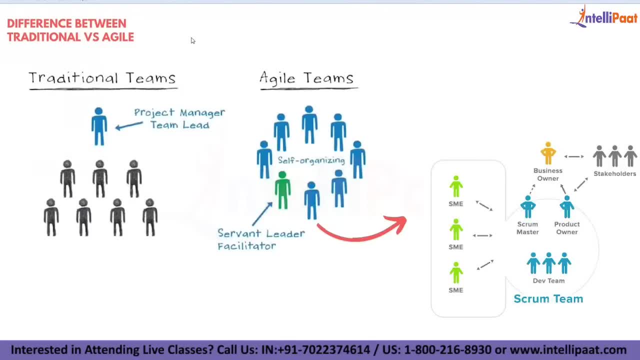 follow that accordingly for a very long time, As long as the team working on it- everybody has to do it at the same time. It's all about mindset. Agile is all about mindset, Where mindset normally human is. that I don't want to give my credit. 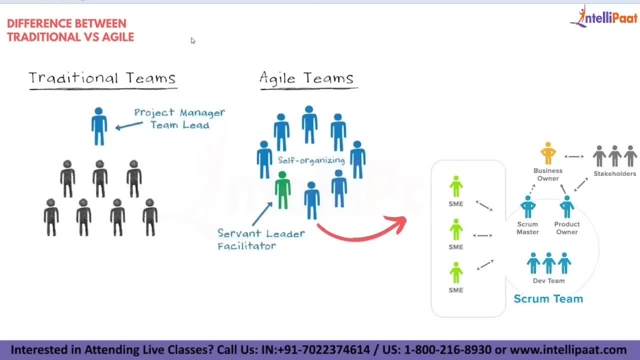 I don't want to share my credit with others. So this is a human nature, nothing wrong in it. but whereas in agile it doesn't. it doesn't work so right. So no individual responsibility or no individual capacity or performances will be taking into. 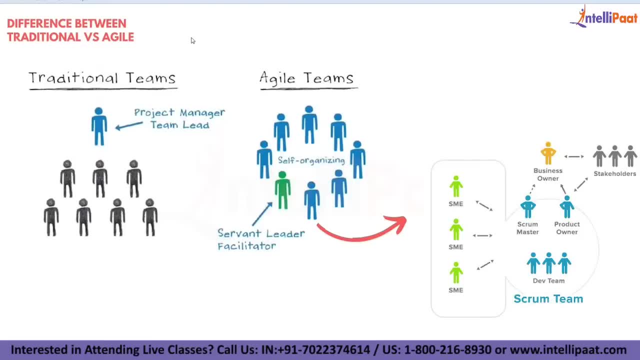 account or configuration. End of the day, it is all about team effort and team success. That is what generally agile tells you. agile never tells you that no individual responsibility will be recognized. Agile never, never increases And of the day, it's all team effort and whatever the success or a failure will be. 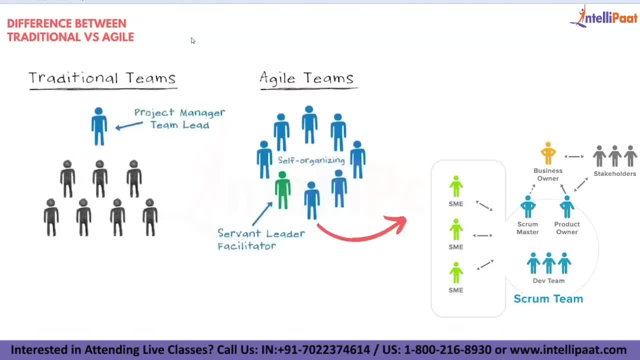 applicable for every team member, So self-organizing. self-organizing means people who are working under the team are self-organized people, whatever the analysis they do, whatever the planning and design, interacting with the client, understanding the requirements, taking up the decisions to work on something. 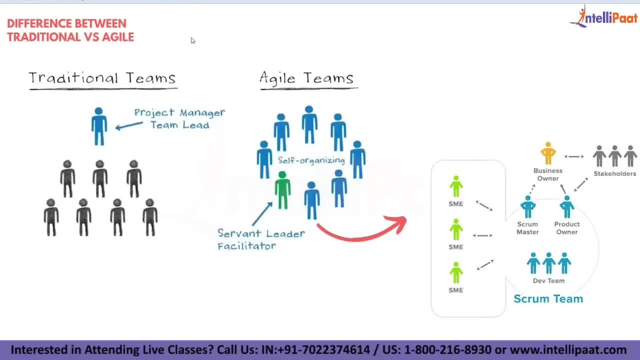 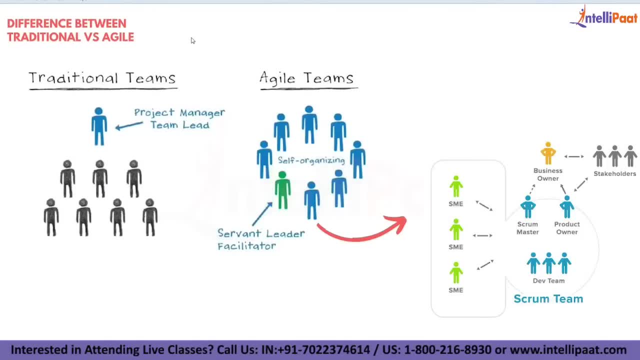 I can say, I can say roughly, we will be having not more than 10 members, right? One team, if you say one team, one team consists of 10 people. right, This is how generally the team sizes, but whereas in traditional teams it's not like. 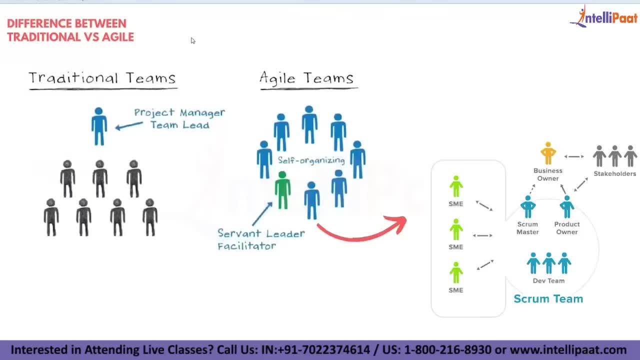 it may go up to 20, 30 people total right One project manager, maybe two, three business analysts, maybe one or two architects. right One major one and other next level architects will be there Database designing. you may be having other people development team, couple of developers. 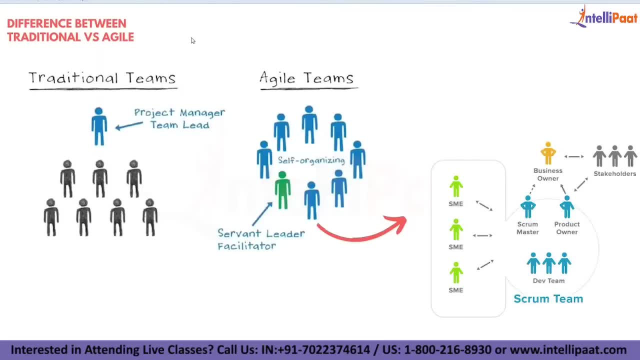 couple of testing testers, couple of user interface, his designers, even for documentation, will be having a separate person. this is how generally the traditional teams will be having, so the team size is also very big. but whereas in agile it's not that. agile is completely confined to the limited people, means only limited people, not 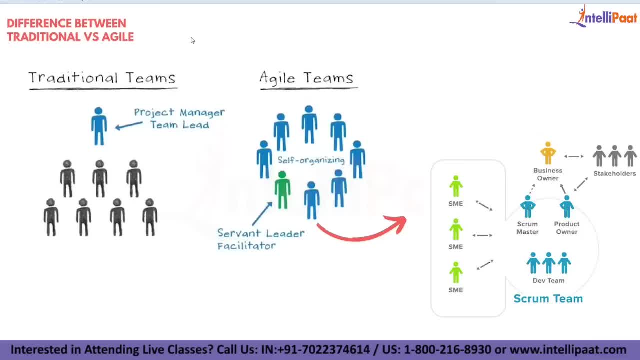 more than 10, so these people has to take care of each and everything. so there will be no other people apart, but here there means there may be an question by someone from you group, from your side. maybe there may be some question. you may arise a question here, raj. is this possible? 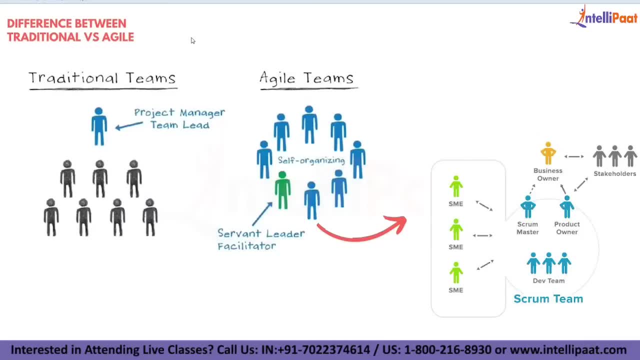 practically to complete the whole thing with the limited of 10 people, right? is it practically viable? because? is it possible? because it's a human intervention. end of the day, people are working, not robots. they cannot work for 24 by 7, right? so is it practically viable and possible? 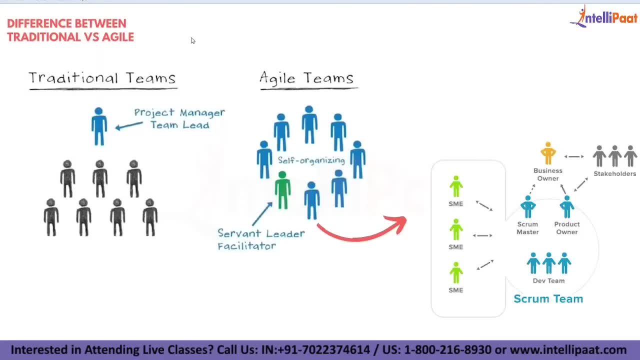 to complete the whole project. let's say, if you can take a core banking project which is taking an year, year and half time, for example, understand, to make it very simple, i'm saying you can take a core banking project which is taking an year, year and half time, for example. 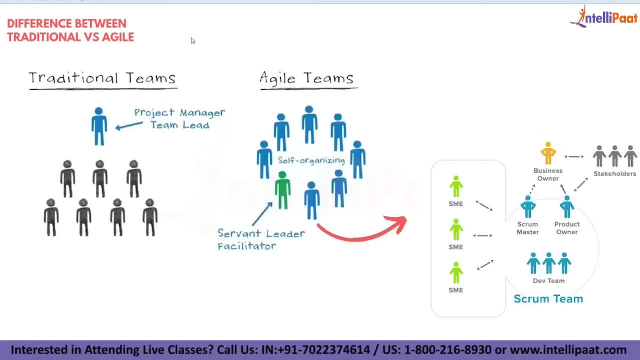 right the whole thing now. is it practically possible? can you expect that the team of 10 people will be completing all these, that too, with standard and strict timelines? because timelines were very clear and very strict, because everything is in weeks normally. whatever we implement, of course, all this comes in the next. so, whatever the implementation, in terms of the 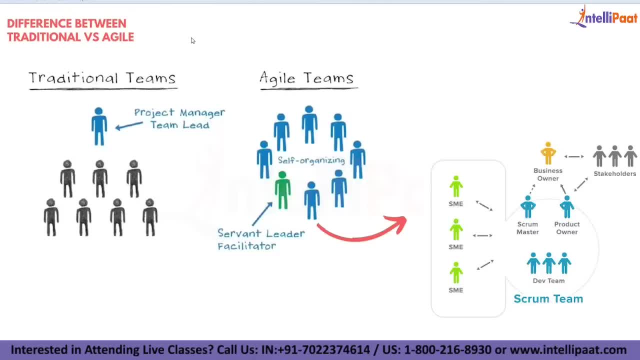 sprint. everything we do, everything is confined only to two weeks, three weeks, four weeks and so on. so the durations were very limited and very tiny in terms of the person, in terms of the size. so do you really feel, is it possible? practically? to some extent, yes, to some extent. no, again, there is. 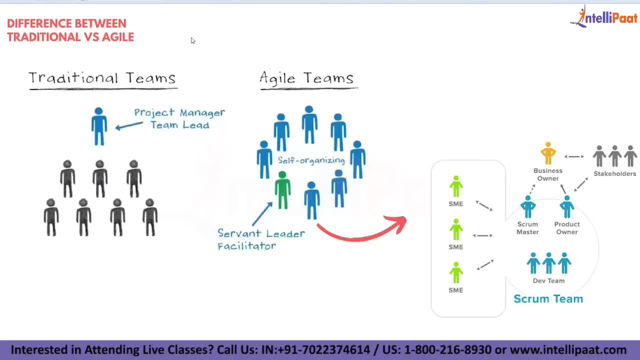 there are two answers: yes, to some extent possible, to some extent no. when it is no. yes when you are going for enterprise level transformation. this is where a concept called a safe- normally we call it a safe- transformation means called a scale design. that's a different story. again that's a different. 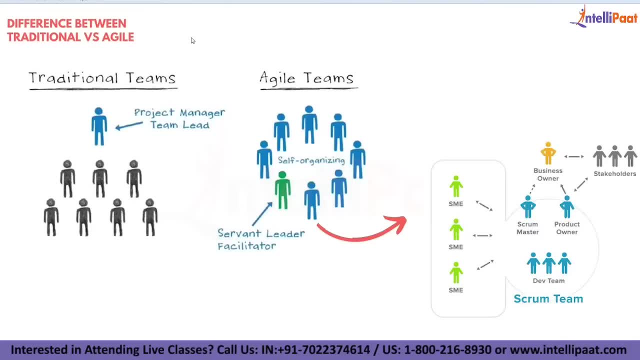 thing where we are transforming the whole organization to the agile environment where you are working for large and complex projects. so that's a different story. again, that's a different. so that time, what is that we require? is we require multiple agile teams in different, different locations working for the same project. whatever the piece of work will be given to you is entirely 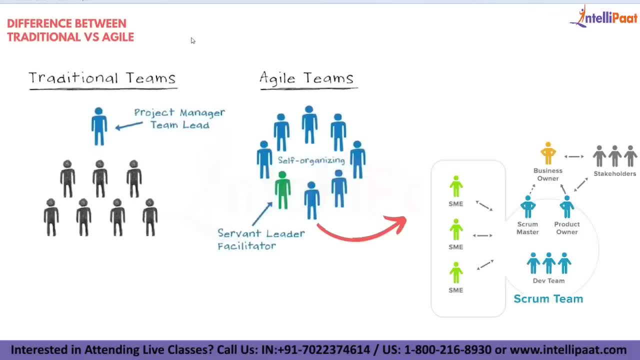 different than other people. that is how the work distribution will be done, but make sure there must be a proper coordination among all these teams to make that application successful in long run. finally, that is a difficult and challenging task, so for that there are different, different principles, for safe will be having. safe principles are there. spotify different, different things are. 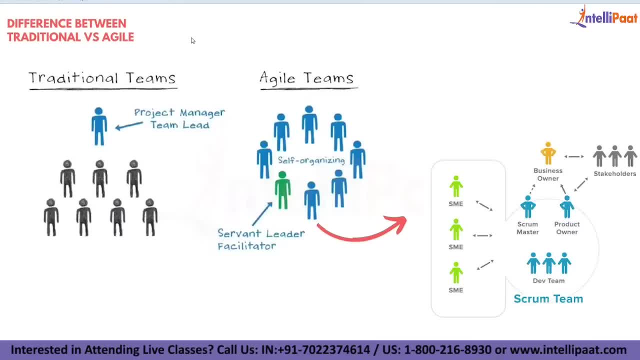 there, so we go to that. so agile is not something that only limited people will work for project. to some extent, yes, because for some projects we do the same for small projects, when there is a limited requirement. all that, yes, we do follow, but not to the full extent, because when we are going for 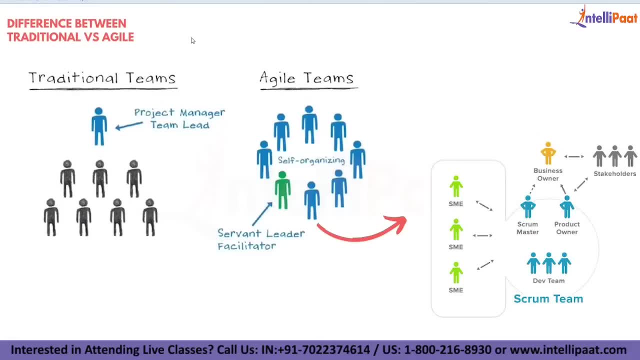 large scale projects where there is lot of complexities in not only the complexity. we don't see only the complexity here, not only the complexity. apart from the complexity, we have to see how big the project is. so based upon that, whatever the team members we have and all, everything will be varied. there are lot of team members are involved, lot. 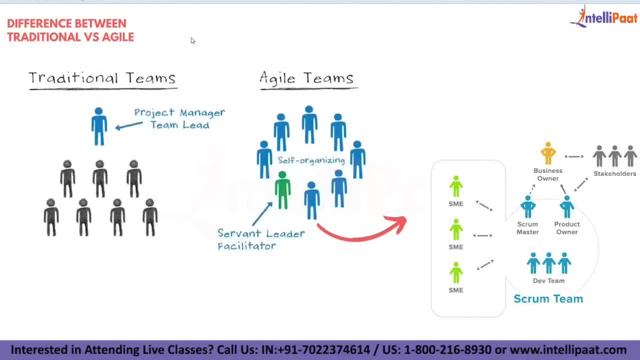 of teams will be involved, not even not a single team. different, different teams will be there right, multiple, three to four teams will be there. there must be a proper coordination with these people in regular intervals. that's what we call it a scrum of scrums. the concept is different, so that is there. 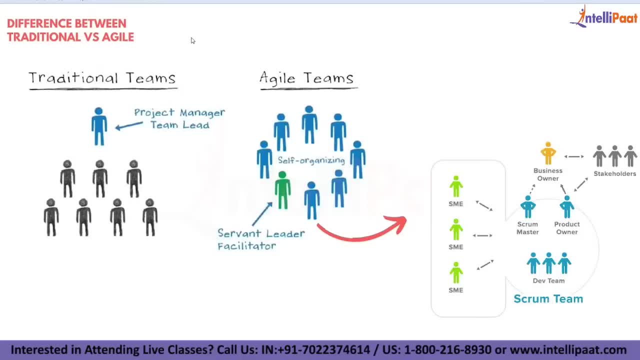 so agile. so what i am trying to say is that agile is a self-organizing team, even though it is limited in terms of the size of the people. on its percentage, hundred percent- agile implementation may not be effective for all the projects. depends on the size of the project, depends on the 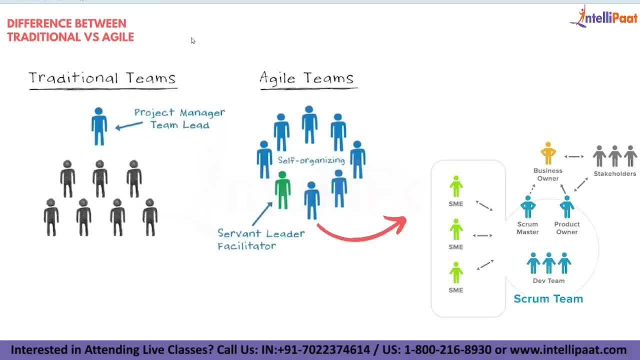 complexity sometimes when you want to transform. the enterprise level means enterprise level transformation means you are transforming the organization to an agile way of approach. so for that there are lot of people required for you. lot of team collaboration is something essentially needed for you to manage, so that is also needed. so different, different things are. 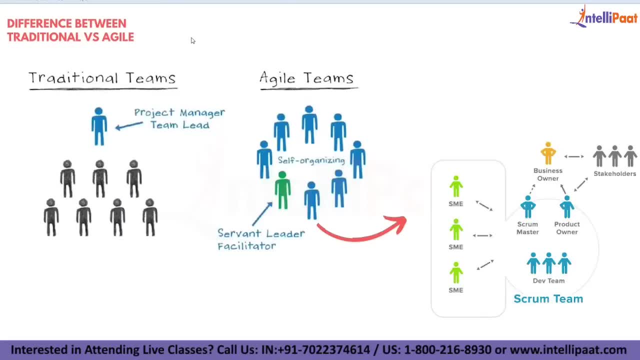 involved in this. so agile is not hundred percent possible. means a single team answer right, not possible for every project. multiple teams also required. so this is the understanding you need to have. so again coming back to our this thing. so this is what generally they see the differences if you can see the traditional team, traditional team members, whoever the members, we 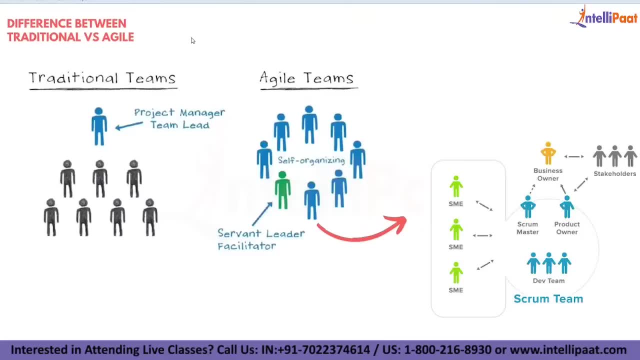 have, and all everything will be different. at the same time, when we talk about agile, agile is something entirely different. it's a self-organizing team where team people will be limited on its percentage, and that, too, agile is role specific. there are different, different roles will be there. 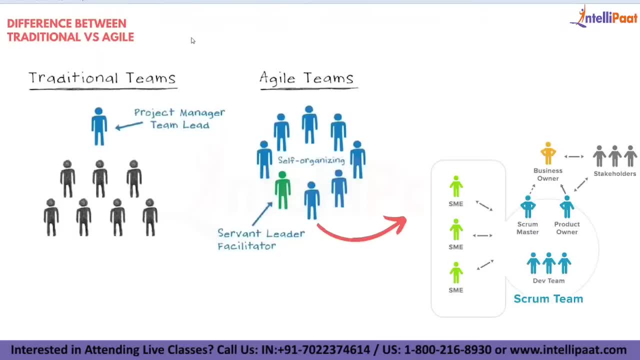 in agile, where different people will be limited on its percentage, and that to agile is role specific, depends on the role. whatever the role will be given to you will be assigned to you. there will be some responsibilities will be given to you as well. so, based upon the roles and responsibilities, 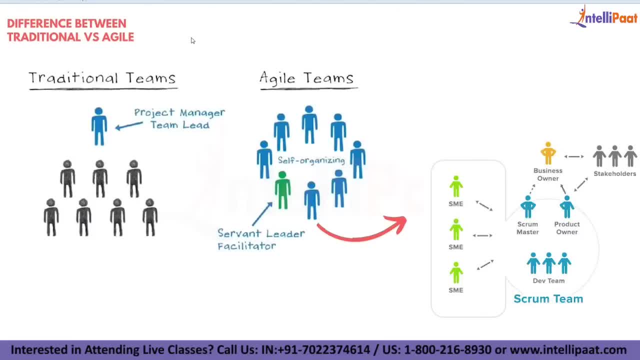 which was allotted to you, so you have to work accordingly. this is what generally agile tells you, but whereas in traditional way of approach and all it's different, but whereas in agile it's a self-organizing team, each and everybody is responsible for the deeds, what they were working. 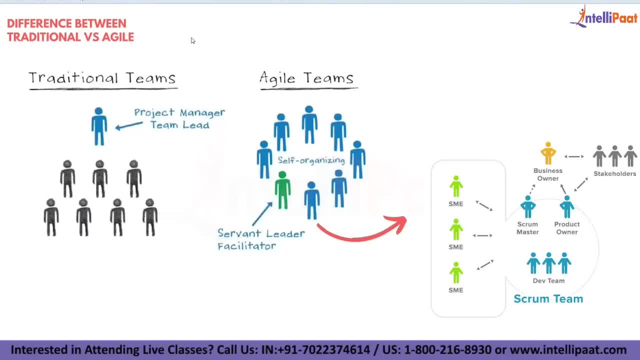 on. so this is the difference you can see from traditional to agile. now, what is the pillar of implementation of agile means agile pillar? this is what we call it as value or we call it as agile values. what are the different, different values do we have in agile? we call it as four different agile values. we 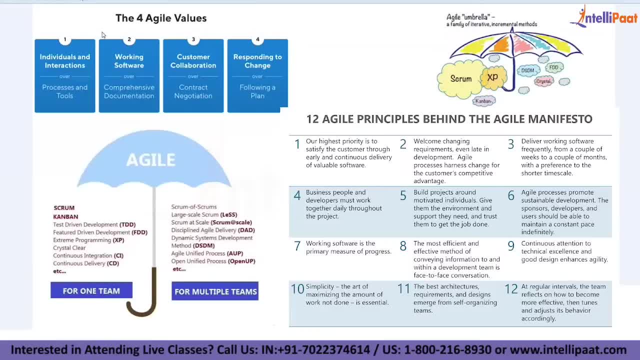 have. so what are the different, different values? agile is having these values. also we call it as agile manifesto, in other words, for this is called as agile manifesto, or values, four agile values. so what are the pillars? pillars of agile, this is what we were discussing here. what are the? 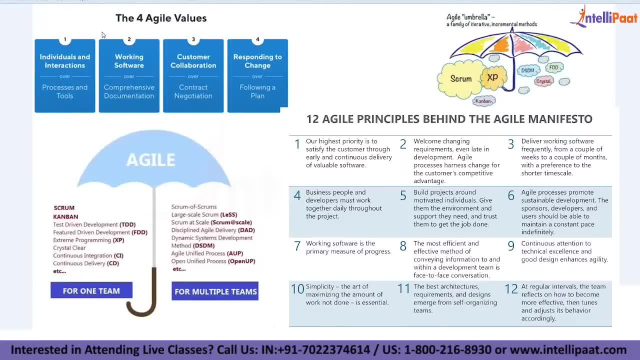 four different pillars, because how it is different from the traditional one, because traditional way of approach known to you guys well, right. so because implementation can be done anytime, so there is no time restriction. even though you have time restriction, there will be an extension of timelines which might be taken by us upon the request of the 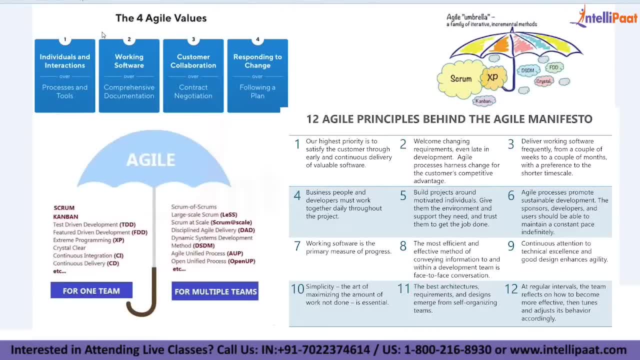 customer rate, where we can request the customer and we can get that, and in individual capacity. based on the individual capacity, people are working hundred percent. we try our best to make it successful, but there are some cases where, due to different reasons, projects will be failed. project failure we need to understand in two different ways. when is technical failure? second, 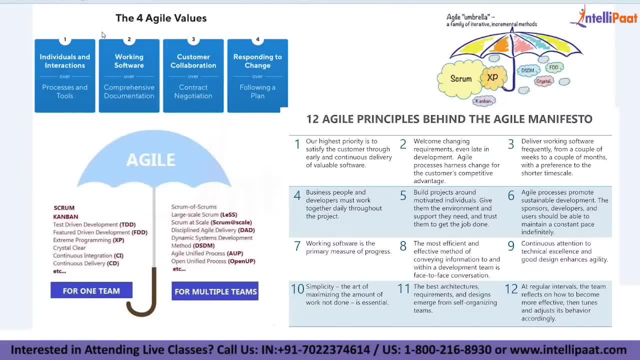 is financial failure, budget level failure. technical failure means we are not. we haven't understood the requirements properly. hence, whatever the application or development we have done so far is not according to the expectation of the customer. this is what we call it as technical failure. next, project failure in terms of the budget budget means over enough budget there is. 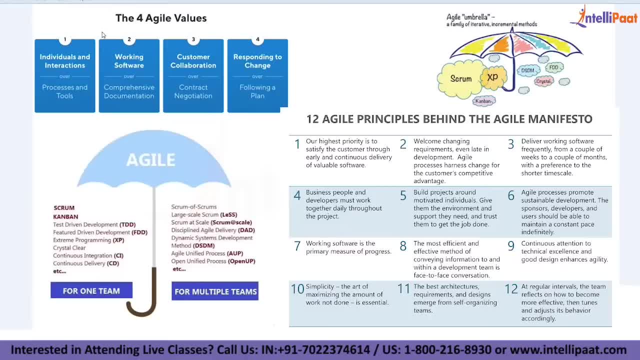 an amount of budget, visual, educated for the project manager what is? project manager is responsible, is not only responsible for project planning and execution, but whatever the budget was allocated, he has to complete it within that limited budget itself. so there will be of no extension of budget will be given, sometimes due to improper practices of agile project planning, improper understanding. 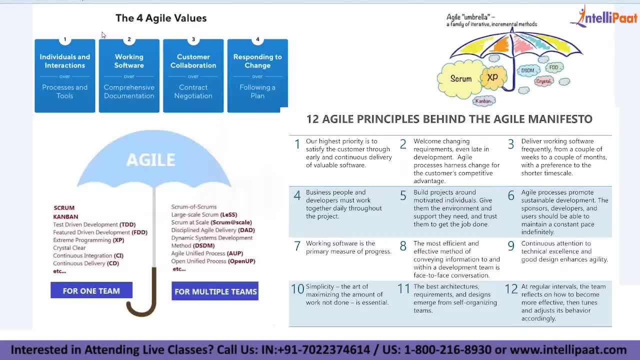 about the technical expertise of the team or maybe lack of coordination of the management team, managing of the teams or whatsoever reasons, because some reasons will be in our control. some are not in our control, right, anything. so sometimes we need to understand the technical experience of the team or, in terms of the project, we need to understand the technical experience. 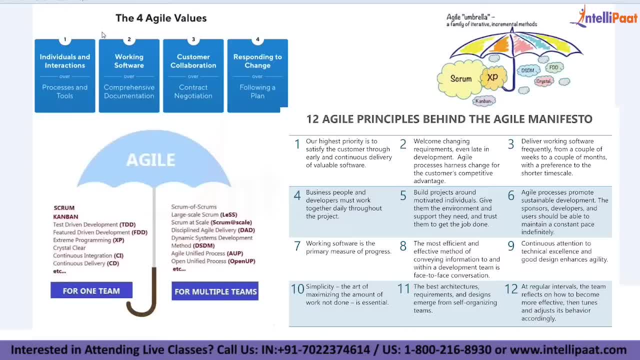 of the project. so sometimes cost over means budget was allocated. but when the project was landed up successfully to complete, it's considered as a cost failure. project project is successful, but whatever are we going to get out of, it is nothing. it's a cost failure because whatever we have taken, 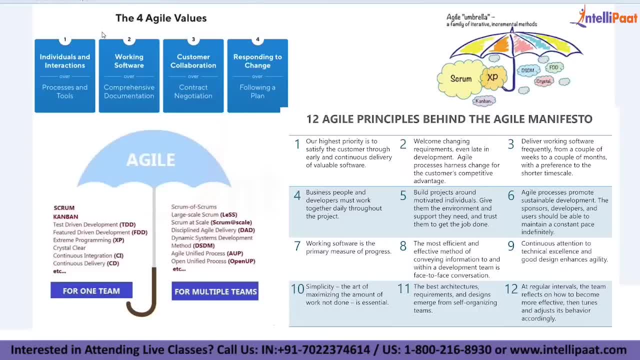 and what we have spent on this has a difference. if the problem is from our end, we have to put it from our side. if the problem means in terms of the changes in any kind of requirements, if this has happened, customer has to pay it right. so this is all depends on the sla, what we have prepared. this is 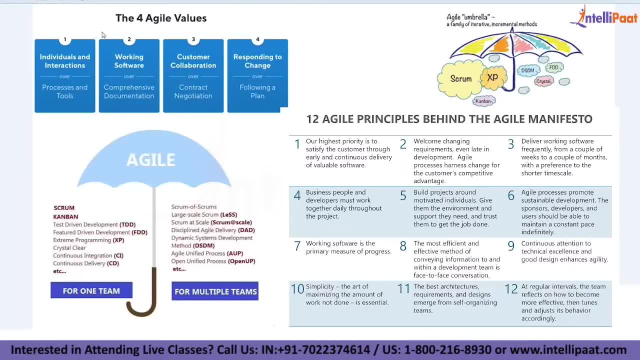 is what we call it as sla. sla stands for service level agreement means service level agreement should be given by the vendor to the client based upon the understandings, what we have and all we have to provide an agreement to the client. so this much duration is there. so in this, within, 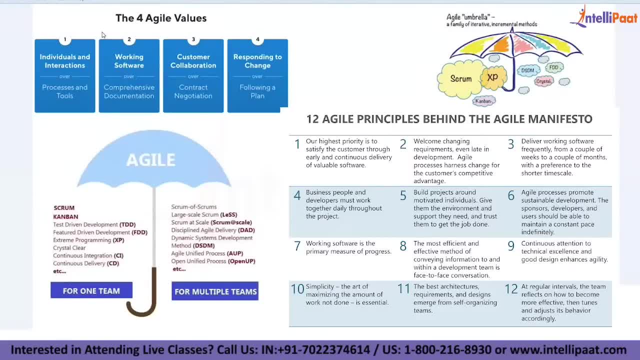 this duration we are ready to complete the project with all the required deliverables, all that stuff. we have to provide everything. so we have to write on a document and we give. so, apart from the financials, what we have discussed, right, so because what? because again, the financials will be different. we go for sometimes, some people go for fixed cost, some. 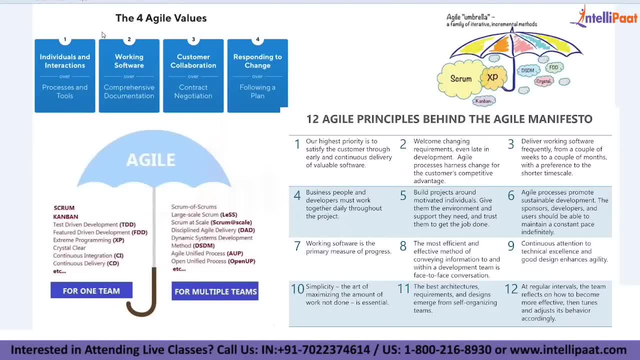 people go for fte. fixed cost means fixed amount of money we are collecting from the customer. client is paying us fixed amount of money and we must ensure that within that limited budget we have to complete. this is one thing, but we have to make sure that no changes in requirements should be. 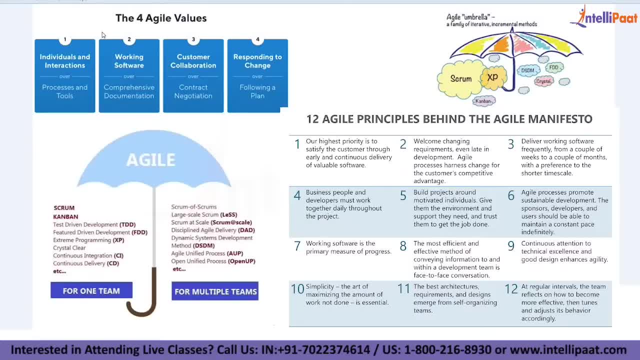 taken place. if any changes done by the customer, again negotiations will be taken place with mutual consent. this is what generally we do in fixed amount of money. second is fte based- we call it as full-time employment means for this project to complete how much manpower we required based. 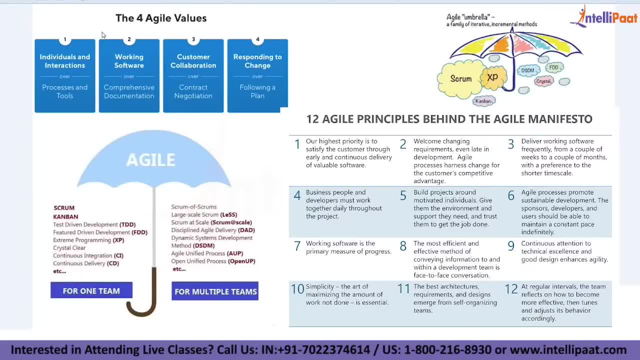 on that. hourly calculation, hourly billing, right wherever. how many dollars are we collecting from the client is what generally happens. these are the two different. once we have discussed all these, so, finally, what is that we do? is that so, finally, we have to provide a service level agreement to. 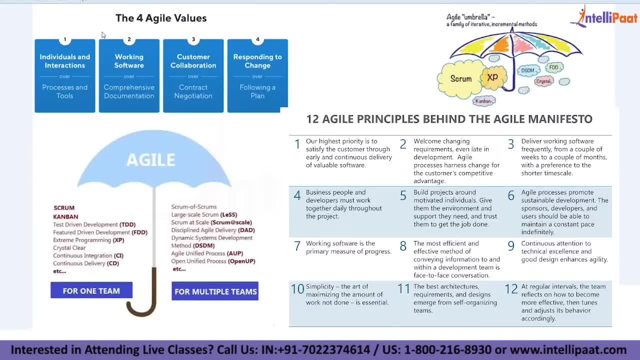 the customer, so based on the service level agreement. so we have to develop the project. so the structure is entirely different. but whereas when it comes to agile, of course, whether you are collecting a final, a single amount of money or the cost of the project, based on the service level, 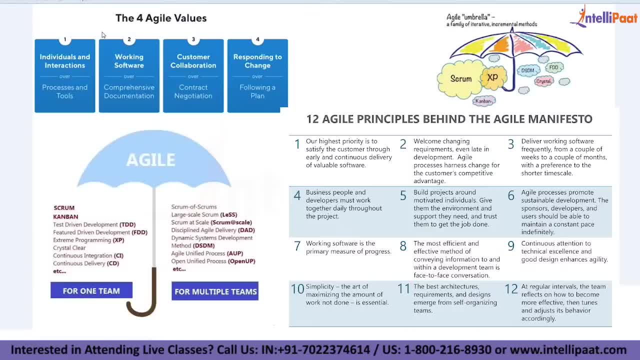 agreement. so we have to develop the project. so the structure is entirely different. but whereas when it mount or you are collecting ft, whatever it is. but the value system of agile is something different from the traditional way the value systems are. for the first part, especially agile is depending on 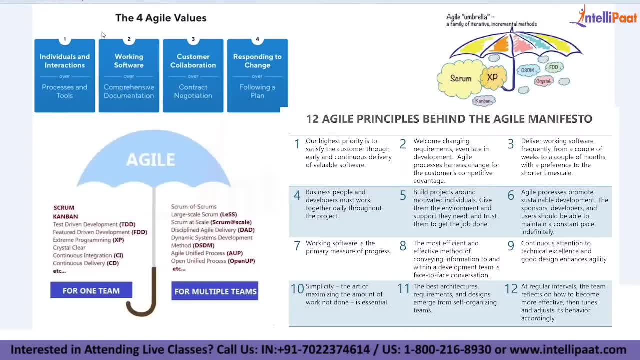 first part is that individual interactions over process and tools. here the understanding is that it doesn't mean that there is no process or there is no tools process. we follow agile, we follow tools and all everything we follow. but more than that, we give importance to individuals and 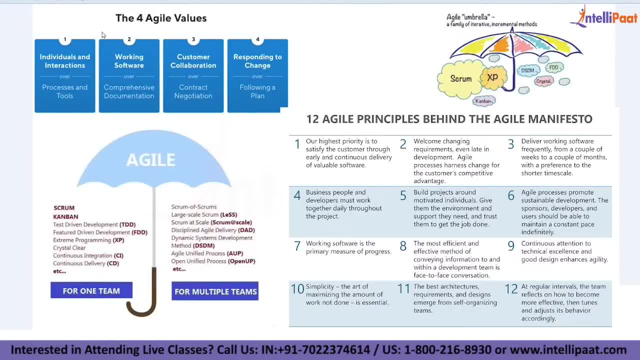 interactions. this is what generally we call it as scrum meetings or daily scrum meetings or daily meetings with stand-up meetings or different, different things. so regular meetings and regular interaction among the people is people happens in agile environment, normally in traditional way of approach, if you see from a context of a ba, when customer, a business analyst wants to transform 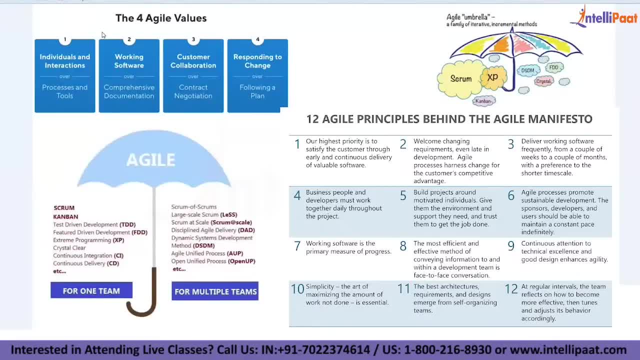 requirements or translate requirements or to communicate with the technical team. how they do that normally they prepare some documentation they give. this is how generally brd, srs or srs are used in agile environment. this is how generally we call it: a scrum meetings or daily scrum. 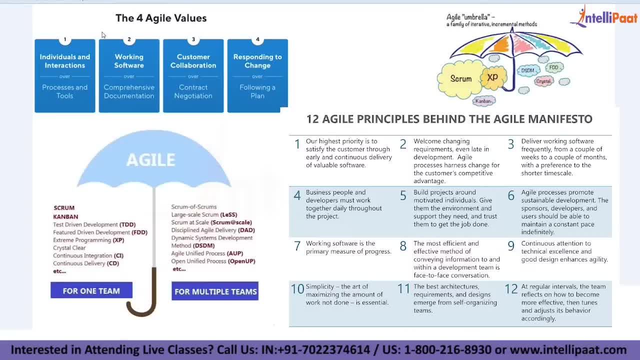 all this will functions if any changes happens in between in terms of the requirements. again, those requirements will be changed in the brd, all that stuff. this is how generally the process we follow in traditional way. there are difficulties, sometimes we may fail in delivering the right thing on the 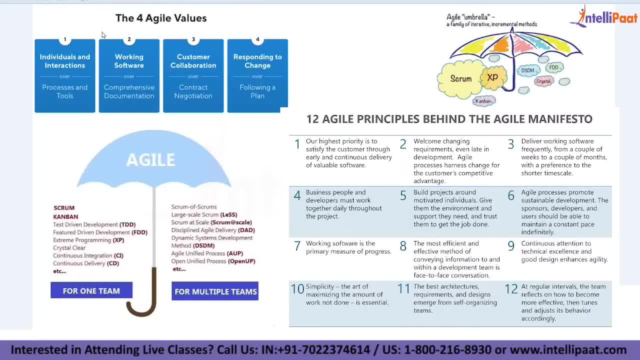 document. sometimes what whoever has understood may understood may not be understood in the right manner. so there are possibilities that communication gap in terms of written as well as the verbal might happen. verbal or written might happen. communication gap may happen for some reason. so it is always helpful when we have in the interaction facility with the team member. so 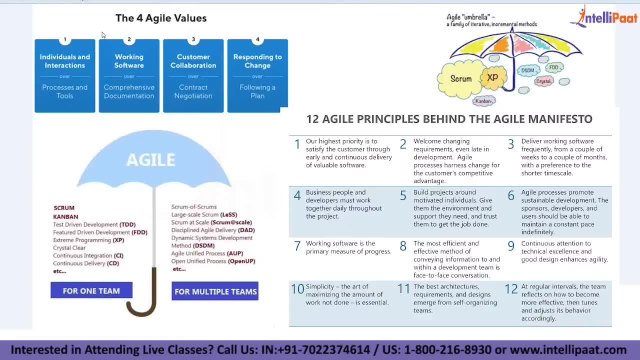 that the communication gap will come down. at the same time, we can have a closed look on work, what they are doing right, so how they are doing what they are doing to attest in they have completed so far, what is that they have completed? so we will be knowing about the progress of work, about 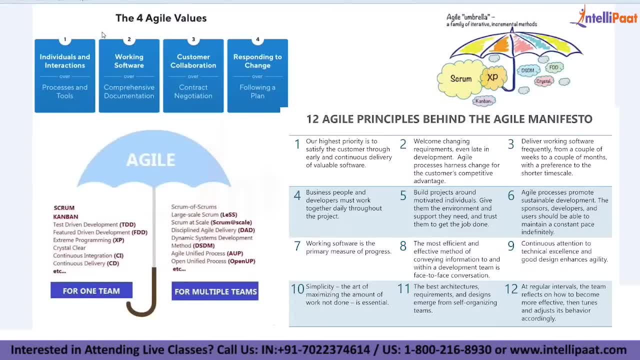 how much they have completed so far. what is the balance? everything can be known to us. at the same time, person who is managing this team, and all have an advantage to see, and, as well as the listen, the practical difficulties, what they are facing, so that corrections can be done with immediate effect. 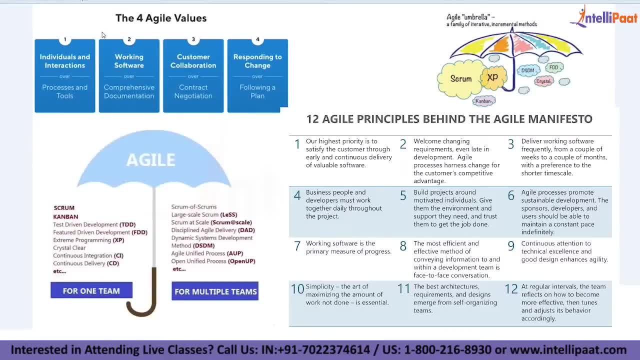 this is an advantage. you can see if you are going for individuals and interactions. so, individuals and interactions: because of this reason, because in traditional model you don't have a facility, because in traditional model there is no much interaction happens. of course there is a part of interaction happens in a way of jad. i hope people who are coming from business analyst 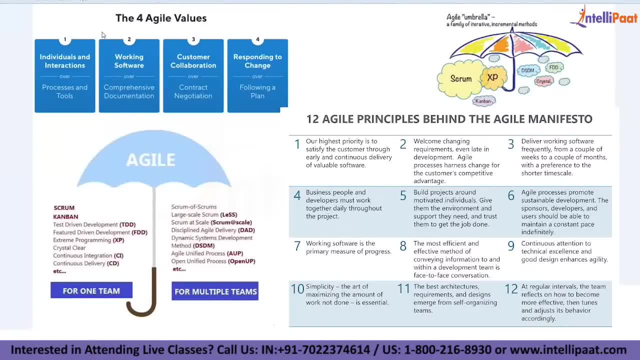 they'll be knowing about this. well, there is a concept called jad. as a part of requirements, elicitation and collaboration, we conduct jad session stands for joint application and development session, which is happens in the initial stages of the project, where we invite all the stakeholders under one roof. their discussion will be taken place and final. 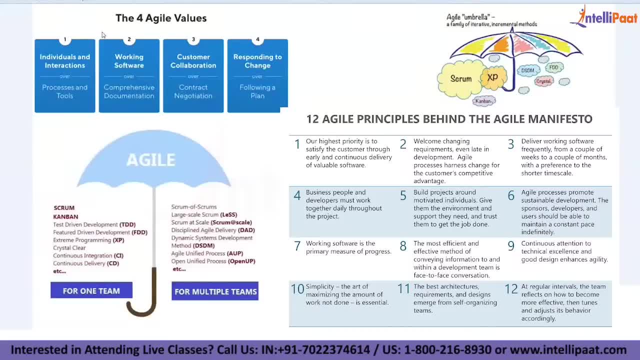 conclusion will be given. there means what they have discussed, right. what is their expectation? what is that? we have understood? all that will be discussed on the platform- that is what generally we call it as jad workshop- which will be conducted in the initial stages of the project, not not. 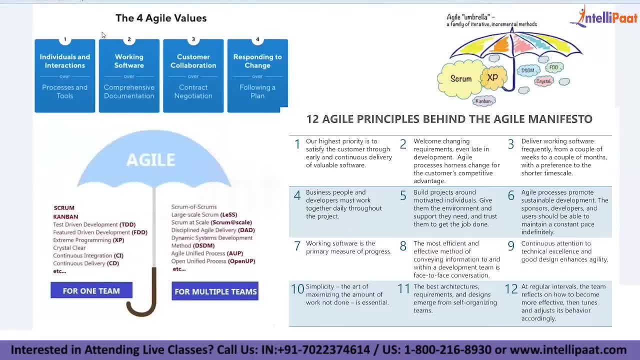 occasional because it's not in regular intervals. it's not possible in traditional way. so there are possibilities that, due to the communication gap, project understanding as well as the understanding of requirements- or sometimes it may leads to failure of the project- also happens, so that problem won't be there again. 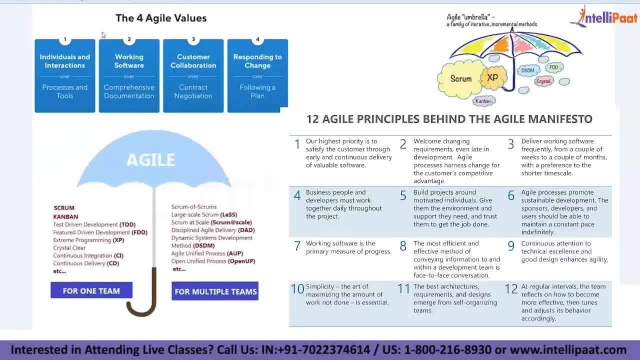 so why? because there are individuals and interactions will be happening in regular intervals with the team members, so that, what are that we are going to do today? right, so what you have, what we have done yesterday, what you are going to do today, what are you are going to do today? the way can you accomplish that? that's the way that you. 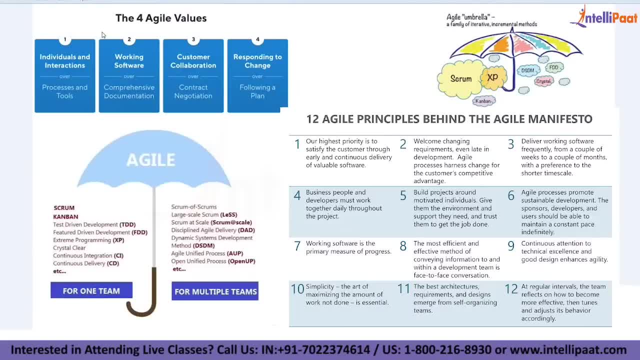 can be done tomorrow, secondary colleges. what is to be done in the beginning, right now, I am going to tell you in an interrupted but first technical analysis. so today We are going to consider what you have written, all the pandas we have upon the project, and we will have the first module: negative right or areas, level of respiration. 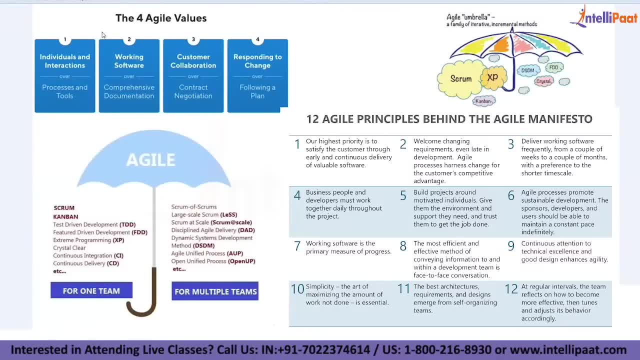 and understanding, Because most of the people have some misconception over that. there is no documentation in agile. It is not no document. I say it is less documentation because documentation is essentially needed even though we are working on agile environment, because not everybody will be experienced. 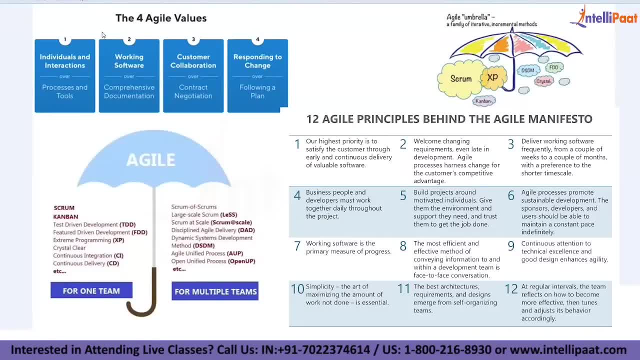 in agile right 100%. There are some people who are new to agile environment Due to the communication gap or due to lack of documentation. they should not feel any confusion over the work, what they are doing, Even though they are technically strong, if you are not providing that facility there. 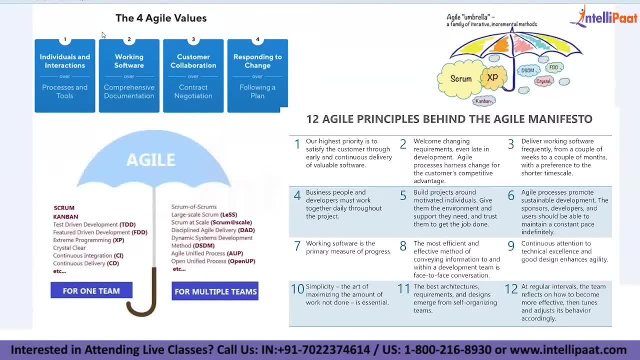 are possibilities that it may lead to confusion over the understanding level. right, There are possibilities. That's the reason why I don't say no documentation. Yes, there are documentation which will be prepared in agile, but not in the form of documentation, something like word documents, all that. 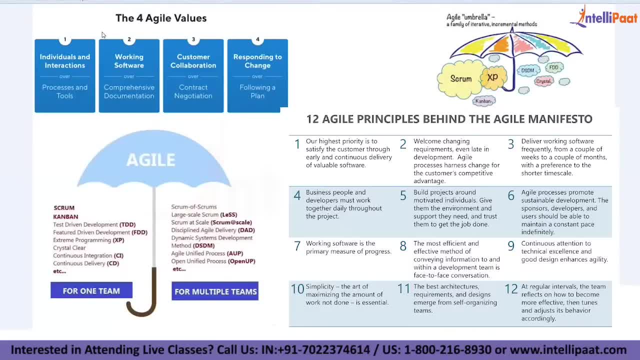 Of course, practically speaking, some people even prepare documents also. That's what I have told in the beginning, 100%. they don't follow agile, They follow the traditional way of approach, Because they are used to, Because I don't say that is wrong. 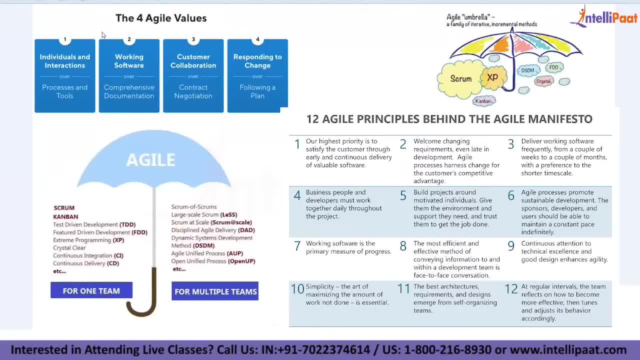 Because, end of the day, as long as we are very clear on what we are doing, nothing wrong in doing it. I never say it's not wrong because their team, they understand it right. So there are things like: as long as they are managing it successfully, as long as they. 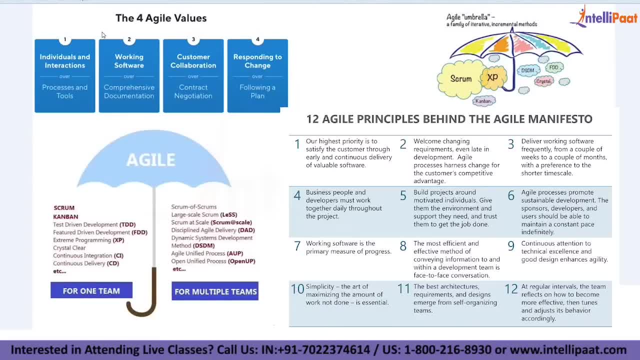 are completing it successfully without having any difficulties or the challenges and all that. it's fine, So we can't comment on it. It is their team and all that, But here documentation will be of very limited in percentage In terms of it. 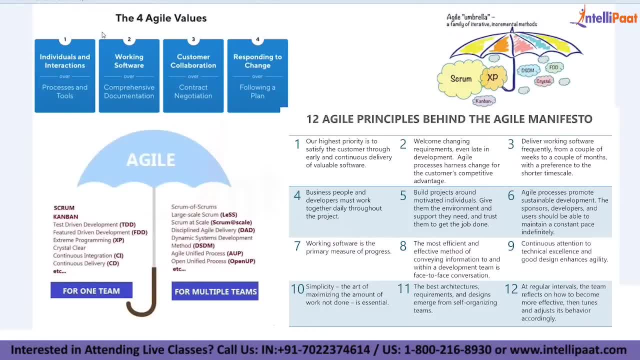 Normally there is a concept called Confluence. You might have heard about it called Confluence because whenever you want to work this application, whenever you want to manage projects and all in agile, there are numerous tools. There are a number of tools, something like Jira, Rally, Windows Azure. lot of tools are there. 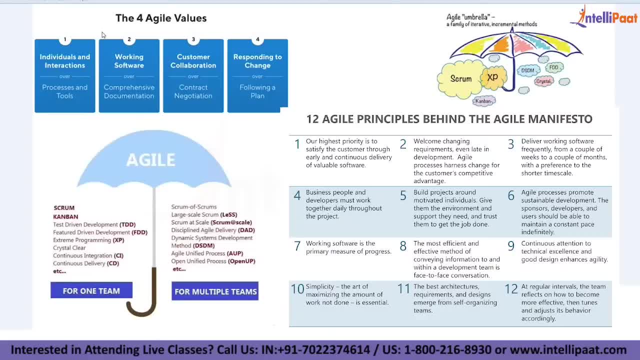 Among all that, there is a tool called Jira J-I-R-A. Jira is a kind of tool which is used to manage the project, followed by bug tracking. all that can be done using Jira software. So in Jira. 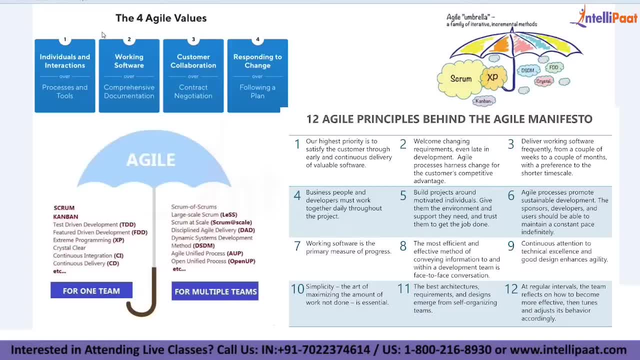 When it comes to the Jira software, it is completely used for project management so that we can write down all the user stories. epics creation can be done Same time. there will be a product back. we are managing all the product backlog, all. 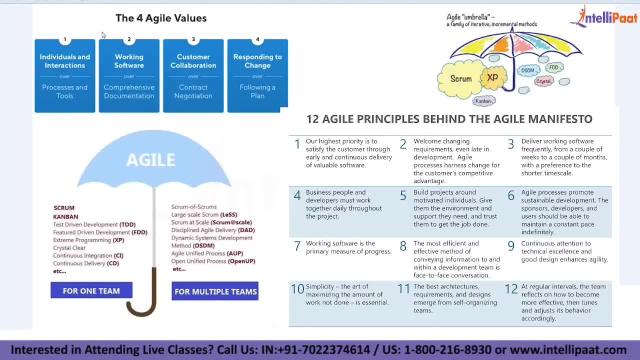 that stuff we were doing. So all these things we were doing in the project itself. So whenever we are working on this normally, whenever we are working on this process normally, there is a tool called Confluence. Confluence is a tool which is used for data. 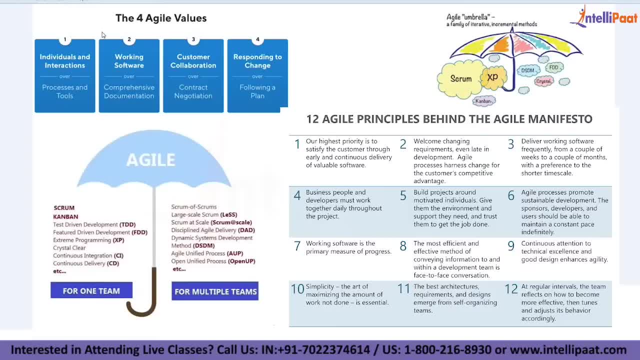 It is used for document collaboration. Document collaboration means where, if you want to write down some product requirements- for example, what are the product requirements we want to write, the product requirements to write- there is an option for you in Confluence. Let's say, as I told you, individual interaction through scrum meetings, daily scrum meetings. 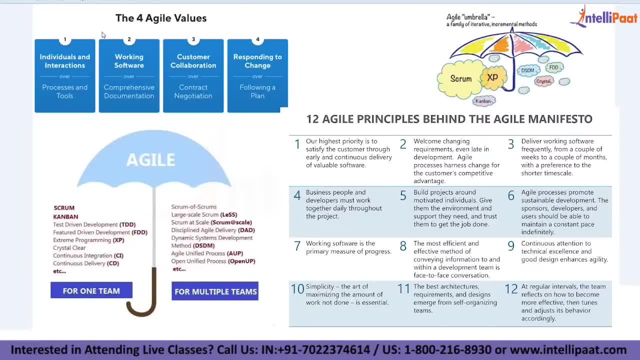 we conduct. That's what I have told you. So whenever we are conducting the meetings, we want to update the meeting notes because what we have conducted so far, what are the points we have discussed, where we have concluded which is accepted. 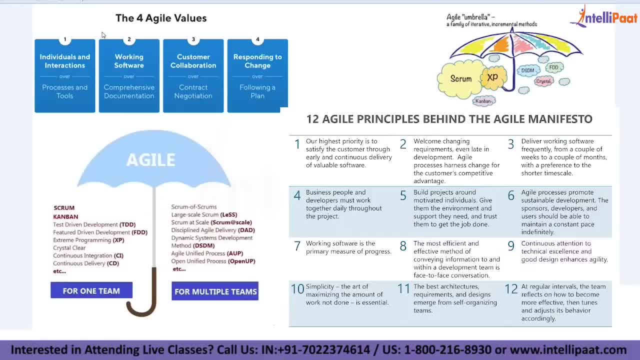 Which is rejected, Which is different Right, That has to be documented. So for that there is an option called meeting notes, So where we can write down all the meeting notes there so that people can see, because, if you add, as we are connecting this Jira with Confluence, so that whoever are there 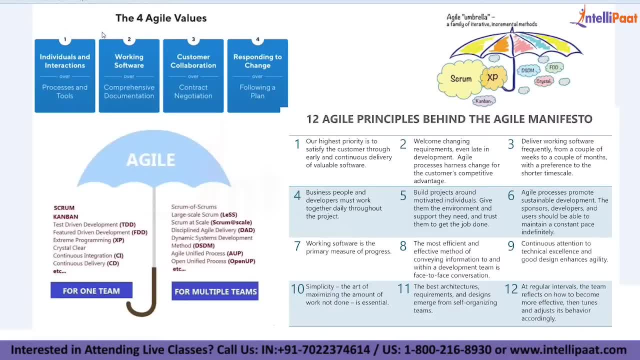 in the team, because whenever we create the Jira as a project management, we add all the people who are relating to the project, all that, So we are. whenever we are adding the people, whatever the updations and changes are we making, everything can be seen by all these people. 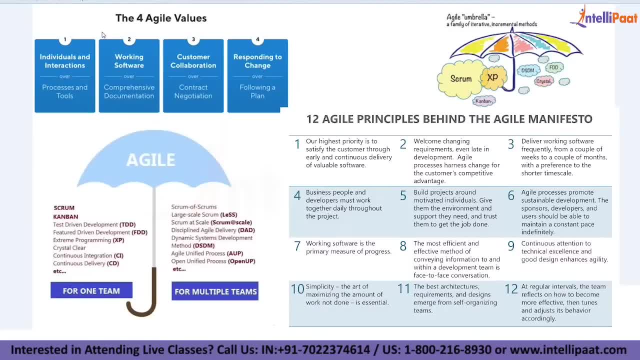 So meeting notes can be updated at the same time. if there is any kind of retrospection we do in terms of the sprint retrospection, all that, that also can be done. So what I'm trying to say is that documentation is very limited in terms of the person percentage. 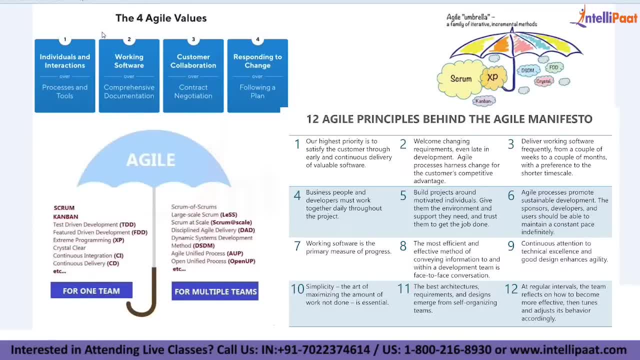 but it is in a form of conflicts. This is what generally widely we are using now, because that is that gives a value addition to the team when they are working on real environment, because in the traditional way we have a facility for documentation to prepare. 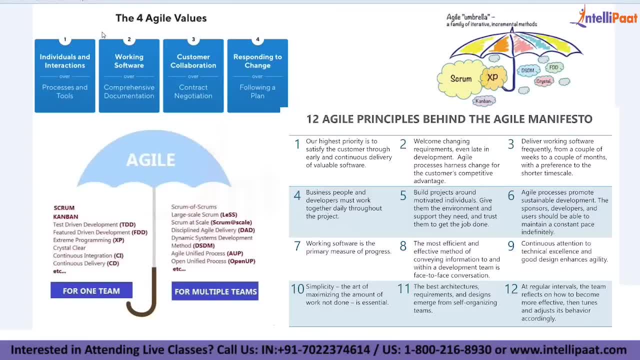 We have all these BRDs, SRS, all that stuff is there, but whereas in Agile you don't have the facility, in Agile we have a facility called Confluence, where there will be less in documentation. So when it comes to this, rather than the documentation, we give more importance to. 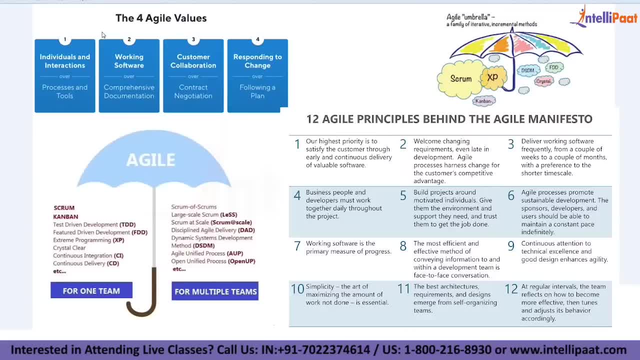 the software. working on software means whenever we get the requirements, immediately we start working on the software itself. And if there is, you could ask me one thing then, Raj: if there is any changes to be made, what is that right? 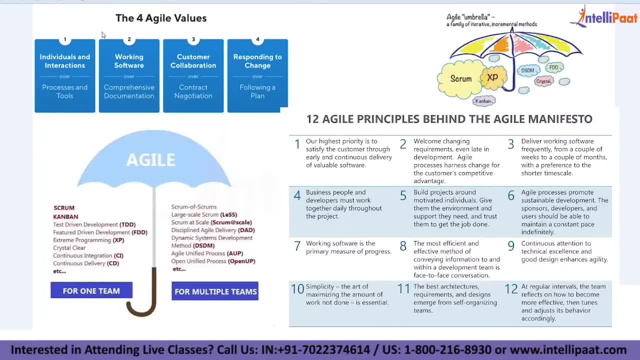 So how are we are going to do the change? Whatever the changes are we going to do, everything will be done accordingly. So, based on that, changes will be made right. So because in between, when there is any change, customer is expecting us to do so with the 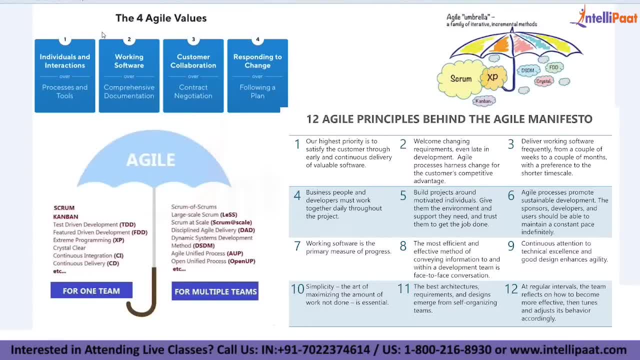 team consent of the team members, and all based on the possibility changes can be done accordingly. So there is no. I don't say there is no planning for project in Agile. Yes, there is a planning, but this planning is short in terms of the percentage. 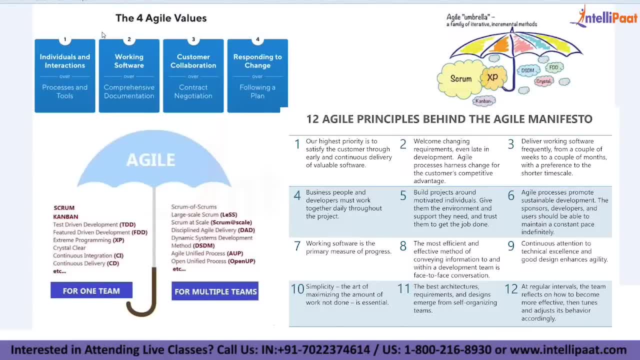 There is no long-term planning, So the planning is confined only to the particular release we plan. So, whatever the work we do, Whatever the planning we do, everything is confined only to the particular release within that particular release we have to complete. This is what generally the working software is, means you are directly working on the 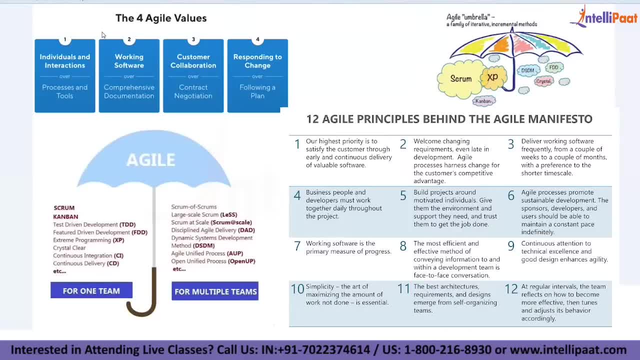 software rather than you are depending on the documentation. So there is no because in traditional model, because every time I'm comparing with the traditional so that you'll be understood better. So if you see that documentation, if you see a traditional way of approach, if you are, 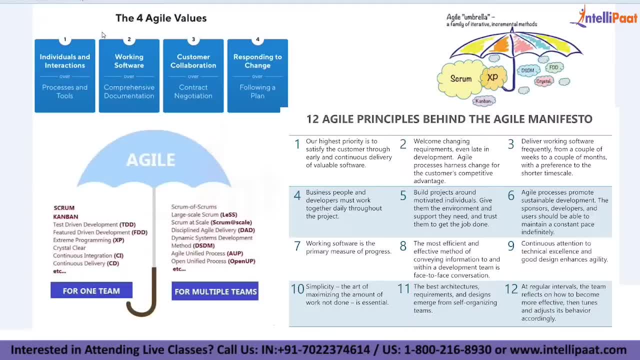 a developer? on what basis development will be taking place? development will be taking place based on the documentation called BRD SRS, what you have received from the BA, because they are the one who is translating the requirements in a documentation format- and the documentation. 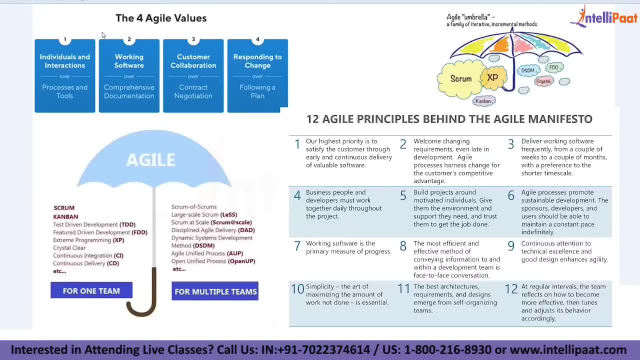 will be given to you as well. So you are taking up the documentation, you are working on that and, finally, you are delivering it right. This is how, generally, the process you will be following. So, based on the delivery, what business analyst has been given? technical people will go through. 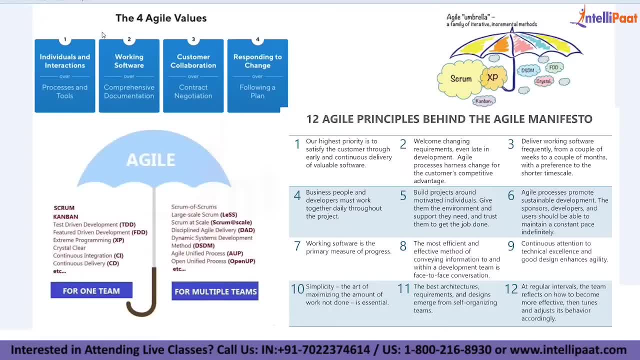 that and they work. whatever the functionalities they are preparing, whatever the non-functionality speeches, Everything is based upon the documentation, what BA has given. But whereas in agile environment you don't have that facility, you don't have that process, because there is no documentation, everything through interaction, because whatever we have, 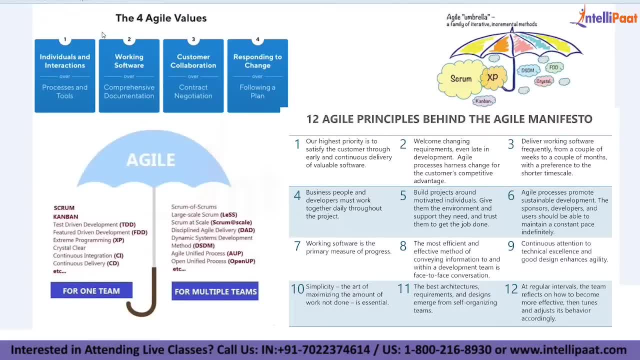 interacted. whatever we have decided and accepted, that will be put it on the practice with immediate effect, without any second thought. we are implementing it to the next level. This is what generally working software stands for Means directly. we are working on the software, not having any documentation on that. 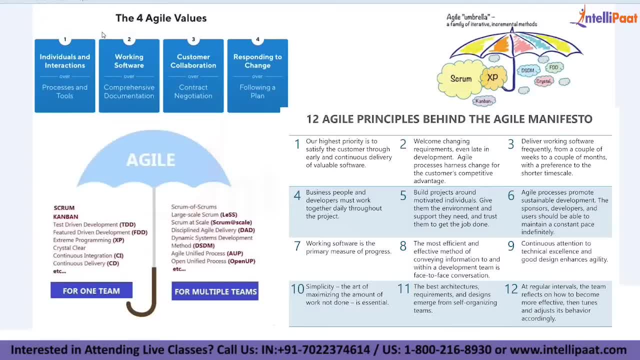 So, whatever the documentation is, So the documentation in terms of the confluence we have and all everything is optional. because that is optional? because not everybody uses confluence, all that right, It's an optional thing based upon the team, what they have decided. 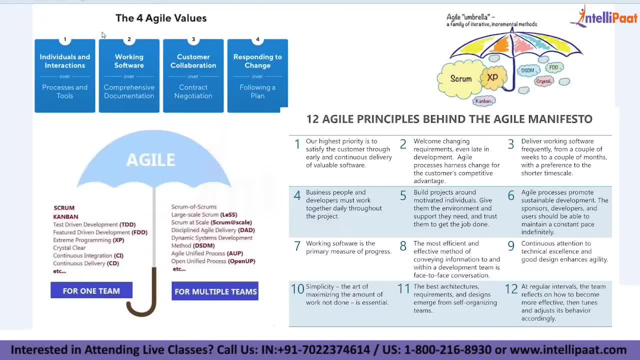 If they want to connect the confluence and all with Jira so that document collaboration can be done, so that people will understand more effective and better. but which is not compulsory right End of the day, it is optional right, So it is not compulsory as it is right. 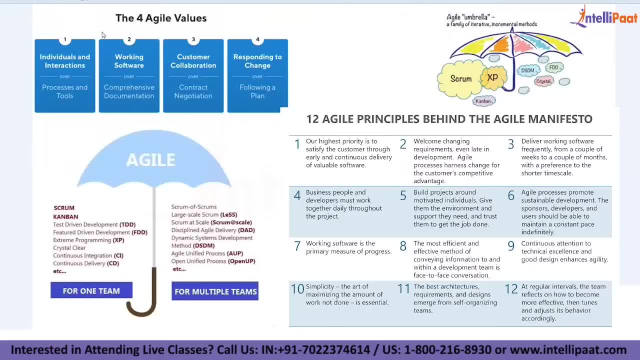 So this is the second point: working software. The third is that customization. The third is that customer collaboration over contract negotiation. So what is customer collaboration over contract negotiation means normal and traditional way of approach. If you see closely, there will be no customer or customer representative will be there in 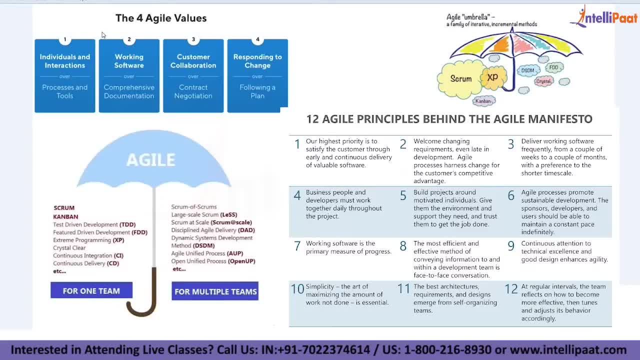 the project because customer is an outsider, always an external stakeholder, where customer has given the requirements. Whatever the work we do, everything is being confined to the development team. Development team itself is doing all the activities: Customer representation, Maybe SMS, and all everything was supporting us from outside and whatever the necessary. 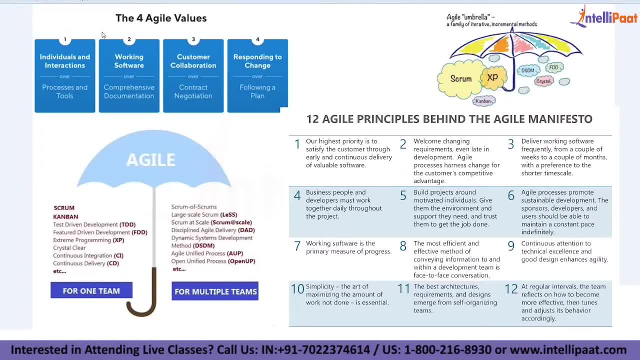 information they want to provide. they'll be providing us everything from outside. This is how generally that works, But whereas here, especially in agile, the advantage is that customer collaboration means customer representative will also be a part of the project development. Whatever the work we do, customer will also be a part of it. 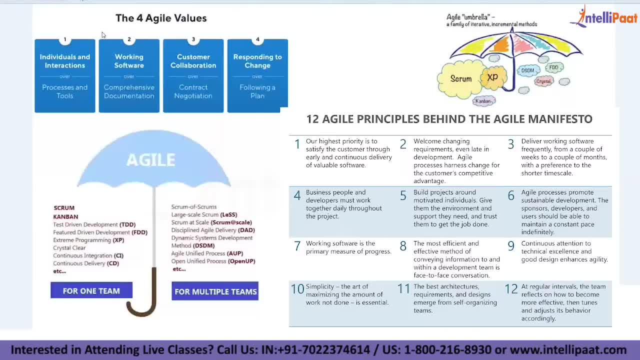 Who is customer here? Customer is not a business owner, right? Right, It's a large MNCs, multinational companies. Business owner means it's all run sometime with consulting, right? So with group of people there will be board of directors, right? 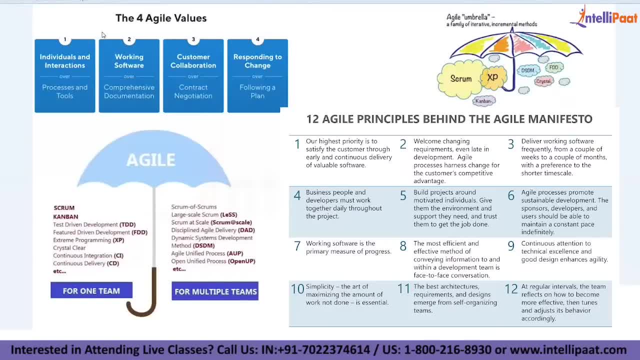 So they'll be taking a position. There is an organizational structure, right, You have a CEO, you have a CFO, COO, all that. So all these multinational companies, there is an organizational structure we follow. So, even though we have an organizational structure, there is no customer who will be coming and 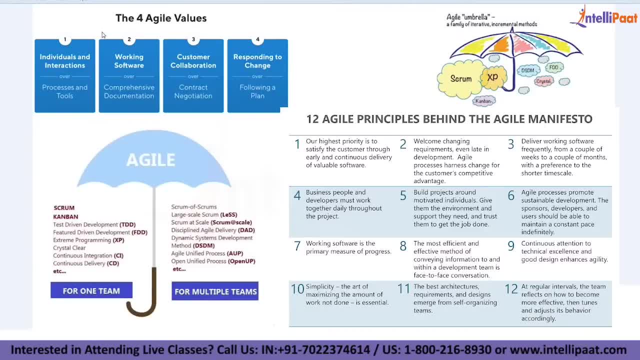 taking us in the project Right Right, There is a role called PO. Normally in agile there are three different roles in that one role called PO. What is PO? PO stands for PO, nothing but product owner. that role will be called as PO stands for product. 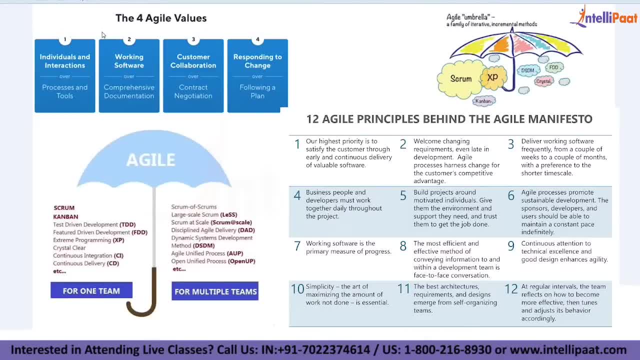 owner- Normally this product owner, nothing but client representative. how practically happens, I'll tell you. Let's say, you are planning to develop a project. All you guys were belongs to one project, right? So you have. you are a team of people who are planning to work on agile environment. 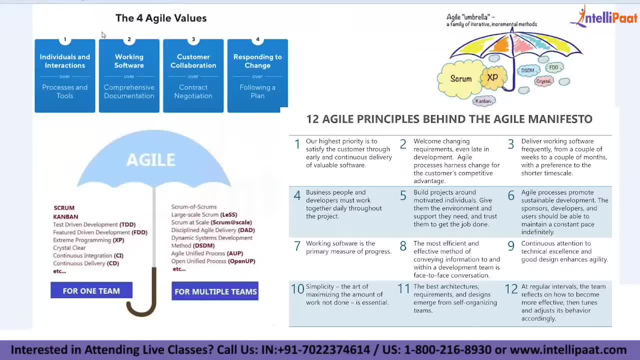 You guys have decided Now: you want to implement the project in agile, Assume that you are experienced or you may be new to so. few are experienced and few are new. Okay, What to do Now? here there will be a role, as I told you, as we call it, as product owner role. 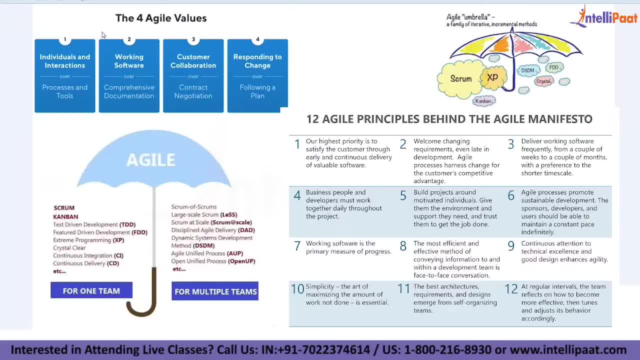 This product owner will be appointed by the client in some occasions. Normally and practically, they will choose a product owner and they will recruit a product owner, Some person who is knowing about the, who knows about the requirements, who knows about the requirements well in advance about the project, everything. that person will be called. 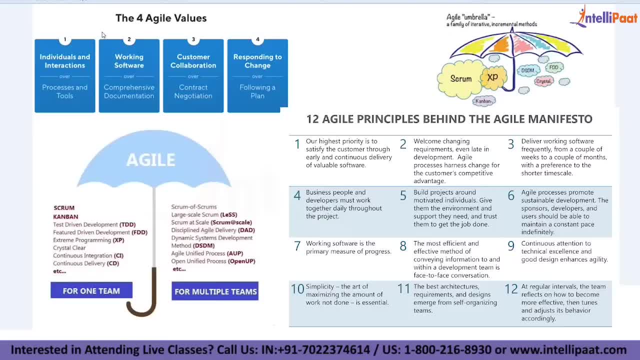 as product owner means what customer wants, what are they expected output right. So all that will be known to the product owner. So whoever is knowing that that person will be called as PO. Normally customer will provide this PO to us in the first level. 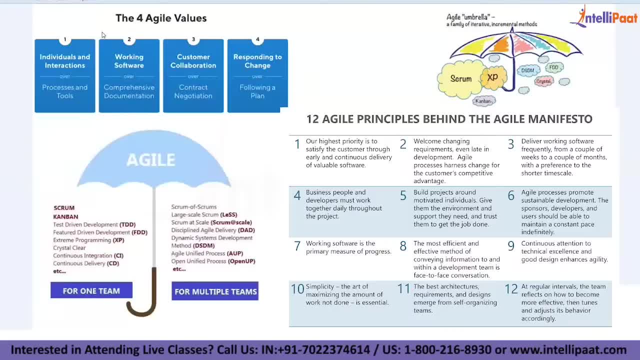 Normally PO will provide this to us. This is the first level, Whereas in the second level sometimes customers won't provide us the product owner and all. If customer is not willing to provide us the product owner, then we will not be able to. 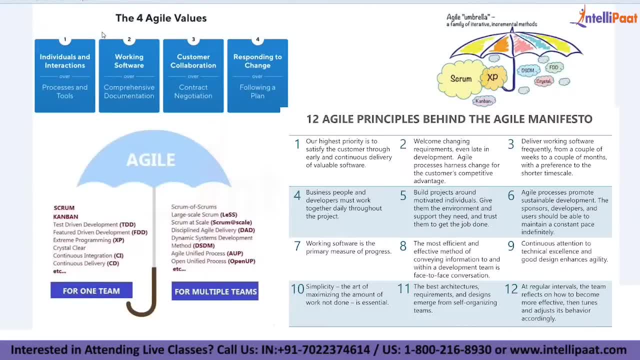 provide the product to them. If customer is not providing us the PO, what we do is that company itself will recruit one PO on behalf of the client. So what is that this PO do? This product owner is the person who is responsible to provide a quality output of the project. 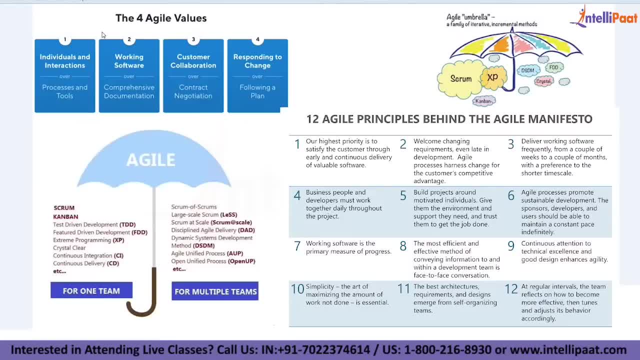 as per the expectation of the customer. This is what, generally, the product owner responsibility majorly lies on. Thus, project owner is responsible, completely onto that. Project owner is completely responsible of what they are expecting. So this is what we do. Okay, So this is what we are expecting, because they themselves were treating as customers. 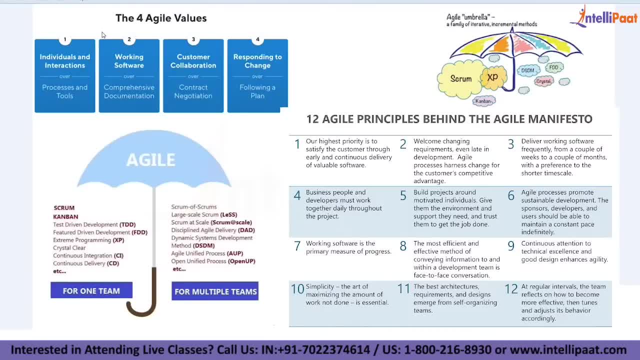 So what is that I want is what I am making team to develop. That is what generally customer collaboration means. So when there is a customer collaboration, of course every, every, every process has its pros and cons. This is no exemption. 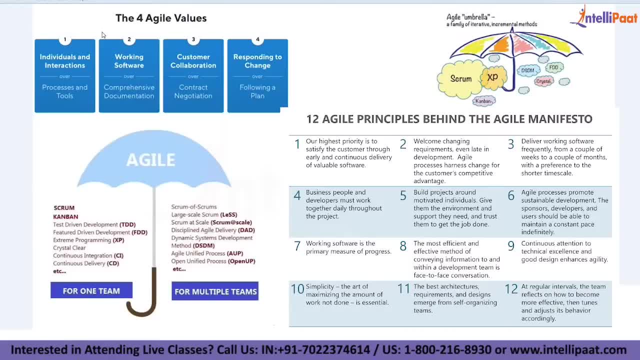 Right, Even this agile is also no exempted, because practically there are some difficulties. Of course, that's a part of a process anyway, right? So we have to learn new things and we need to add up new, new strategies, and we have. 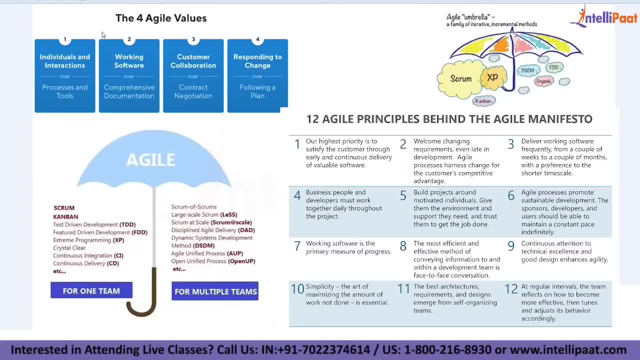 to move further. Right So, this is a continuous process, So there is nothing to say a hundred percent perfection, everything of that sort. Right So, because agile is not something new, agile has been derived from the old models, what we are using successfully at one point in time, but due to the practical difficulties, 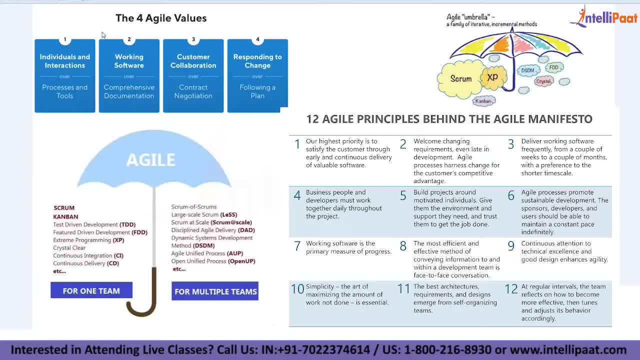 what we have faced over a period of time and all slowly, the practices and the value systems have changed And we have named it as agile Right. Agile is not born new Right. It's not a new born instant, due to the challenges, what we have faced, based on our experience. 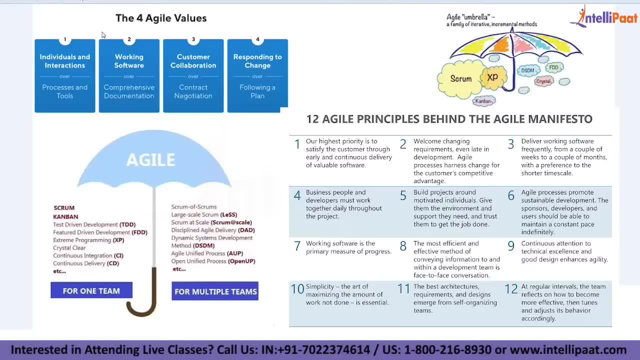 Okay, Okay, Okay. So we have changed upon the models, what we have used and all slowly, we have refined to the text and, possible slowly and based on the challenges and the practical exam difficulties, what we have fixed. Just a quick info, guys. 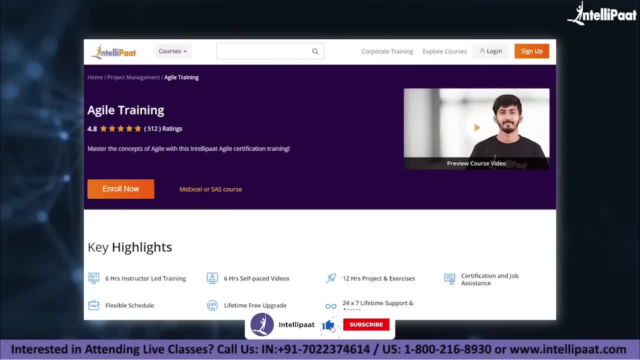 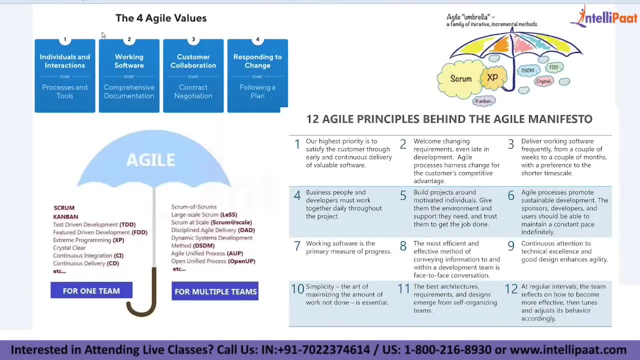 Intellipaat provides agile training mentored by industry experts, The course link of which is given in the description below. Now let's continue with the session. A new system called agile has been derived from the old ones, Right, So that is not a hundred percent entirely new. 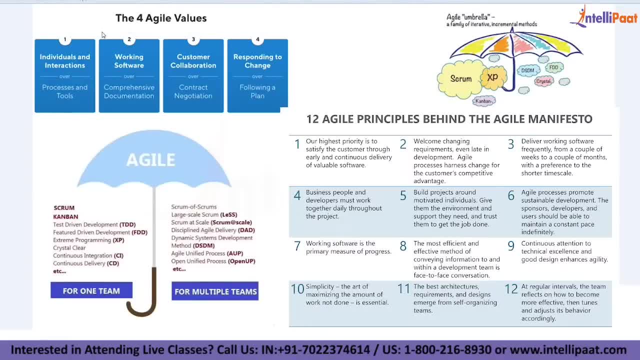 Because this is purely a new system, This is purely a different one. So, the same way, every process or everything will have its own pros and cons. That's a different, that's a known thing. So, customer collaboration, the advantage for you, for customer collaboration, is that what? 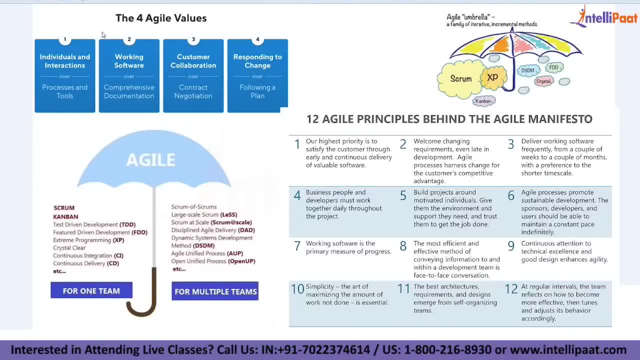 is that they're expecting will be known to each and every person who is involved in the project well in advance. That is one advantage you can see in customer collaboration, because there are less percentage of communication gap. You could ask me one thing: Can you expect there will be of no communication back in gap if a customer collaboration will? 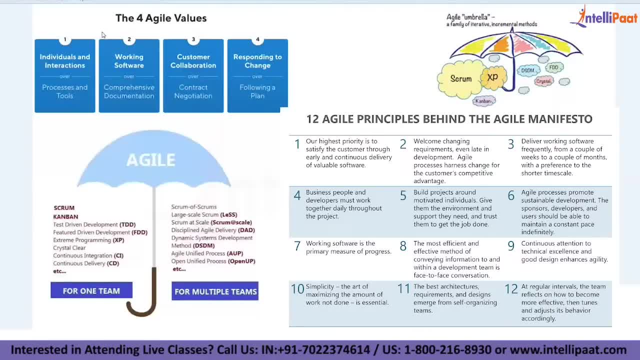 be there. but a hundred percent is not guaranteed because there is nothing called a hundred percent Everywhere. 99% is what the standard thing is. Nothing has a hundred percent. So there are chances will be very less that I can see practically speaking chances will. 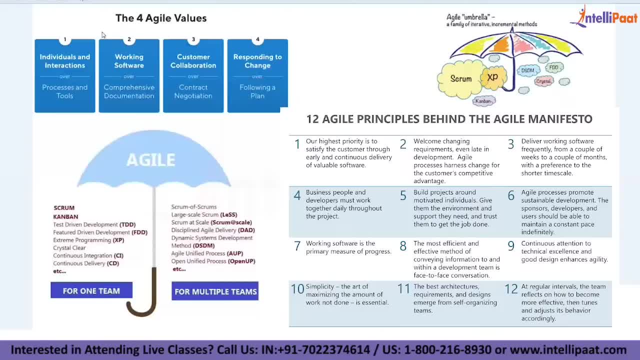 be less because product owner knows everything. So what is their expectation? What is that they want? As long as if they have a clarity, But subject to demand conditions. Terms and condition is that product owner should have a clarity first because you could ask them, and then product is so clear about the one. what is their course? 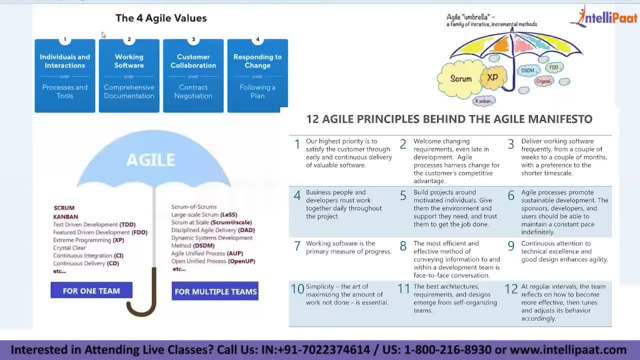 Obviously there are some conditions. but if a product owner is confused on something right, If customer product owner is not to the extent possible, if he doesn't have a clarity on something, obviously there is a communication gap might be raised. So there is a percentage of probability, of percentage, that thing will be there. 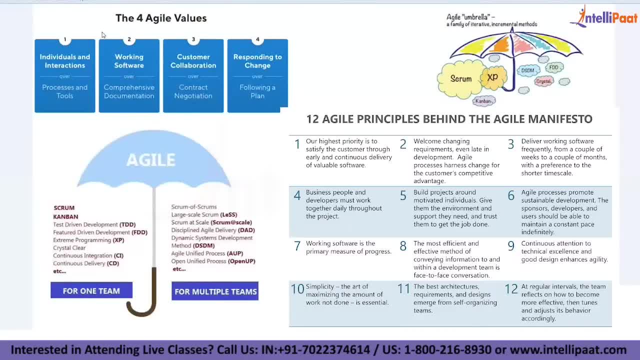 But the major advantages are payments and accounting, But the major advantage of a collaboration in that the customer will be there with us all the time as long as we are working on the project. So what are their expectations, demands? everything will be known to the team members. 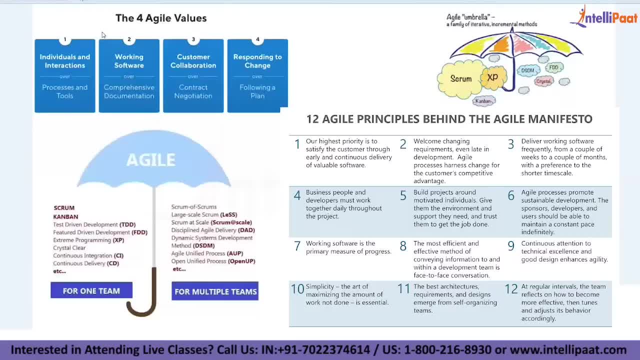 Well, in at once. at the same time, what we have, what we are doing, will be closely watched and observed by the product owner because, in a way of conducting regular meetings- we meetings- all that customer will be knowing about what is that we have done, how far we. 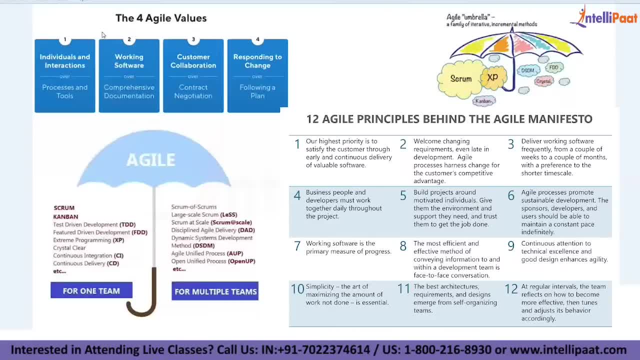 have completed? what is that Not it completed so far, Because anybody who doesn't think something sounds interesting. practical difficulties when people are working on, even though we do the our own practice prayer, but end of the day, this is. there are some practical possibilities and complexities of. 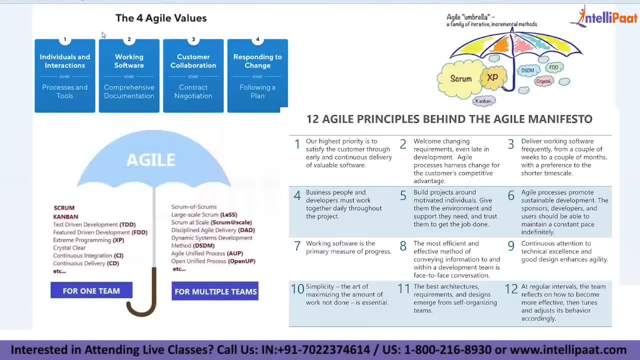 implementation might be taken place in between, which is not something guaranteed. sometimes it happens that practical difficulties team might be facing for different reasons, which- because 100 percent that cannot be identified. so for negotiation purpose also it is. you have an advantage because customer will be there with you all the time. there are possibilities that. 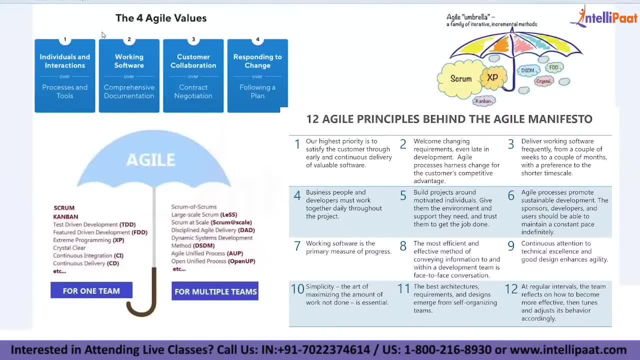 negotiations can be taken place with the customer. so whatever we want to make some changes out of, it can be done accordingly. so this is another advantage where you can see in terms of the customer collaboration here. so customer is collaborating with you all the time in a way. 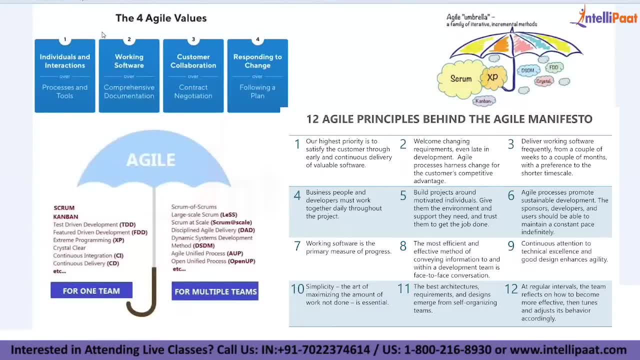 of the role called product owner. but remember one thing: this is a role of product owner you see only in scrum. if you follow practice of scrum, then only you see this. but whereas if you go for can, ban or something like that sort, you don't see any this product owner, even the team members who are 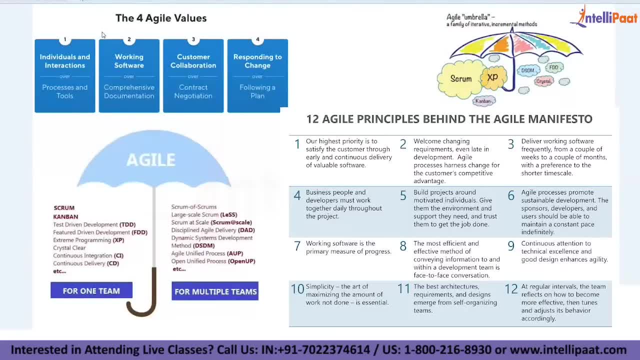 responsible to complete the task. they themselves have to take care of all the requirements, and all directly from the client. so there is no middleman called product owner. if you call privo as a middleman, there is no product owner. in can ban the same agile, remember, in the same agile, value in agile. 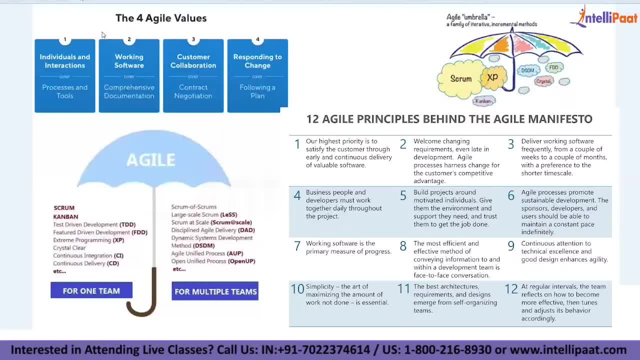 if you follow scrum, the approach will be different. if you follow can ban, the approach will be different. if you are following can ban and all that's, you'll be having more of product owner. all that if you follow a practice of can ban, again, you don't. 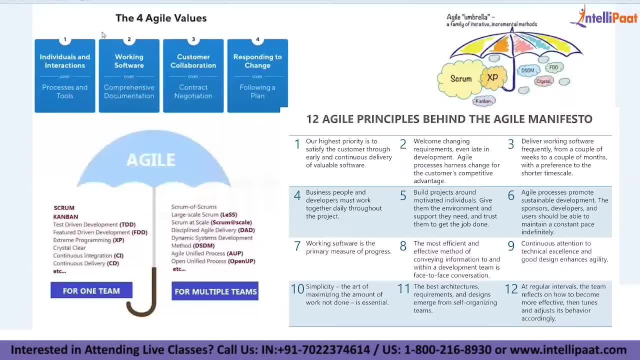 see any product owner, something that with whatever the development team- normally those people we call it as development team, right so even in can ban there is a team, team, development team we call so that team is responsible for the all the ones, right so? even requirement gathering everything. 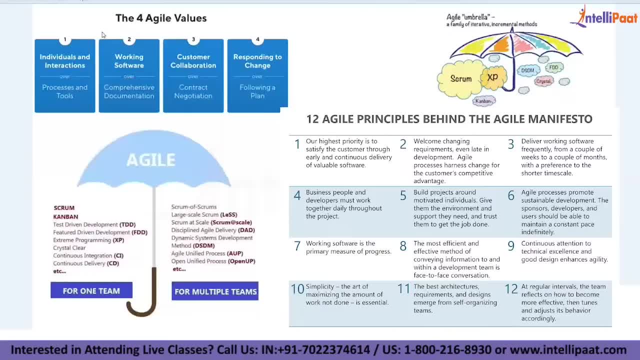 will be looking after by the team itself, not by anyone as product owner, as separate. but this is possible only in traditional scrum, all that stuff. but the value system, customer collaboration, yes, means customer is directly interacting. interacting either way, whatever the way customer is directly interacting and whatever the requirements. 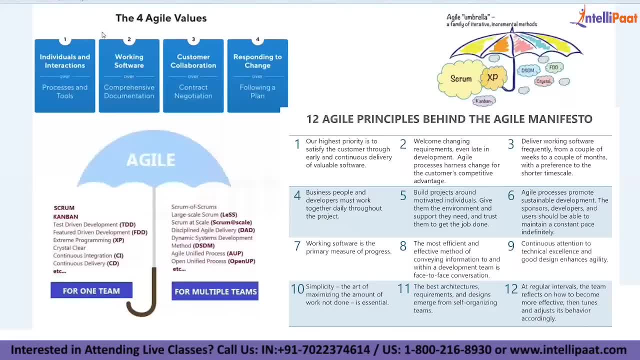 they want us to develop can be done accordingly. this is why this is how generally. the third point: consumer collaboration means customer directly involving in the work what we are doing, so that, whatever the necessary output, they are expecting everything every day because it's a day-to-day activity, because agile is something confined to limited ones. 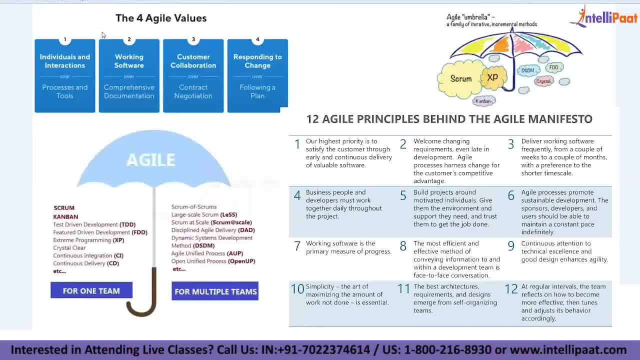 if you have taken up some sprint to be completed, it has to be completed in two weeks time. one week, two weeks, three weeks and four weeks and so on. within weeks it has to be completed. again in weeks it is converting into days back backward. you can say right, weeks, week to days, days to hours. 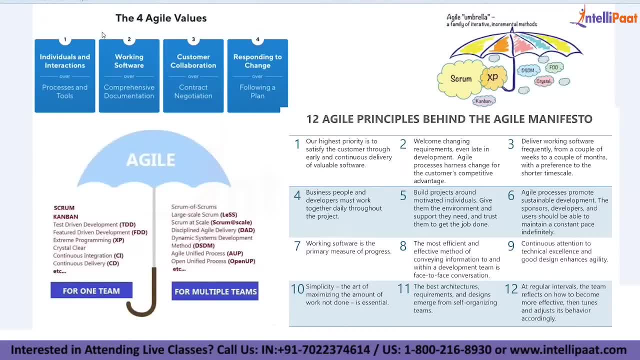 this is how generally the calculation is. so each and every one hour, each and every, each and every hour is important. each and every working day is important because normally, whenever we take the calculation, we take working days, not the week, not the holidays, even any national holiday, something that will be taken out, that will. we don't consider that. 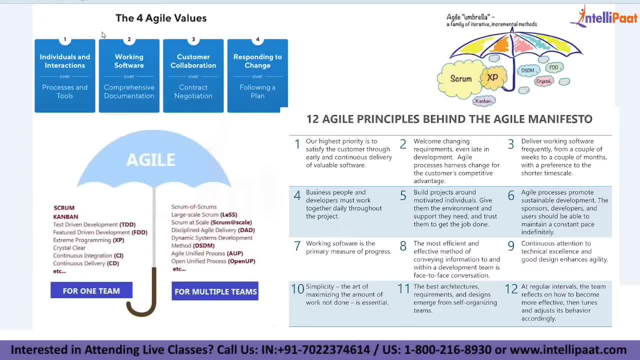 if it is, for example, if it is weak, we take five days into consideration. no, saturday, sunday: even in this five days there is a national holiday or something like public quality, we will, we have to take it out. we have to consider only four days. so when, when it comes to the 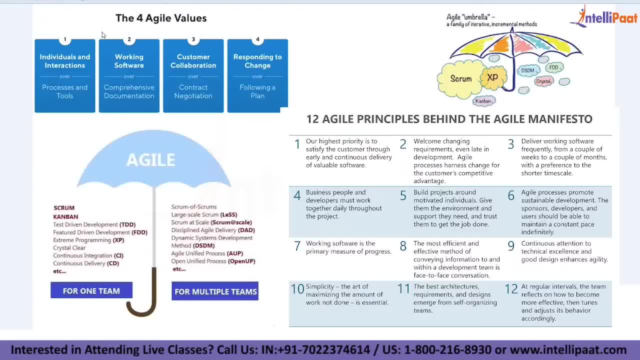 planning right when we are coming, when we see, like, how much manpower we have, how much time we have to complete, right, if you are calculating all that stuff, this is how generally we do. so customer collaboration is what we do here, right? so this is third point, next responding to: 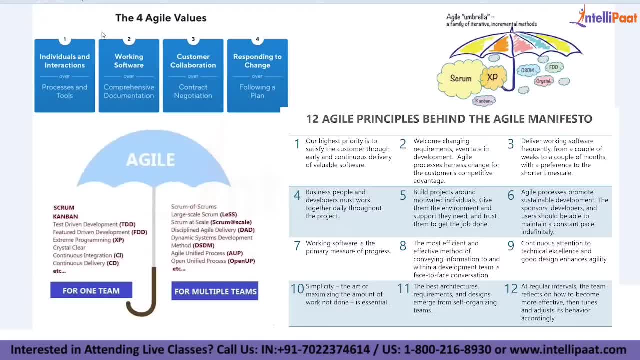 change over the following plan means there is no proper planning. i don't say proper planning not in other sense, there is no plan, perfect plan for this. if there is a change, which is inevitable, which has been requested by the customer, how to make this change happens, how is it possible to? 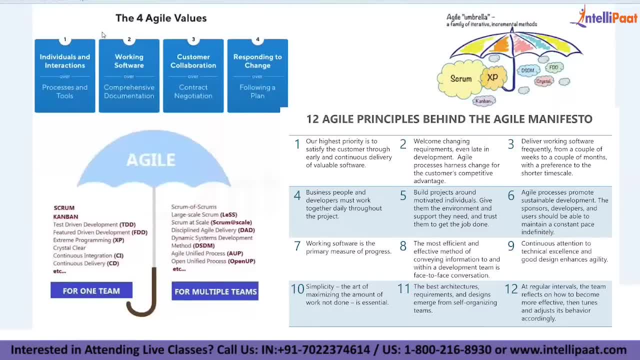 implement the change is what generally the perception of the team will be having. so means, whatever the changes customer is expecting, we have a facility that we do as what we can, but this is with the consent of team. normally we do. it is not that, as i told you, that there is possible. 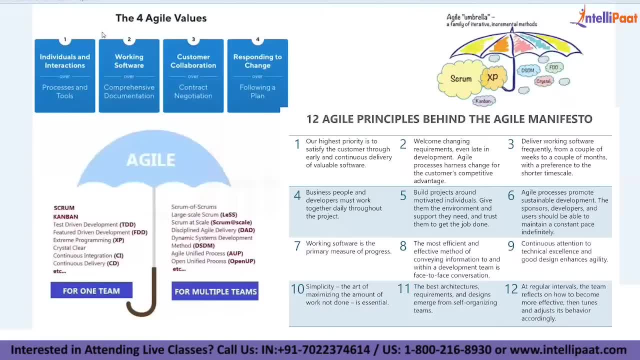 there is a possibility of changing doesn't mean that we do the changes with immediate effect. it is not practically viable to do. because that's a practical difficulty, because whatever the spirit sprint we have created for the sprint, there is a scope will be defined for that particular sprint. so 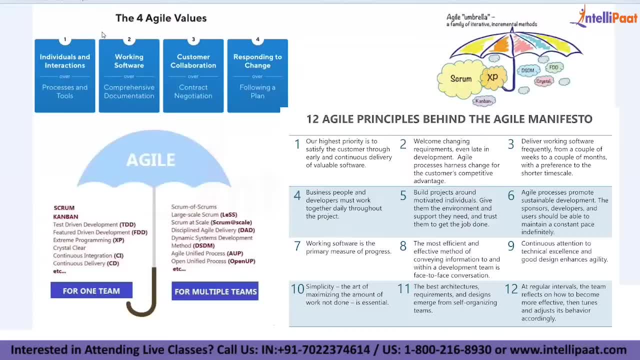 not be deviated. if scope has deviated, obviously the sprint, the total plan of sprint focus, will be deviated by the team members, so it will be impacted on the particular sprint, what we have initiated and what we have planned so far. everything will get deviated because of this. 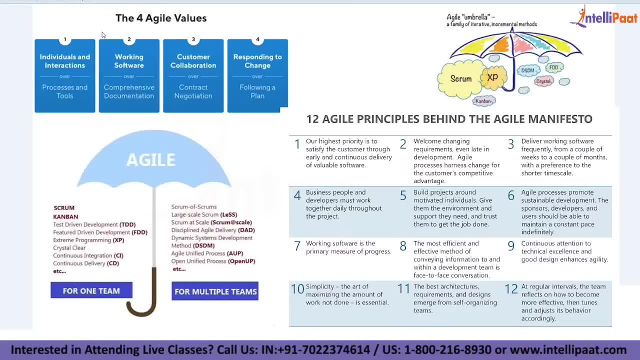 so end of the day, that is the team responsibility. team has to decide. team members have to decide whether is there any deviation can be accepted here or not. so it doesn't mean that responding to change is accepted doesn't mean that we are accepting with immediate effect again, 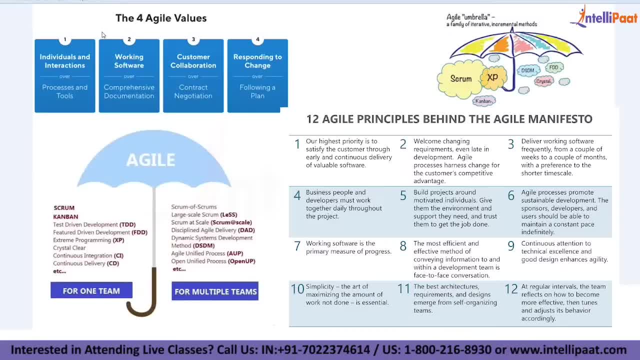 to terms and conditions, that it has to be accepted by the team members and again, negotiations will be taken place with, interactions will be taken place with the product owner, with the proper consent, whatever we have, and all, finally, implementation will be taken place further. so, otherwise, there is no changes, nothing will be done with immediate effect. so that's not practically possible and we 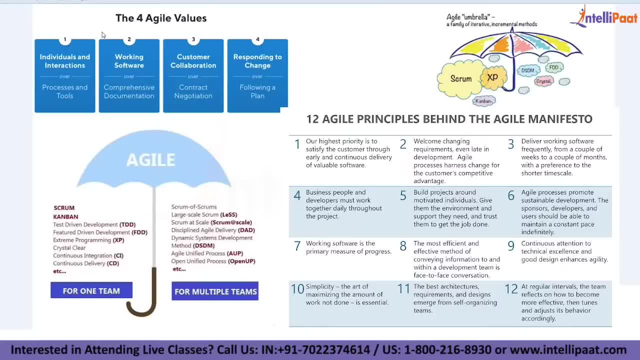 don't do that also. so these are the four different agile values which normally we use in agile. so one is individuals and interactions is what we do first, because we'll be focusing more on individuals, and interactions means day-to-day interactions will be there in agile. this is what one value, first point. second: working software. we are 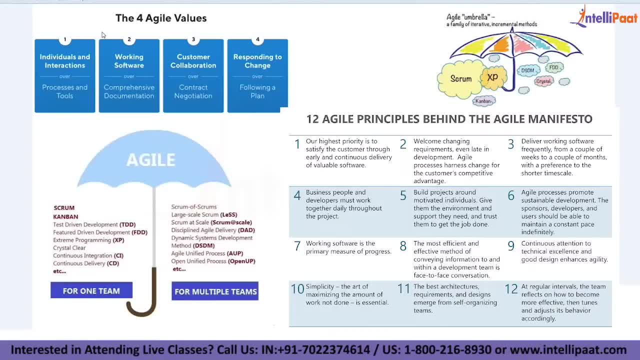 directly working on the software, as we are not following any kind of documentation as separate, because interactions we have made, so based on that, we start understanding and start working on it. that's how generally it happens. third is customer collaboration. customer is collaborating with us all the time, so what are their expectations? everything will be known to us so that we can do it. 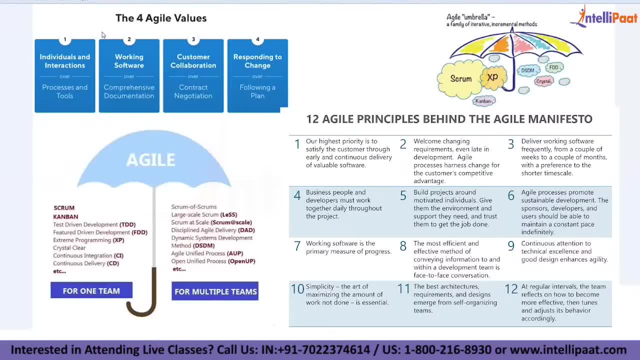 properly. next responding to change. whatever the changes you want to do, response is based upon the responses and all that changes can be done accordingly. so these are the four major values. this is also called as agile manifesto, so this is basically. agile is being uh, focused more on. 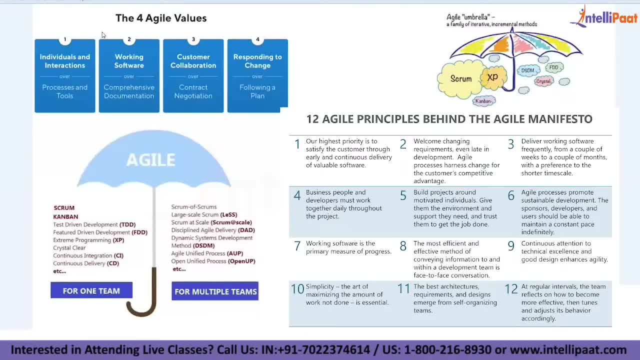 if you've got your. if someone is asking you how different from traditional to agile is this? this is the difference you see from traditional to exact on a high level. note, in terms of the agile is concerned, this is: these are all comes under the agile values, or we can call it as agile manifesto. 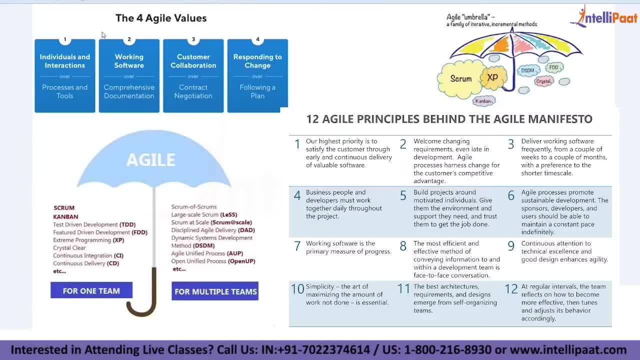 also so this is all about agile introduction, how it is different from the traditional to agile itself. at the same time, what are the different, different values, as well as the manifesto principles which we follow in agile. if you see agile- see, agile is a umbrella right, if you can. 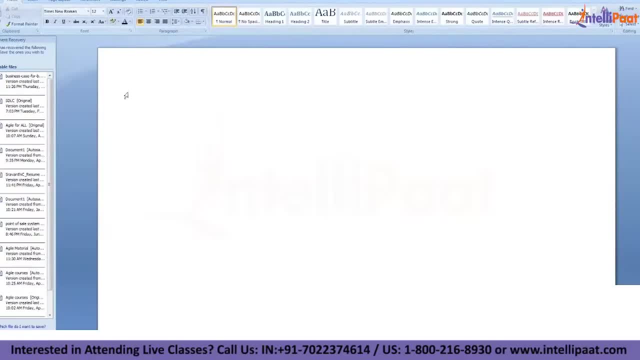 take agile as an umbrella right. so if you see agile as a way of approach or umbrella or a methodology, whatever it is, there are different, different screen work, frameworks, processes will be there under agile. one is scrum. scrum is a framework. remember right, scrum comes in the 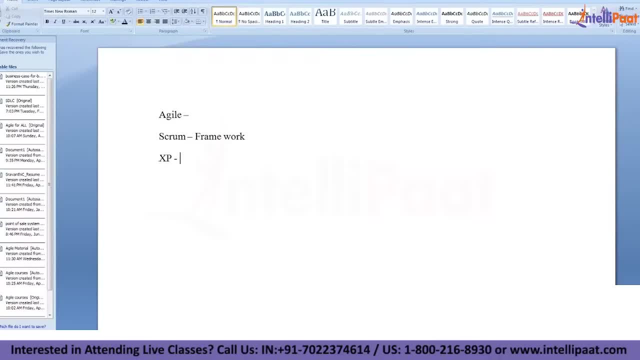 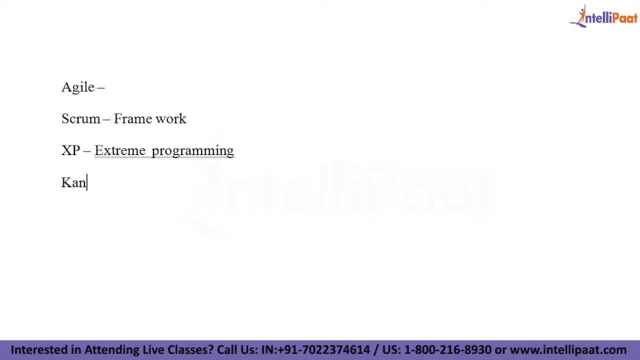 framework. scrum is a framework. next xp. we have xp stands for extreme programming, extreme programming. next we have one more called kanban. right, so kanban is a model, is a development model. especially this is a japanese model. kanban, which is something close to lean process, all that stuff, this is one. 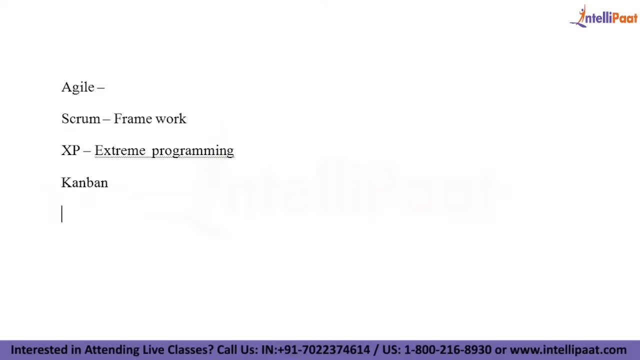 thing, kanban. next we have a other process called rup transfer, rational unified process. this has been powered by rational software corporation. earlier it was there rational unified process right and next we have other process. earlier normally this agile, and all everything is derived from this, dsdm. 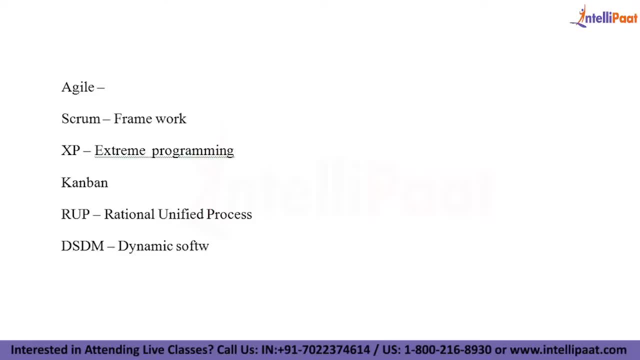 stands for dynamic software development methodology, right, so these are the different, different frameworks and processes which are there under agile. somebody follows scrum, somebody follow xp, somebody follow kanban, rup dsdm. so normally the all, not all these major ones are these, these three i can say simply because 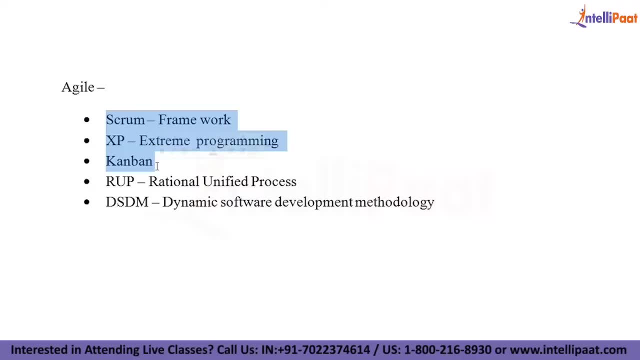 i don't want to make you confused by putting all the information here. major major things is scrum, xp, kanban. these are the three major things which will be part of under agile. some people follow exclusive scrum, some people follow exclusive xp, some people follow kanban, sometimes scrum with. 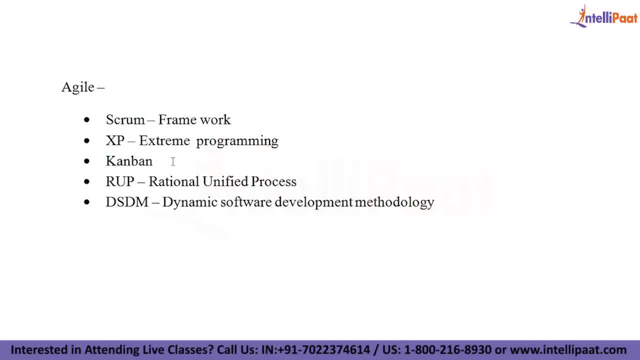 kanban combination right. that is what we call it, a scrum ban. scrum ban is, i'll give you an example, for example, your work. you are providing a solution for a manufacturing and automobile sector. normally, automobile people uses a process called lean lean process. in the beginning, in the first session, i think i might have given this point to you, if i 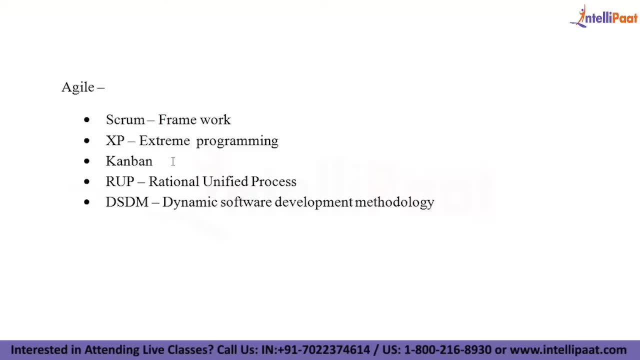 remember- i'm not sure- lean process. lean process is the one which is being used to minimize the uh production loss in terms of the time right. so they want to maximize the effort and they want to maximize the effort and they want to maximize the effort and quality delivery, all that within the life limited timeline. they want to make utilization of the time. 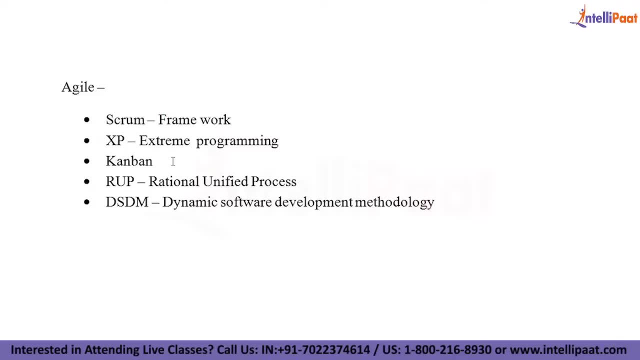 quality of time will be used. wastage of components, wages of time, everything can be minimized using this lean process. in the clean process, there is a process called kanban, which they will be using here, customer, right now, whenever we are following a practice of scrum, ban what we. 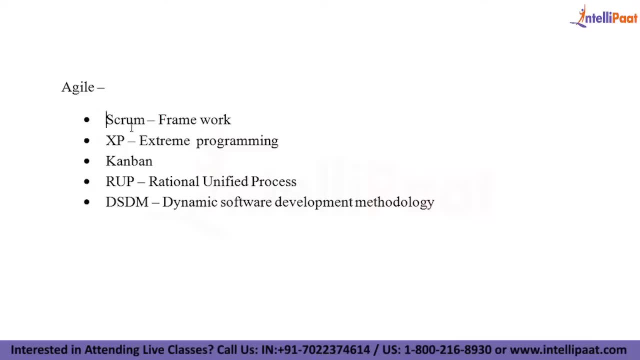 do when we are implementing scrum. we follow practice of scrum and kanban also, sometimes scrum with kanban, sometimes scrum, sometimes only xb right, sometimes scrum with traditional model. something like, as i told you in the beginning: right, we follow agile. underline: normally we say that we follow agile. 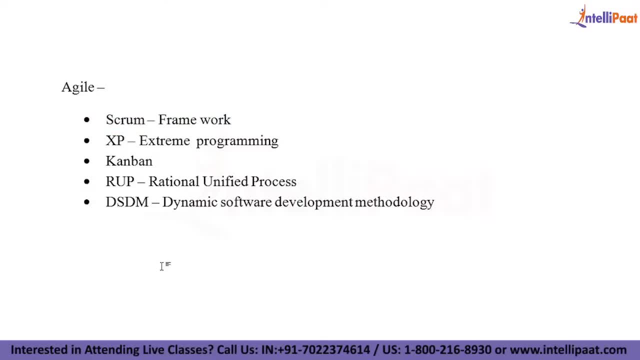 but whatever the practice of development, we do everything we follow the traditional way. hundred percent agile won't be used. traditional way of approaches will be the major part. sixty percent traditional, forty percent agile. i don't say wrong, right. so depends on the team, depends on the experience, what they have. so it depends on the comfort. this is what we are going to use in the next session. 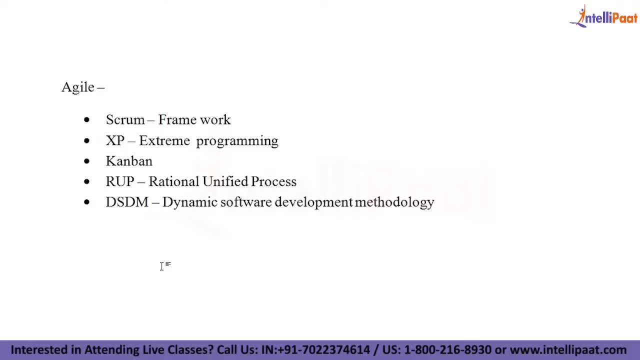 is also very important creation and this will be varied. so, whatever the frameworks, processes and all everything part of agile, somebody follows scrum, somebody follow xp kanban. it's entirely different. depends on their experience, what they have earlier at the same time, what they believe. for some people follow Macron. people think that scrum is the right thing, right. some people 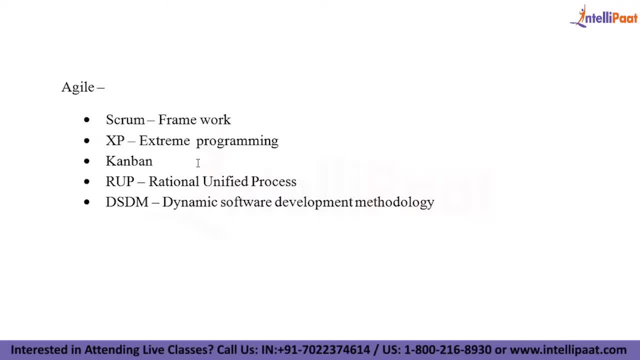 feel that xv is the right one. so, end of the day, that is their discretion, team and management discretion. with that, whether which which process they are following, and all everything, will be it by the team itself they have to take the decision on. uh, not by the anyone else apart. 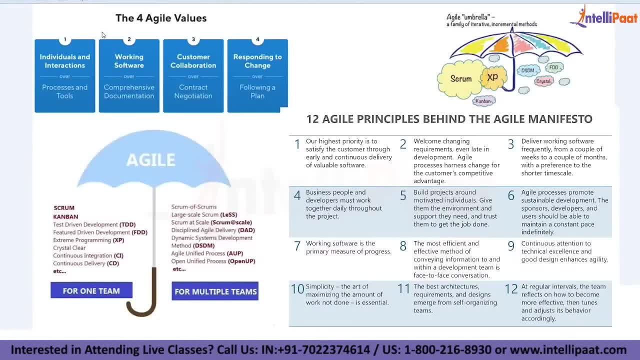 right, so they are the one who is taking the decision on that. clear to you? is it clear or not? normally, when it comes to the product owner role, customer will be given you the person right. the customer will appoint a product owner. for example, i am the one right, so customer will give is a. 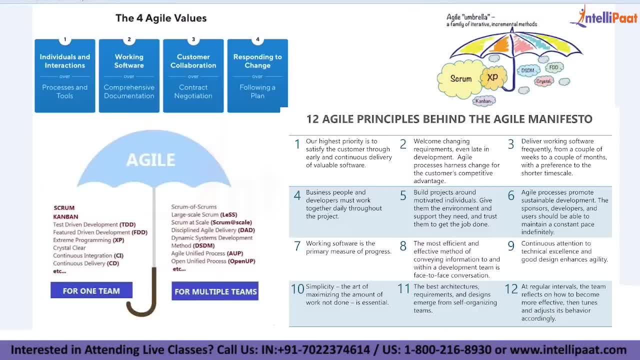 product owner. he'll be taking care of all the product requirements and all everything from here onwards. he'll be organizing all that stuff right. this is one thing. for some projects. this is how it happens. customer will give you the product owner, point number one in some cases. 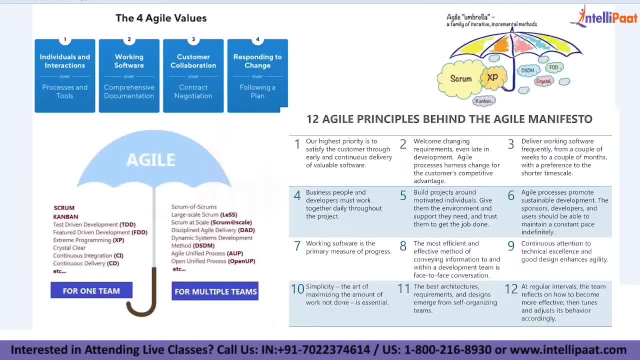 there is no product owner given by the client. so whenever the team management, whenever the management has decided agile and all that, so they recruit product owner as separate, this product owner is the one who is working on behalf of the client. that's how it happens that one or this and whatever the principles am i explaining you here. what are the 12 principles? 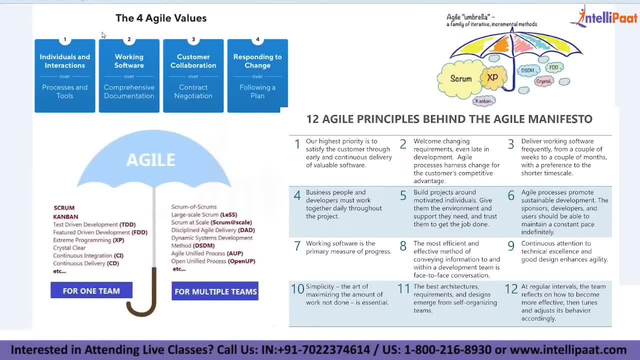 and all that, everything are behind under the agile manifesto. the same points. whatever the points we were discussing on the value system, the same thing will be repeated here. the first point under agile principles is that we give high priority to the customer satisfaction, so customers will be satisfied when we are delivering it on time, followed by this: whatever that they are expecting. 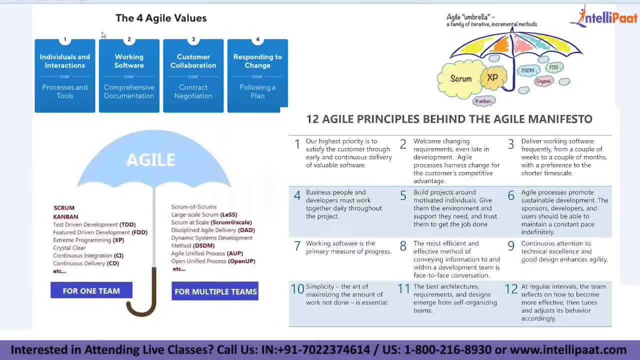 from us. so whenever we are delivering, customer will be happy. so the major priority, especially in agile, is to provide the value-added services to the customer within the time limits which was finalized. so far. right, this is what generally, the first priority. second point is that changes can be done at any point in time. 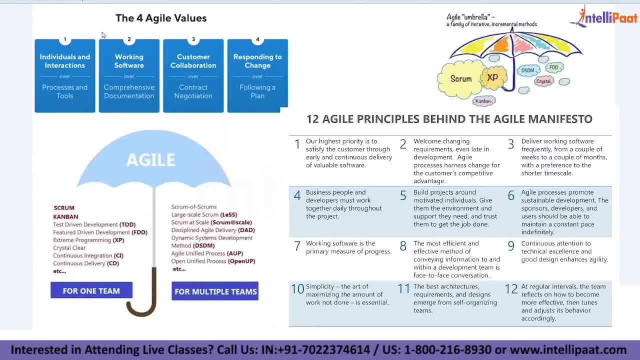 whatever the changes we want to make in the process of application development, even in late development, normally in the traditional way of approach, if you see changes, whatever required us to do in between the project, in middle of the project, is difficult. i don't say it is not possible, it is difficult due to the 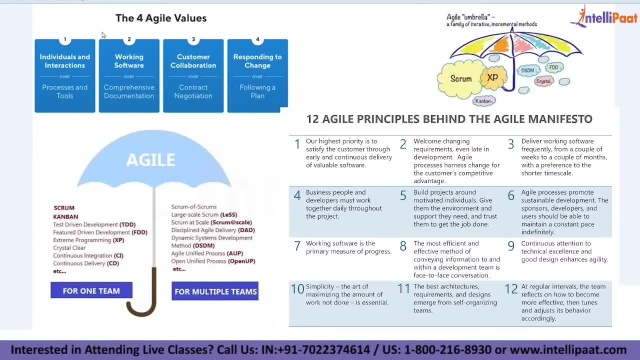 again, you need to go for analysis, right? so someone has to do the analysis part. someone should do the planning and design part. after that someone has to do the coding part. so a lot of people are involved, right? so different, different people are involved for different activities. so coordinating them- again, reworking on that takes a lot of time and energy, manpower. 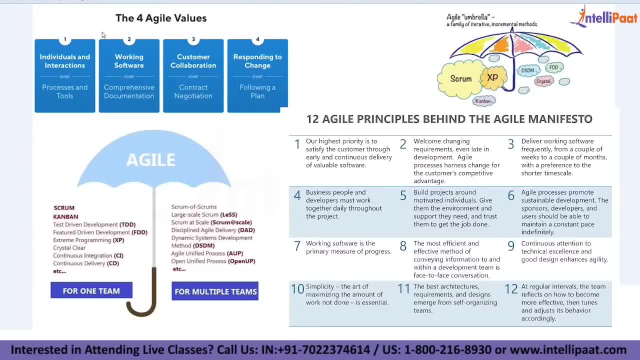 automatically. when manpower has increased automatically, operational cost will also get increased. at the same time, we have to make sure there should not be any kind of technical complex, but whereas, when it comes to the agile environment, the approach of agile development will be in such a way where, whatever the work we are doing, everything is something. 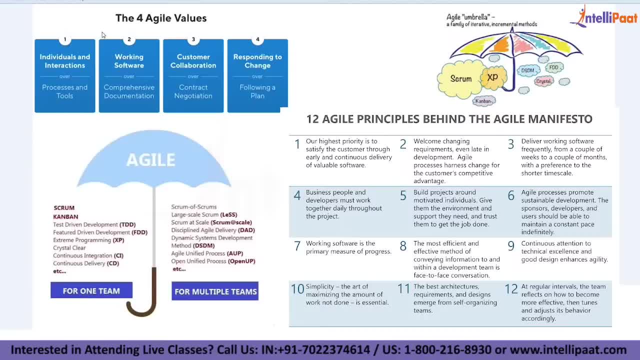 relating to the user story, because this is how generally user stories comes. you the user story. i will tell you sometime we'll start, i'll explain about it, so we'll write it on a shorter format. in simple terms i can say whatever the requirements we have normally in. 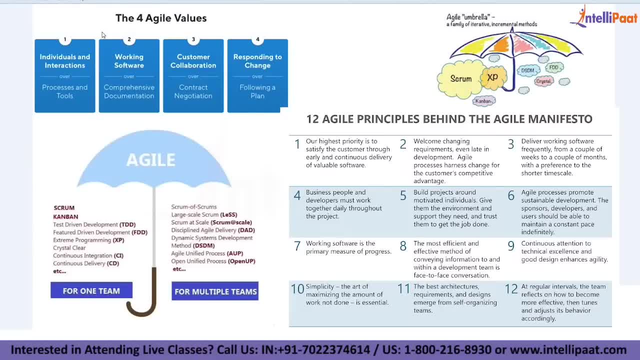 the traditional way of approach. we write documents something like brdsrs, all that and whatever the functional, non-functional requirements, everything will be written on the document itself. but whereas, when it comes to the agile environments is concerned, whatever the requirements we were writing, everything will be written in a shorter format. that is what we call it as. 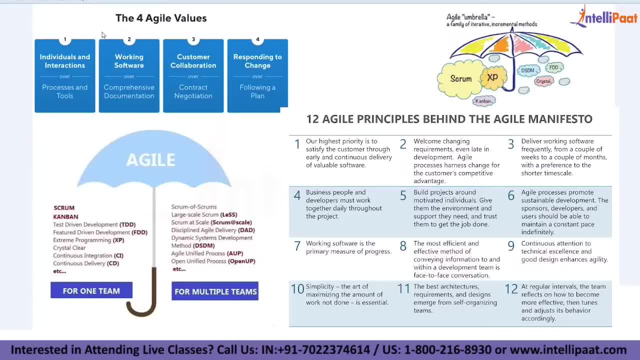 user stories transfer so that user story has independent on its nature. so whenever, whatever the changes to be made into the existing one can be done accordingly. so that is the second point. the advantage in agile is changes can be made at any time, any point in time. but there is a difference. 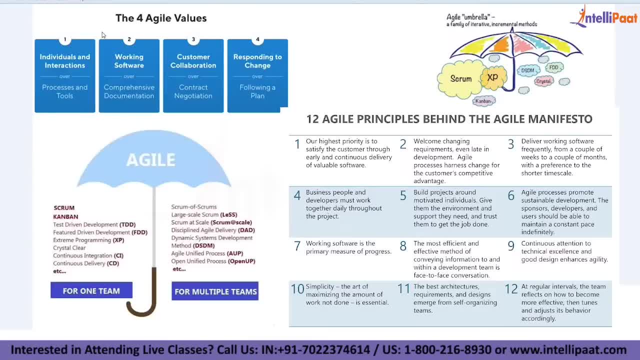 again, if you remember, yesterday i have told you, whereas in scrum there is some difficulty, means there are some challenges, whereas when you follow kanban, practices and all that can be done, but still hundred percent, as i said, like hundred percent, there is no this thing. so there is, but so. 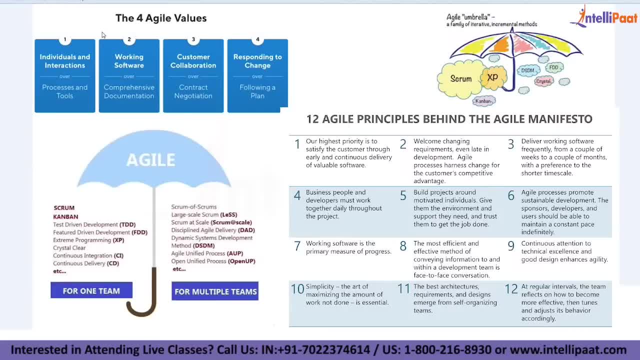 it can be manageable, right? so that is the second point. third is that whatever the delivery of the work we do, normally it will be on the beats time, usually in agile environment, if you see the agile as an high level, especially in reference to the traditional model when we are comparing. first, 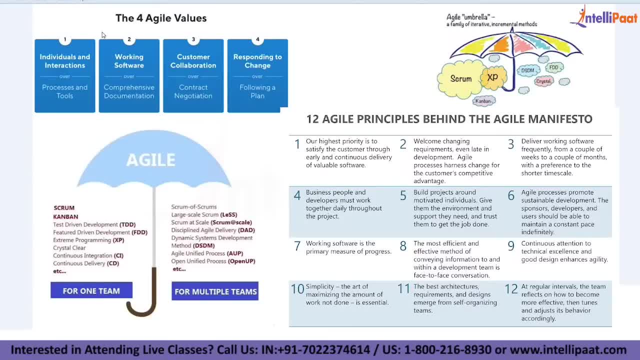 at least to complete project. it will be taken not less than eight months to one year, right? so this is the. this is the minimum thing for any project to start and to complete it. but whereas when it comes to the agile environment, as a stated earlier, this is all focused more on the release, because release planning is what will be done. 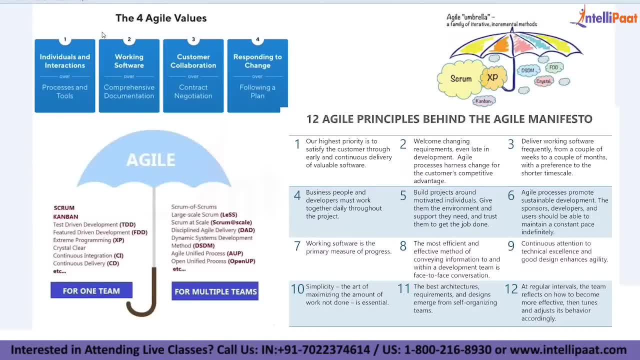 prior. so, based on the release planning, implementation will be taken place. so, whatever is that we have started or whatever the release we have initiated so far, based on that, implementation will be taken place. so when we talk about release, release is not something full for the whole project, right? so 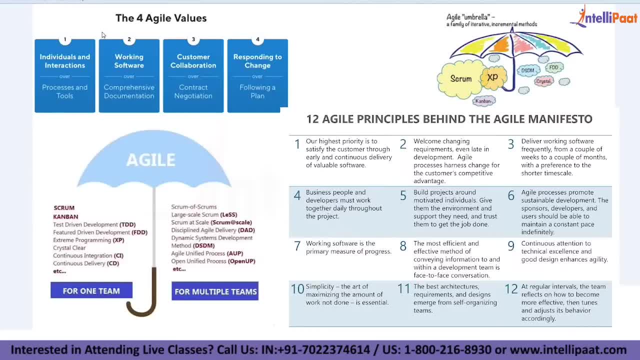 we are not taking the whole project into an account. whatever is required for the customer is what will be taken initially so that piece of work will be done. we are dividing that into consideration. assume that the release planning we are making in three months of time. this three months can be divided into weeks, right, for example, if it is three, three. 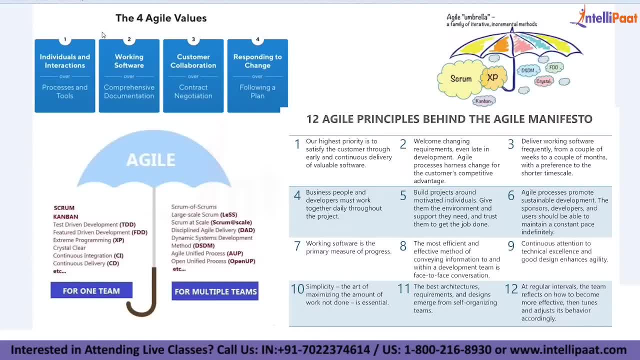 months, four into three and, on an average, 12 weeks. right again, these weeks will be converted into days, days into hours. so, whatever the delivery of work we do, especially in reference to the agile itself is concerned, everything in short, iterations. when we talk about short iterations and all it. 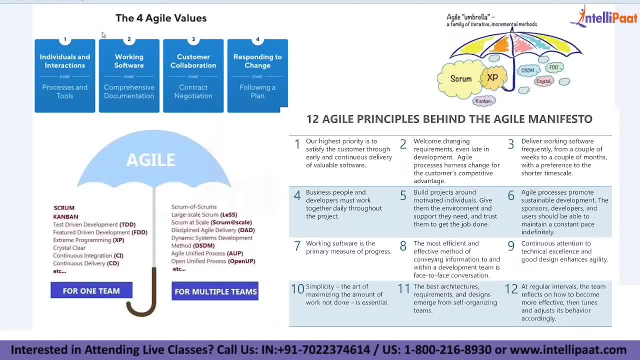 will be based on the weeks. normally, weeks are the one we consider. weeks are the point we consider into. we'll take into consideration. weeks are the one we'll be taking into an account. this is the third point under agile. the fourth point is that even business, people means business. 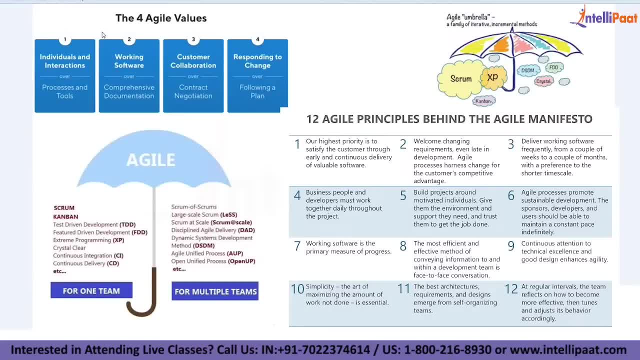 cross functionalities. in simple word I can say. fourth point is that cross functional teams because there will be a difference between the business functional people as well as the technical people. because functional people knows about the functionalities of the existing process, all that stuff. maybe a business analyst is one, one of the person who knows about. 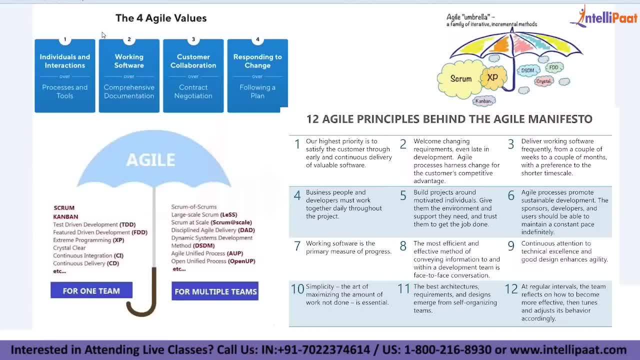 the functionality. not only that, even business users, all that people right at the same time, technical people. technical people means development team, testing team, all that normally, both all these people, usually these two people, will do different things right. functional people were externally supporting us, except BA. remaining other people will be within the project and they work accordingly. 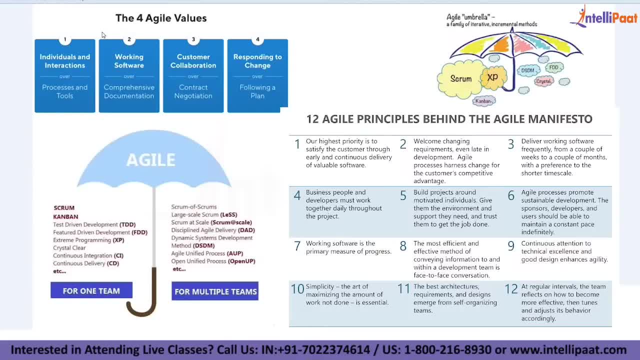 this is how usually the structure follow everywhere, but whereas when it comes to the agile itself is concerned, even business people, development people, all these people are under the same platform. this is what we call it as cross functional teams. everybody works for the same cause. everybody's target is to complete whatever has been identified and finalized right. 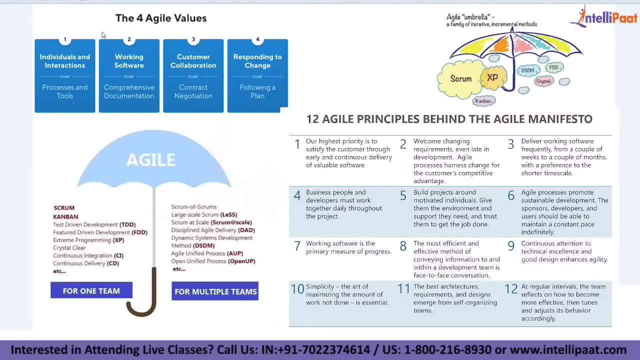 so everybody works towards that. hence, there is nothing as that. I'm only confined to this because, especially in agile, the major difference you see from traditional to agile is that you need to have a multitasking ability. that is essentially needed. of course, even though you are a developer, you may 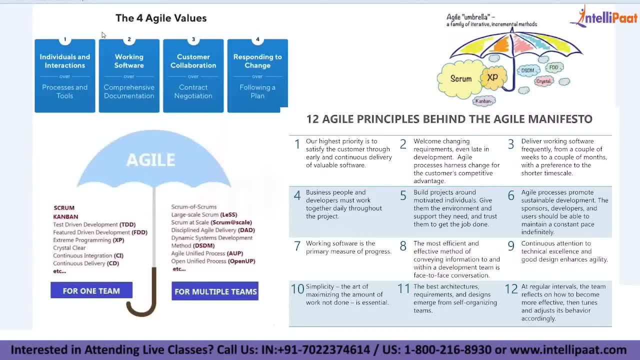 be expert in development or, as a part of that, you may be good at coding all that stuff. so, apart from that, what else? the what else is required for us is to know about the other aspects as well- means you must be good enough to participate in a group. I'm saying right. 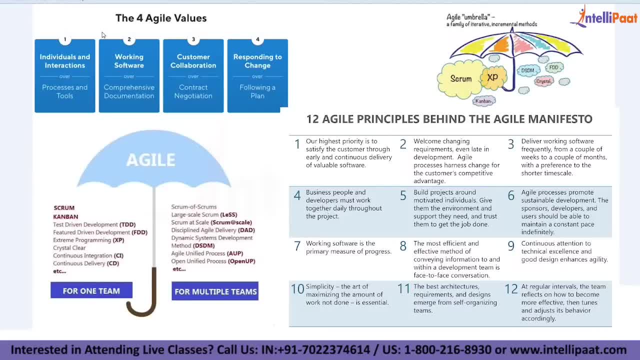 not as an individual. in a group you may be required to work as in into analysis. maybe you may be required to participate in planning and design, not only into implementation testing. if there is a requirement so we have to cross, we have to do the those points as well. so that is one thing. 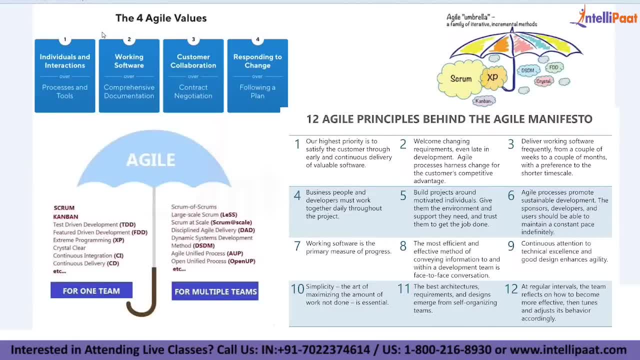 something essentially needed in agile because small iterations. we are taking that to time frame. it's completely based on the time frame so that if someone is absent on behalf of someone, someone has to take that responsibility. this is what, generally, the fourth point is. the fifth point is that 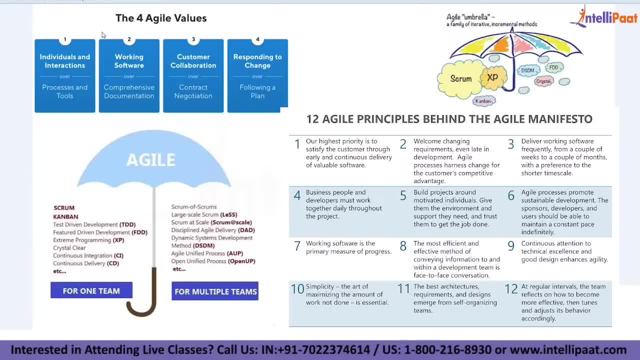 whatever the projects we were developing, everything is based upon the motivation of the individuals. all that, so it's all a group of activity we do. everything is depending on the trust as well as the motivation among group, which is essential needed especially happens in agile as well. next, the sixth point is about sustainable development. 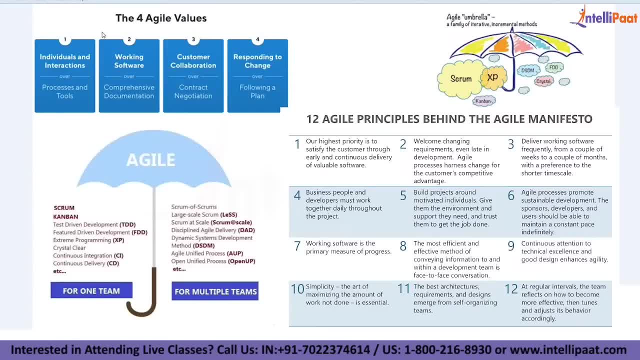 whereas, whatever the work we do, everything is in sustainable mode means you don't see any kind of gems and all everything which are huge in percentage, right. so because whatever the changes and all everything, we were identifying those changes and we are doing it parallelly- depends on the possibility: whether are we keeping it in the present one or we are transferring it to the 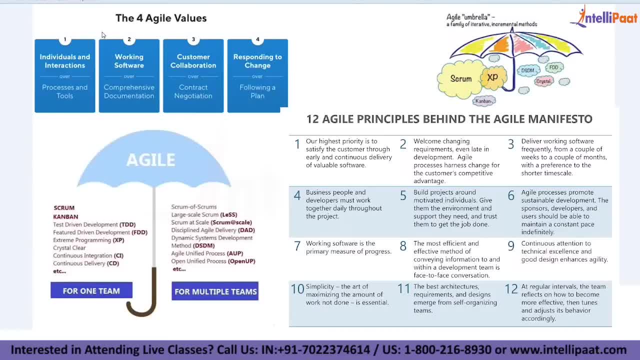 next one is what we're doing anyway, as I mentioned earlier. so there is a possibility of sustainable development, especially in agile is possible when we are comparing with the traditional model, because if there is any volatility in requirements taken place, that is really difficult and challenging task here, right? so, whereas that part won't be there in agile, because we have an 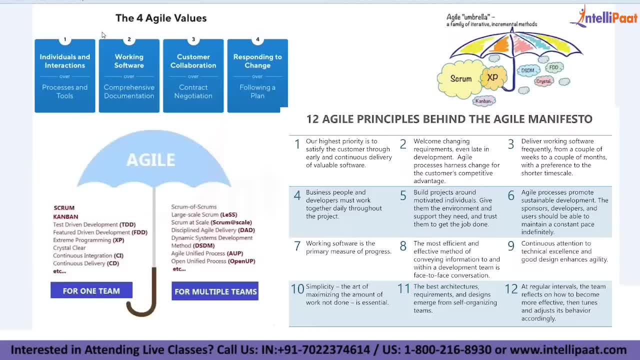 assurance that changes can be made at any stage. so structure of agile will be something of that sort, right? so this is the sixth point. at the same time, whatever the work we do, the seventh point. when it comes to the seven point, whatever the work we see, everything is based upon the. 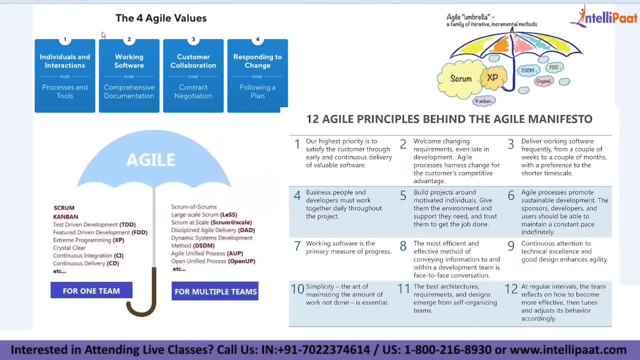 progress of the work. right, measuring the progress of the work is what measuring of the work is means. whatever is promised, what we have assigned, what we have completed, is what we see. this is what generally happens in agile. at the same time, 80 point is about face-to-face conversation, if you. 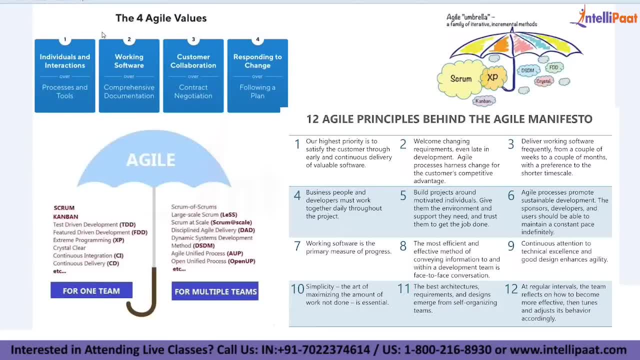 can see the first point I have mentioned you, individuals and interactions- where there will be lot of interactions because, especially in agile, if you, if you are working on agile, especially in agile teams, all that stuff, whatever the interaction we had, and all everything is the major aspect- means face-to-face interaction. 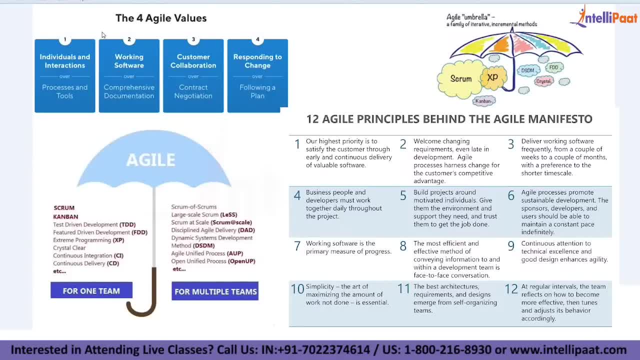 among the team members is what normally we do, normally this kind of nature you don't see in other ways in the traditional model. if I'm communicating, for example, if I'm being a business and decision right, so I am the one who is translating my requirements into the technical 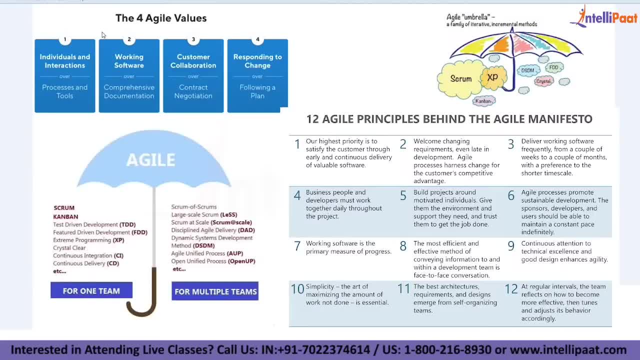 format or a business related format, and preparing documentation. my documentation speaks not me all the time. I will speaks when it is required, but most of the times my documentation speaks. you know, on behalf of me, what is that I want to present. everything will be there in the documentation, but there are some difficulties because sometimes 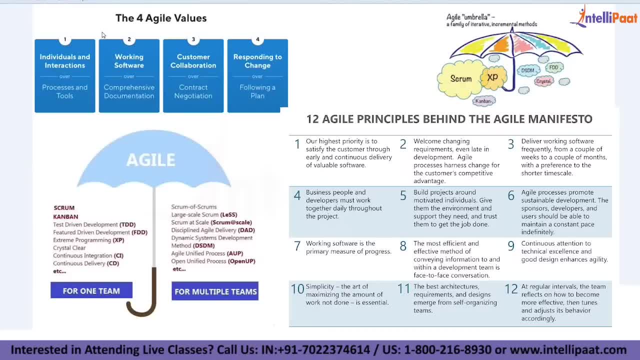 people may find difficulty to understand what I have prepared. it may be due to because of my mistake or sometimes maybe they may be in a position to may not be in a position to understand those properly. these kind of problems might be arrayed in long run because the projects will be of very 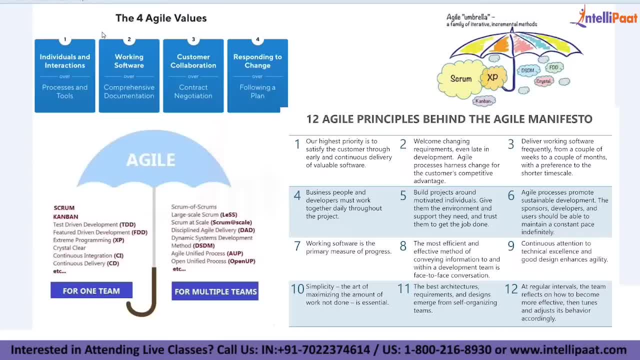 very large in size. right, it will not be there for two, three months. all that stuff will be taken at least here a year and a half to complete. so it is always helpful, especially in terms of the short term deliveries. it is always beneficial to have a face-to-face conversation among the team members. 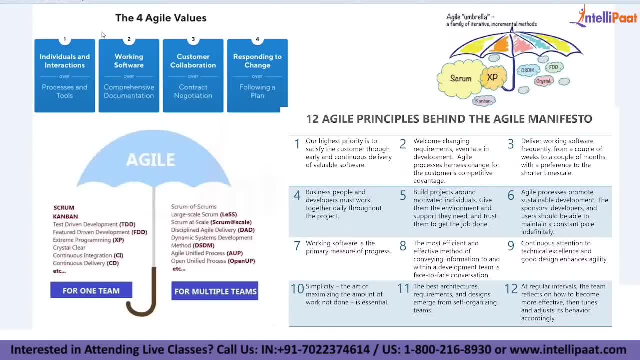 which is essentially needed, but because we don't have that much time even to prepare any documentation, because, for example, if I am the one who has understood the requirements, translating into document and again providing it to you, it takes a lot of time for us. so that much of facility you don't see in agile. so that's the. 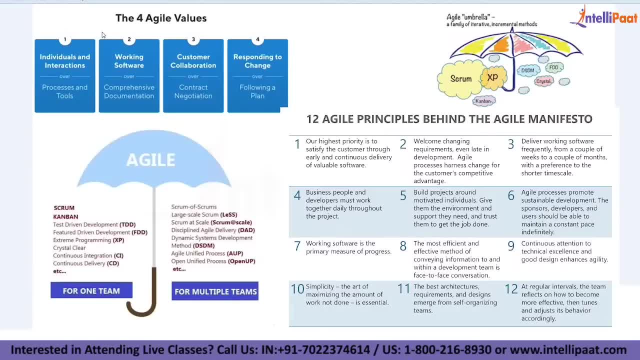 reason why it is always we are depending more on face-to-face conversation. that will be. that will happen in a format of normally we do like scrum meetings and all we call it as scrum meetings. usually scrum meetings will be conducted day to day, every day for about 10 minutes. we sit, we. 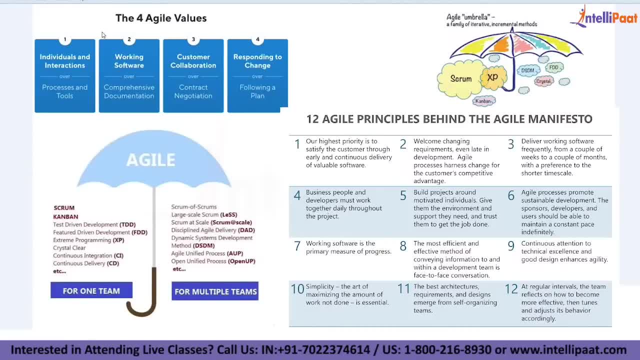 discuss about. the team members will discuss about what is that we are doing right, how we are doing so. what are our tasks to be completed for today, right? so what could be the challenges, how to overcome that? so everything will be discussed on day-to-day basis, so there is less part of, less chances of the complexity or 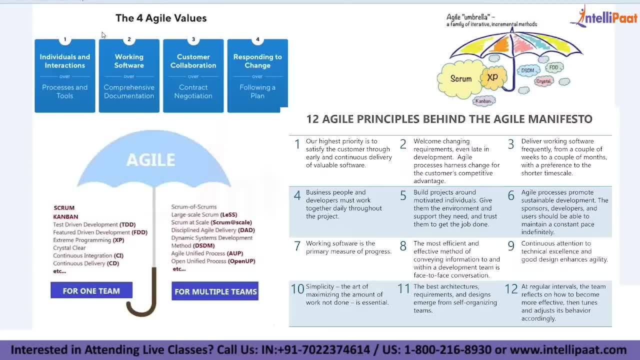 less chances of the confusion over the team members due to this pro video, this addressing, I think, interesting mode, right addressing mode of conversation. next, commute: continuous patient attention towards technical excellence is also there. that is one thing, at the same time, part of it, which is not done. so for that generally there are some report, Generations and all everything we 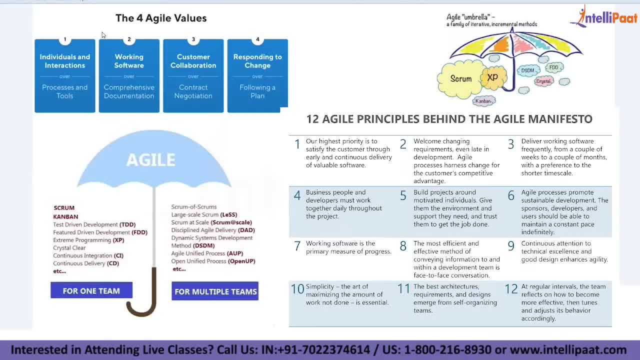 do. usually, scrum Masters are the people who normally prepare this Velocity Chats, all that. so, using those Velocity Chats, they come to know what is that promised and what is that we have completed. so how many more? how much more work is there for us to complete? so for that, what is that? 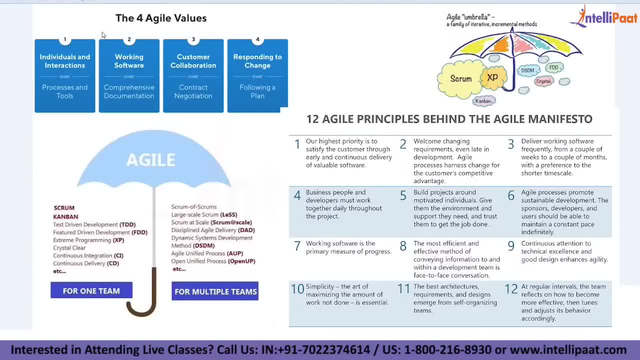 decision to be taken based upon the reality, what we have understood. all that will be done by team scrum Masters. usually they prepare different, different charts. that's a different thing. next, architectures, requirements and all everything will be done by the team itself. because you don't see any exclusive architects. because if you see for any application development, especially in 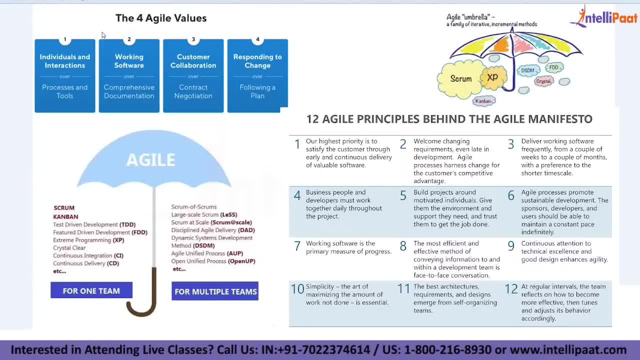 reference to the traditional. I'm comparing. you might have heard about a role called solution architect. solution solution architect means the person who develop architecture for the project, who creates a roadmap to develop the project from the technical point of view. unless, until, if there is no technology which is 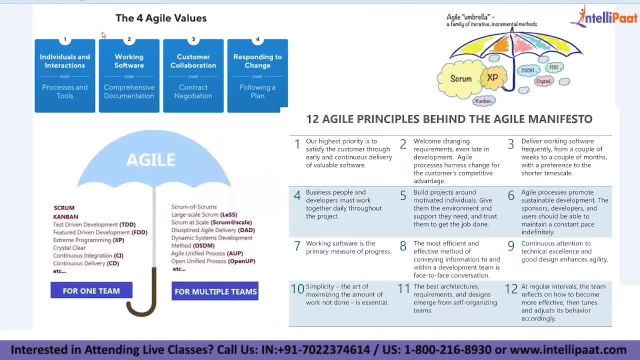 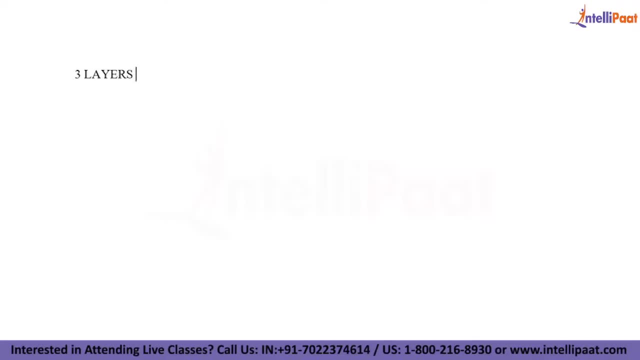 integrated because when you are developing an application, application normally if you see from a high level mode will be of three different layers. normally first layer explain you on the board. we understood better. normally if you take any project, project will be of three layers. right, the first layer, we call it as presentation layer. 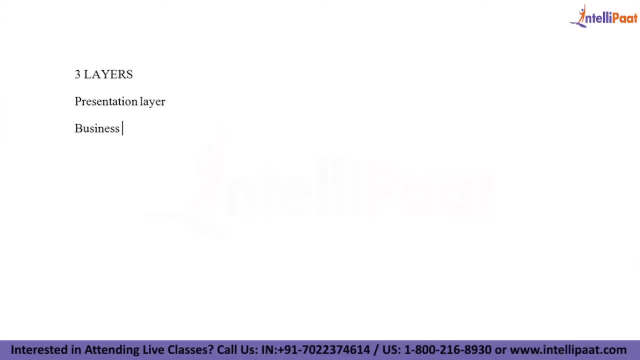 first thing, we call it as presentation layer. second, we call it as business or logic layer. first will be called as data line. there is a constant connectivity between these. among these three is important. presentation layer means what you see on the screen. business and logic layer means whatever the code we write, everything comes under business and logic. for example, 1 plus 2. you. 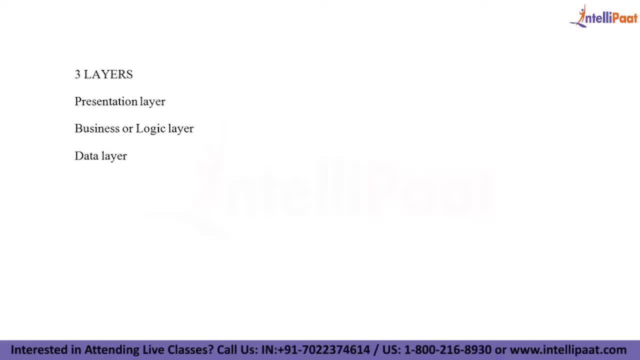 have given. whenever you press Enter button you are getting a reply called three. being a user, are you doing an addition Here? note: there is a program which was written by the developer in back of it for addition, not for one plus two, right, it is one plus two, or it may be 500 plus 300. so a developer has written a program for addition. 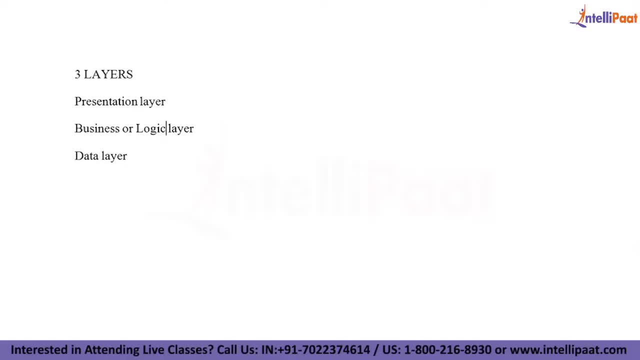 so, based on the program, what they have written and all you can see the output there. right, that is what generally so, the logic layer, so where logic will be implemented here accordingly. this is the second thing. the third is data layer means whatever the data we are uploading right through. 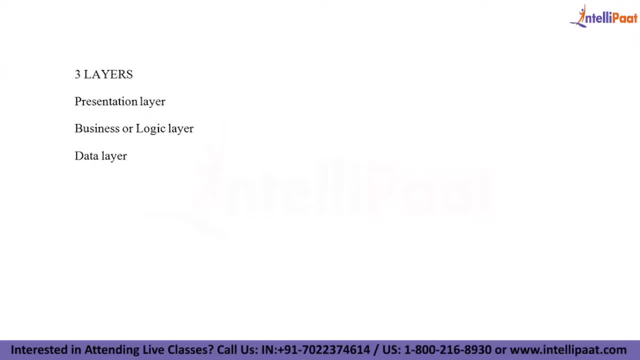 we are presenting through presentation layer, everything will be stored on the data layer itself. of course, for the database designing, everything has to be done by the database designers: all that follower, followed by this, if you are extracting the data, for report generations and all everything. so there is a connect among these presentation business logic layer data. 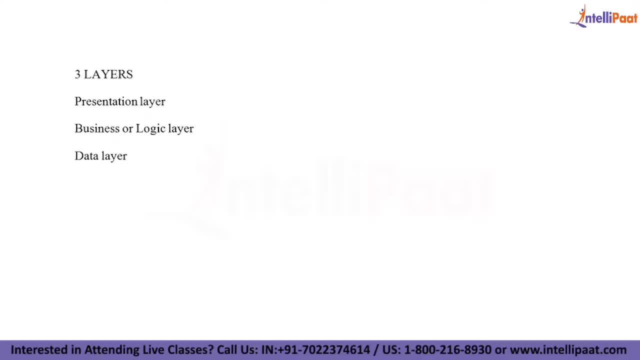 layer all that stuff. so, which is something technically connecting with this. this is where generally a solution, architects are the people normally come from the technical background, because architects are the people we consider them as technical people, not the grandpa's teem and grandpa's auperatorial architect. so the way we doing those things, 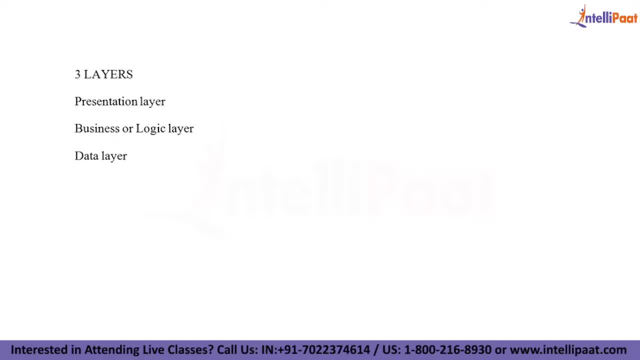 is. we are using the Maxwell's problem logbook, which is forces, the simpler version, which the functional ones, because functional ones never become solution architects, because solution architecture is completely a technical thing, whoever is having more than 10-15 years of experience in developing technological technical applications for different, different clients. 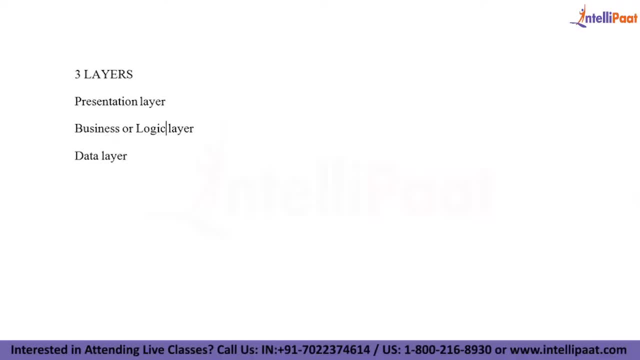 whoever is having vast knowledge about the technology- transformation, programming, coding part, all that stuff- so those people will become architects. normally, solution architects is highly recognizable and important role for any organization, especially for project development. it is one of it. i don't say that remaining other other roles are not important, but this is one of. 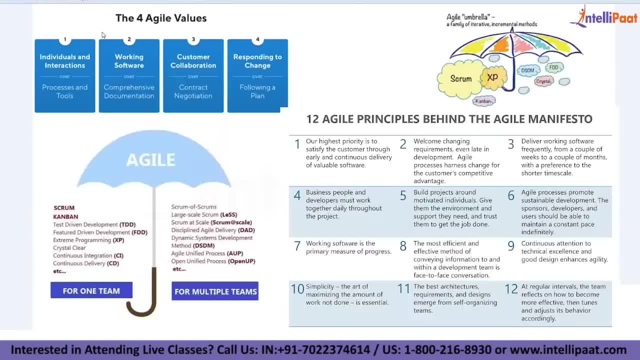 the important role like this is what generally the layers and all about. so there will be architects, normally traditional model, you can see the architects, all that stuff- but whereas in the application development in reference to aj, whatever the architectures we prepare, everything will be done by the self-organizing team. self-organizing team need not be a developer, even architect can. 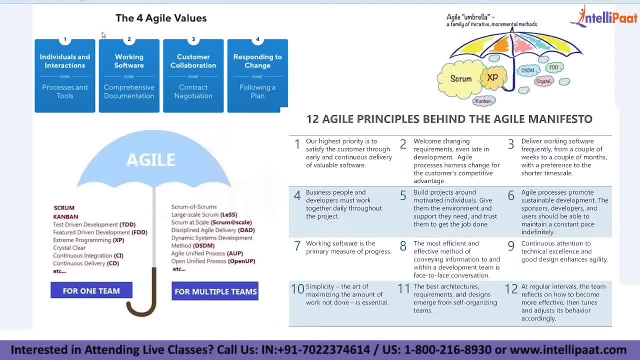 also be a part of self-organizing team, right? so you don't see any person as separate, even an architect, whoever are there as separate, right, so that architect may also be a part of self-organizing team sometimes. otherwise, these people are well experienced in terms of the technology, all that. 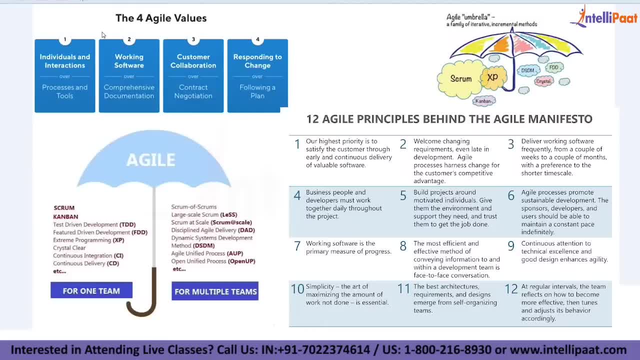 stuff. these people can also become architects, so they can develop architecture, as what they understood so far, all that. so this is the way it is done. so that's the way it is done. so this is another point here. at the same time, whatever the requirements in this behavioral 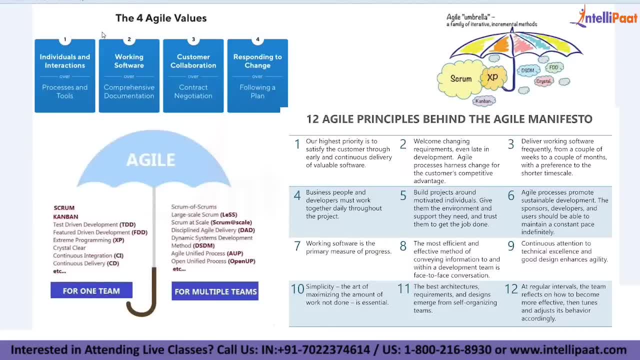 attitude, behavioral tendencies, understanding about the team efforts, team works in regular intervals and all it is also needed. so these are the major 12 principles which are there behind agile manifesto. so whatever the points we have discussed in the agile manifesto, the same thing will be reflected under the principles. now we were shifting our focus from agile to the 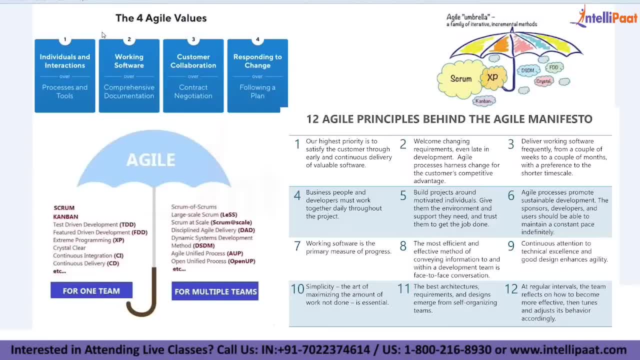 next level. so the next level is this: you can see this umbrella, whatever the umbrella you can see in an umbrella format. you can see that because, as i mentioned you, agile is a process or a way of approach. there are different, different frameworks and processes will be there under agile. there are 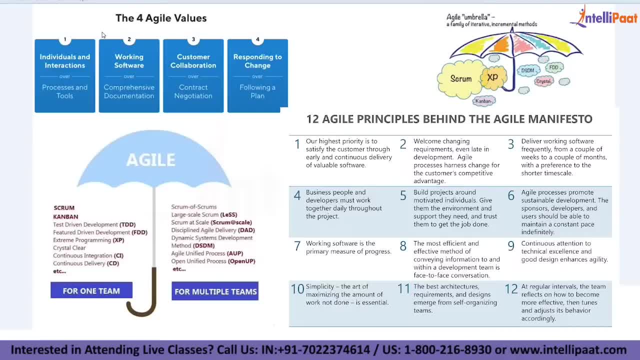 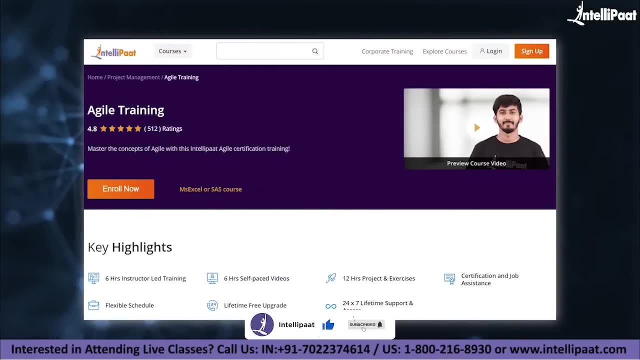 some processes, something like scrum, can ban lean bstm at the same time, rup, rational unified process. all that right. so different, different. just a quick info, guys: intellipad provides agile trading mentored by industry experts, the course link of which is given in the description below. now let's continue with the 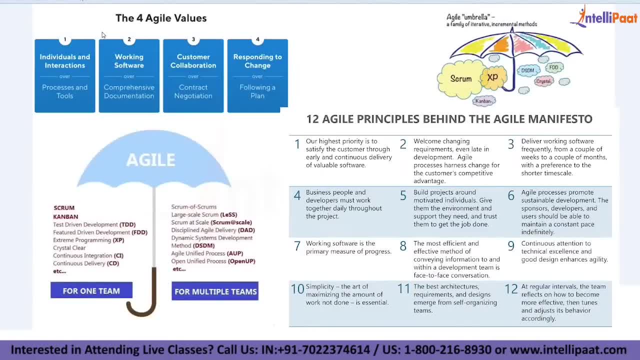 session. frameworks and processes will be there in agile depends on the expertise. what the team is having depends on the requirements and the need. whatever the model we were choosing and all everything will be varied. normally when we talk about team- one team and multiple teams- you can see in this umbrella, you can see for one team or four teams. you can see for one team, you can see for. 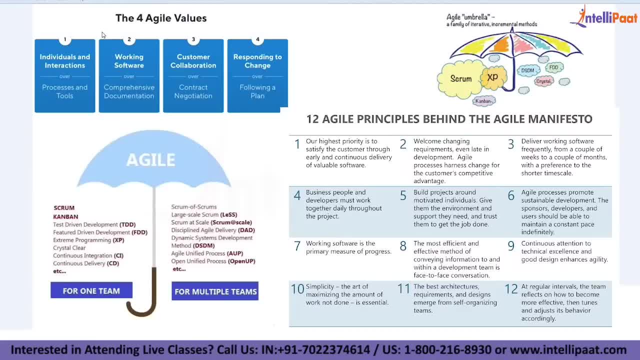 multiple teams, so the difference is very simple. one team means the combination of product owner or a developer, tester. all these put together somewhere around 10 people. this is all called one team. sometimes one team is sufficient for you to complete the project. so when the project size is, 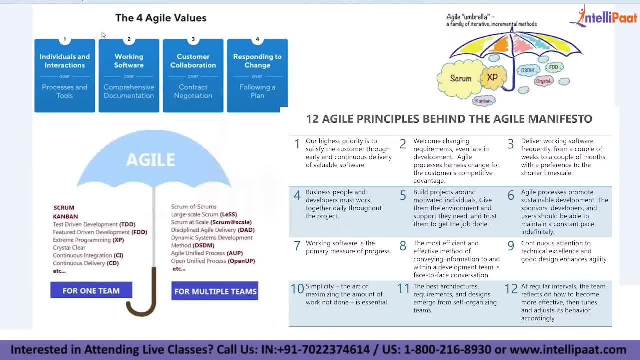 very small in complexities or also small. usually one time is sufficient, but it will not happen in all the cases, because- because all the cases are not something the same, because the case will be different from one another. it will not be the same. so sometimes you require multiple teams to work on the project, especially. 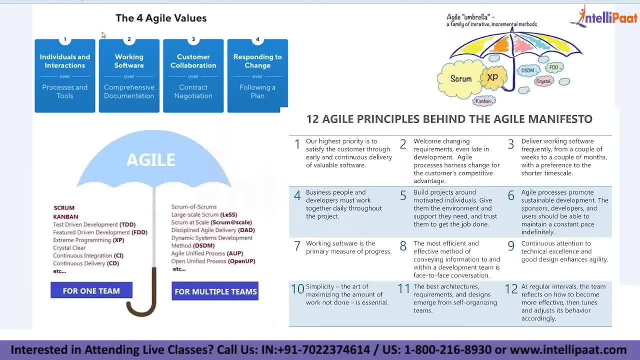 in large scale enterprise transformation level, where, whenever you are transforming the whole organization to the enterprise level format, where you have to deal with multiple things, the application will also be very large in size, complex in percentage, so you require multiple teams involvement. at the same time you need to have a proper coordination among those teams. 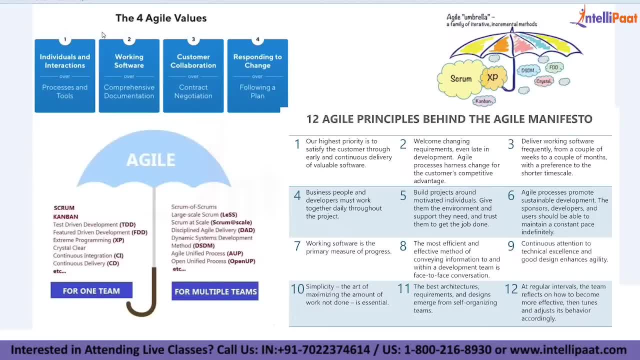 so this is what general is a concept called scaled agile framework. we call so more than agile. i can say in simple terms: i can say more than again. we have other other thing. next level is called safe, safe, s-e-f-e. safe, safe stands for scale agile framework. this one scaled agile framework means agile square. i can. 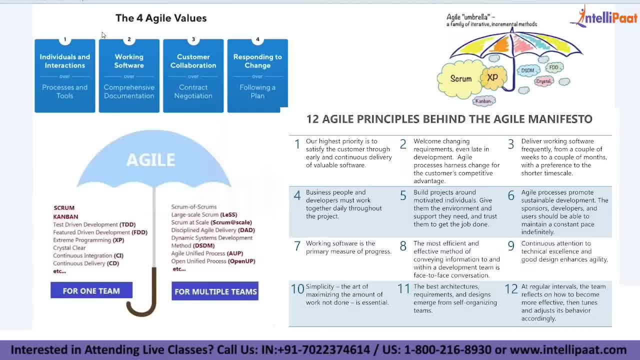 say: right, agile into agile. so this is what generally scaled agile is means for large scale transformations. when you have multiple teams, when there is a coordination is required. so scaled agile framework can all everything use. so you are following scaled agile framework. again, there are different models for that: spotify, all that stuff. that's a different story, so different, different. 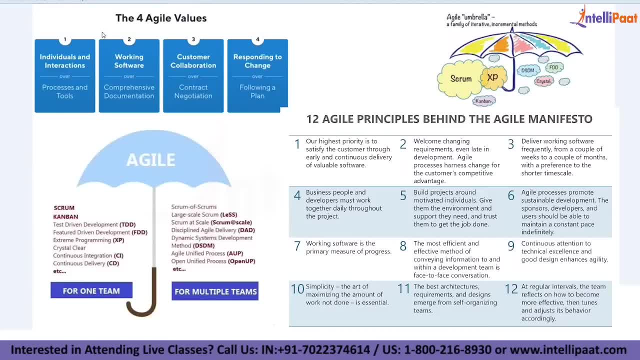 frameworks agile is having. so, whatever and whatever the process and frameworks people follow, they have to be abide with the value system. what agile is having? followed by the principles which was identified and defined so far. everybody has to follow the same. so there is no deviation here. but 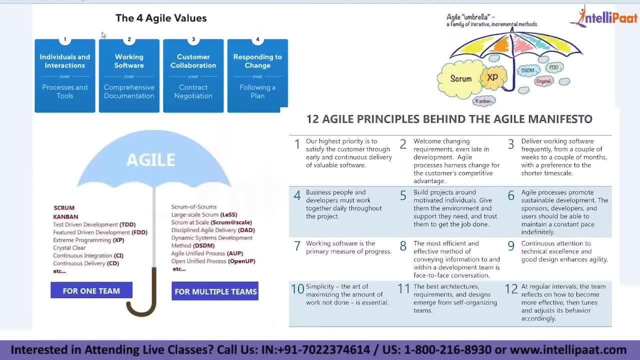 the way of approach when we are dealing the project, and all depends on the kind of framework we have: the process framework, or the process we have identified or we have chosen. at the same time, the kind of experience, what we are having or what we carry. it depends on it. it will not be remain. 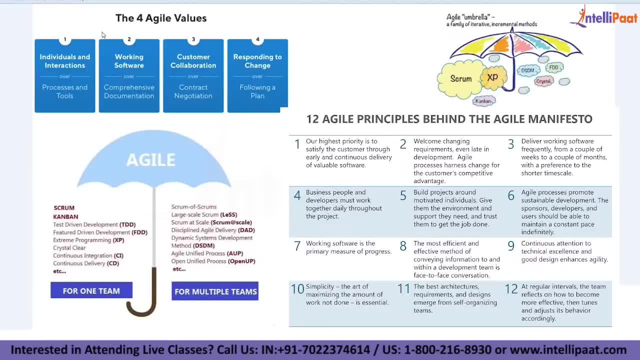 same for everyone. it depends on the kind of expertise what we have, depends on the kind of team, what we have and all everything. these things will be varied here. so but here is a question, because yesterday also i have counted this point, Because most of the people will have a doubt here. Raj, we heard more about Scrum than any other else apart. If you have an idea earlier of Agile, I'm saying somebody whoever is having a basic knowledge about Agile can ask me a question that, Raj, we heard more about Scrum than other things. Other CAN BAN XP. we heard very less about this than Scrum. What could be the reason? 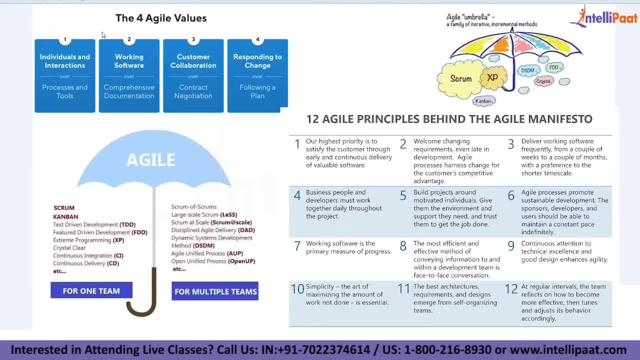 This may be a question that might be raised to the people who are already known about Agile earlier. the basic one I'm saying The answer is very simple: Agile in terms of the implementation of the project, especially for the people who are new to Agile, especially people who are new from traditionally. you are experienced traditional model, you are used. you worked as a developer tester and something of that sort earlier. 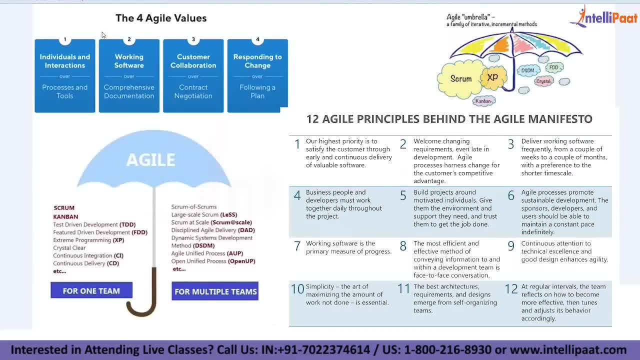 Now team has initiated. now organization has decided to implement a project in Agile environment, So the team is very new right? So, even though you may be, having experienced people, maybe you can count it on fingertips. Either you need to hire people from outside or you have to train your people from other external sources. You have to do either way. 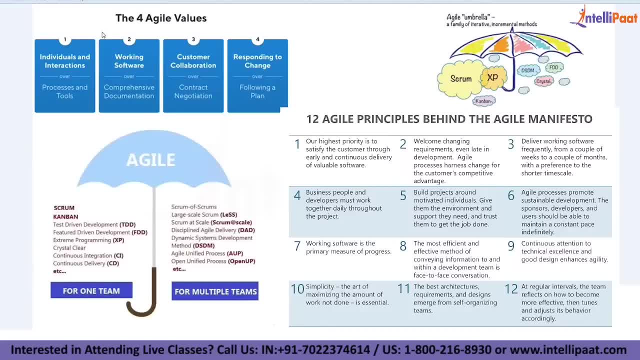 But remaining other people who are working on the Agile and all everything will be normally. those people will be brilliant, Right? So those people doesn't have any experience on that. So for these people, Scrum is a framework which is highly useful to them, rather than XP Kanban. 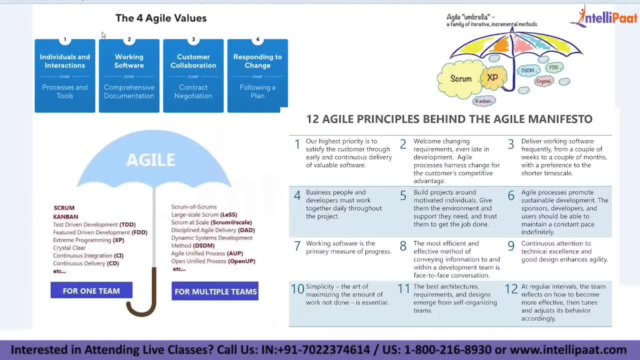 Because XP Kanban, even though it has its own popularity in terms of the complexity, in terms of the addressing system, all that has some difficulties. Difficulty, I don't say it is not technically strong, It has its own difficulties. Something like development approaches will be there. 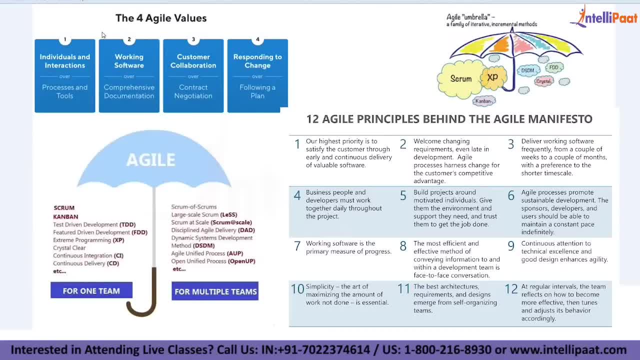 If you take XP, something like extreme programming, all that. So there is an approach called a pair programming, test driven development. So different, different approaches normally be followed At the same time. Kanban is a model, something development friendly, developer friendly, where tasks, boards, everything will be designed. 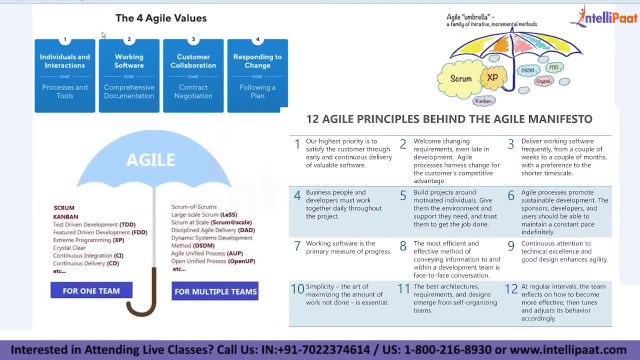 At the same time, whatever the work, everything has to be taken care of by the team itself. So there is no specific wholesale career impact. But whereas in Scrum it is not like that. Because in Scrum, why are we going for Scrum? 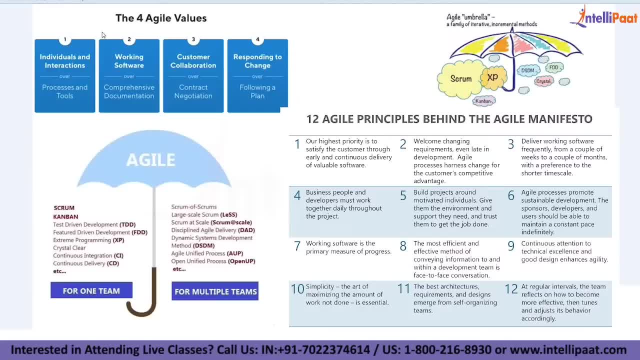 Because Scrum is friendly As well as easy to people to understand as well as enough. That's the reason why more prominence is there for Scrum. At the same time, success rate and as well as the usability is also more for Scrum. 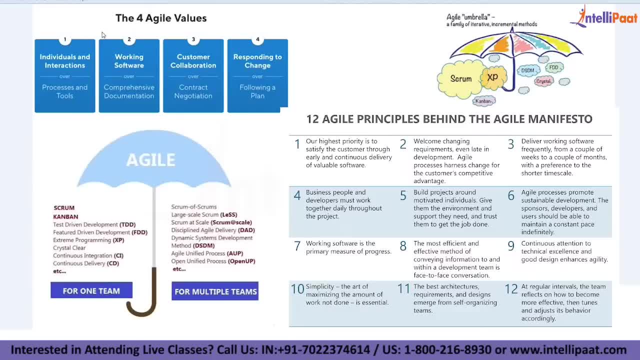 That's the reason why we have more to go to Scrum rather than the many things. So our focus normally will be on Scrum for the throughout training. So this is what one point I'd like to mention Now, especially in reference to the Scrum. 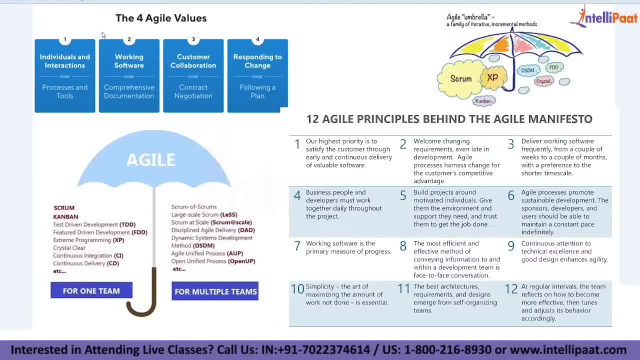 When you talk about Scrum, then, as I told you, if you remember when I explained about the comparison between the traditional and the Agile teams, as I mentioned you, it's a self-organizing team. At the same time, team size will be limited. 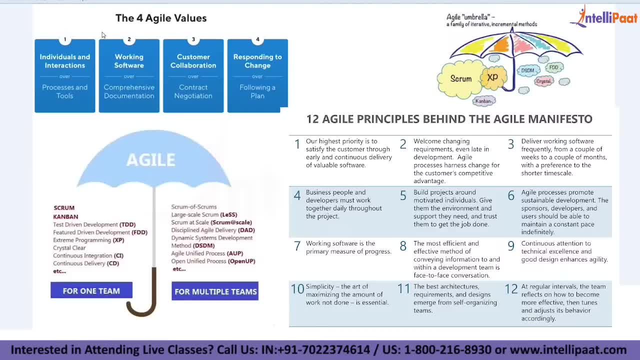 Isn't it? That's what I have told you. That's the reason why, first of all, let us understand what are the different roles to be there in Agile. The first thing, what you need to know, Because we have known about, we have understood about Agile. 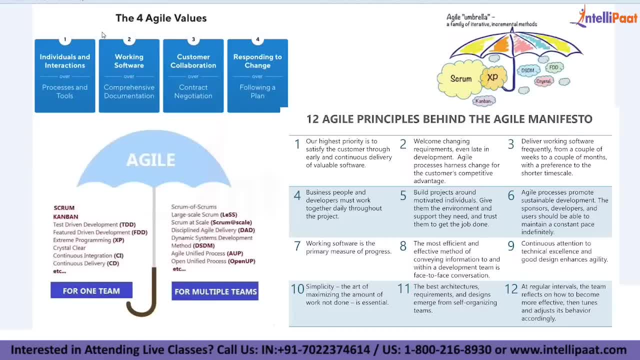 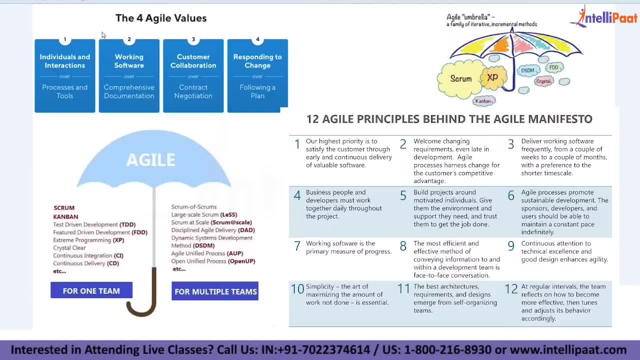 At the same time. what are the values? What are the different, different frameworks and processes up there under Agile we have discussed? Now we need to discuss about Scrum. Why Scrum? For what reason? all that So that also I mentioned you. 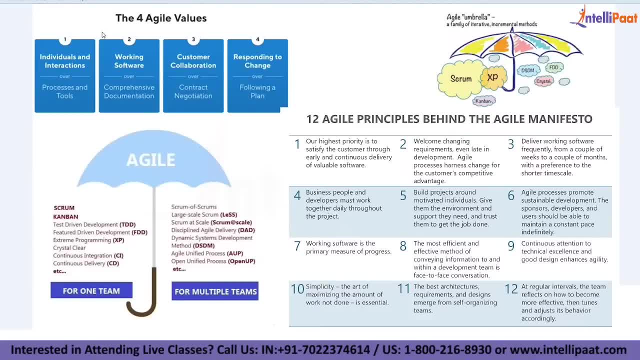 But in reference to the Scrum, there are roles are there, Because if you see traditional model, you can see like project manager, business analyst, architects, developers, testers- all these people will be there, But whereas when it comes to the Agile, it is a different thing. 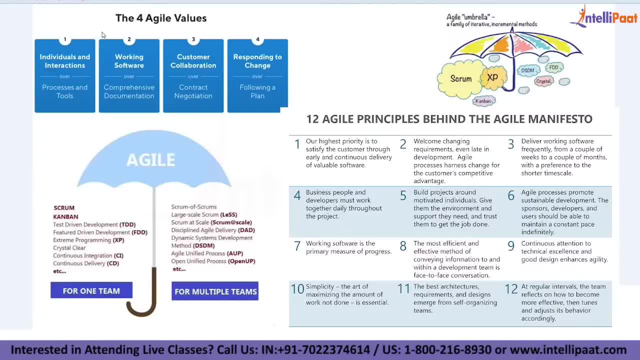 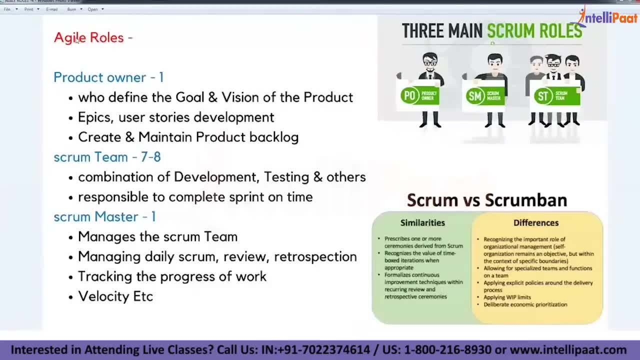 It's, the process will be different, completely different. In Scrum, normally, there are three different roles. Yeah, so this is the diagram. Yeah, so this is it Right. So, especially in Agile, the roles will be three. 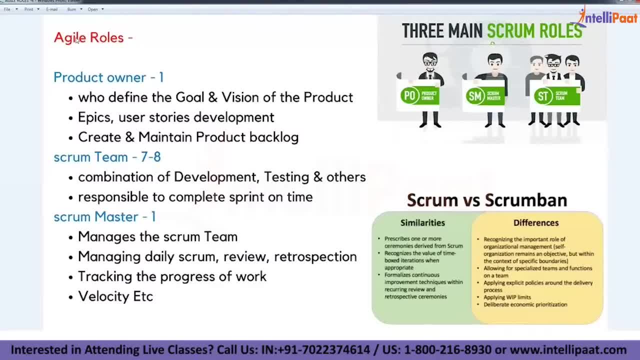 Remember these roles you can see in Scrum, whereas in Kanban, XP and all this kind of thing won't be there Because the complete team, only team, will be there. Team will look after each and everything. So that is one kind of- I don't say- drawback. 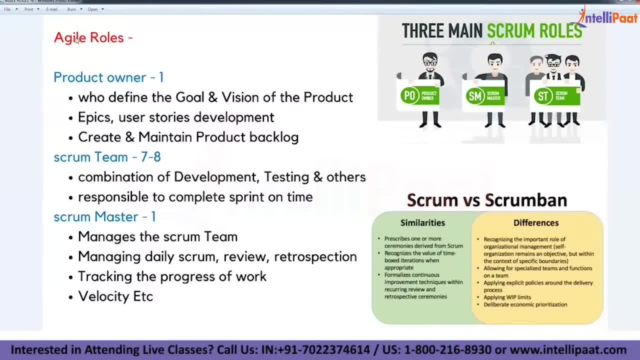 This is that. that is the nature of Scrum. XP will be that sort, Right So and nothing more. But this is something easy for team who are newly to newly transforming to Agile. It is more helpful to them because whatever the roles, whatever the Agile we have and all everything. 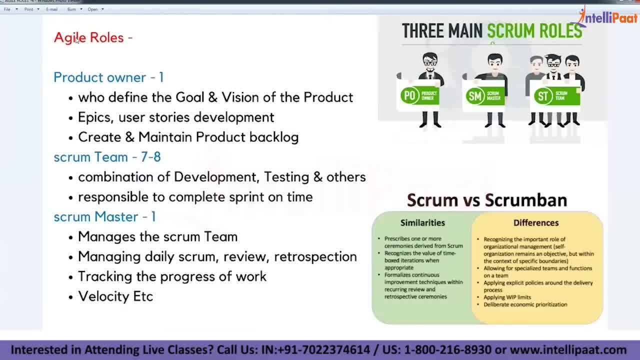 because people were adjusted to the roles right. So earlier designation: because you have a project manager who will be looking after that. There will be an architect who is taking care of the solution, architecture right. So all that we have seen because people who are from the traditional model were experienced with that. 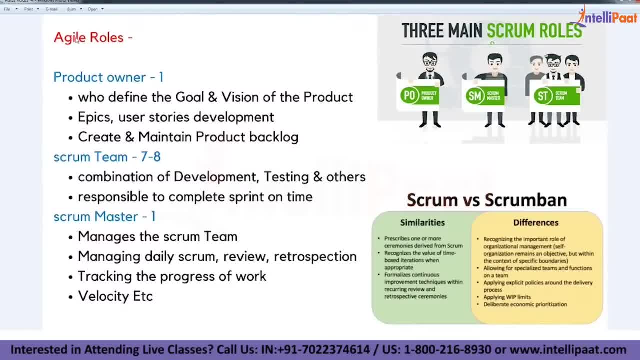 Now, when it comes to the Agile itself is concerned, Agile is all role specific, as I mentioned to you. So this is more connecting. It is because people can transform themselves easily here, So that's the reason why people will be more about Agile roles here. 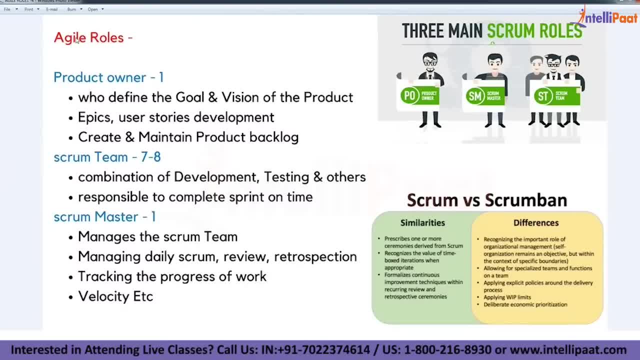 Normally in Agile. in reference to the Scrum itself is concerned, it is all role specific, where roles will be divided for three different things. The first role- we call it as product owner. You can see here on the screen. Second will be called a Scrum team. 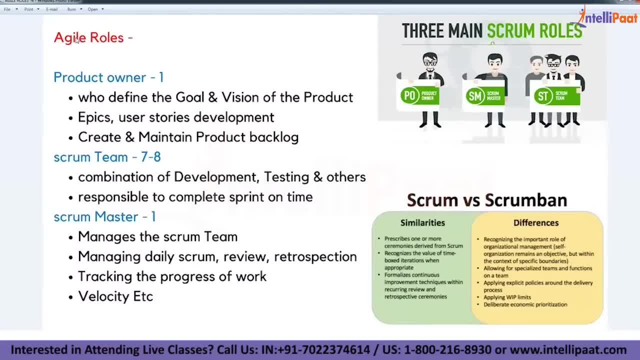 Second will be called a Scrum team, Followed by Scrum master. You can see three different roles in Agile. One is product owner. Second, Scrum team, Followed by Scrum master. Three different roles. Now what a product owner and who is product owner is right. 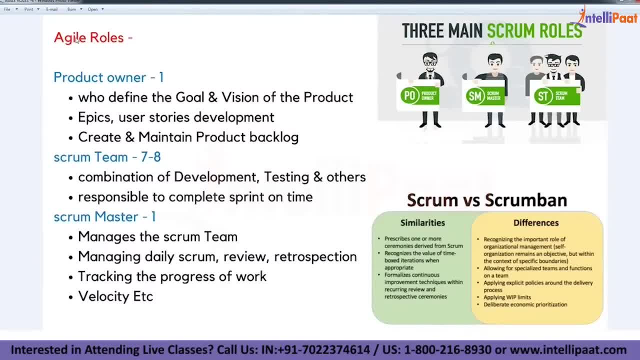 So this is the first and foremost question we need to understand. Product owner usually is a role will be played by an individual who maximum focuses on the. what the customer expects Means in what way we have to provide value added services to the customer. Is what generally the perception for any product owner? 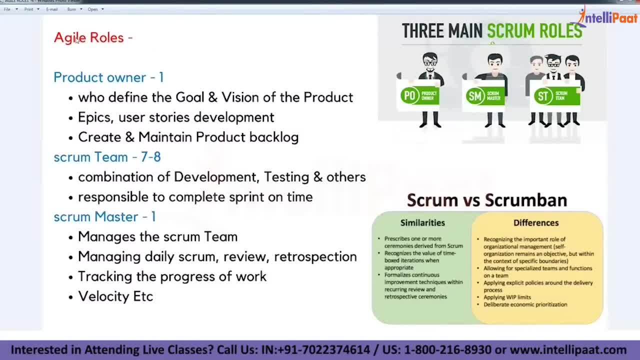 Product owner never thinks from the team perspective. There is a clear difference between the role of a product owner and a Scrum master in a high level. note: Product owner always thinks from the customer perspective, Scrum master always thinks from the team perspective. but he must make sure what is that product owner want he has to meet. finally, 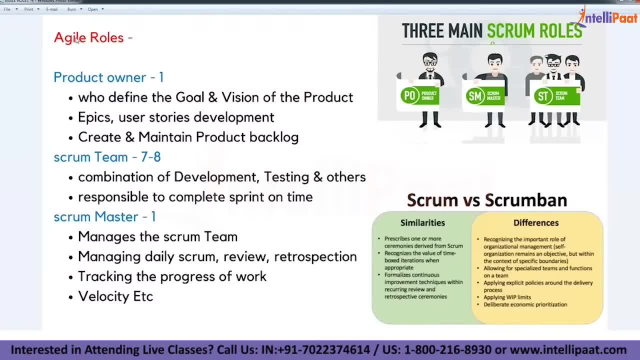 But at the same time he has to take care of the welfare of the team also Scrum master. So that is the fundamental difference. Apart from the remaining aspects, the fundamental difference is that normally product owner is the person. yesterday also we have discussed the same point. 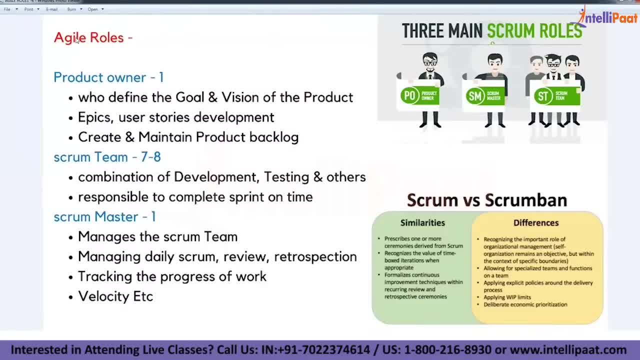 Let me repeat the same: product owner, nothing but client representative. first point, this will be. this role will be recruited by the customer. usually, if you are developing a project so far, for example, from XYZ organization, we are developing an application- product owner will be their person, their individual. 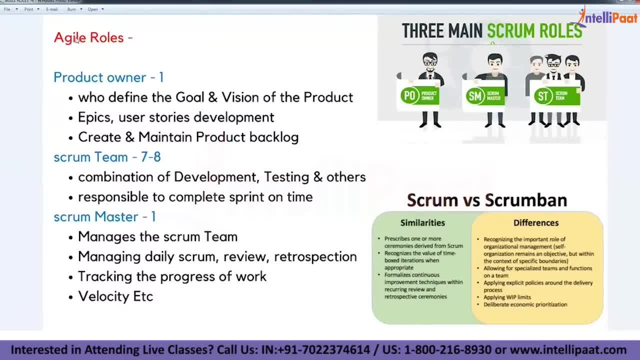 Whoever they are sending, it is a material to us, but product owner will be there. The fundamental thing is that product owner is a product owner. Your, she is a product owner. They must be having a clear understanding about that. What is they want? 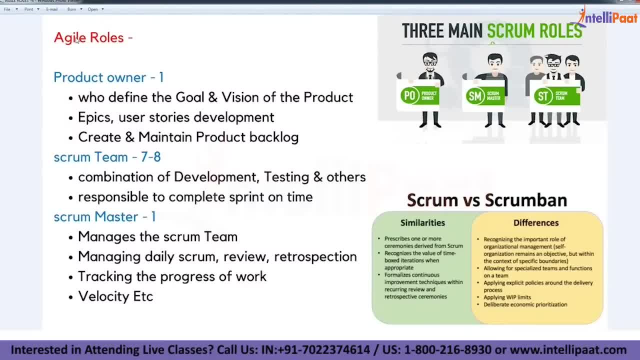 What they want should have a clarity for them for sure. First, whatsoever reason, They should have a clarity. If they are missing in clarity, then gone, Everything will be, Everything will go away. So a product owner should have a clear understanding about what is. 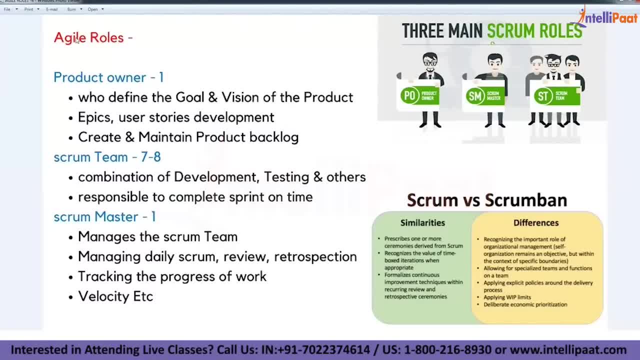 that they want, what is that they are expecting from the people, so that clarity should be there for a product owner. that's the reason why most of these people and all everything comes from the customer side. point number one: if not, if nobody is sending, so we have to recruit a product now. 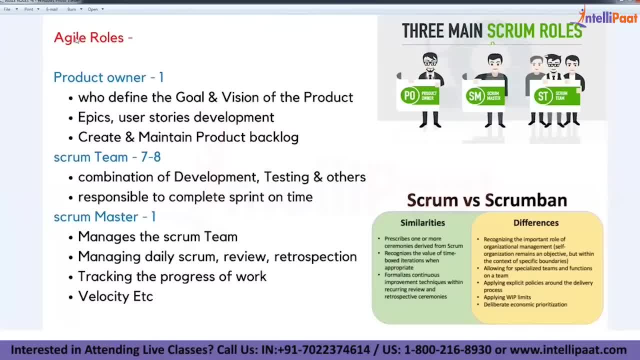 here is here we need to understand one more point: there is a role called b in in traditional way of approaches. you can see so, the role of business analyst. you can see so, business analyst is the person who will be taking care of by the business requirements all that normally earlier used to. 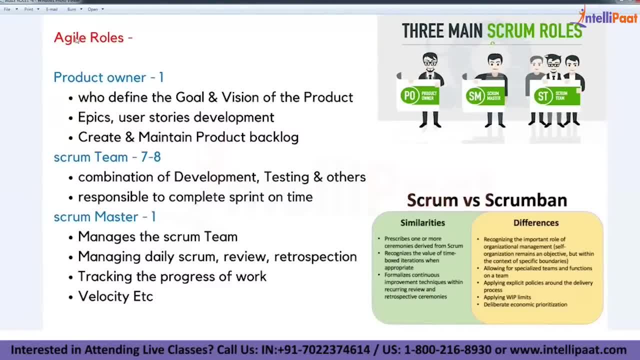 have in the traditional in the beginning days- when i started, of course, in the in the year of 2001, sometime even i could see i remember- usually we used to have two different roles in application development. when we works on project, we used to have two type of analyst. earlier now it was. 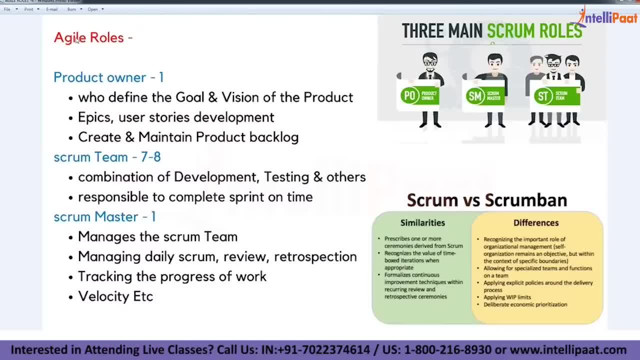 changed. anyway, the transformation has been taken place. earlier we used to have two different roles, so one is business analyst, second is system service used to have two different roles. business analyst means completely focusing on the business perspective, business requirements, all that systems are list. completely focusing on the technicality means, if you want to develop- for example, there was a point of sale- 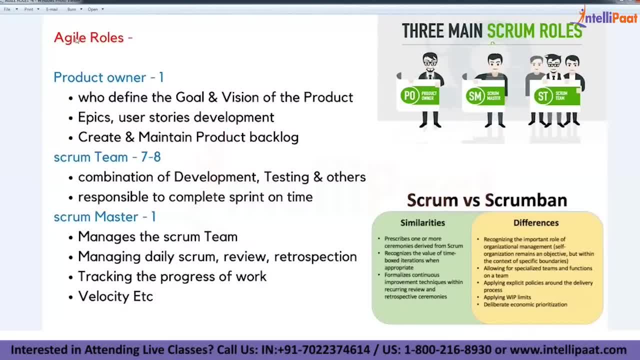 system. what is point of sale system? point of sale system is a billing system. so billing system we are using normally in retail store whenever we buy the products against to the billing, all that stuff, whatever the billing happens. that is what we call it as pox point of sales system. 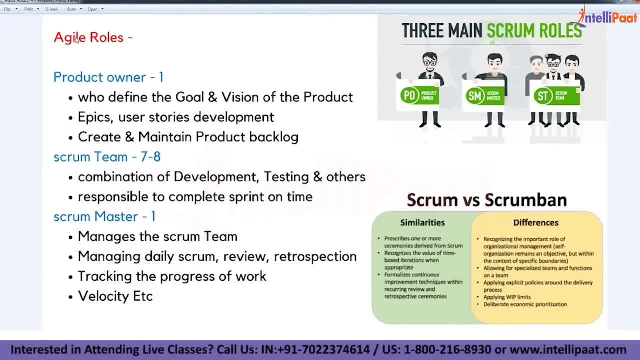 now a customer wants to develop a point of sale system because assume that there is an existing pos. customer has some difficulties in using this pos system because the application was very old. they were using for very long time. the present situation: the volume of business has increased, lot of features were involved, a lot of services of the business. services have increased so that 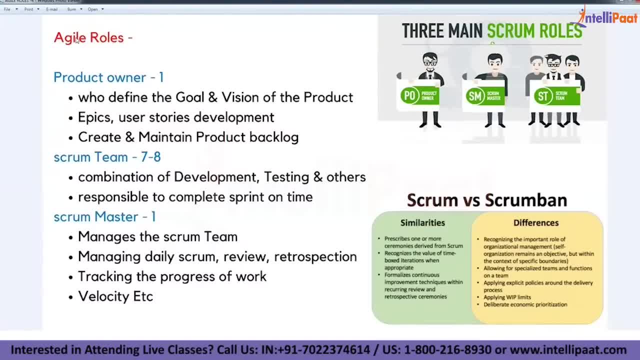 existing application is not performing well so they want to have some solution to be taken into a contract. so they want someone has to provide solution for them. usually it's: all these activities will be done by the b, whatever the business related thing, functionally related, whatever the solution they were understanding. so by understanding the existing 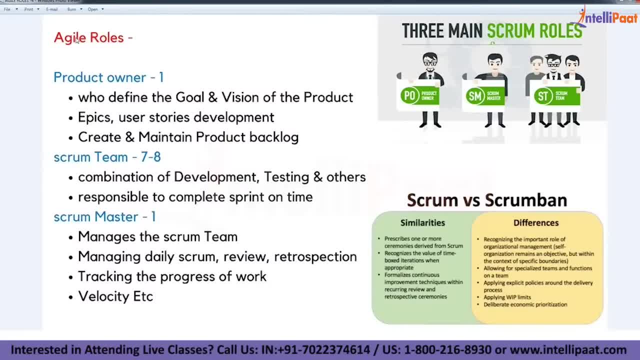 process, followed by proposed future. all that by keeping all these in mind. business analyst will give you the business solution now technical solution. technical solution means how you are transforming from business to technology, is what we call it as technical solutions: transfer understood right. business solution is different technical solution. 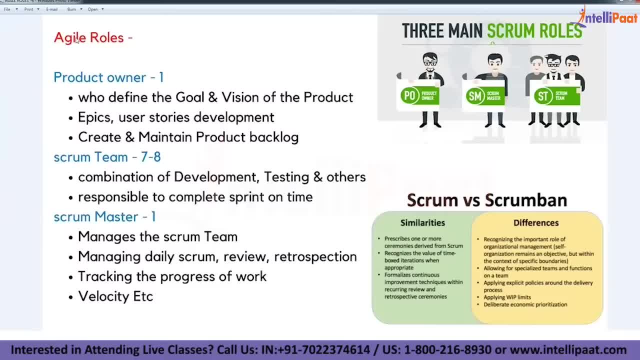 Let me explain you that first, so that you will be having a clear understanding. What is business solution, What is a technical solution? Let's say there is a POS application. let's say there is a POS application customer is using for very long time. 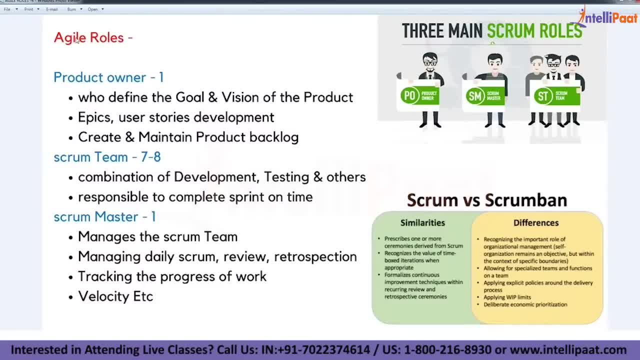 Now due to the configuration is very low because assume that they are using since last 10 years. the configuration was very less at that percentage of time because that time the volume of the customers were also very limited to them. Now the customer base has increased. the amount of time for building should be very faster. 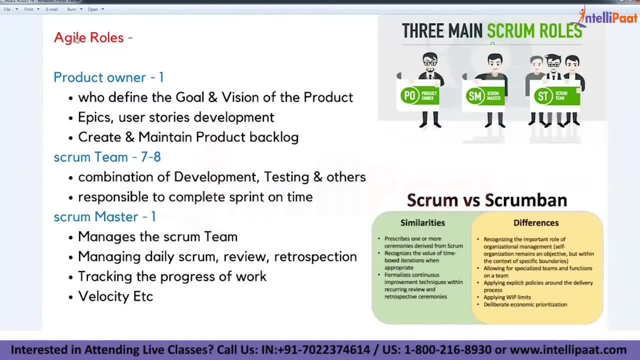 but it is not happening due to the configuration issue, because the configuration is very slow, because old configuration. Second, they want to generate reports online. they want to see because they have multiple stores in different locations. they want to see everything online, but they couldn't do it. 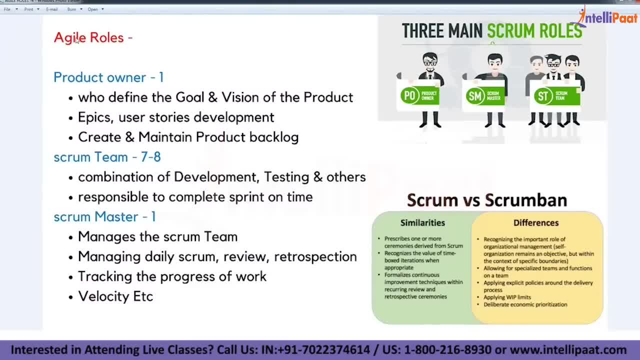 That is second point. Third, if there is any problem in terms of the technicality, because, end of the day, point of sale system is an application and a server system, right, so it's a hardware device. If there is any problem, someone has to come and troubleshoot it, repair it till the time. 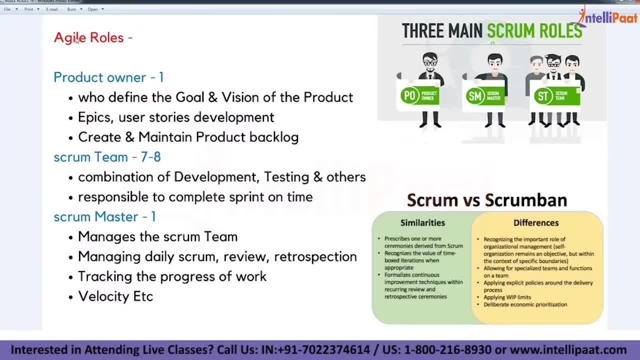 that system will get halted for some time, right, so pressure will be more in other roles. This is how generally, the practically, the customer is facing the problem Now. customer wants a solution to be provided first. So for this, please address right. so these are three problems. one is configuration is 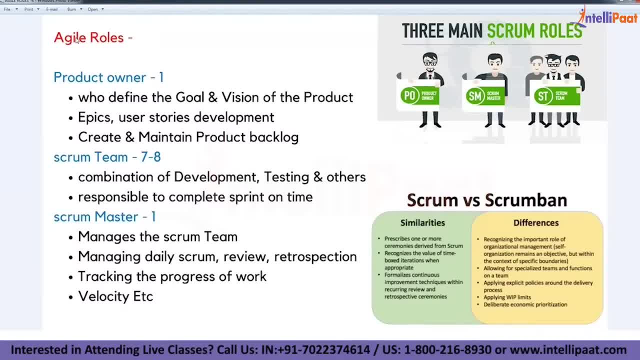 very slow. you want someone has to upgrade the configuration is the one thing. Second, they want to generate reports online. this is the second problem. Third problem is that if there is any kind of repair comes across, someone has to troubleshoot for that. it is taking lot of time. 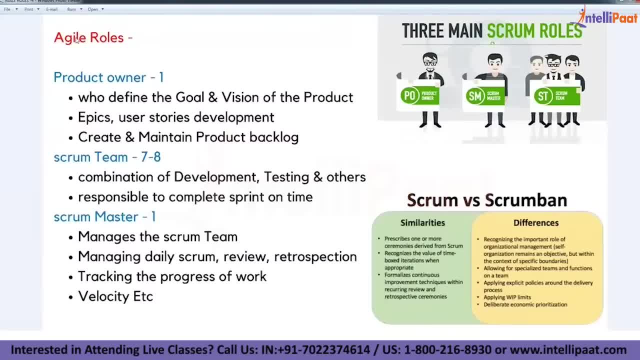 So more pressure will be on the other other roles. So this is the problem they are facing Now. a business analyst- what a BA do? a business analyst is the person. try to understand this. assume that developing a cloud based POI system is what the solution. 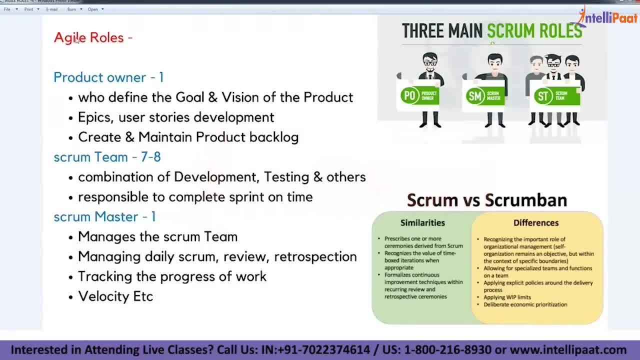 A business analyst has been identified. what is cloud based application? cloud based application means whatever the POS application we have will be developed on the cloud environment, something like either by using, like Windows Azure or something. there are different, different cloud service providers nowadays. we got So they identified a cloud service provider and they want to develop an application on. 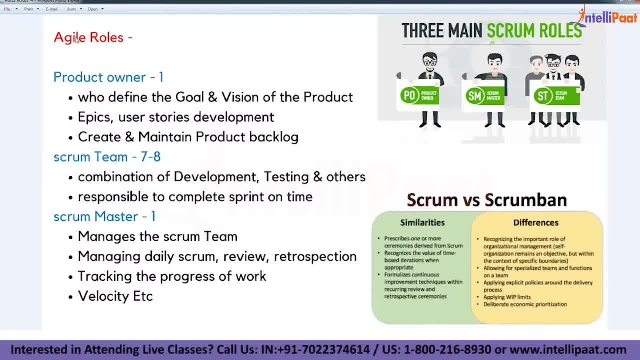 cloud because of the cloud system. the advantage is that they don't require any kind of infrastructure. even a small retailer or a mid-level retailers can use it. What is that they require is a laptop or a desktop with a proper internet connection, So they have to make sure that they need to have a proper, decent, fast internet connection. 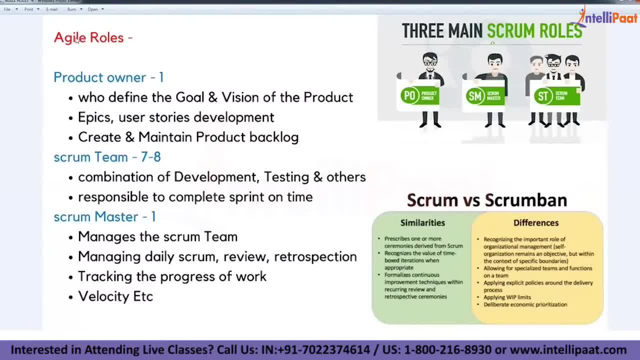 is required, so that they don't require to maintain any data, nothing. everything will be uploaded on cloud, whatever the reports, everything will be uploaded in the cloud itself will be generated, because there are there are templates available there. If you give the figures, numbers, and all, automatically reports will be generated. is we assume that? 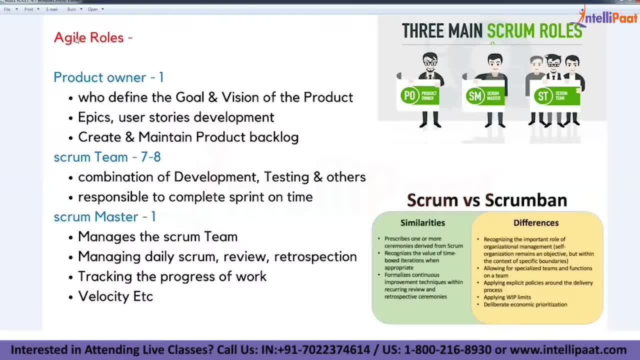 if it's a business Owner wants to see all that, so they can see anywhere online. at the same time, there is nothing for repairing anything. so there is no repair. nothing because it's a cloud application management will be taken care of by them and that it's cost effective. it not be much cost. 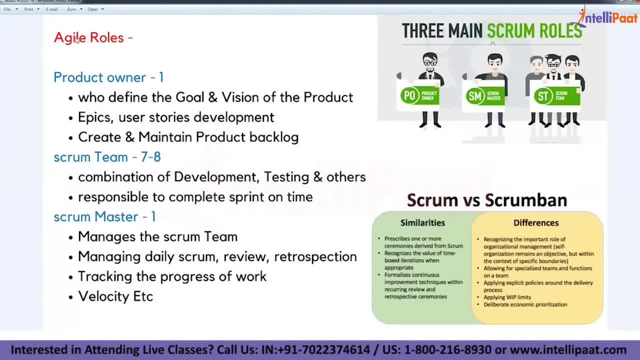 for you. So what are the services customer is using for that they have to pay- pay per use kind of stuff. Now, the developing cloud based point of sale system. whatever business analyst identified is what we call it as business solution. Okay, Now to develop that. how to develop this? what technology is required? so, configuration related. 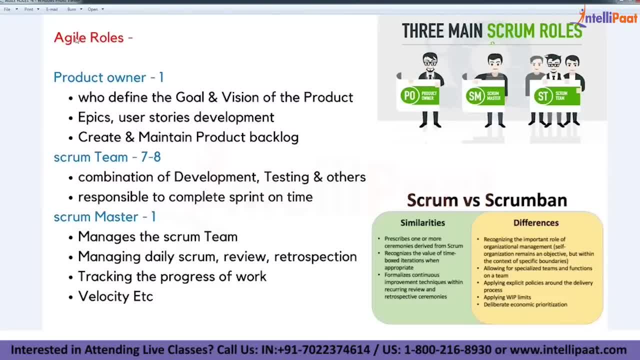 things. even though it's a cloud, we need to identify right. So these things normally takes care of the systems and I'm just giving an example. This is how earlier was, in the beginning, this, but now the slowly the transformation has taken place nowadays. Now we were, we were calling this, as nowadays you can see in job profiles, we can call it. 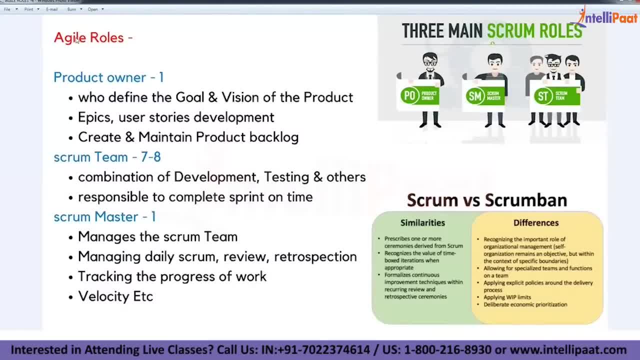 as business systems and list. This is how the transformation has been taken place. in most of the profiles I'm saying somewhere other way you can see a business analyst also, but normally because the point is that earlier you don't require any technology because technical expertise and all everything was not much. 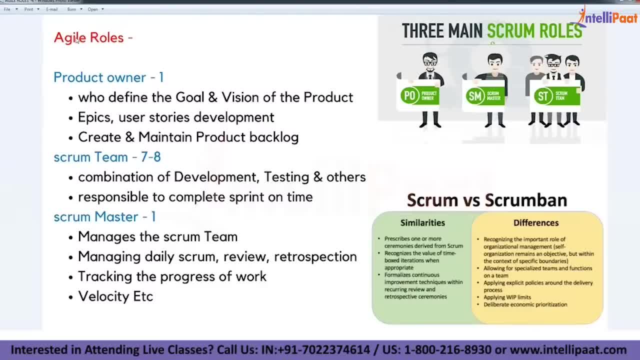 required because when we started our careers in the year of 2001-2003, you don't require much technology required because there are technical people who will be looking after all that. But now the situation was not that. So you must be. I don't say that you must be expertise in coding, development, all that, but the situation. 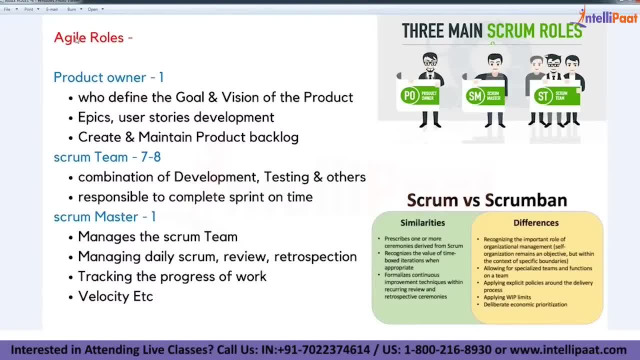 has changed in such a way, person who is working as a business analyst should have a knowledge about the technology, knowing about the technology, transformation of the technology, how it is changing. so that sort of understanding is required. So that is how generally the transformation. So this is what generally the role of a BA, in short, right. 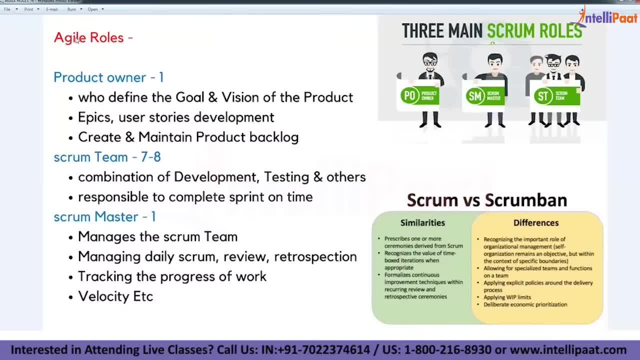 This is what we now. most of the people will have a confusion here, Raj. if I am a business analyst, I have worked for about 5 years or 10 years in application development, wherein I am experienced in traditional model but now in agile. what is that my role will be right? 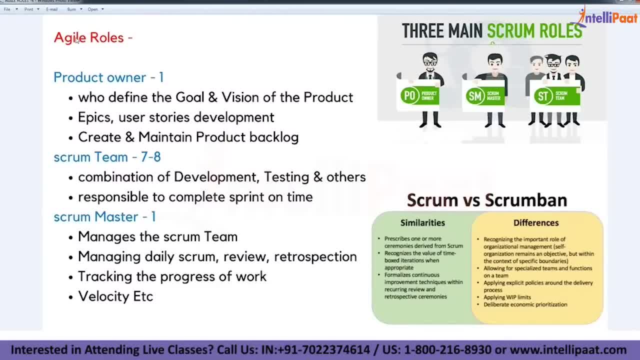 So what role will I be playing? fundamentally one thing: if you talk about agile environment or agile, you don't see any role as project manager or a BA. no role as BA, project manager- nothing. So whoever is working under agile environment must be there, especially in reference to scrum. 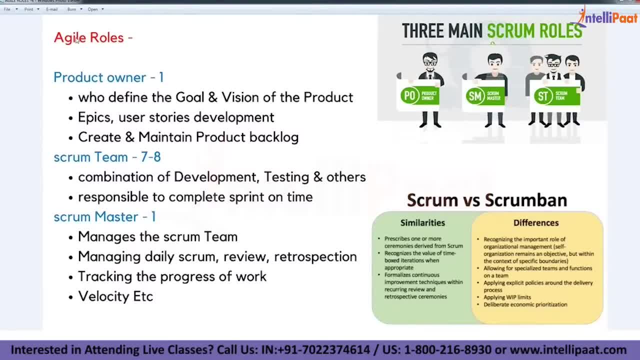 again, You will be under these 3 rules. either you will be a product owner, you will be a scrum team, or else you will be under a scrum master. Most of the times. most of the times if you are a business analyst- most of the times. chances: 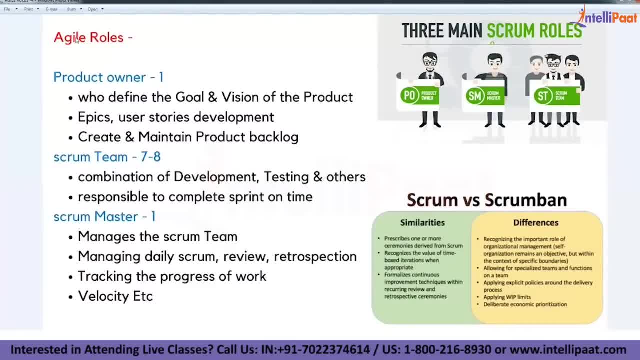 will be that you will be acted as a product owner. why? because if you see the responsibilities of a product owner comparing to BA, it is all more of similarity. right, You can see the similarity between those 2 things. that's the reason. who are working under? 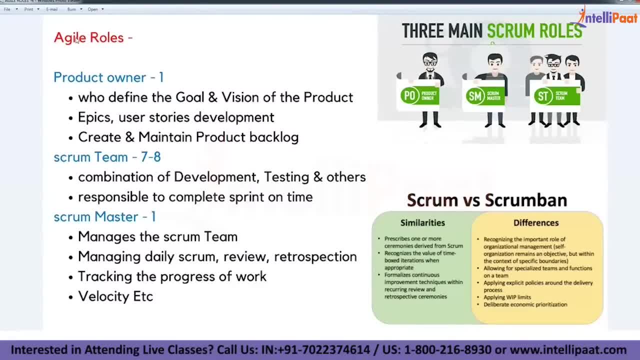 agile environment. If you are a business analyst, chances are more that they become product owner. why? because product owner is a client representative. business analyst is also a client representative, hence product owner is a role. but nowadays even we also see practically: they were, they are taking. they are taking even business analyst also because business analyst project managers. 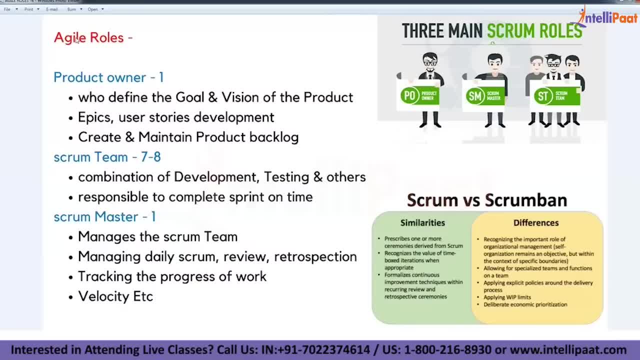 also, people were taking for different different reasons, because they require some additional manpower support. that is the reason they are taking. But if you are a BA, when you transform your kid to agile, normally you will become a product owner because the roles and responsibilities for something similar, hence product owner. 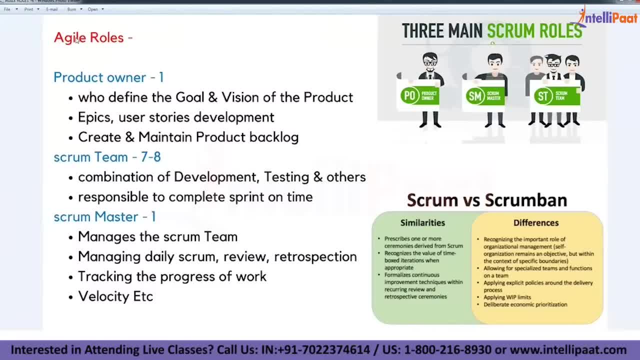 is the role. So this is one thing I must tell you, because I could see some persons who are relating to BA, the reason why this is helpful to them. I hope right. So this is point number 1.. Next, what product owner do, right? 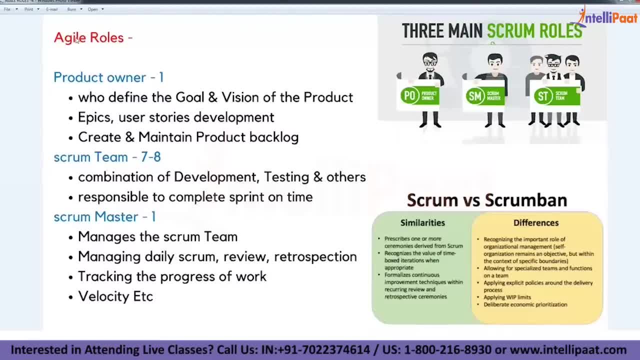 So, as I stated and earlier mentioned, you product owner is the person who will be focusing more on about What product customer wants and what customer requires. this is what generally the product owner mentality will be. So always things from the customer perspective right: what product, what customer wants, what? 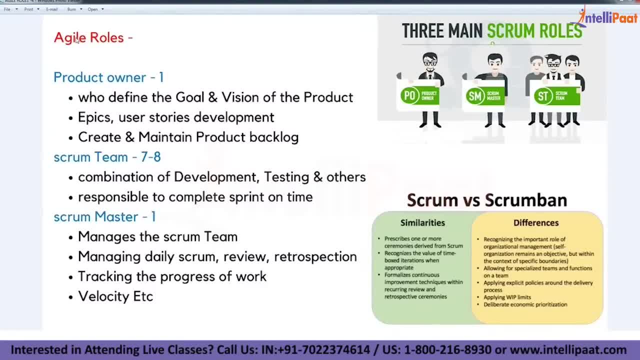 customer demands. this is what generally So a product owner is the person who has to define the goal and vision of the product, which is the first responsibility. What is goal and vision? Goal and vision means what, finally, we want to achieve. Let us take our point of sense, let us assume that. let us, because I have taken example of 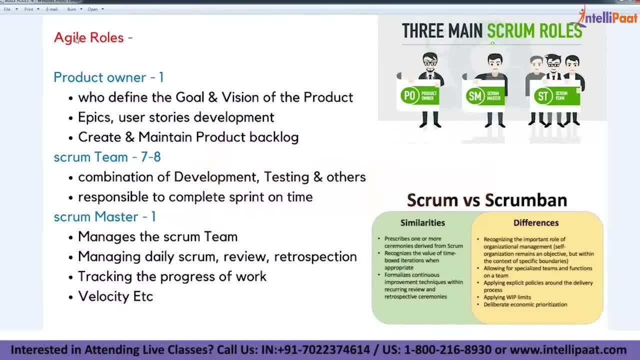 POS, right. Let me take the same example here. we want to develop a point of sales system- right. this is what the customer required. either it could be a cloud base or a traditional, whatever it is, but they want a point of sales system to be developed. 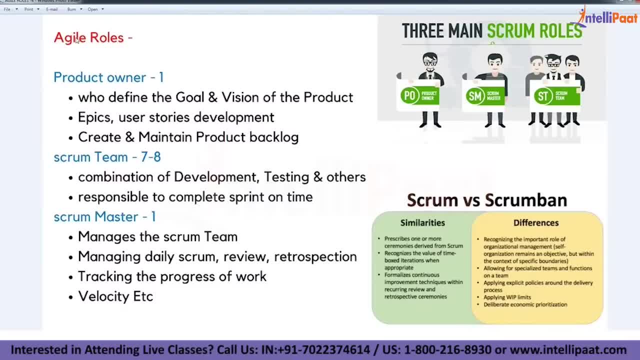 So what should be the reason? see, developing a POS system is not an individual entity in the organization, because it is a part of the business. you take a retail store point of sales system is a part of the retail store operations, directly or indirectly. this POS system is supporting the business, right. 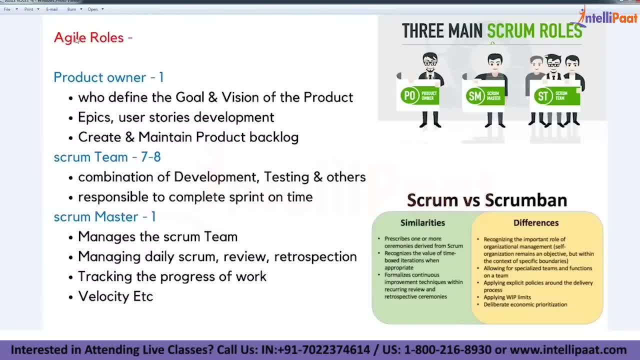 So if someone is investing money to you to develop a point of sale system for their billing, all that, there must be some goal and vision. without having in goal and vision, nobody is investing money right. So a business owner is investing money. for what reason? for example, I am a business owner. 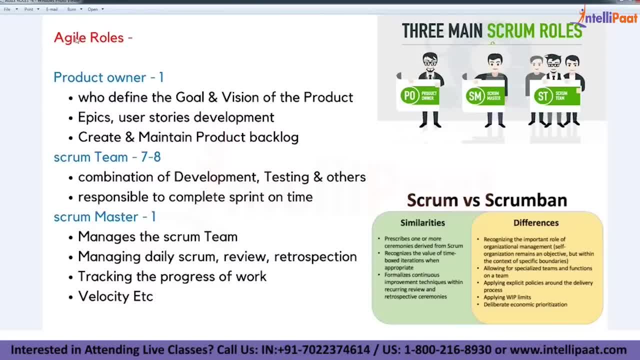 I am coming to you guys and I am asking you to develop a point of sale system. I am ready to spend some amount of time on that, So I want to pay you this much of money. so why am I paying? because, directly or indirectly, this POS application is benefiting my business. in what way it is benefiting, it can be benefiting. 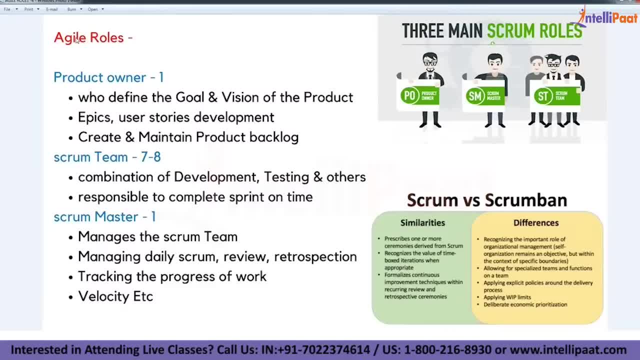 it could be benefiting for two different reasons. either it will be a part of enhancing my organizational performance. because of this, my organizational performance will be increased. this is one reason. it could be one reason. Or it will increase My revenue cycle- anyone right. so, whatever the solution we provide for any customer across, 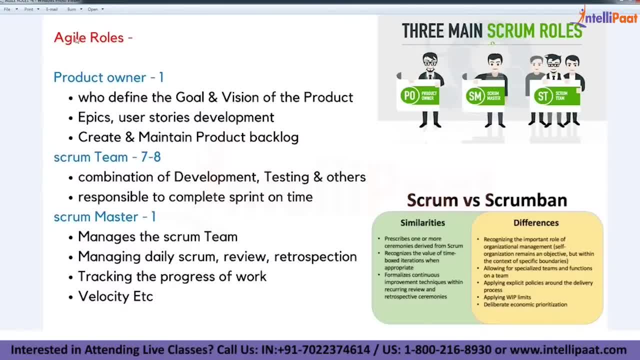 the world. you see any technical application you take. these are the only two things. one is enhancing the organizational performance, at the same time increasing the revenue cycle. you can see any organization, any solution, any application we develop, end of the day it lands there either. it is helpful to enhance the organizational structure and performance. 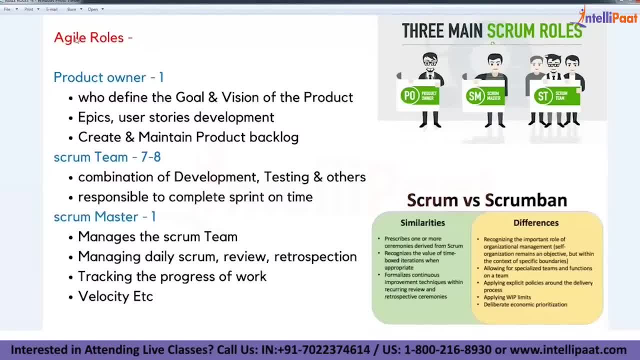 of the present this thing, Or else It will be helpful to increase the revenue of renew life cycle, either directly or indirectly to the client. So if you are a product owner, assume that if you are a product owner, the very first thing you need to know is that you need to define the goal and vision of the product. 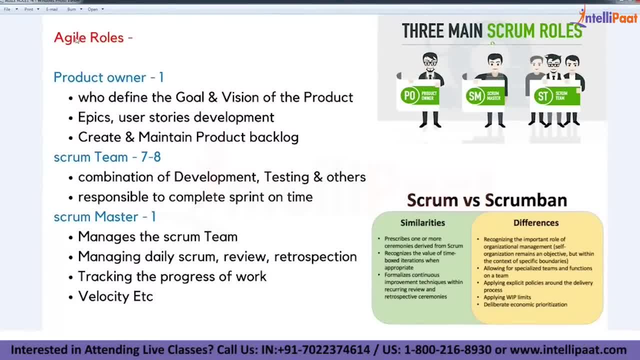 the first thing, what must be the goal I want to reach, followed by vision. normally, this goal is of two different types: business goal, project goal- two different things. being a product owner, The focus must be a business goal, not the project goal, because you are nothing to do. 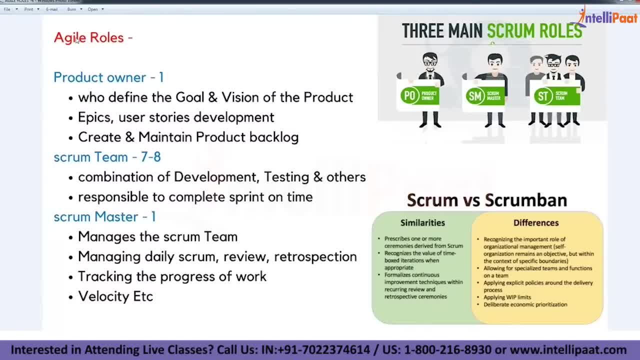 with project implementation. all that because you are a business owner or you are a product owner. you have a business goal. this is what I want to achieve, or this is what I want to reach in coming years, or in coming months, or in coming days or in coming hours. this 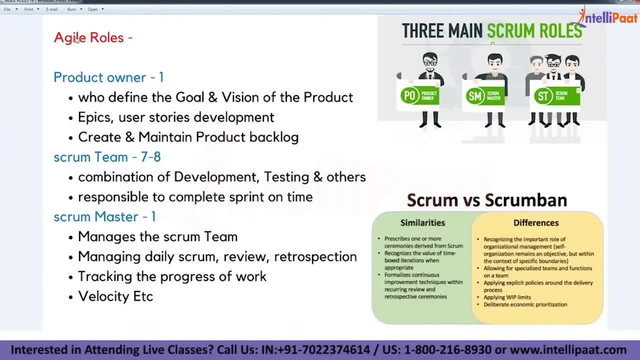 is what your business goal is. at the same time, vision right. so, based upon the business objectives goal, you will be having a vision, because every organization is depending on three things. Any organization you take, inception of the organization will be depending on three different things. because you take any organization, goodwill of the organization will also be elevated. 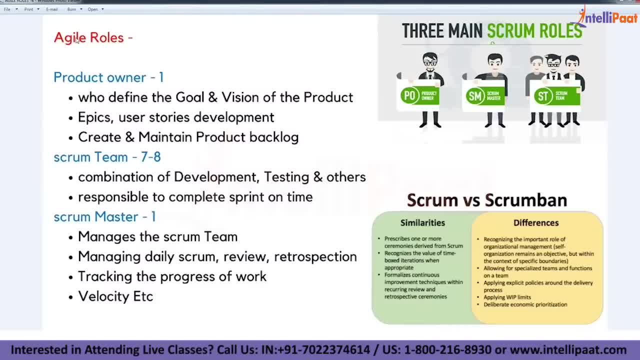 on three things they have to be withstanding. on these three. one is objectives and goals. point number one. second, vision, followed by the mission. right, mission means how they are performing. vision what they want to become. business objectives and goals means what they want to do. so every organization, whatever the decisions they take, business decisions. 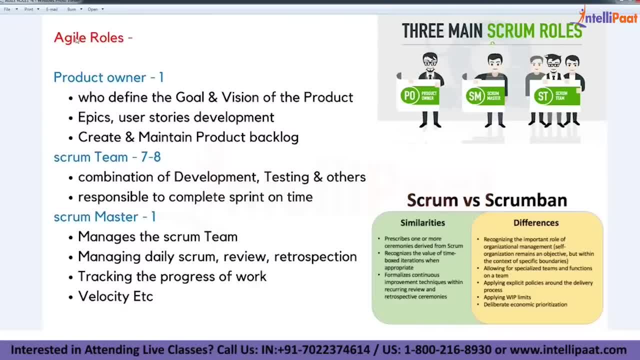 everything must be within this, this thing, then only the company has a goodwill, because maybe sometimes organizations may lose financially sometimes, but end of the day, goodwill not. we cannot count goodwill in each and every time relating to monetary right, financially of course, financials required for a new organization, for sure. I think there is undisputed fact. 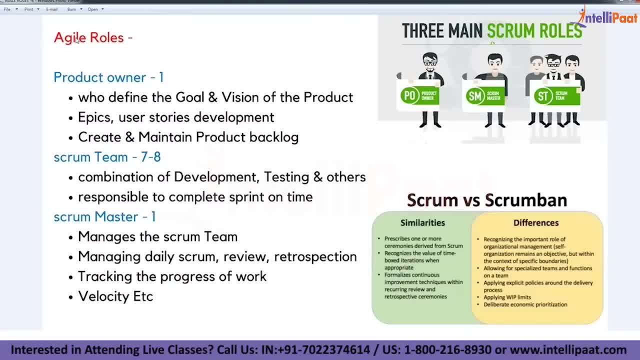 disputed fact. but if you are talking about the goodwill of the organization, it's completely depends upon the kind of activities they are performing and what kind of services they are providing. end of the day, right? so, without deviating their vision, which are deviating their business goals and objectives, followed by mission, right? so there are some policies. 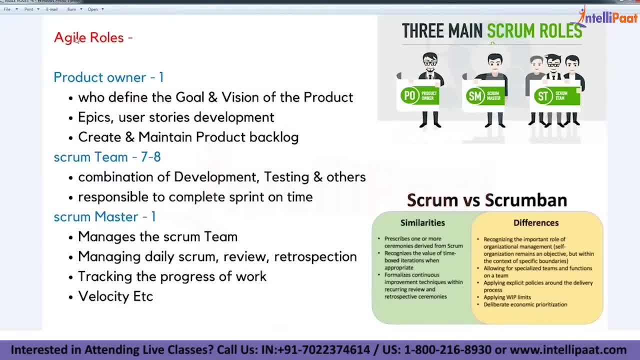 principles, all that which you have to be bad with. so that should be the structure right. so if you are a product owner, first of all you need to understand, you need to define the goal and vision of the product. so what is that, finally, we want to achieve? if someone 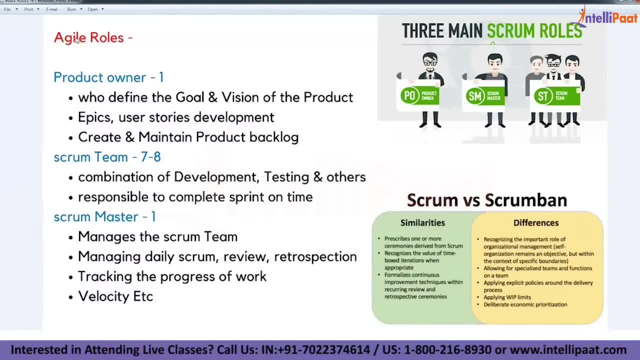 is developing a product to us. this is what the first point, so that clarity should be there. the clarity should not miss for miss, i mean, it should not miss for whatsoever. reason point number one now: once the goal and vision is done, the product owner is the person who has to create epics, followed by user. 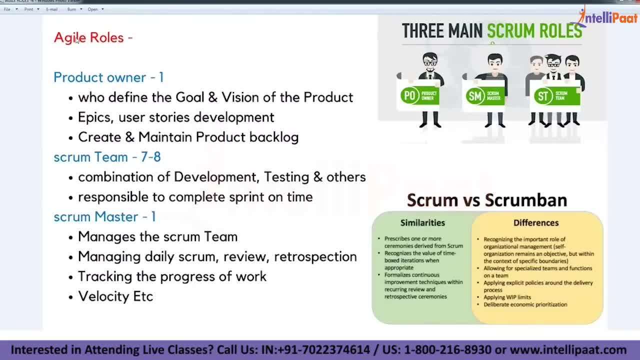 stories all that. normally, let's say, a point of sale system is what a customer is requirement. customer requirement means po. requirement is that they want someone to develop a point of sale system. developing a point of sale system. there is a hidden goal, right? so there is a. 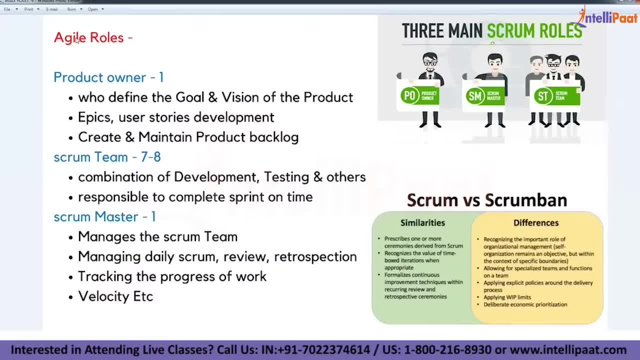 business goal and vision which was already clear for customer. they have because they conducted meeting right, so they have before because, see, you are a, for example, you are a business owner. you are giving in a project to some client, so you are identifying some vendor to develop solution for your project problem. what is that you do being a business owner? your team will. 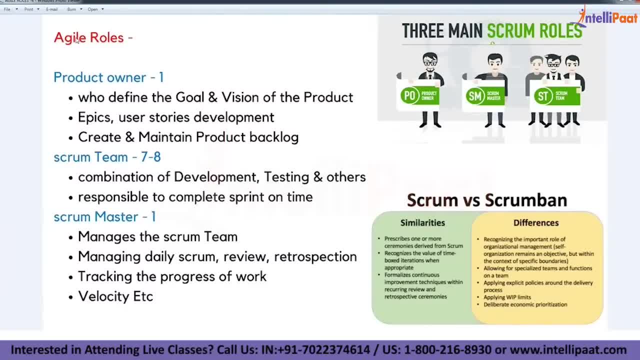 decide that you are a business owner. you are a business owner, you are a business owner. first to discuss: right so what are our problems? right so what kind of solution are we expecting? so, situation of the business, everything. so, first of all, you need to have a clarity. 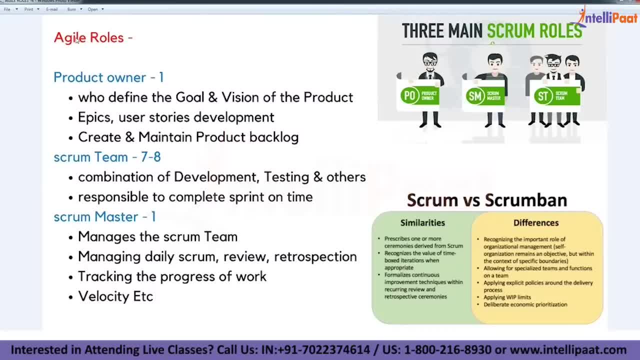 otherwise you don't come, you don't go for blindly. we don't go directly to the vendor and ask to develop a solution, right. so we need to have some clarity, because when you go to the vendor, client vendor will ask you: boss, what is that you want, right? so what is that you are expecting from? 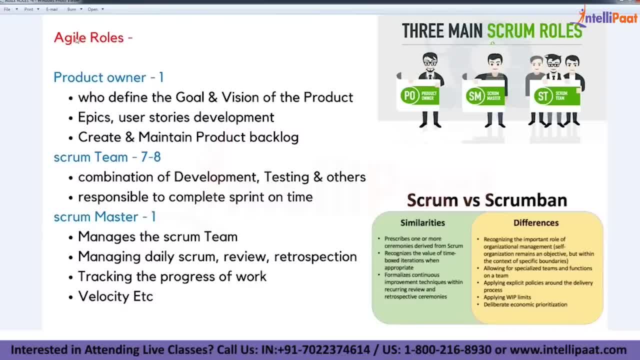 me at least to that, at least for that extent, we need to have a clarity right. so we need to have a clarity right so we need to have a clarity right, so we need to know about this. so goal and vision is required. point number one: developing a. 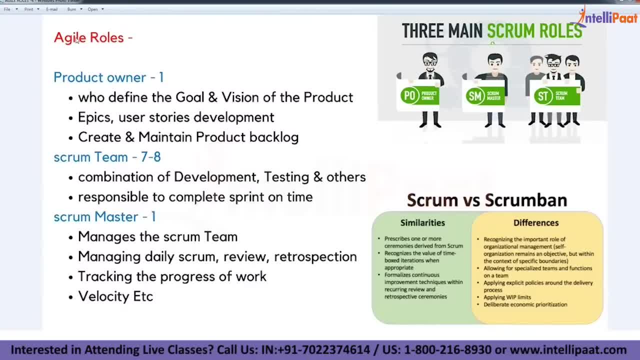 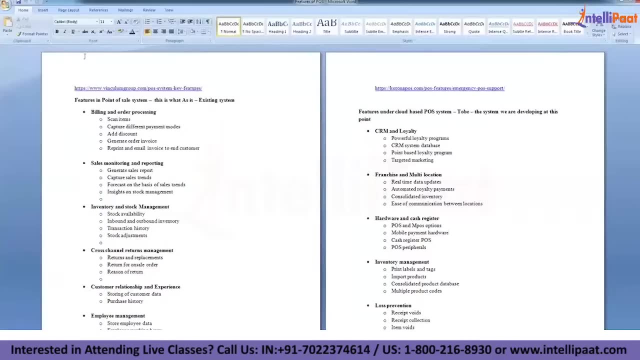 pof system is what the thing they have decided? assume that now, if you want to develop a point of sale system, point of sale system must be having some features and functionalities, isn't it? what are the features? for example, these are the features. let me explain you it. for example. these are the 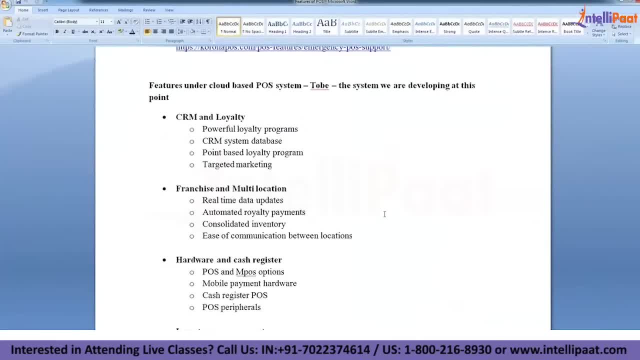 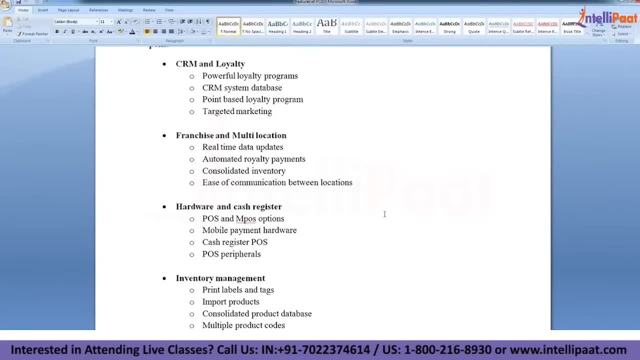 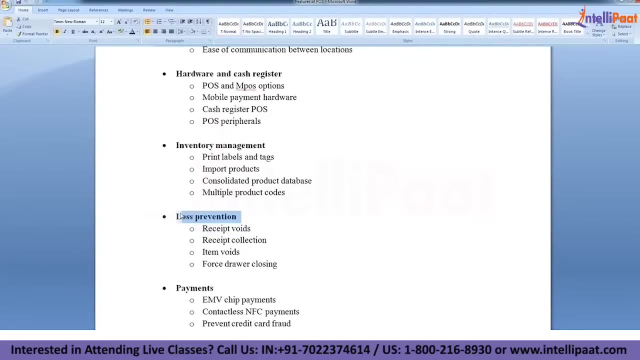 features. let's say it's a cloud-based application- right, cloud-based system. these are the features: crm and loyalty right, franchising and multi-location hardware and cash registers, inventory management system. so these we call it as features. right, large scale of solution is what we call it as epic. okay. 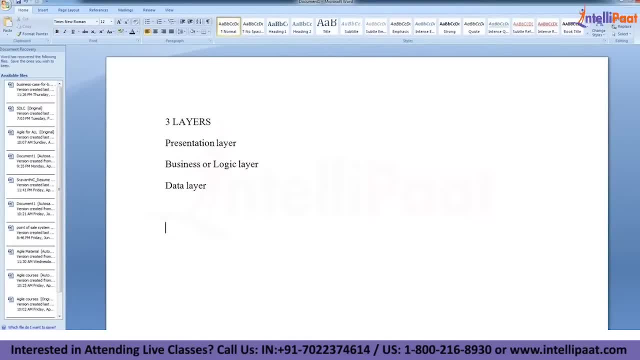 epic, nothing but normally we call it as feature, but in agile we call it as epic. epic, nothing but large scale of solution. large scale of solution is what we call it as epic stands. epic means this: epic, nothing but feature. you can understand that in simple terms: epic, nothing but feature. large scale of solution is what we call this: epic. 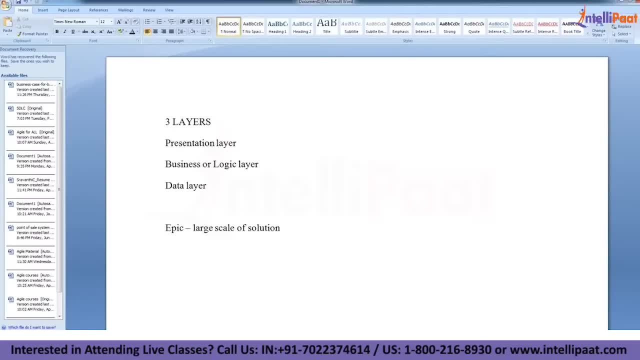 right. this is first thing. now, if you want to develop a feature, what is that you require? you need to have some features and functionalities means you need to develop some functional and non-functional requirements. if you talk, if you speak about, epic is nothing but a feature for. 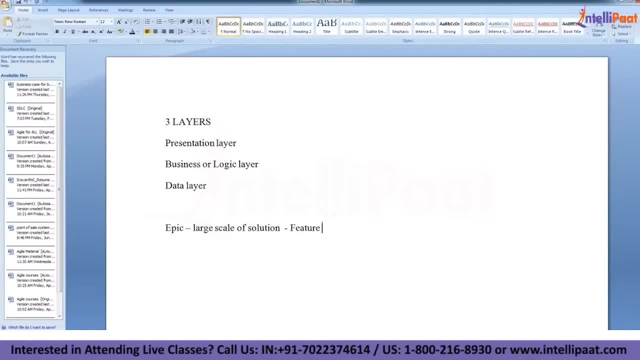 example. right, if you talk about this as a feature. every feature should be having some functional and non-functional requirements- functional and non-functional requirements, because these functional and non-functional requirements must be developed. then only the feature will be useful. otherwise there is no point of using the feature. I'll give you a simple example, which is relating to: 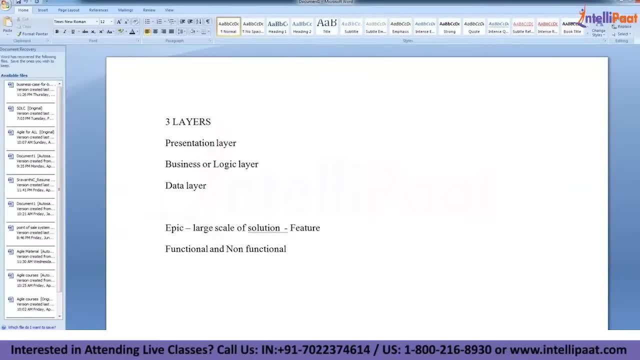 so that you guys will understand much better. now you have bought a car, you are driving a car where you have used this car to drive to the locations wherever you want to go, right, so this is for that reason you have bought a car. now, bye, there was a device called GPRS tracking device which was given by the customer manufacturer. 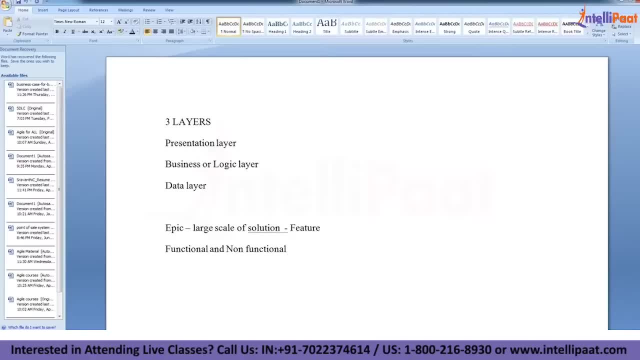 to you For what reason GPRS tracking device is being used for. GPRS tracking device is a device which is used to show you the directions because there will be some locations which are not known to you. If you want to reach the locations and all there must be someone. 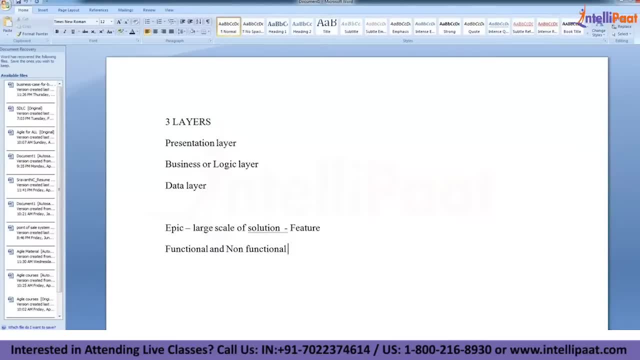 to guide. Who is going to guide you this? This is being guided by GPRS tracking device. Assume that GPRS tracking device is a feature Among different features involved. this is one kind of feature which is there in the car. Car is nothing but project Understandable. 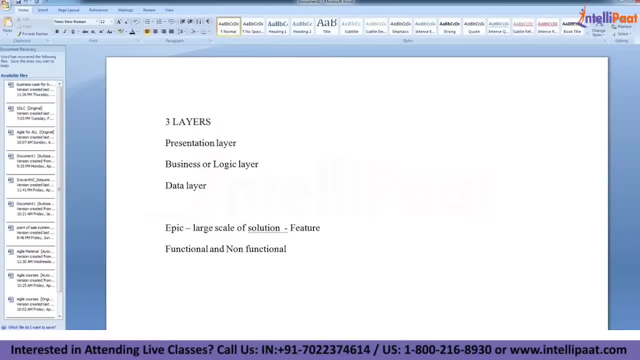 Now feature called GPRS tracking device. Now you are driving a car, You want to reach to the destination point, So for that, this device, you want to use This feature. you want to enable, You have to use it. If you want to use this feature, what is that you require? 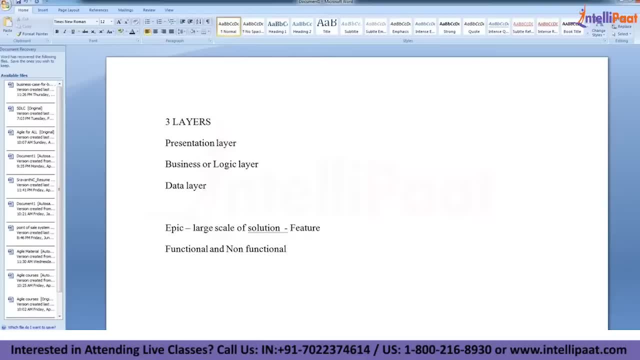 first. First, you have to enable it, You have to enable it, You have to enable it, You have to enable the location where you are now. You have to select the location where you are now. first, Point number one, Point number two: You need to select the location where 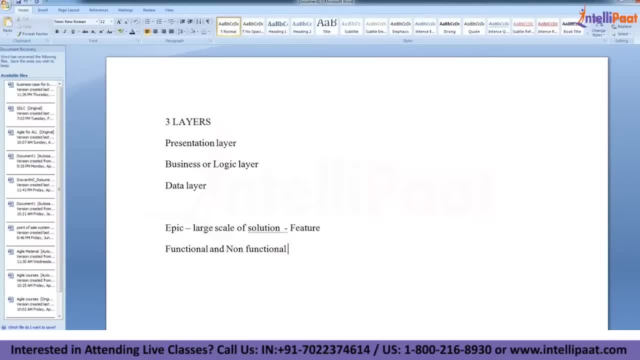 you want to reach finally, Right. So whenever you are selecting these two, you need to have an option for submit. So whenever you are submitting, click on the submit or okay button, whatever it is. It will show you the direction, How many miles or how many kilometers it will. 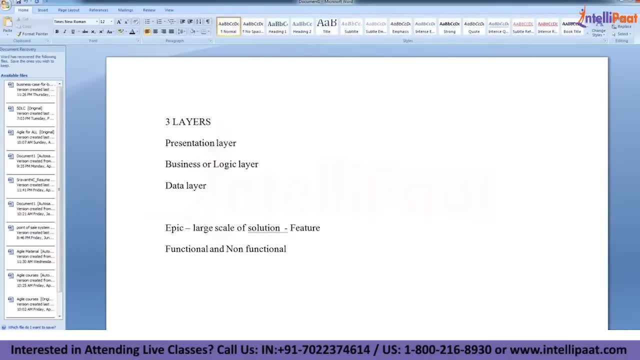 be taken for you to reach. This is what the road it will show. Next, you will be having a button called start Right. So whenever you start, click on the start button. it will tell you right. So go straight, go left, go straight, go right. all that stuff Once. 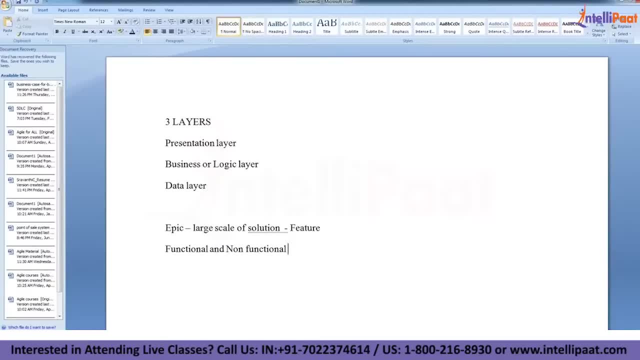 you have reached the destination point. it will give you a voice message that you have reached the location. This is either in the left or right hand side of yours, right. This is what, generally, the device is telling you. Now assume that nothing of this, whatever. 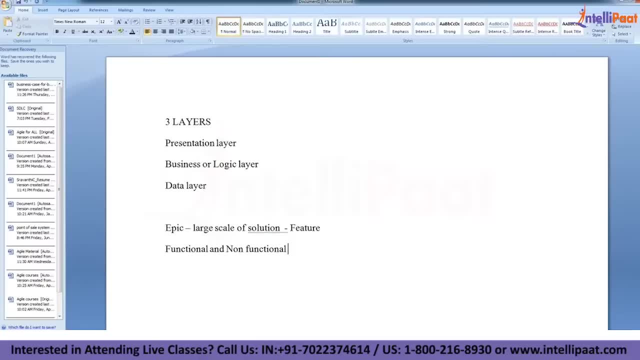 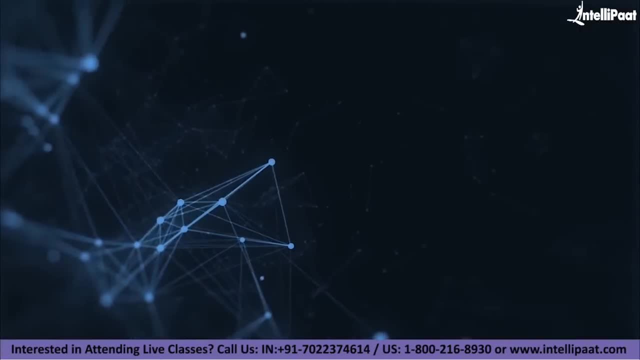 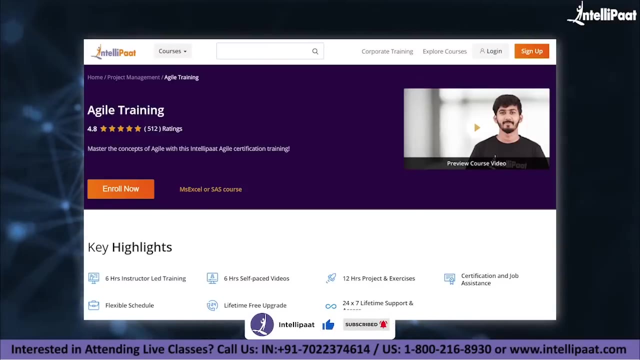 I have explained you so far. was not there in there, uh, was not there in the feature of GPRS tracking. Is this having any value for that? Just a quick info, guys. Intellipaat provides agile trading mentored by industry experts, The course link of which is given. 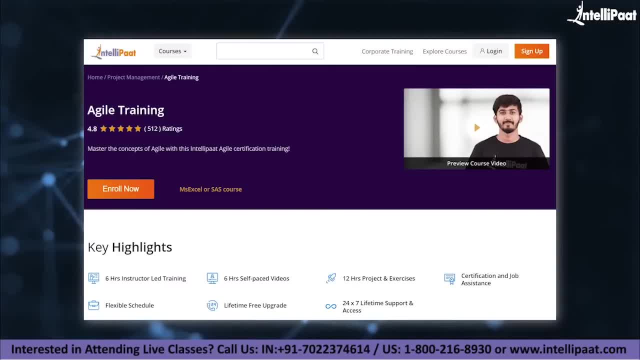 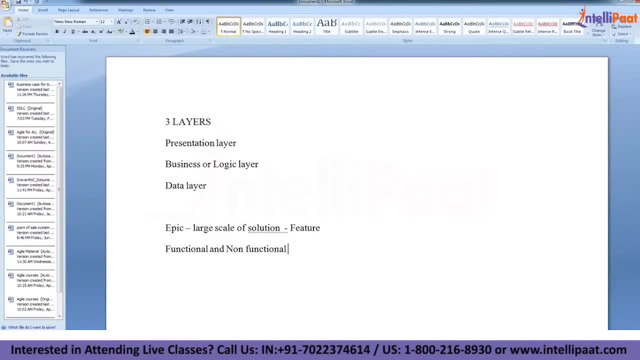 in the description below. Now let's continue with the session. Right? So there doesn't have any value. So, if you're talking about GPRS tracking devices, feature when this is be helpful, when this is be useful. there are some functionalities which has to be developed. 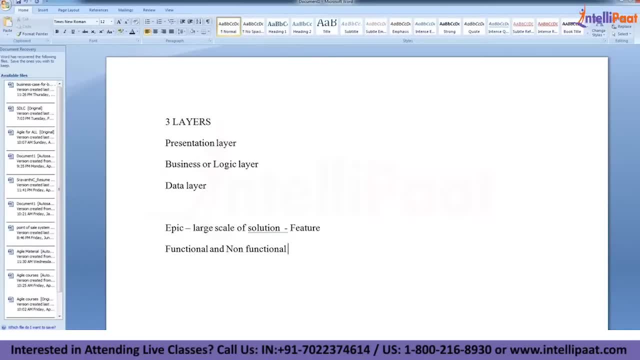 in GPRS tracking devices, right? So what are the functionalities? Well, the functionalities are. you know, you have to have a feature that has a value, Otherwise it doesn't have any value. So what are those features, Whatever I have explained so far, So those we call. 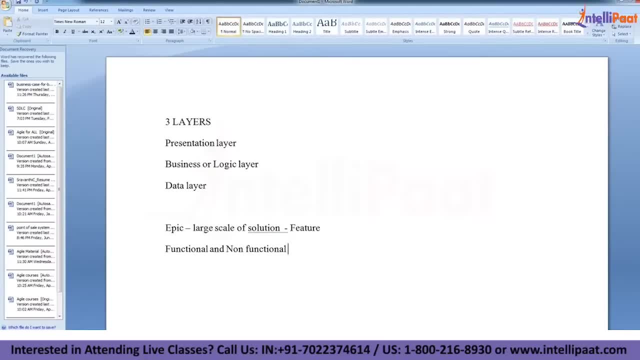 it as functionalities. So every feature must be having some functional requirements. Now, what is non-functional? Non-functional means how it should behave, character of the functionality, how it should behave. This is what non-functionality. non-functionality means performance, scalability. 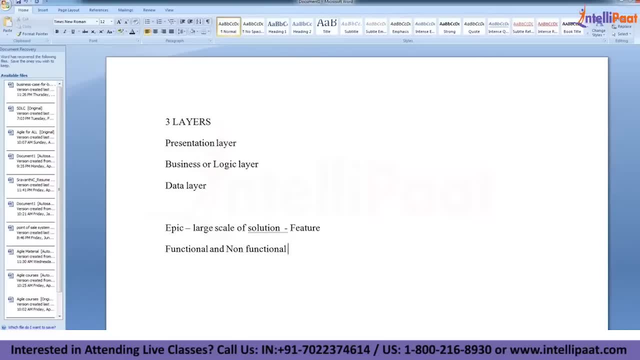 right. So all that comes under non-functional. Let's say: you have reached the location and you have reached the location. You have reached the location and you have reached the location. You have crossed even After once. you have crossed after three, four minutes, you have. 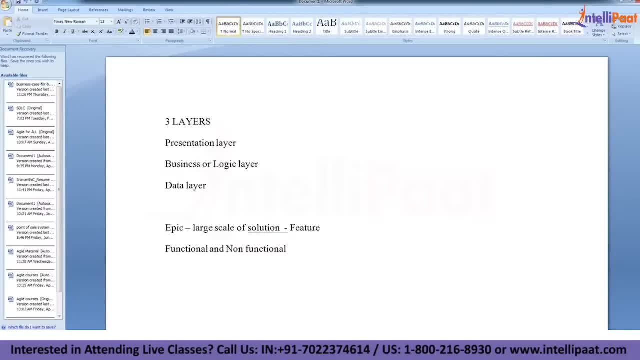 got? you got a text message or you got a voice message. What do you feel when you're driving a car which is located, which is the location you are, which is not known to you, right? So you're simply, you're driving the car. Anyway, you have an idea that, anyway, you get. 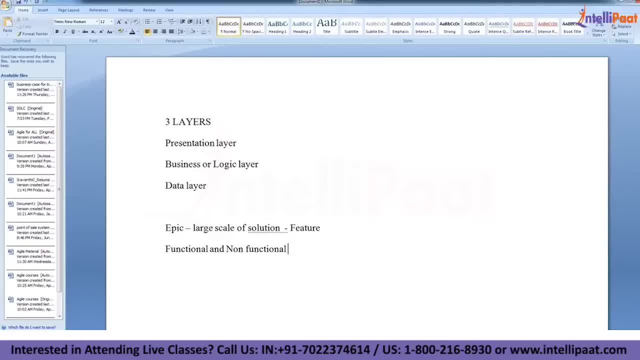 a voice message, right, But after three, four minutes or so you got it. So what do you feel? usually, being a person who is driving the car, you feel that this device is not so accurate because it's not. It's not giving you the instructions to you prior, right, It's giving late. Maybe it could. 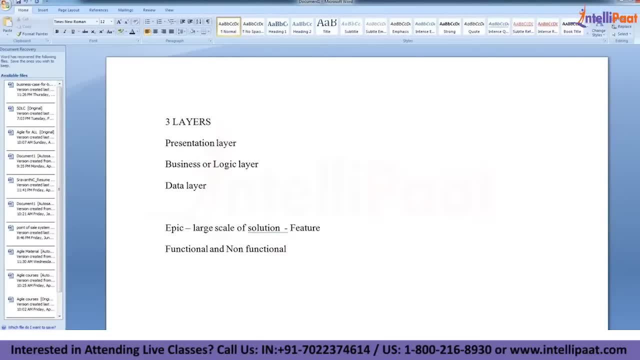 be for whatsoever reason. So what is that? You see you, you'll be deciding based upon the performance of the device at that level. So what features and functionalities we are developing for any customer? end of the day, that has to be performed well, right, So you? 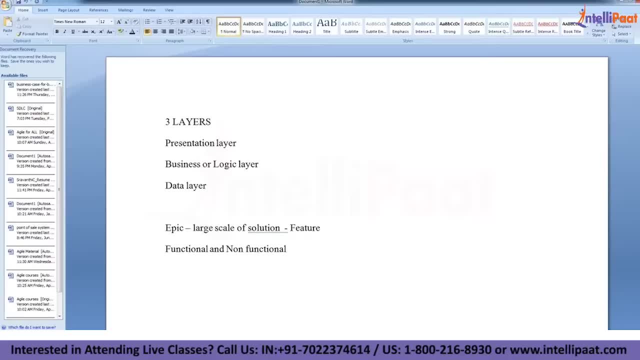 are developing a, for example, you are using an e-commerce portal for shopping all that stuff. So you have chosen the products, you have kept all these in the cart. Finally, you have edited something, you have paid. Finally, you have decided the products, You paid the. 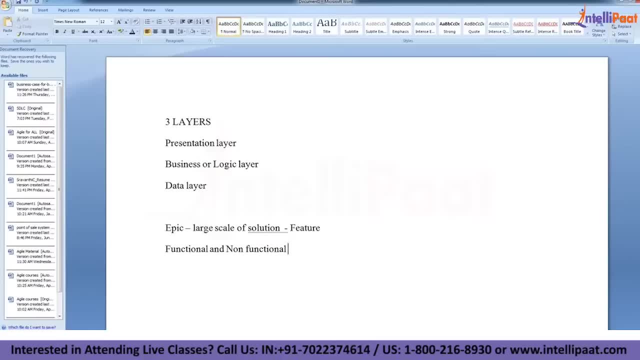 bill online using different, different payments. What do you have paid it Now, once you have paid, if you normally the rule is that, because normally these instructions, why I'm saying all this? because non-functionalities will be explained by the client. client will tell. 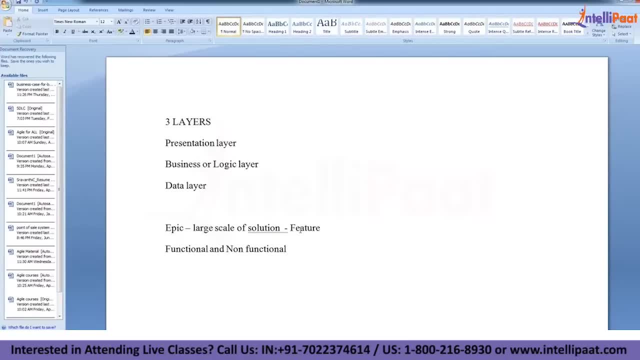 you right. For example, once customer has paid within fraction of two or three seconds, he has to get a reply message. What reply message sucks? Thank you, Uh, thank you with shopping with us, So that you will be receiving your products in another two to two to three business parking. 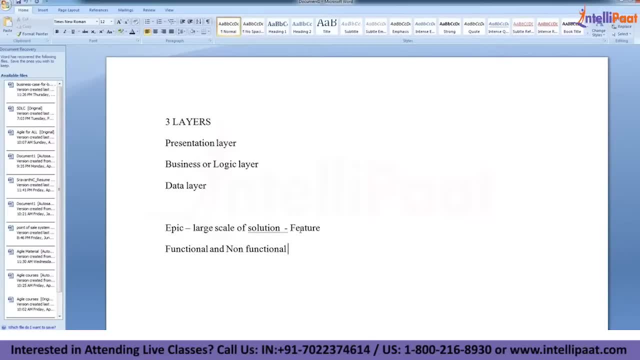 this to your doorstep, right? So this is what the message then? only, being a user, being a customer, you feel happy, right? Assume that it is dated. It is delayed, right? So pay. payment was paid, It was debited from your account. everything done, but you have. 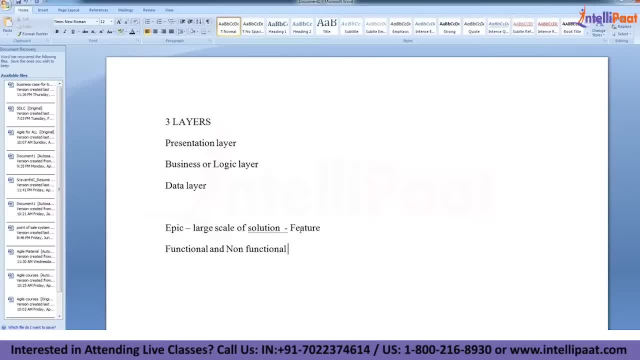 not get. you have not received any kind of reply message so far. What do you feel Right? So you may feel suspect. Is it because it is detected in my account but I didn't receive? whatever the reason could be Right. So it was delayed maybe five minutes or 10 minutes or 15 minutes. So if it is happening, 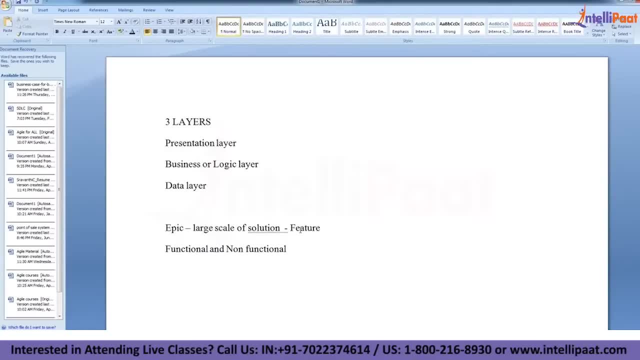 every time, right? So if it is a happens runtime, okay, fine, It may be because of server issue, all that, but assume that, understand and think that way, that it is happening every time. So what do you feel? Normally? you feel that it is inaccurate right? So it's not so accurate. 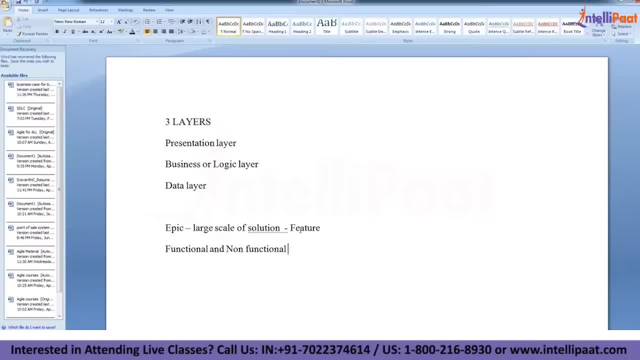 as what we understood, what we think of. This is what we call it as non-functionality, So functional requirements are required, non-functional requirements are required. So what we call this non-functionality, So functional requirements are required, non-functional requirements are. 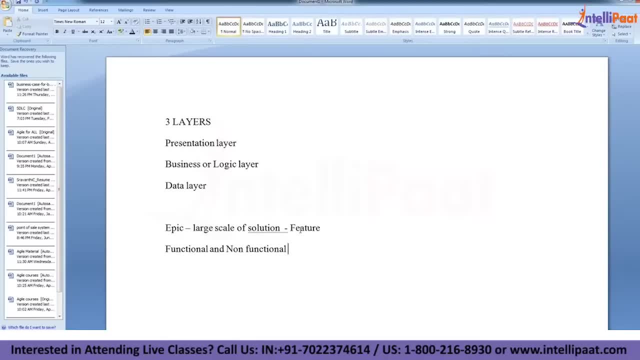 required non-functional requirements will also be there. So, normally, whenever we are preparing documentation, whenever a business analyst is preparing documentation, this functional and non-functional requirements will be prepared on the document usually. But whereas in agile area, as I mentioned you, there are no documentation and all everything. What is that we have to? 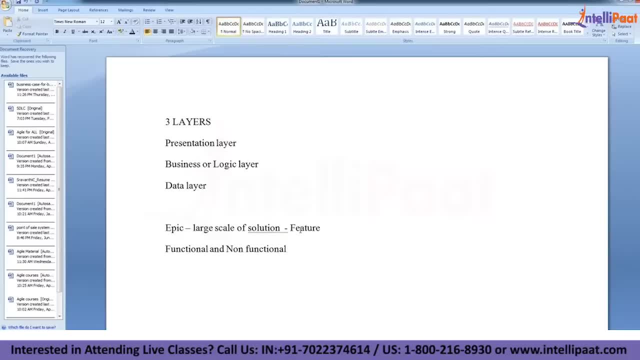 do? We are writing user stories. So what is user story means, whatever the functional and non-functional you are writing, That is what generally we are writing in a form of user story. So what is user story? User story, nothing but a short description of what user story is. 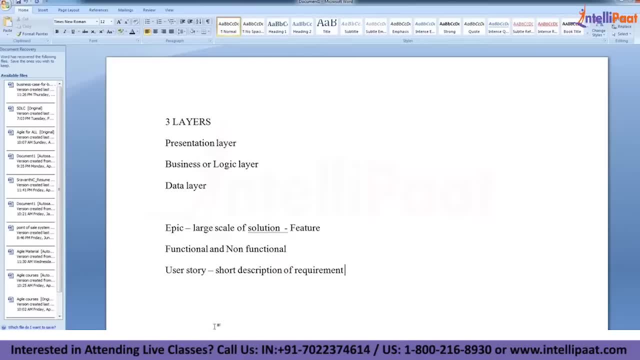 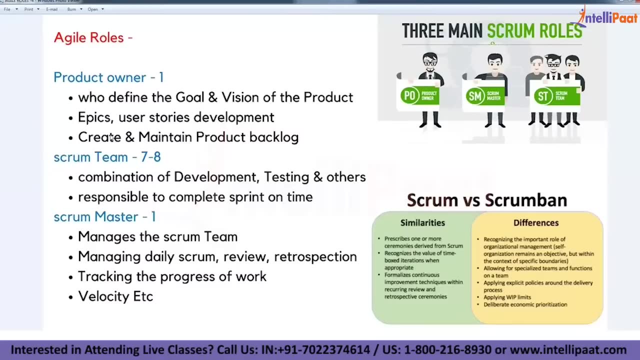 Short description of requirement. So epic has to be identified, right. So epic has to be created for every epic. Epic means large scale of solution or, as in feature, whatever it is. So for every epic. what is that you require? You need to have multiple user stories. 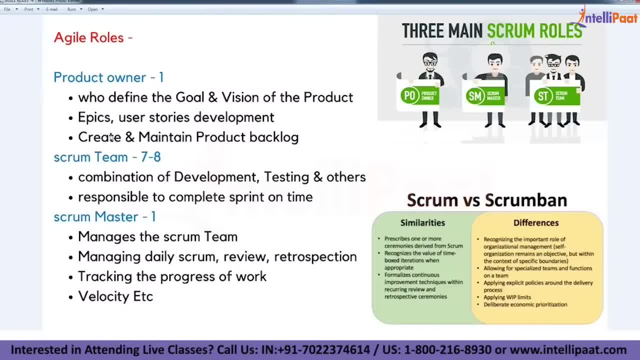 either functional or non-functional requirements. You need to develop some user stories for that. What is user story? User story is nothing but short description of the requirement. For example, customer wants you to develop a login page. right, This is one thing. So 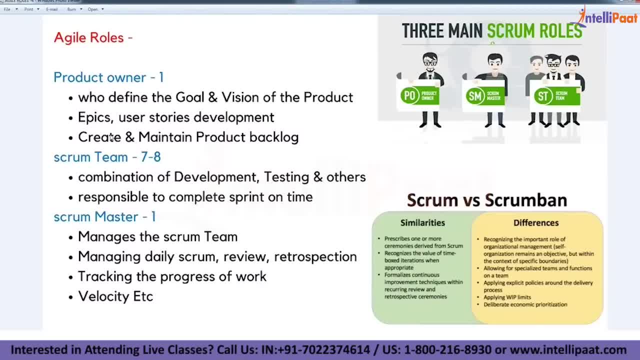 how we are going to show this. Assume that you are a product owner- right, You are. all belongs to the product owner. Assume that you are all product owners. You want to explain the same thing to the technical team. How do you do that? In what way you will be presenting 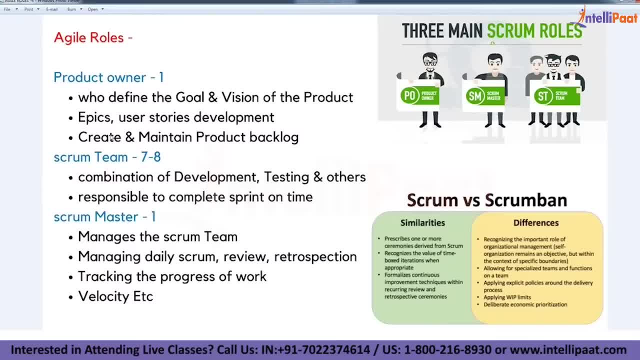 this. This you are presenting in a form of writing down the requirements. So you are going to write down the user story. User story is very simple: How to write user story. that I will be explaining after the next session onwards, you will be knowing it. How to write. 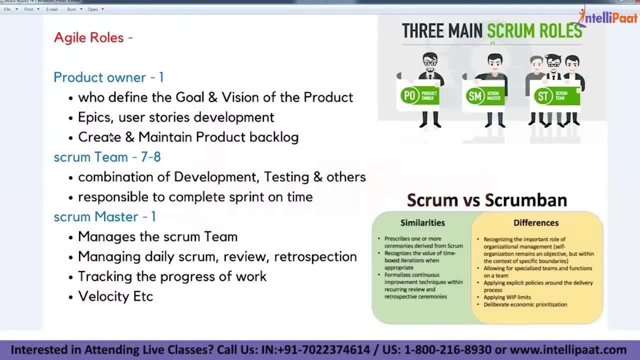 user story. To write a user story there is a template we follow that I will tell you later. So writing down the user stories, all that stuff has to be done by the product owner. So there will be epic, followed by epic, There will be user story. This is what generally 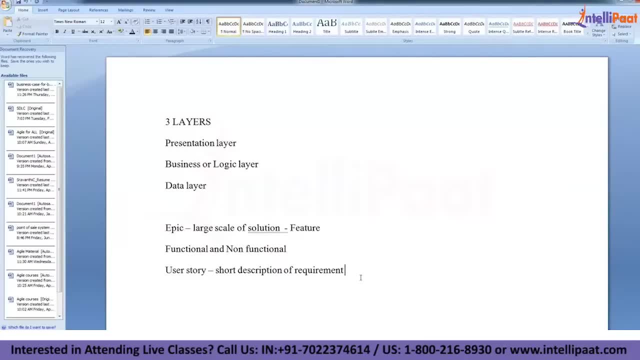 we write. But user stories can also be minimized. That is a different thing. User story can be minimized into subtasks. All that we can do Because whenever we feel in real environment that user story is having a complexity, in order to reduce the complexity, whatever you. 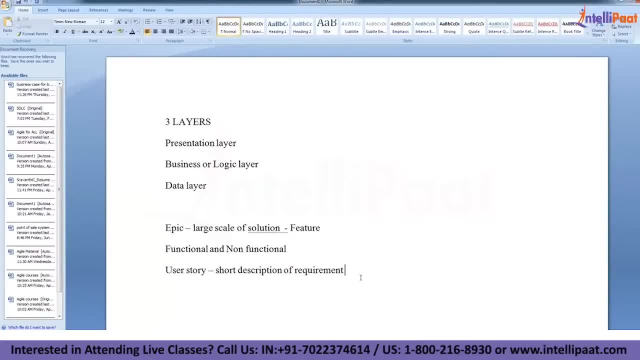 do that user story will be diluted. It means divided into multiple chunks, Those we call it as functional tasks. So again, those tasks can be divided into subtasks. So that's a different story. That is not going to. So creating of epics, writing down the user stories, 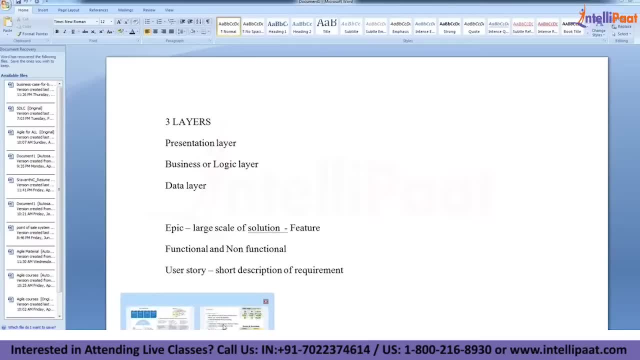 is what generally a product owner does, So that's a different story That is not going to So creating of epics, writing down the user stories, is what generally a product owner has to do. This is the second point Now. next, creating and maintaining product backlog. 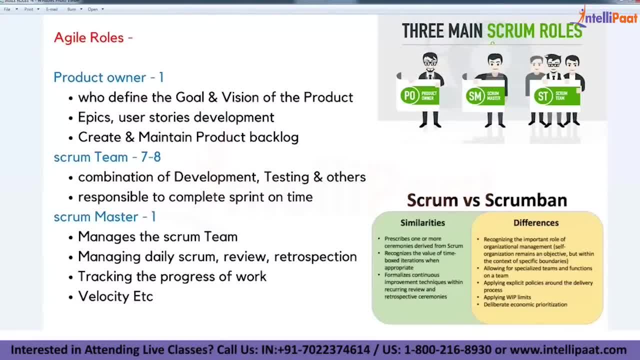 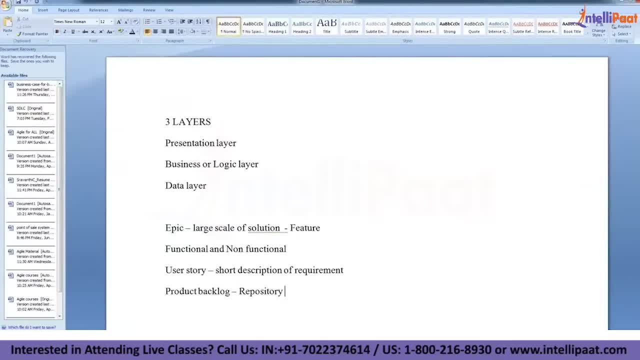 This is also a responsibility of the people. What is product backlog? Product backlog? nothing but it's a repository to store all the user stories. Repository to store all the user stories. This is what generally product backlog stands for. Because, for example, 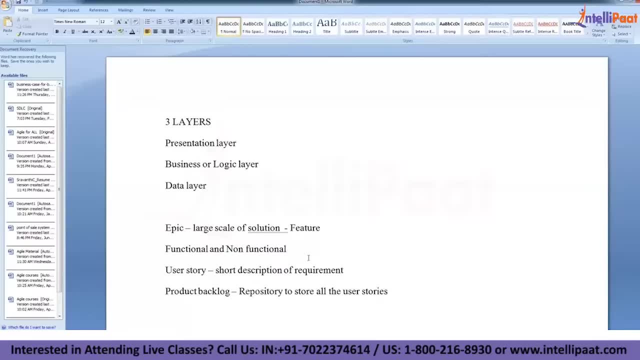 we were writing multiple user stories. This may be crossing somewhere 40,, 50, 60 user stories. we were writing: Where are we storing the user stories? Where are we storing the user stories? Where are we storing all that information? That story is nothing but product backlog- Product backlog. 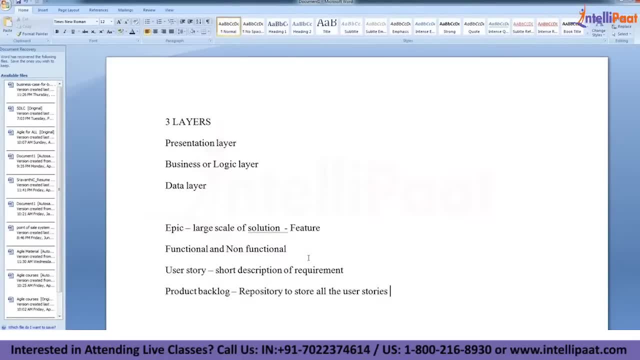 is nothing, but it's a repository to store all the user stories in that. So you are storing all the user stories so that, based on the prioritization and all- whatever the sprint planning and all everything we do, it comes in that next. 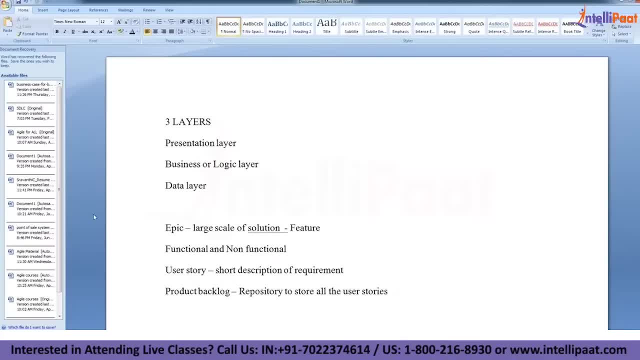 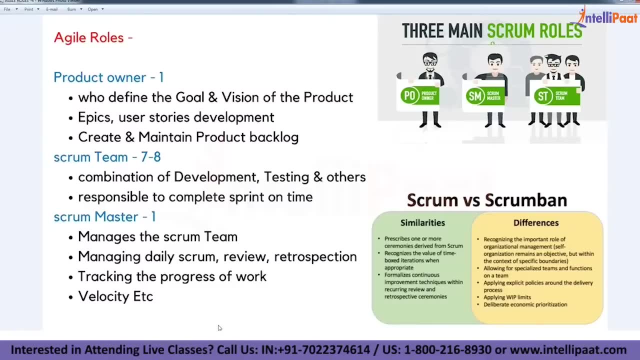 So, being a product owner, the major responsibility we do is that, first of all, we have to define the goal and vision of the product. That is the first thing, being a product owner, you to do, unless until if you are failed in doing this project or the the work, what we are doing. 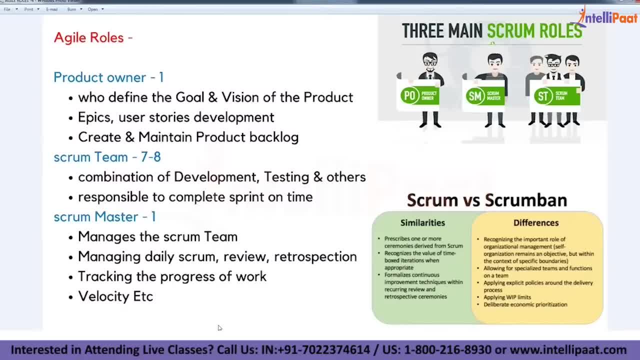 going to do will be under the tool drops right. so going goal and define a vision of the product is important point one. next, you need to develop epics, followed by the user stories. this is second. what is epic, what is user story? i have told you how to write and all everything that we discuss. 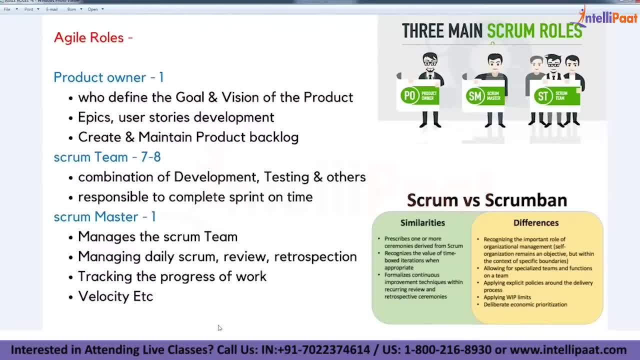 it later, because our discussion is confined totally to what are the roles and how it functions. so how to write, and all comes under the next level, how to write user stories. for that there is a three-step procedure. is there that we follow at the same time when you want to write a user? 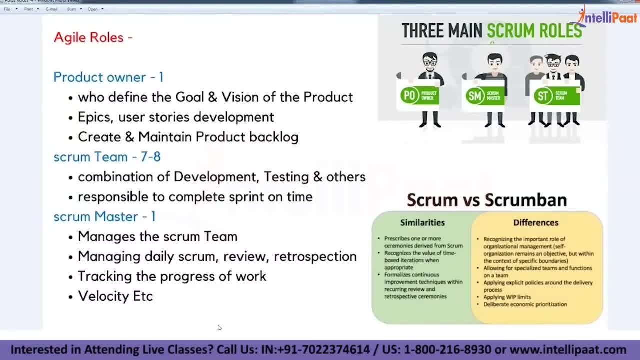 story. there is a principle: invest principle is there? so, based on the investment, because user stories cannot be written like, as, as what we feel right, because it must be having a value, it must be having a quality. then only that user story will have an identity and recognition, otherwise there. 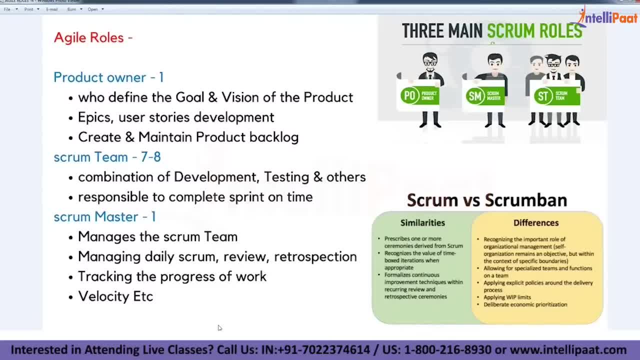 is no part of it. so user stories that there is. there is something like: i'll tell you right, so this is user story. next, whenever you are writing down all the user stories, there must be a repository to store all that. so where are we storing all that? this is where we 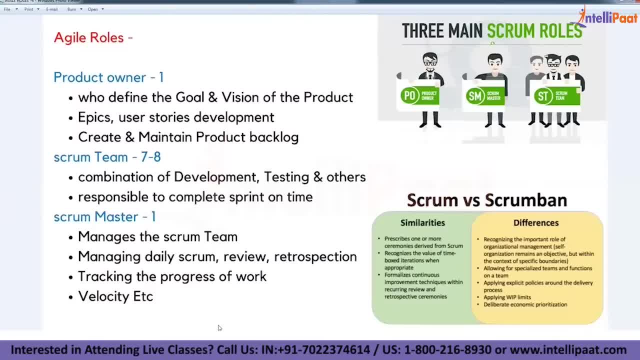 call it as product product backlog. so you are creating a product owner, product owner. if you are a product owner, you have to define the goal and vision of the product. is your responsibility. you need to write down, understand the epics followed by the user stories, creating and. 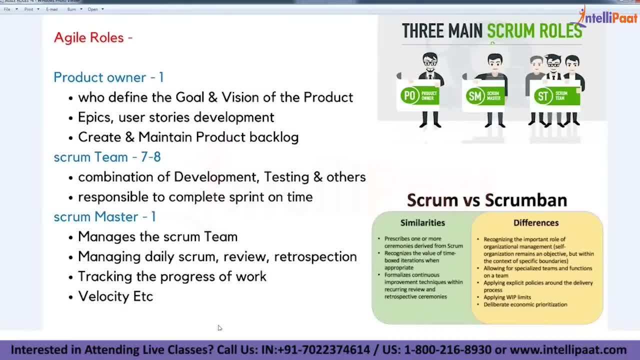 maintaining product. so this is what: generally, being a po, you're responsible. so most of the people who are from a business and this background we landed. if you are, if you are in agile, this is most of the times- you'll be a product on a majority of occasions. i can say: right, this is one thing. second, next role will be called a scrum team. 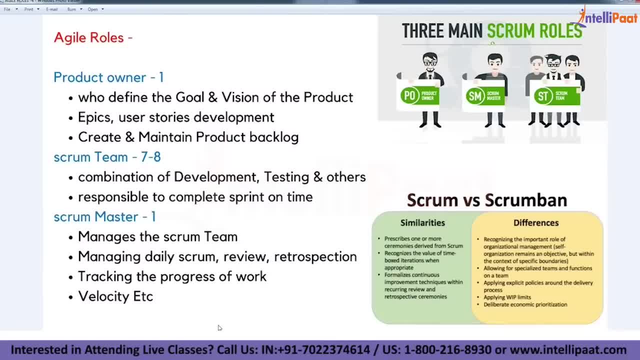 what scrum team is. this is where almost this is what i have told you. right, cross-functional teams like both developers, testing team. even sometimes you may be having a business analyst or architects. right, user interface designers- you and ux designers. right, user interviews. all these people will become sentence. scrum team means people who are responsible to complete. 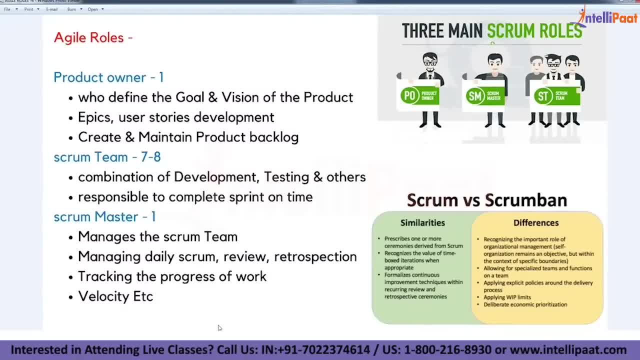 the amount of work which was given to them is what we call it as scrum team. scrum team- nothing but development, in simple words, because we are what we are talking about: scrum. that's the reason why we are talking about scrum team, right? so when, when people are using kanban and all everything, 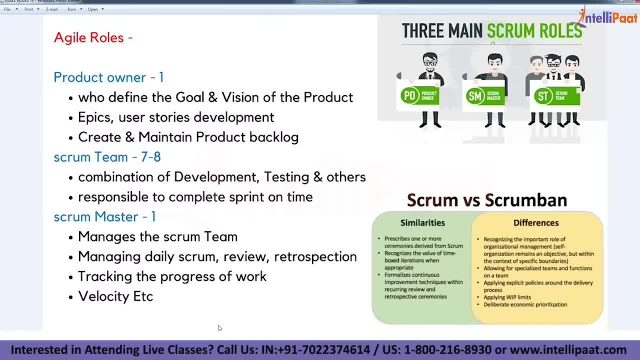 they call it as development, not scrum team, because scrum the reason, scrum team, otherwise it normally it is considered and called as development team. what is development team? development team? nothing but members who are combination of all those people will be under the same team, so these people should have an expertise: multitasking. that is what i told. 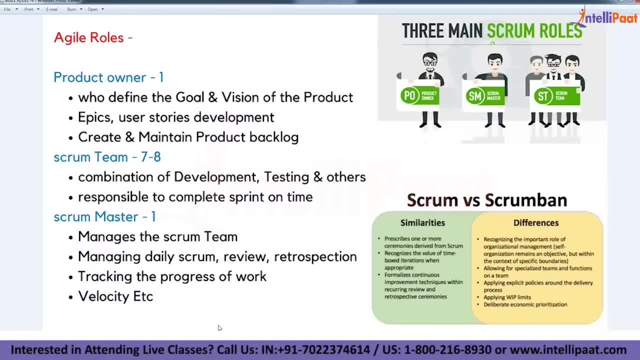 you. in the beginning itself, multitasking is what essentially needed for the team members to perform right. so if you are a team member, if you are a scrum team member, you must be capable enough to do it right from the analysis part to deployment and delivery. you have to be involved in each and 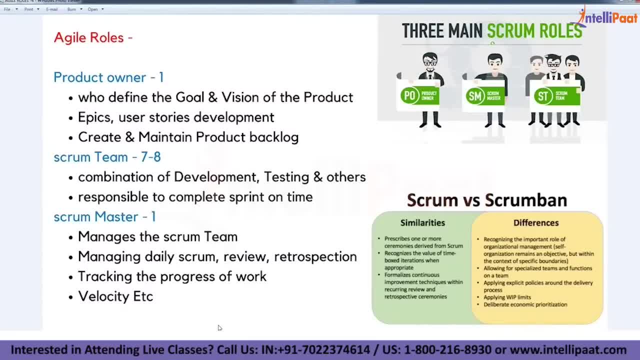 every stage means you must be capable enough to handle all that stuff. this is what generally, the scrum team responsibility is. normally these people will be somewhere around seven to eight people in percentage for one team, right. if you have multiple teams, seven into two, right? so this. 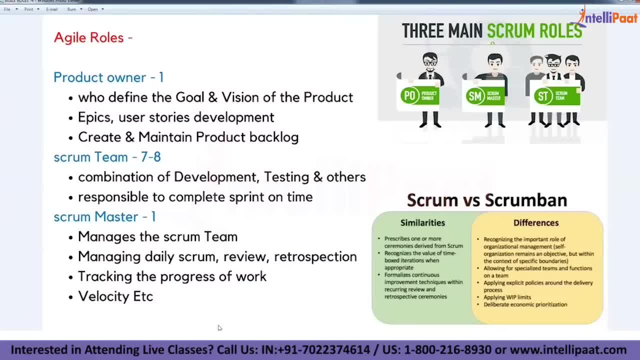 is how it is right. so, every one thing, you will be having somewhere around 78 people. in simple terms. so if you are a scrum team member, you will be having two developers, two testing team, maybe one database designer, user interface designer, maybe one. sometimes they'll be hiring a business analyst. 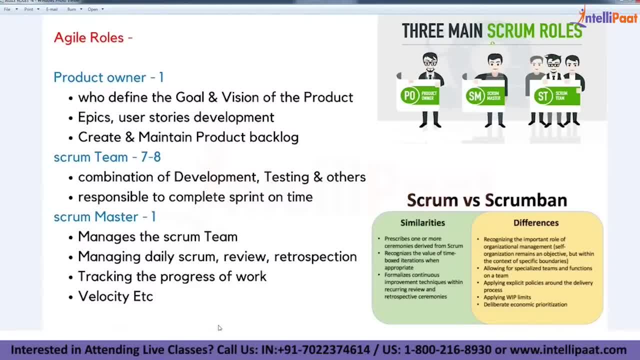 also right. so because one business analyst is a product model, you may be require one ba, who will be with the team members to coordinate different, different things. depends on their interest, depends on their business. they'll be adding people, but the team members who are in the scrum team. 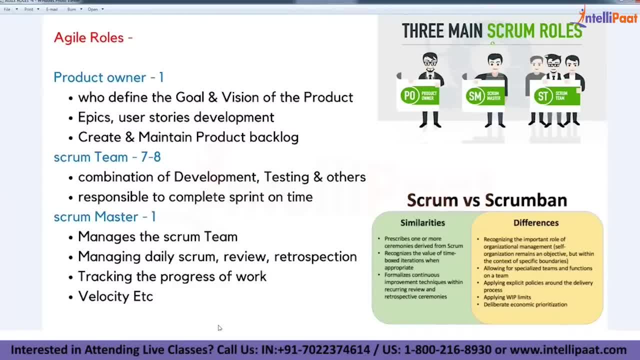 members are responsible to complete whatever the given task to them means. whatever the task, normally these tasks will be divided as a sprint. usually we call it a sprints, sprint development. all that stuff comes into picture that i will tell you. so usually, whatever the activity means in simple 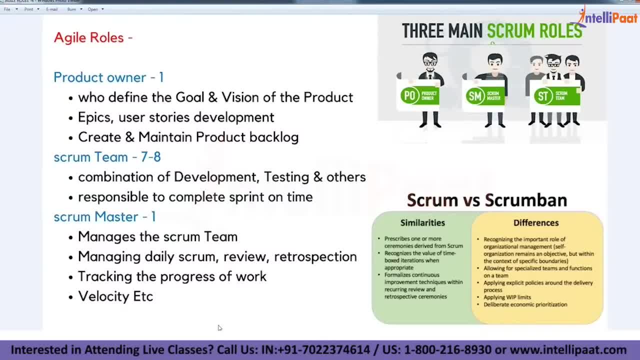 terms, whatever the task given the task, completion is the responsibility of the team. decision should also be taken by them. normally, in traditional model, if you see project manager or project management team and all, everything will decide right project planning, all that will be decided. responsibility will be more on their shoulder. 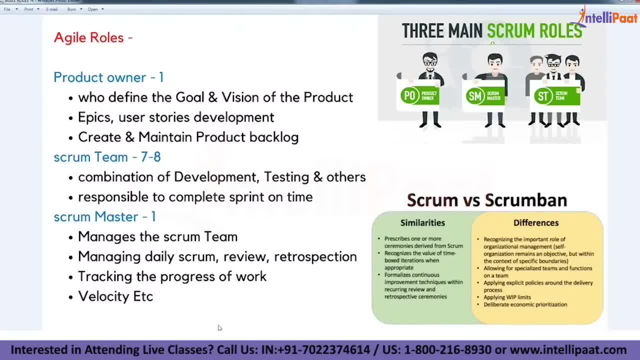 but here, here is self scrum team is a self-organizing team, so there is nothing called boss, there is nothing called pressure. all that, of course they have a pressure because when? because in the beginning also i told you why. tactically, because, as in, as i am into agile. 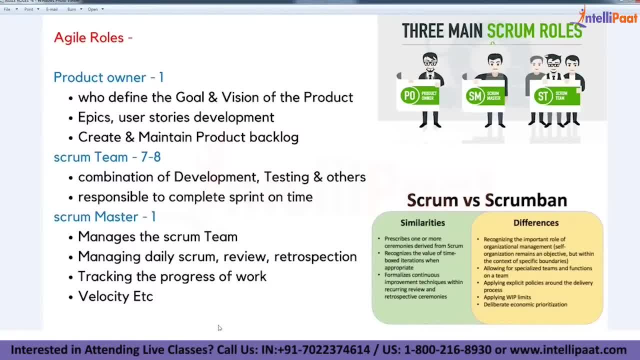 coaching because i am an agile coach now. so what i can, what i could see closely, because i am dealing with lot of clients, i am dealing with lot of business owners, all that stuff. what i could see is that why they are wanting transform their organizations or the 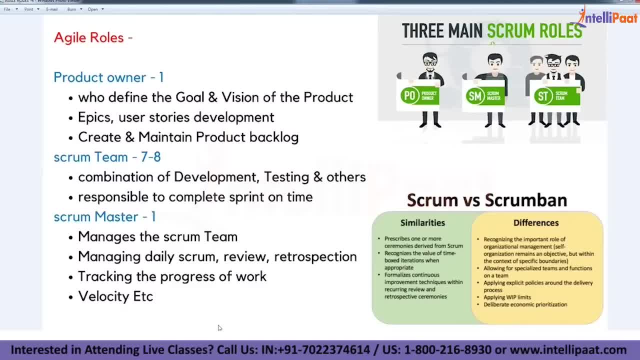 projects into agile because they want to make everyone accountable- responsible first, see slowly, when i am putting a pressure. see, i want to make you accountable and responsible for the deeds. what is that i have to do? i need to give you responsibility for everything. so i'm giving. 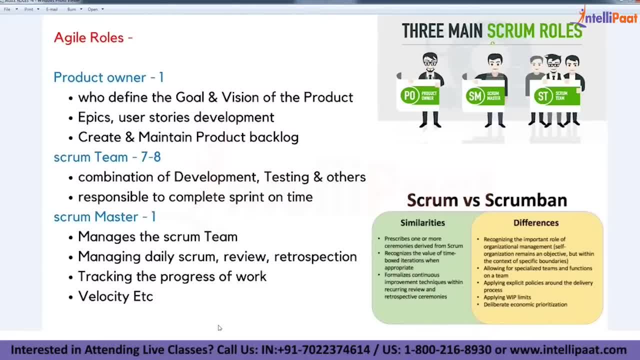 responsibility automatically. you will be accountable for sure, right, so i need not do anything for you, right simply. if i do that, you will be accountable and you will be. it means this: the persons who are not right- i'm saying right, so this is not in a negative sense- people, some people. 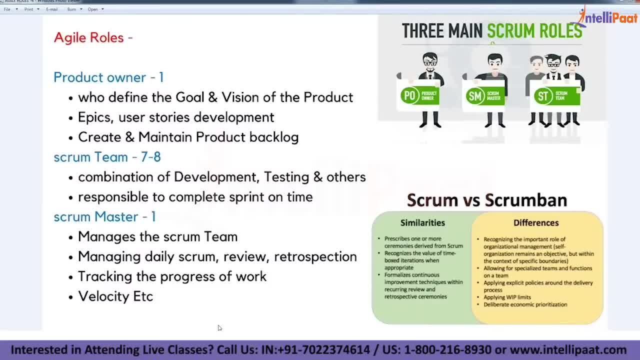 try to escape, right. so people say that this is not my work, this is not mine, all that stuff. for them, this agile is the right one because they are accountable for everything. they are responsible for everything. responsible and accountable for everything. that's the reason why multitasking. 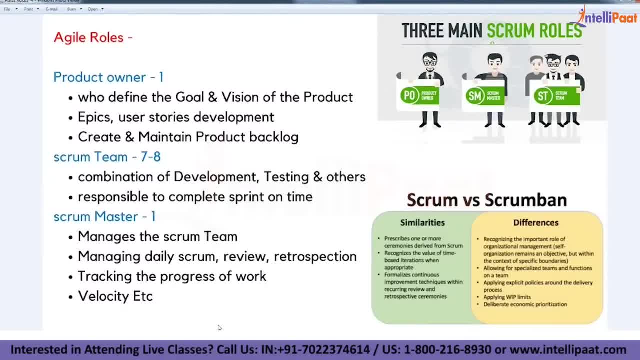 is required means, whatever the piece of work must be given to them, they have to complete within the timelines. that is what generally scrum team must be capable of. so whatsoever reason. for example, if i am giving two weeks time at any cost, in two weeks you have to complete end of the day for. 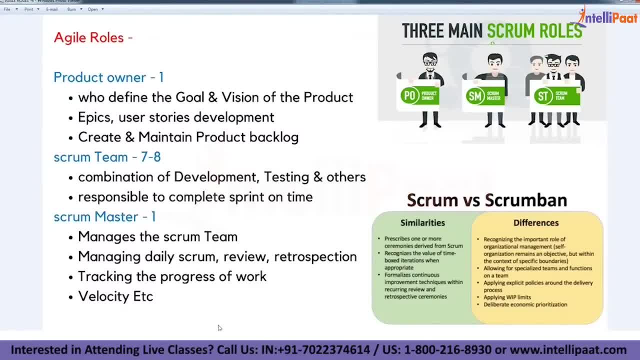 that what is required- team spirit, team management is required. team effectiveness, right team dynamics- all these were matters. so no individual performances will be identified or recognized in agile as a 100 team effort, self-organizing team. whatever the decisions they are taking, everything is belongs to them. what work to start, what to initiate? everything that responsibility, everything. 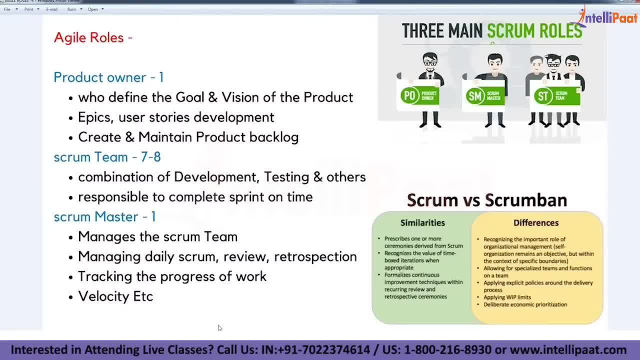 will be on their shoulders. normally in the traditional model, that's not the way task will be given. these people will do it, but here, whereas in agile and all responsibility will be given to them. so it is everything in their, on their shoulders. they are the responsible persons of. 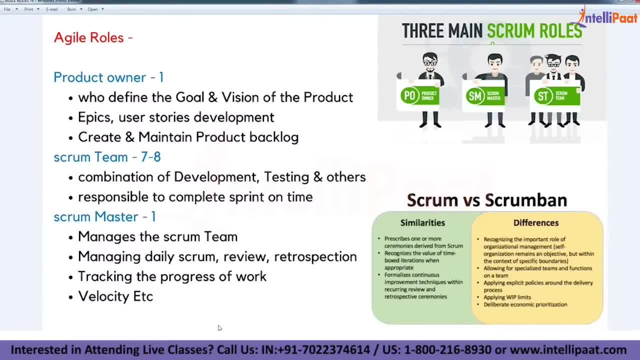 the deed which is being initiated, which they have to work on, so they are responsible for everything. this is what generally scrum team stands for. so, right from analysis, planning, design, implementation, testing, deployment- if they are completing two weeks, for example, if i have given a task where 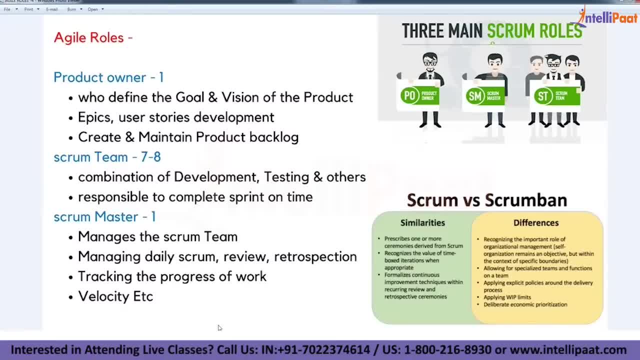 i'm asking you to complete in two weeks means two weeks. the whole thing has to be completed. you cannot say that i just excuse me, i did, i do. you cannot say that it is analysis or planning, design two weeks that particular task, whatever the user stories we have given to you, you guys. 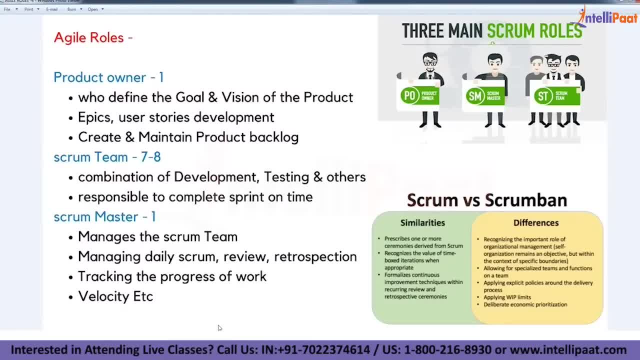 have to be completed in two weeks, all everything right. so you dusting, everything has to be completed and you have to put it straight. this is where generally cross-functional teams, this is where generally these teams called as cross-functional- cross functional means everybody- are involving in these activities and all these these people target is to 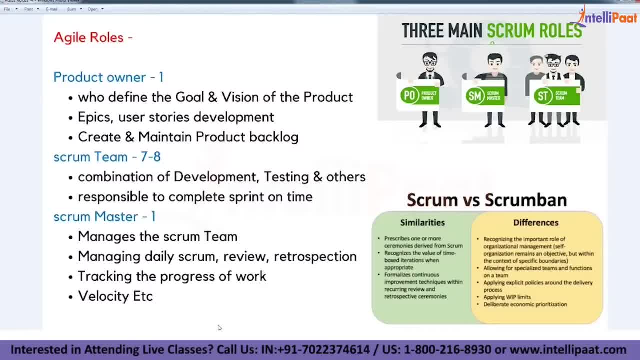 reach whatever the goal and vision which product owner has defined, if they are failed in doing it. so there is no point in working on it, because product owner will always, always have a right to cancel at any time. whatever the sprints they have defined and all they can, product owner will. 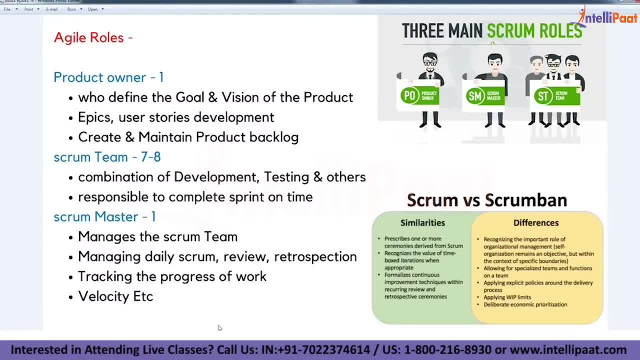 have a right to cancel any time, so that that is what generally product owner will have: that authority over the team, all that stuff. so scrum team is responsible for that. now scrum master, scrum master- nothing but more or less a project manager. no, i'm not comparing project manager to scrum master. 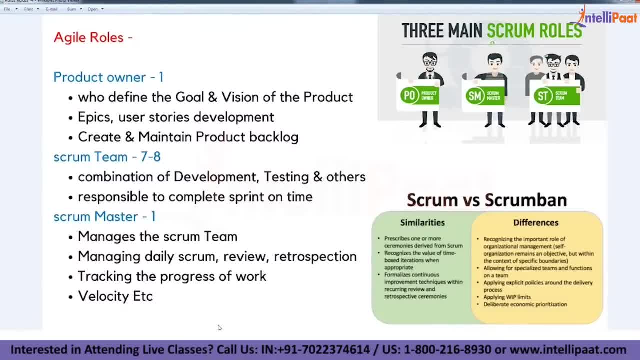 because project manager, roles, responsibilities, authorities will be different practically speaking, but scrum masters doesn't have that, because that's a reason why scrum master will be called as like what i can say, like scrum master will be more or less like a: they are licensing the team. that's it right. so they are licensing the team. 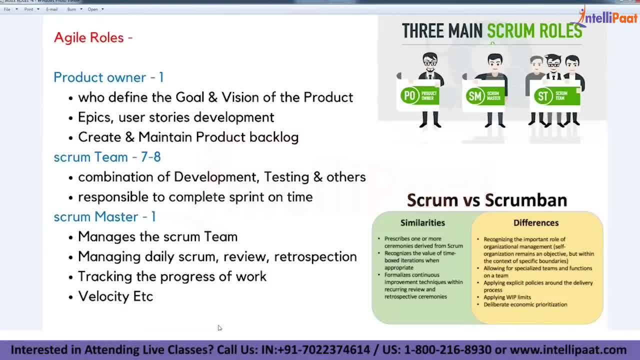 and whatever the requirements they want to have, right. something like assisting the team, right. so whatever the challenges they are facing, all that will be taken care of by the scrum master. so scrum master is some more or less- i can say- a project manager role. i can say more or less. 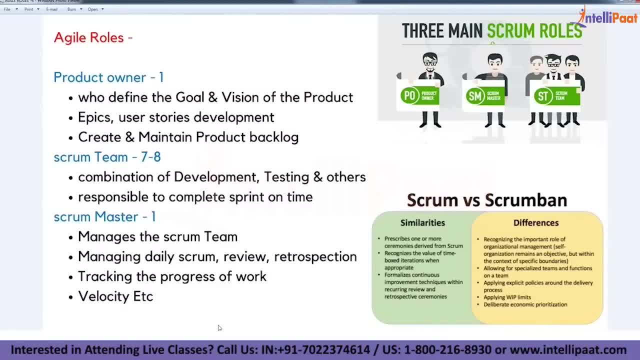 to that extent possible, more or less as a project manager, or is what generally scrum master do? usually scrum must is the one person, but scrum master responsibility and role is more important in the job because they have to manage the team first of all. first point right. so they need to understand. 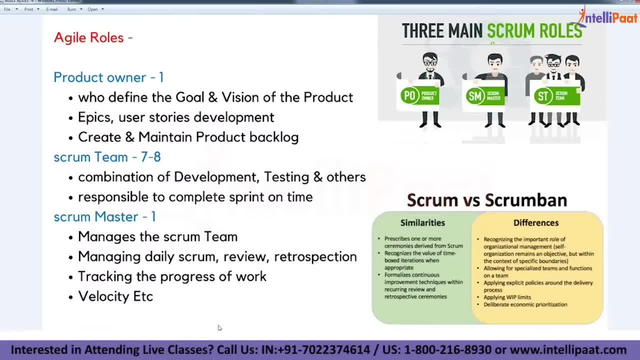 whether these people are capable enough to complete or not, because some people recruit. see, recruitment will happen usually, but we never know whether these people are capable to do it or not. some people will hasten to do, some people are reluctant to work right, some people will have 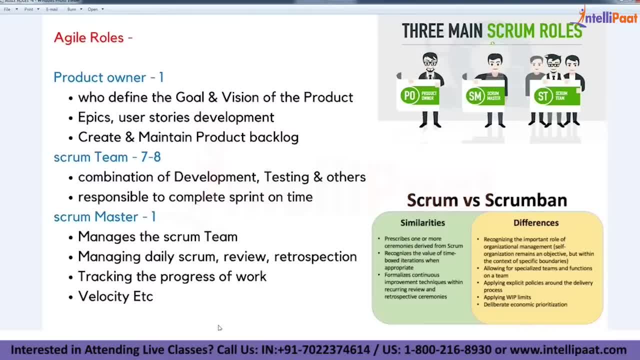 some pressure, right, because they are technically strong, but these people will be. there is more pressure. automatically these people will raise their hands. this is different, different, right. so we have behavioral traits, especially an agile, especially because- because we are i- if you can take mine as a profile, i can say i was a. 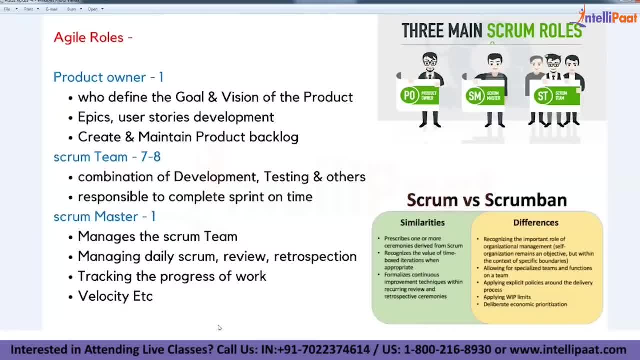 scrum master earlier. then i was turned as myself, as an agile coach. now i'm an agile coach, exclusively, right. this is how my transformations. so if you see a scrum master role or an agile coach- because agile coaching experience should also be there for a scrum master, so these people should also 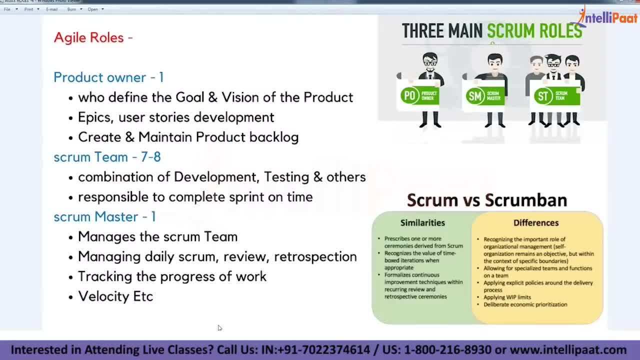 have experience in understanding the behavioral traits of the individuals. behavioral coaching- all this comes under agile, because it's not something uh like managing the team and all. you need to understand the behavioral traits of the individuals, because some people are technically strong, as is stated, but they are not there. there is more pressure, but right, so they can't work. 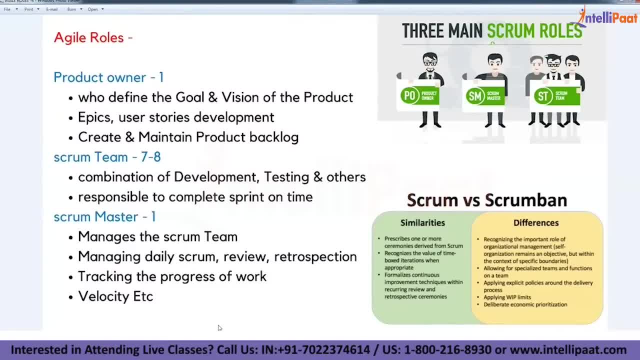 some people doesn't have any technical knowledge- because not to the extent of the technical knowledge, because not to the extent of the technical knowledge possible- but they know how to manage things. so we have to deal a lot of people and at the same time we have to make people to work in the stipulated timelines which was given here. all that stuff. 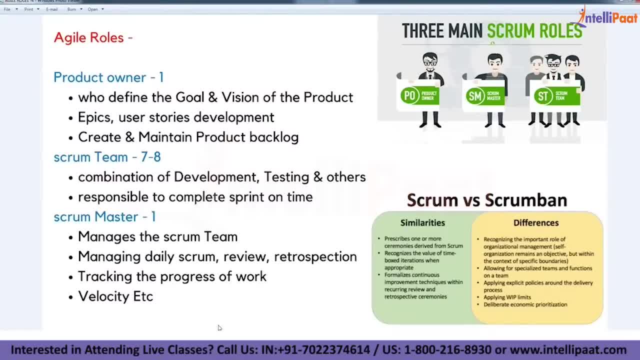 same time, scrum master, it is also having a responsibility to track the progress, what is being given to them. because, for example, two weeks is the time i have given. i have to make sure if i am a scrum master, i have to make sure that you guys have to be completed this with con time or 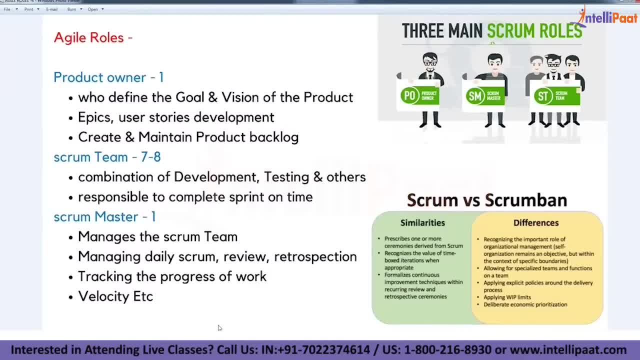 not. i have to see. if you are not completing the work, what will happen. whatever the release date we have given will be a failure. so, being a scrum master, i am responsible for all this, so i have to track the progress of the work. velocity, right. so velocity means, let's say, for example, there is one. 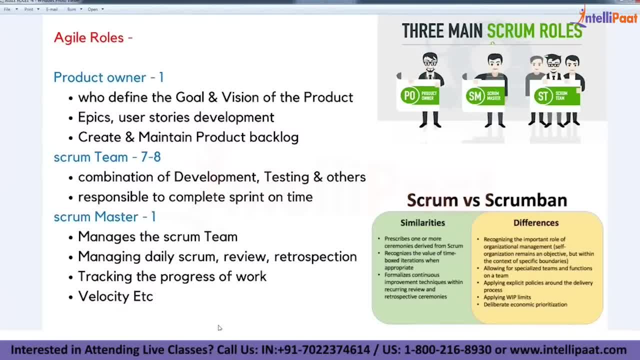 sprint. i have given what is print. i'll tell you later next session i'll tell you what is print. there are different things. when i explain you about agile planning process, you will be knowing about all this here, because we are confined only to the roles and responsibilities. so i'm explaining. 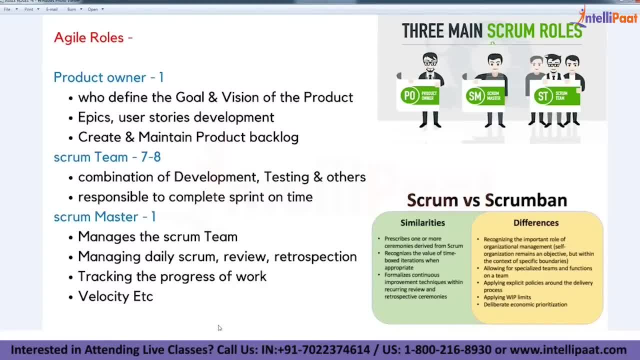 all these things to you in this session. so velocity means, for example, there is a sprint which was the same as the previous one. you guys have completed only three. one is left even on the next sprint. also, you did the same four. they completed one for whatsoever reason. if this is the case, i may be. 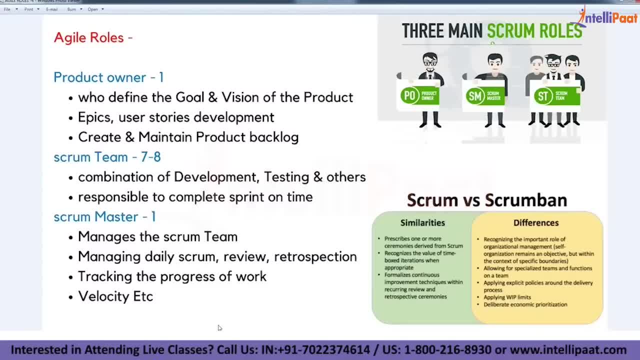 having a doubt that you guys cannot complete the release planning. what are the release planning we have? we may be failed. so what is that i have to do? being a scrum master? i have to do this velocity planning on that right. i have to see what is that i have given. what is that you have completed where? 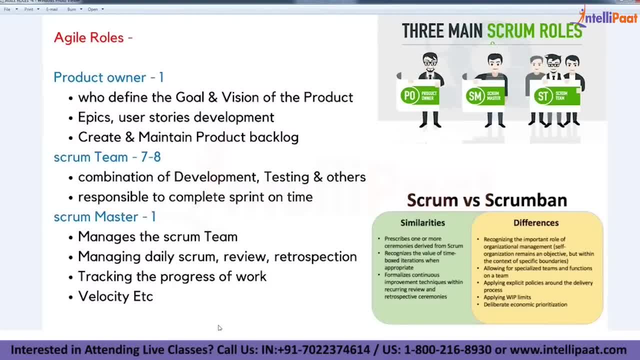 what is the balance? so, if this is the case, these people are capable enough to complete. if not, what are the things to be taken care of? means: how many sprints? additionally, i have to create all that i have to do being a scrum master. scrum master is a different role and different content. all together, this is a pretty so this. 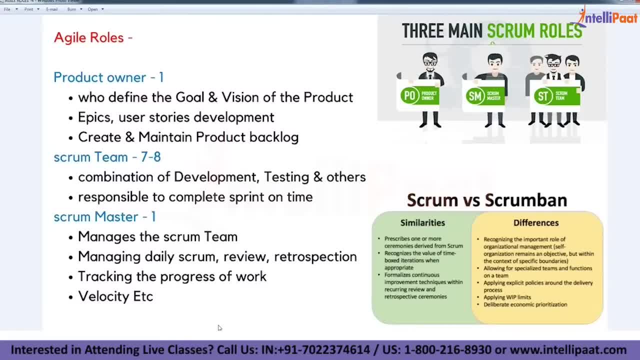 is what generally scrum masters do. scrum master, or in more or less i can say something like a project manager job, scrum must like a project manager job. this from master major responsibilities to manage the team at the same time. managing the regular works like reviewing the sprayer sprints. all the retrospections on that same. 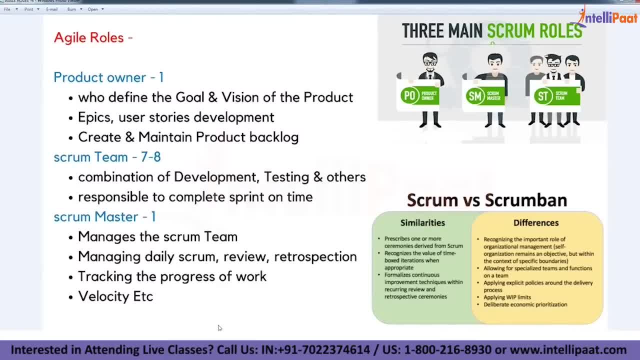 time, tracking the progress of the work, velocity, all that stuff will be done by scrum master. so these are the three different roles, but apart from all, above all, scrum master should make sure, whatever the given timelines, whatever the goal, as well as the vision, which product 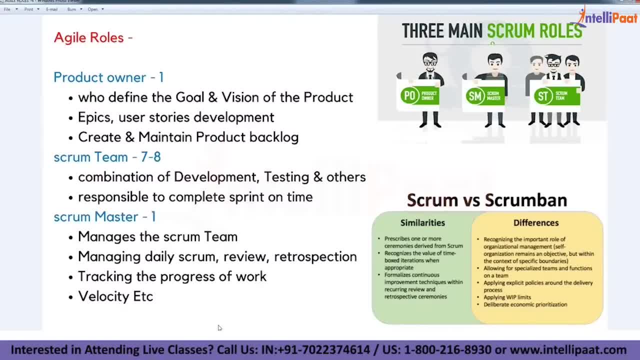 owner has track. all the scrum master always try to achieve it. that's what generally the connect must be. so then only scrum master role will be successful. otherwise there is no point of success here. so these are the three different roles, so all put together somewhere around nine to ten people, you will get one team. 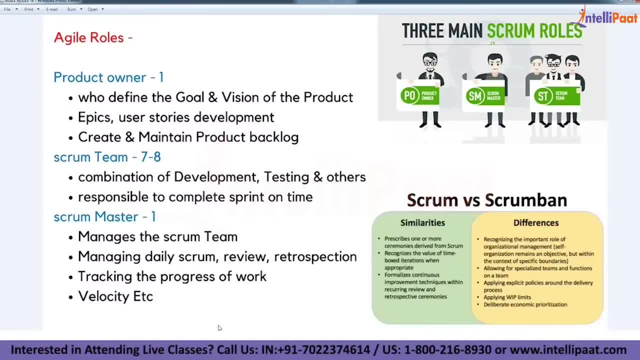 consists of ten people: one product owner, seventy eight people of team, one scrum, which is all about the roles of agile. now, when we talk about scrum, due to the roles which was decided, which was divided into three different parts, which make people to understand much better, because the person who is coming from 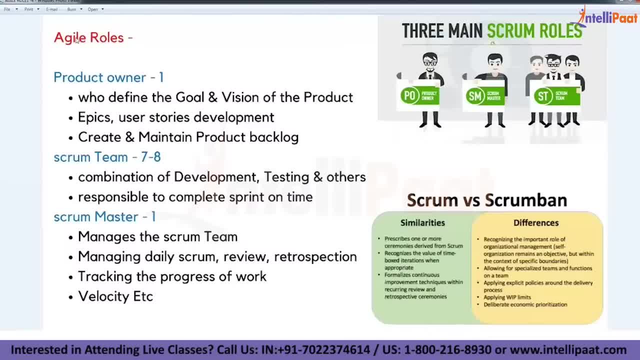 the traditional environment, traditional project development can adjust to the framework and all everything in an easiest manner comparing to the other ones. the reason why most of the people tend to work scrum due to one reason: the reason of imparting agile, scrum under agile, and all everything is due to one. 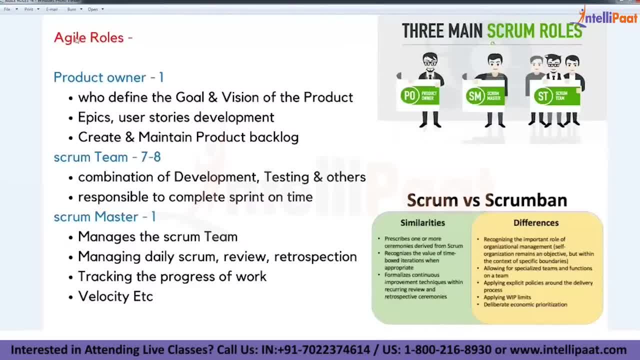 reason is this: at the same time, flexibility of development and whatever the works we are doing, and all everything will be in a formula, and it will be in a formula, and it will be in a formula, and it will be in a user stories. right, this is what general user story stands for. user story- nothing. 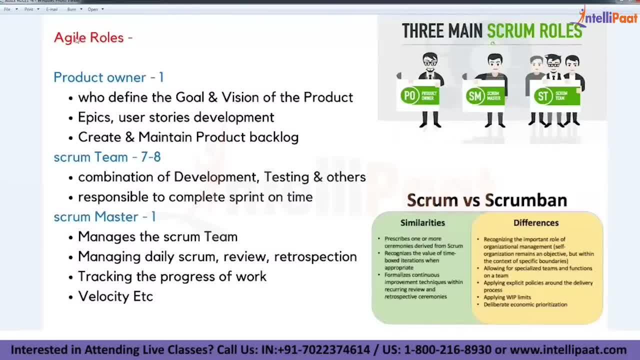 but a short description of requirement. this is what generally, user story is all about, so that user story development- everything can be done. agile environment, especially in scrum framework, which is easy for a team members to understand the process well in advance. that's a reason why most of the people go for. 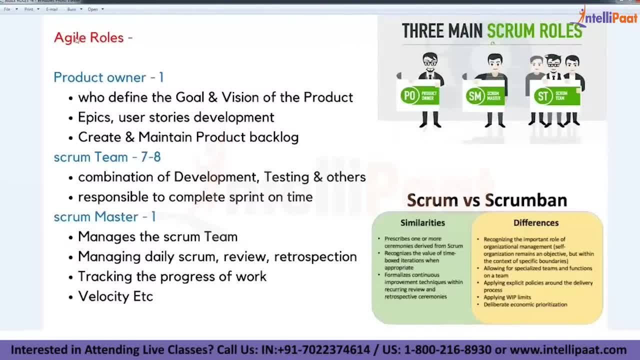 scrum due to that reason. but in that scrum, whatever the roles I have mentioned so far, we call it a scrum as it was, but majorly towards scrum, because if you see an XP and canbed- because this also have explained you earlier- because if you can see three major ones in agile, one is scrum. second, 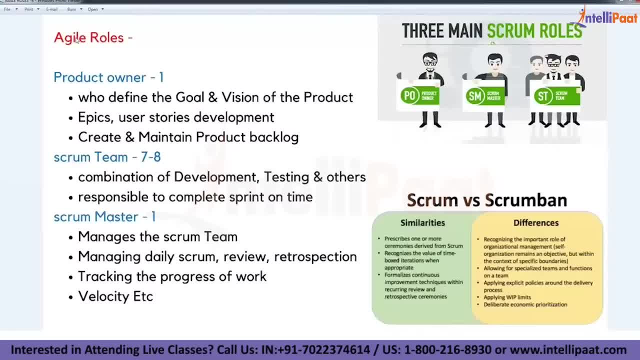 is a XP. third is canbed. so I gel is a prominent one. these roles you can see, but in reference to the roles when we are comparing along among with scrum, XP doesn't have any rule specific, like you don't see any kind of product on our. 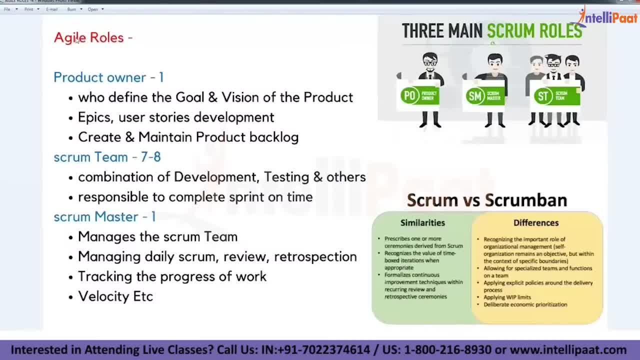 scrum team's cremasse- all that. there will be a development team as a whole so that development team responsibilities will be concerned by the thinking team. there is a development team as a whole so that development team responsibility possibility is to complete the whole thing right from the requirements, understanding and completing. 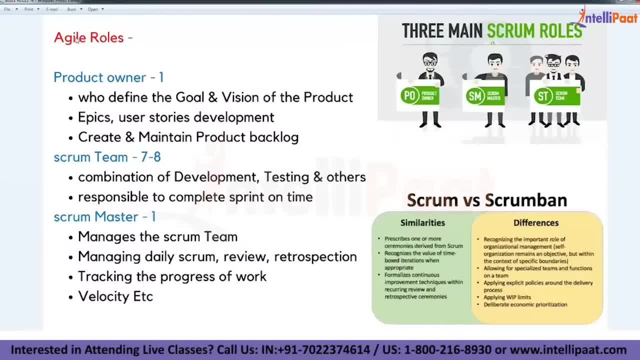 the works and all everything is completely towards the development team itself. but apart from that, of course, they are using different, different software development methodology, something like peer programming, tdd, all that stuff. that's a different story. at the same time we have another process called canberra methodology. even in canberra methodology you don't see these kind. 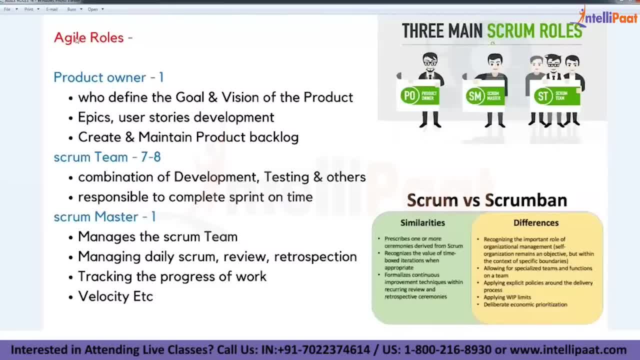 of roles, whatever roles we can see, and all everything won't be there in canberra. so again, kanban has a development. development team will be there, so the team itself will be looking after all the things. here we are writing down the user story, but there you don't write any user story, or? 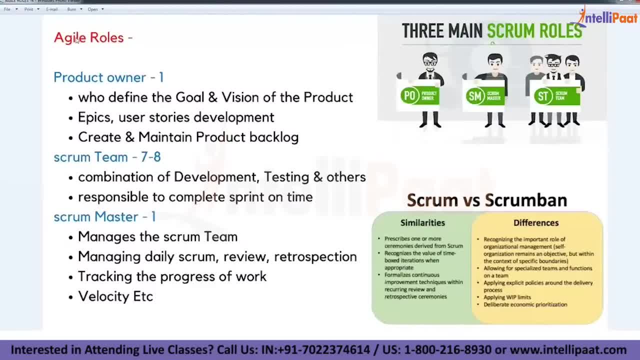 something of that sort: directly task will be taken and it will be implemented accordingly. of course, every framework and process has its own pros and cons anyway, that you know well. so, whatever the roles we have discussed is, product owner is the first role. who defines the goal and vision of the? 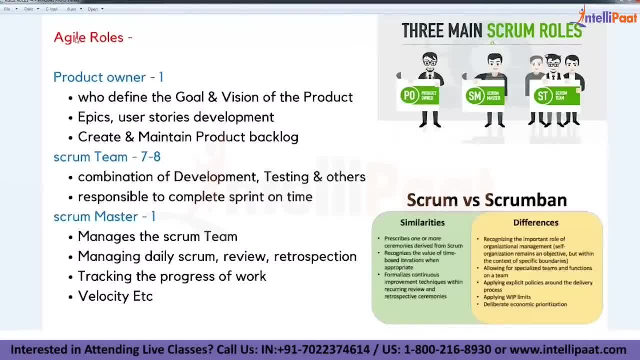 product, writing down the epics, user stories, maintaining product backlog- all that. next, we call it as scrum team members. it's a combination of developers, testers, user interface designers. it's a cross-functional team. i can say scrum team is all about a cross-functional team where people must have multiple skills, because if you are a 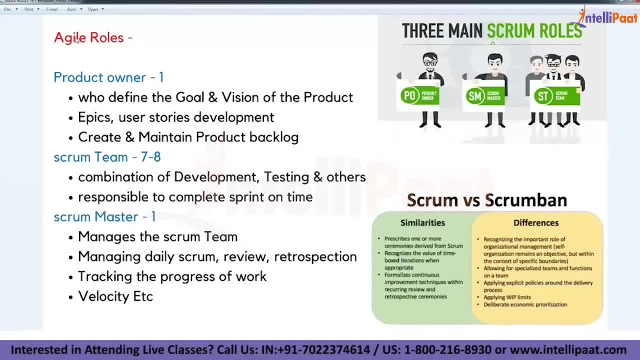 developer. you cannot confine your responsibility only for development. you must be capable enough to handle other activities also when it is needed. so cross-functional teams and multitasking is more required in scrum team. so whatever the development of implementation and reference to the project itself is, comes and everything will be. 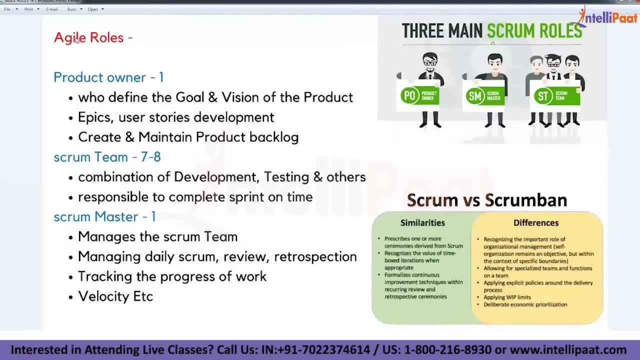 looking after by the scrum team itself, followed by this, the third role, as i mentioned about scrum master, more or less something like managing the team, right tailing whatever the task team is doing and all that managing that task, followed by this: whatever the review, how much work they have. 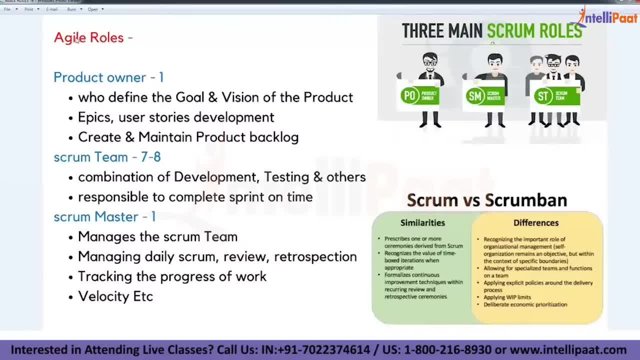 completed so far? what is the balance of work? so, whether are these people were capable enough to complete it or not? if there is any kind of doubt instance, what are the other strategies to be used, to be implemented, to make, to implement in real environment, to make it complete within the 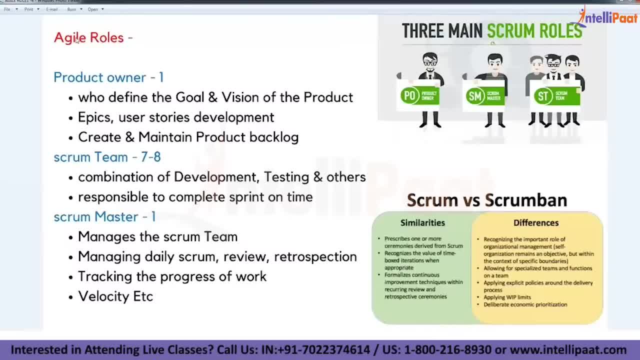 specific release. so for that, how to track the progress of the work velocity, all that will be looking after by the scrum master. so these are the three different roles will be there in agile in reference to the scrum frame. now, apart from this scrum framework and all, let me explain you there. 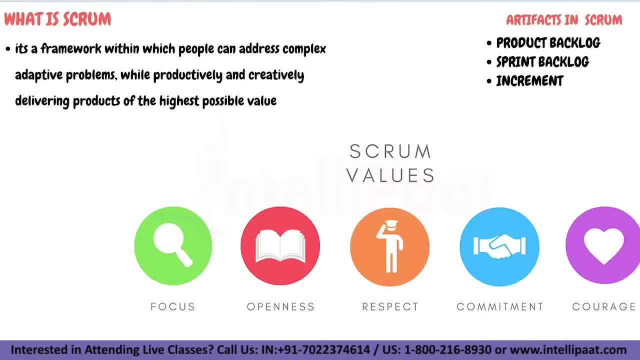 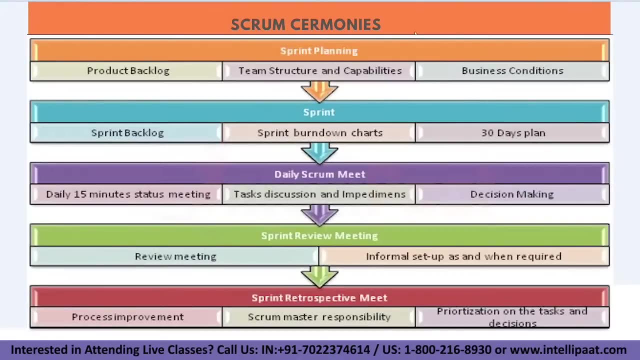 are things like something like scrum ceremonies, because whatever the implementation of work we do, especially in reference to the scrum and all will be of majorly of two few different things. one is about scrum ceremonies. second is we call it as scrum artifacts, all that stuff. so there are two things we need to discuss under agile scrum. 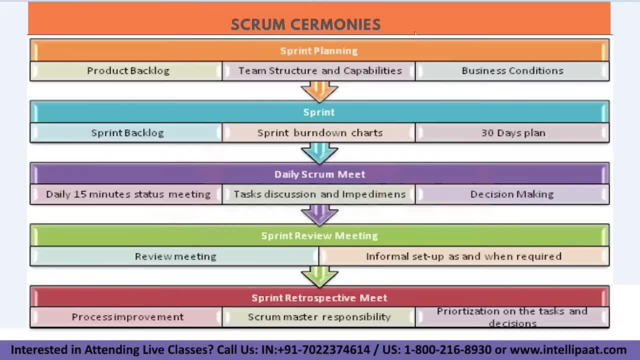 one is scrum ceremonies. second is artifacts. so scrum ceremonies means how project is implemented or how product is implementing in scrum will explains about these scrum ceremonies and all these are the standard procedures which normally we follow when we are following a practice of scrum. 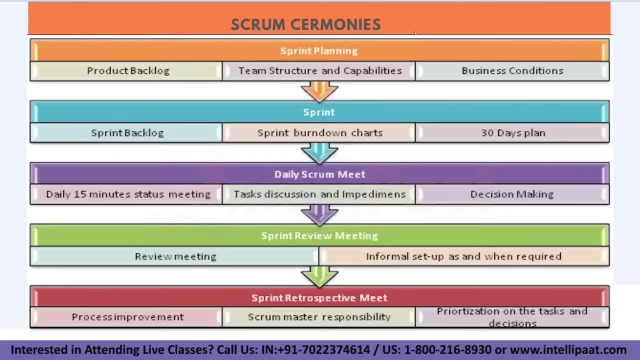 so we will start with sprint planning. this is the first scrum ceremony, so, followed by this, we do daily scrum meetings. sprint planning means where we do the detailed planning of sprint all that. so of course that will be explained in next slide. whenever i am explaining about agile planning process, you will be knowing about the detailed 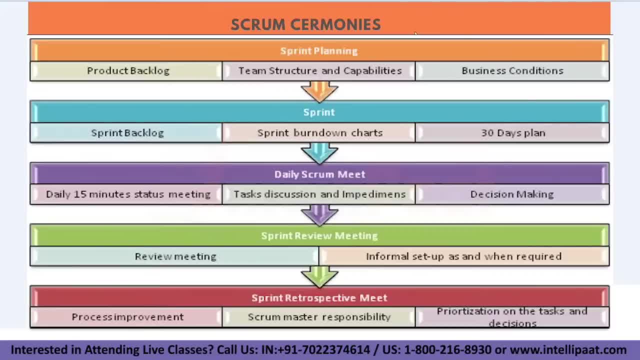 part of this. so the first is sprint planning, where we do the whatever the splint be in order to develop and all everything will be planned. so, followed by this daily scrum meeting- we call it as daily scrum meeting. nothing, but especially in agile, if you see, in the traditional model, the 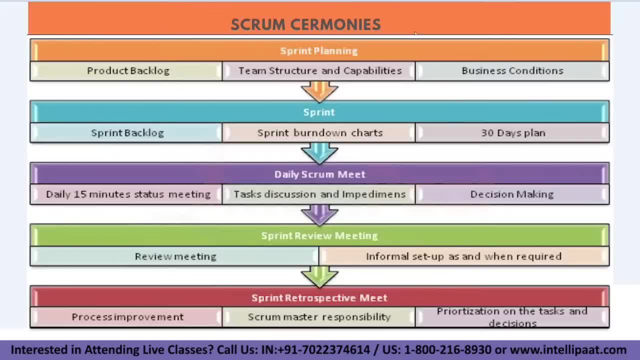 interaction with the team members is happens. this is about, uh, sometime between 15 minutes every day. normally we discuss like. this is what generally we call it as daily scrum meetings or scrum meetings. different different ways people will pronounce that normally we conduct meetings, so the advantage. 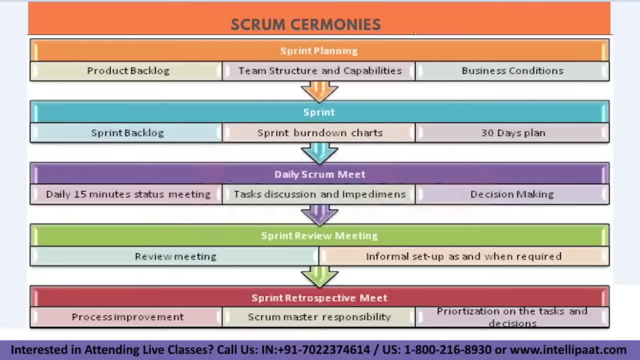 of meeting is to interact with the team members who are involving in the project, so that it will be easy for us to interact with the people and we will be knowing about what are their inputs and what is the task to be done, to be today itself, if there is any kind of challenges they are facing. 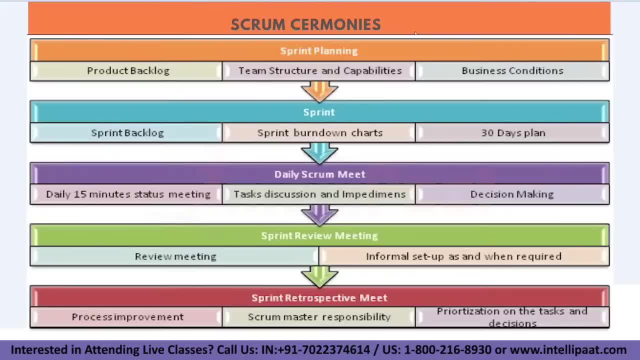 and all how to overcome those challenges. all these things comes under daily scrum meetings. all that. this is the second segment. the third: we call it a sprint review meeting. review meeting means whatever the review process and all happens here, followed by retrospection, all that. so these 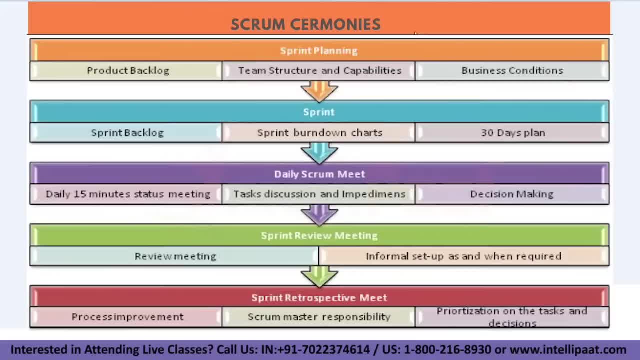 are the major scrum ceremonies which normally we follow. if we are following a practice of scrum in reference to the product development, we are working on a giant environment. apart from the vision creation, product vision, all that stuff- these scrum ceremonies has to be followed by the team. 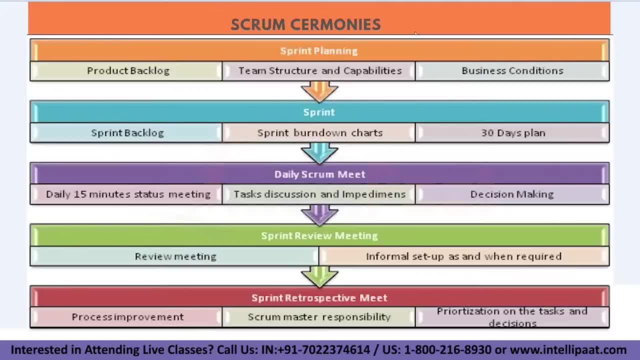 members for sure. so the team members- and reference to the scrum team member as well as scrum masters- majorly these are the two different roles- will be played, an important one, of course. product owner will also be employed, will be also be involved, but in the level of sprint planning initially. 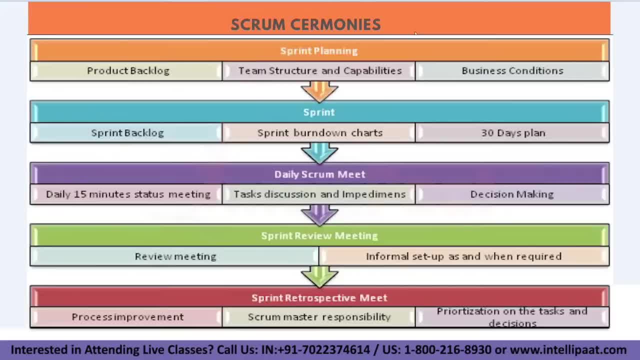 not in the level of daily scrum meetings, review and retrospection because, as i mentioned, product owner is the person always try to see in what way we have to satisfy the customer and all. so review is review meetings and all everything. product will be involved, followed by retrospection. all that stuff not majorly into retrospection, but 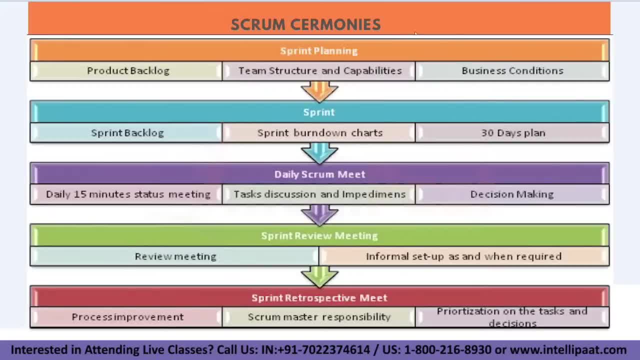 review meeting: yes, review meeting, product owner will be allowed, attended, but major role will be played somewhere in the spring planning because whatever the products, backlog items do we have and all everything will be planned there itself. so these are the different, different scrum ceremonies which normally we follow in reference to the scrum itself. so, apart from the scrum ceremonies, 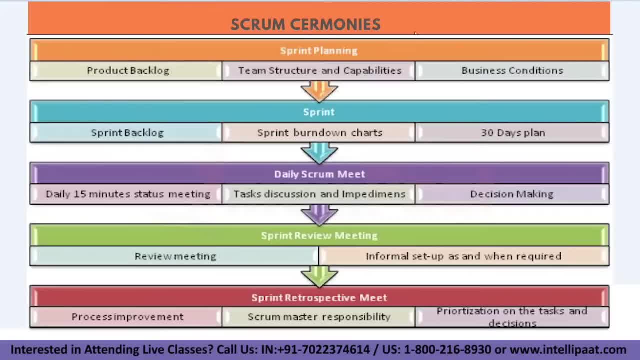 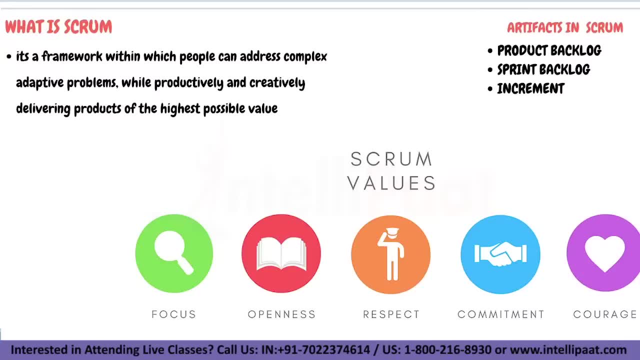 there are some scrum artifacts, we call it from. artifacts means whenever we are implementing scrum, there are some artifacts we follow because if you want to implement something in sprint planning, what is that you want to implement? for what reason you are implementing, what items are we taking? and all everything comes under the product backlog. this is the first and foremost. 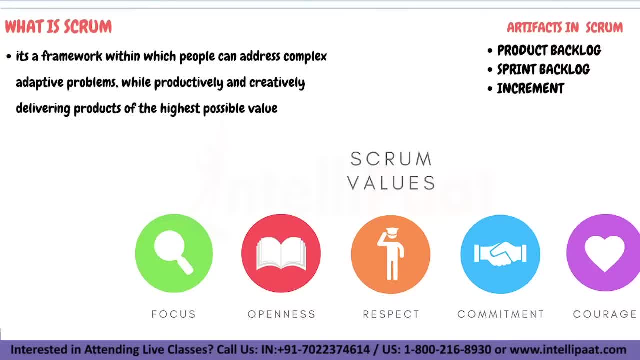 thing we normally follow. so product backlog is one thing. from product backlog we have sprint backlog as well as the sprint increments. product backlog, increments, refinement process and all everything are the three things. so these are the three different things will be there in scrum artifacts. we are implementing up the products and all everything in agile, not only the value system. 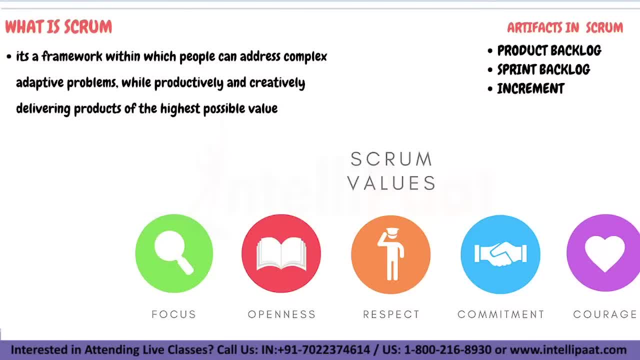 of agile values, principles, all that what we have discussed so far. along with that, one must be knowing about the artifacts of scrum, followed by the scrum ceremonies. all that right. so this is one report, the overall view about the scrum. so why scrum are we using? for what reason? 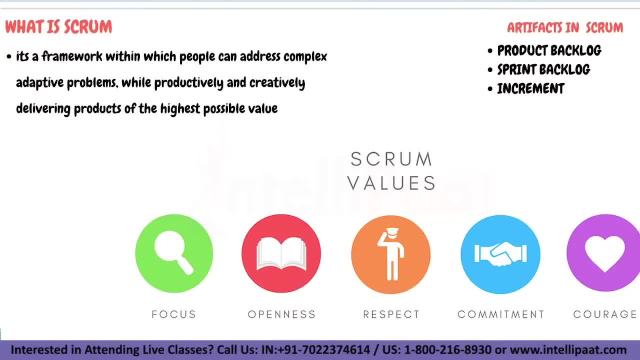 and what is the value system scrum is having. so what focus? we are focusing more on all these things that comes under the scrum part. so now, today i'm going to explain the scrum pattern about the planning process, because how different agile planning will be in reference to that. 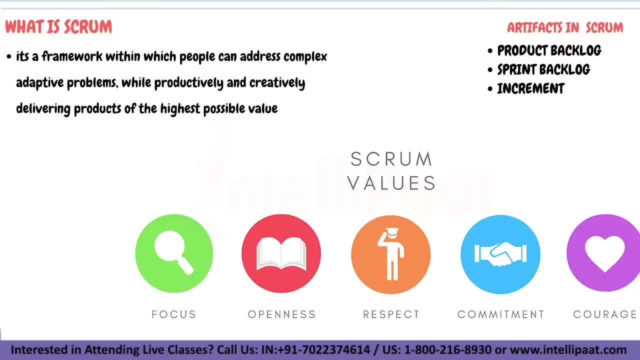 comparison to the traditional model. because in the traditional model- you know, if you remember, when i explained about the sdlc process in the beginning, i hope you might have understood- like analysis, planning, design, implementation, testing, right, this is how generally the process happens. that's what generally the structure we follow in traditional efforts. but whereas when it comes to 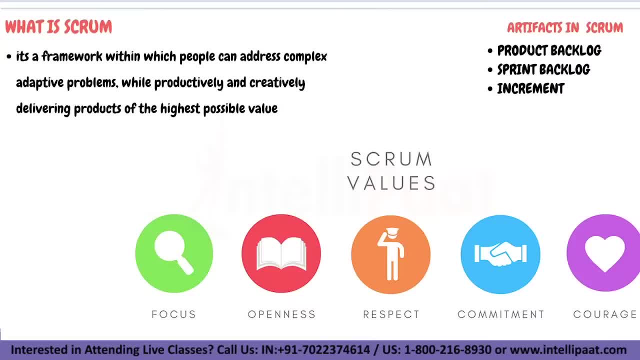 the agile approach itself is concerned, it is something different. it's not something based on traditional approach. what we follow, it is not something of that sort, because the traditional way of approach is completely different to agile. because agile majorly focusing on the release part, because if you take a project, let's say, for example, you are developing and core banking- 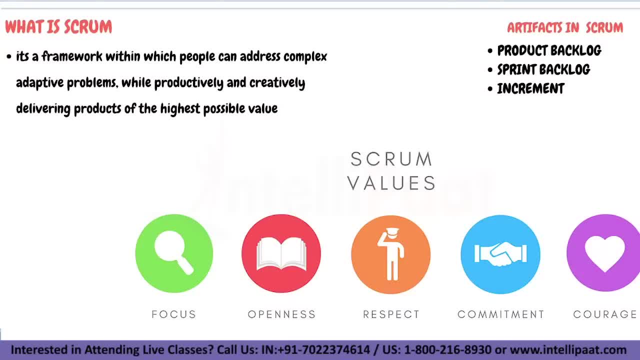 application for one of your customers. you are not developing all the application at a time. so what is that you are doing? you are breaking down into releases, right release one, two, three, four, so on. so, based upon the release planning, what we have made so far, implementation will be taken place. 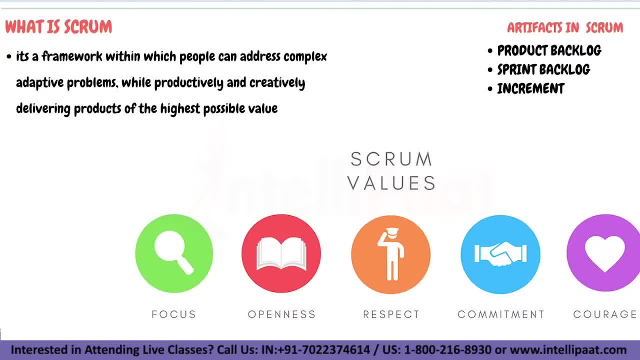 so the release planning, especially if you see traditional to agile, when you are comparing traditional to agile, the major difference you can see is about release part means release planning will be made so based upon the release planning and all implementation will be taken place. this is what generally so there is a difference, you see, from traditional to agile, for very clear. 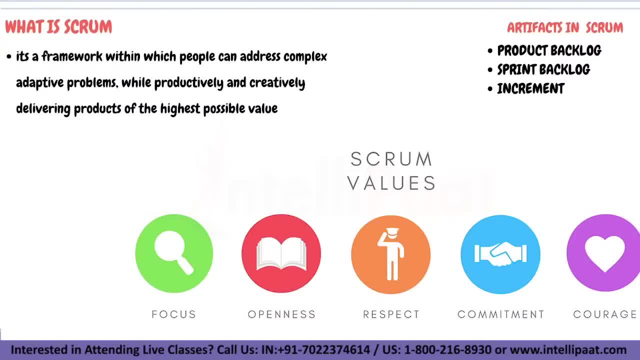 because that's the reason why adoption and adopting towards agile planning process could be difficult for members to understand, because the transformation itself is a difficult and challenging task for many of the people. so, due to multiple reasons, due to might be they may not have towards exposure towards the agile. 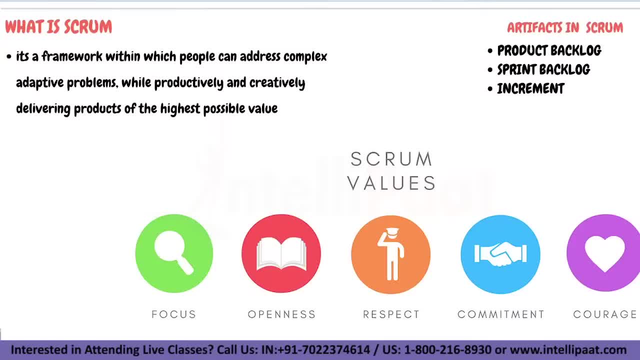 environment earlier might be reason they may not be ready to face the challenges within the stipulated time to complete. reasons might be in different, but of course, whatever the reasons, it could be. so one end of the day, people have to understand the process of agile environment well. 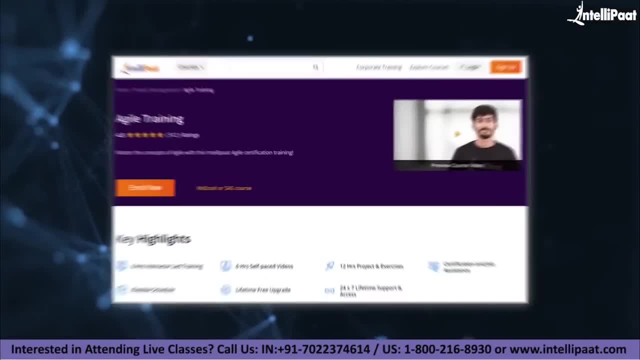 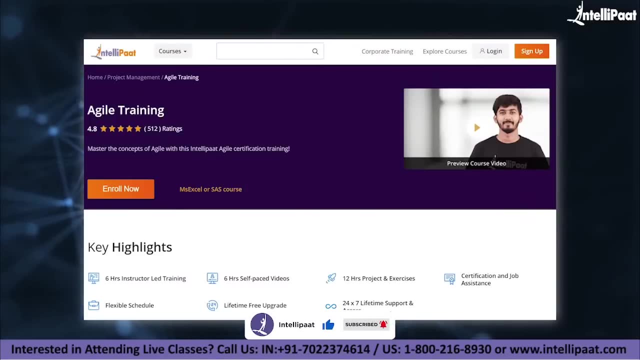 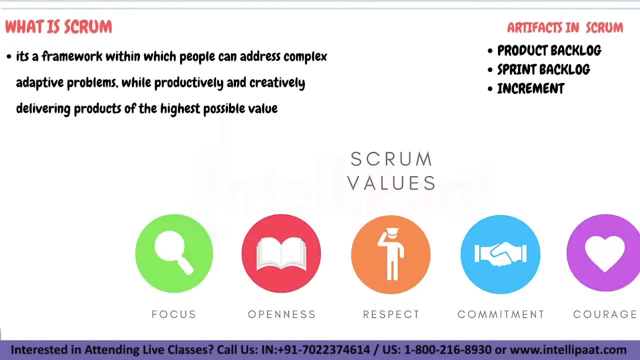 in advance before they want to implement. just a quick info, guys: intellipaat provides agile trading mentored by industry experts, which is given in the description below. now let's continue with the session. so if anybody wants to move towards the agile environment, so they must be knowing about the planning process of agile first. 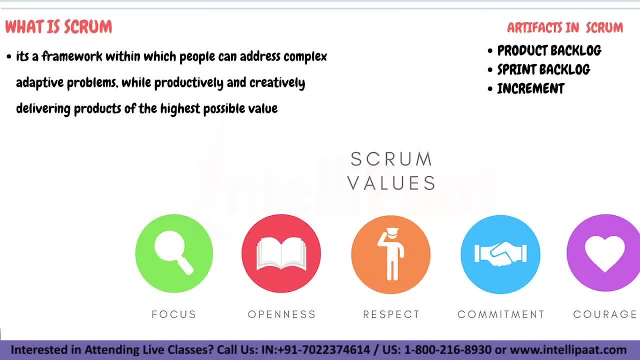 so what are the steps means? whatever the sprint planning, review, retrospection, whatever i have told so far, along with this product backlog, right. so whatever the head terms we have discussed, even in the last week, in this week as well, till now. so everything will be a part of the agile planning. 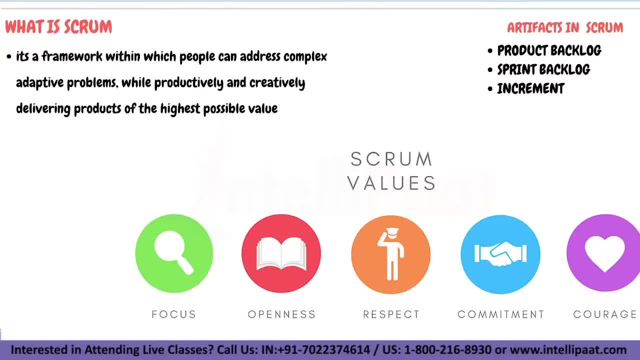 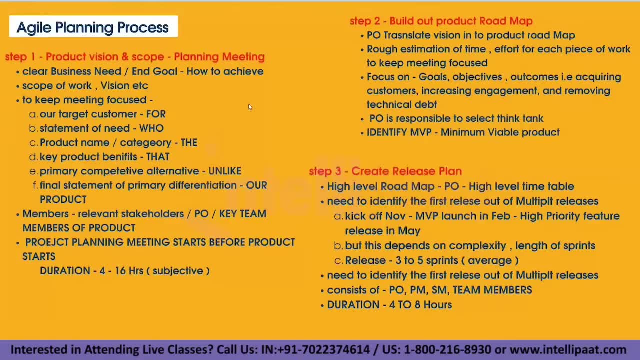 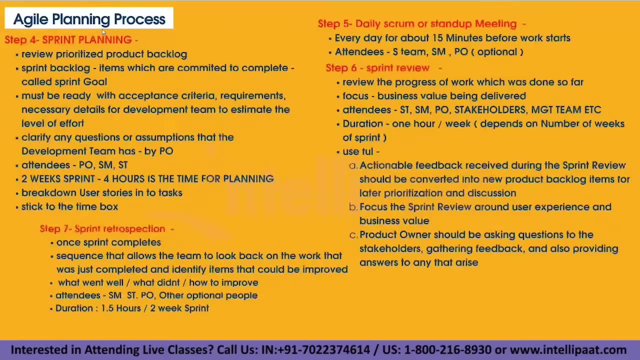 process, which will be as different, different steps. the steps of agile planning process will be as follows. this is what generally agile planning process. let me explain you an overall view. so this agile planning process completely into seven different steps, total seven steps will be there in agile planning process means if you are implementing a product to the product product. 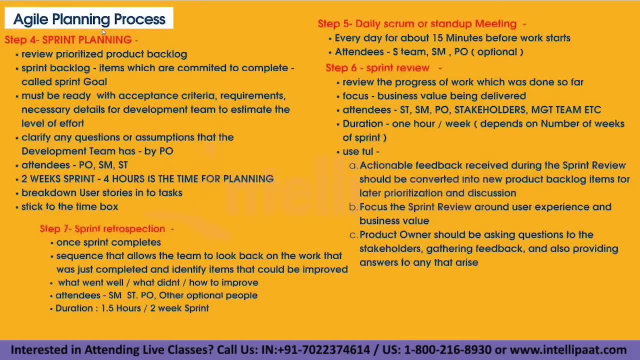 in the any, any kind of- uh, you're developing any kind of product for customer requirements, all that stuff. the agile planning process will be divided into seven different steps. so this is for me- you make it to- to understand much better. so i have just divided into seven different steps so that you guys can understand well in advance. 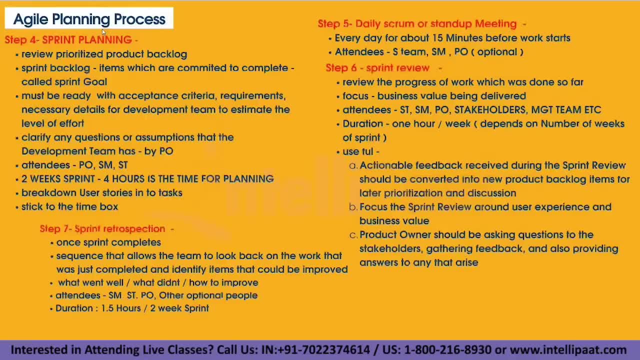 the first, we call it as product vision and scope. second is about building out their product roadmap, followed by this release planning, which is essentially important, as i mentioned earlier. at the same time, sprint planning, daily stand-up meetings, review and retrospection. so these are the seven different steps you can see in agile planning process. now let us understand. 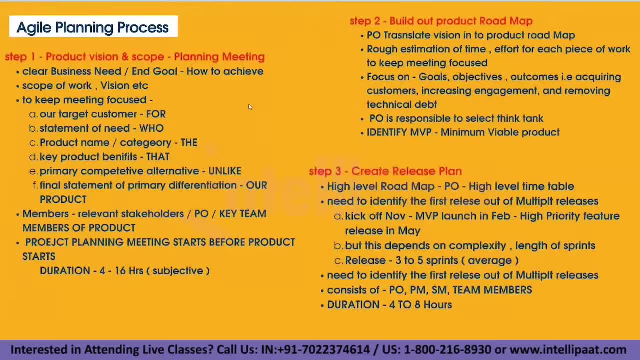 how it is different from the traditional one page, because in traditional one, as you know, will be in phase where we call it as analysis phase. analysis phase means where we are trying to understand the business problem from the customer. right, so we need to understand the existing process. what was their existing process? right so we need to study about what is their. 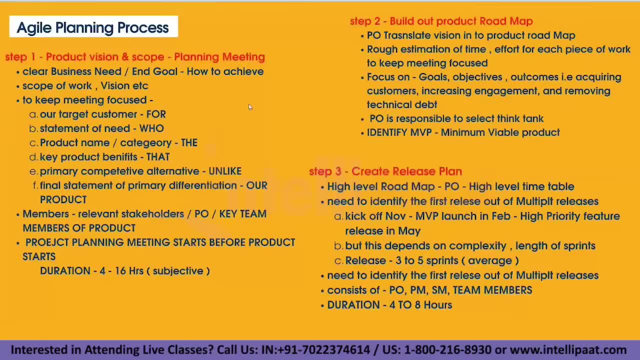 proposed system solution. they are expecting all that. normally, being a traditional team, we study, but here, when it comes to the agile planning process, there are two different things we need to understand. so one is about the team who are involving in implementation of the project product at the same time. even you can see from the customer end also. this is where generally these 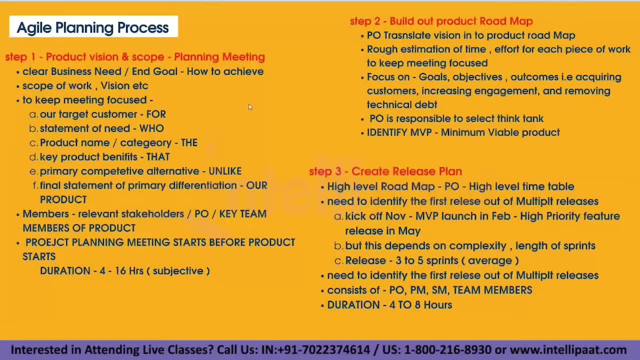 product owners. all these people will be involved. now, the very first step, especially in agile planning process. when we want to implement an application or a product in an agile planning process, the very first thing is that we need to have a clear understanding about the product vision and as the scope. this is essentially important for any of the product to start with. 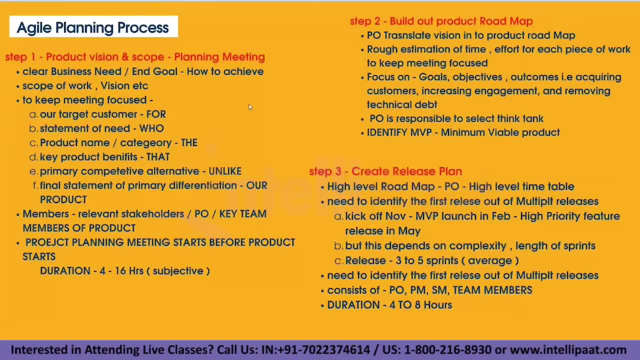 why? because creation of product backlog in addition to the product backlog creates a lot of issues. so creating the product roadmap for any of the project is different, essentially important if you want to create a roadmap followed by the product backlog. and all a team means customer. i'm 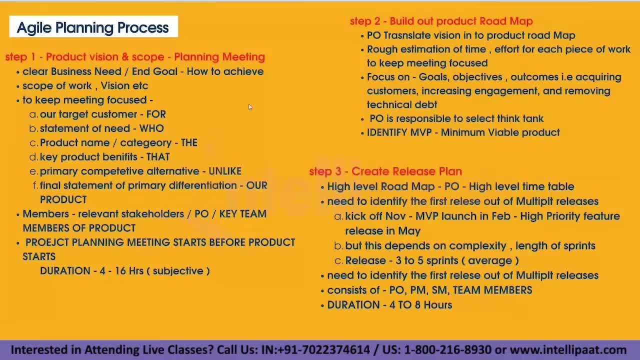 saying from the stakeholders in the point of view they must be having a clear understanding about the kind of vision and the scope what they want to achieve so far, because if they are missing in clarity and understanding about the vision and scope what they wants to achieve in the future, 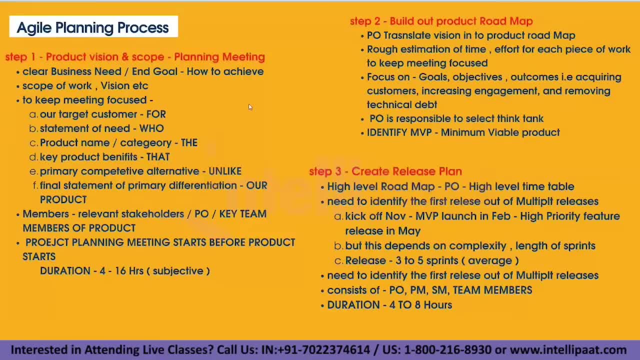 right. so whatever the requirements and whatever the expectation they are expecting from the agile part and all, everything will become a failure, obviously because you don't see any kind of connect between these two, because product owner- not only a product owner about to that, stakeholders itself are in a state of confusion where they don't have a clear understanding about. 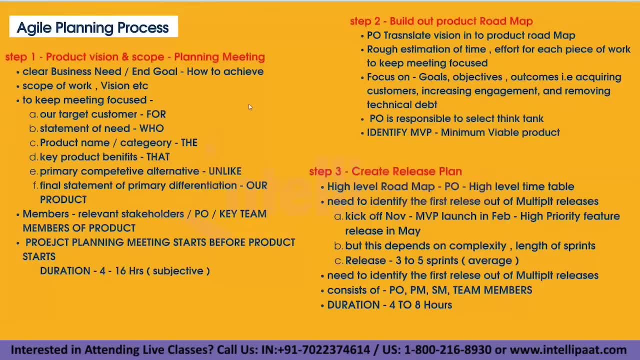 the vision and scope. hence, obviously, the product will become a failure here. that's the reason why the very first step we need to understand about this is to create, and as well as to understand, the product vision and scope of the product. this is where, generally, the planning. 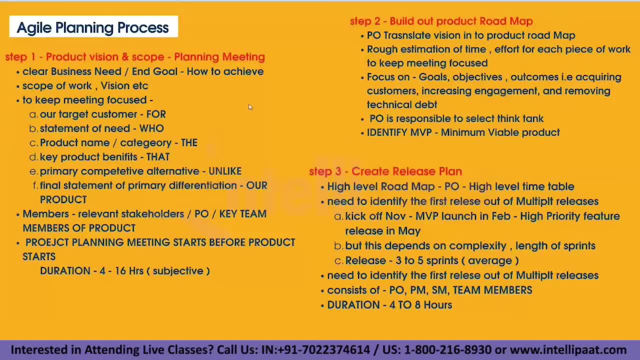 meeting will be conducted in this planning meeting. there are few points we need to discuss. first of all, we need to understand the need and goal of the product to be achieved. so whenever we need to understand about the need and goal of the product, we have to understand about few. 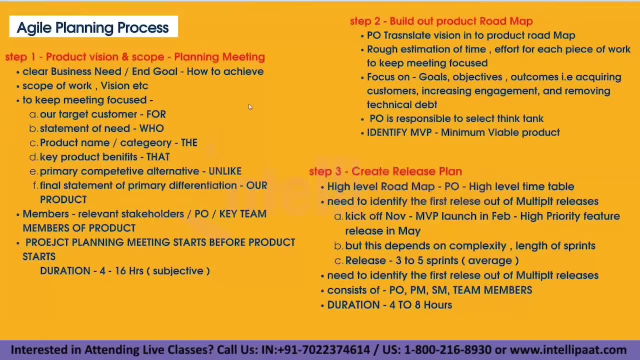 different things. the first point, in reference in reference to the first point, i'm explaining this here. so the first point- we call it as clearly about the business need, all that right. so first point is this: yeah, first point is about clear business need and goal and how to achieve it. now, if you are a stakeholder, if you are the 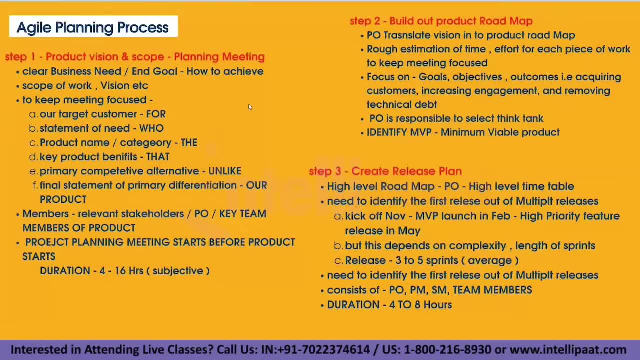 customer wherein you want someone to provide solutions for your business problem. the very first thing, you need to have a clear understanding about the business need, followed the followed by the end goal. so, when you are trying to understand about the business need as well as the end goal, 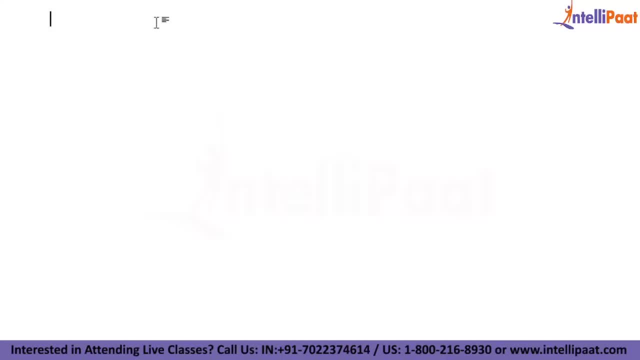 this may be for two different things, for example, as an example, i'm just taking here, for example: first point: customer type one. i can say i can write it as type type one because this business need, as well as the scope, goal and all everything will be for based upon the two different types. 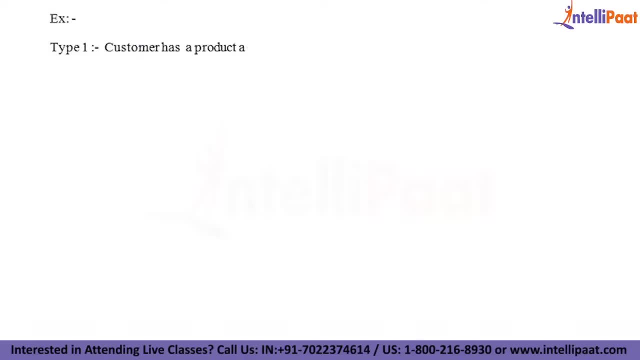 first is customer as a product and expecting someone to enhance it. this is the first point. means type 1: customer has a product. at the same time, customer is expecting someone to enhance it. means here there is an existing application which was there for the customer for a very long time. customer is using an application. 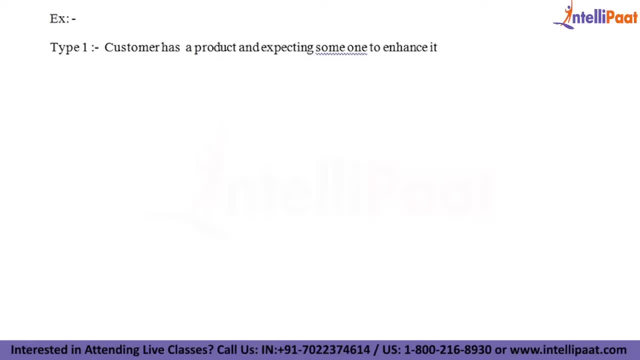 for very long. let's say there is a core banking application which customer is using for very long. so now, due to the business process changes, whatever happens, customer wants to upgrade this application to the next level. assume that roughly and say so. what is that we want? first, 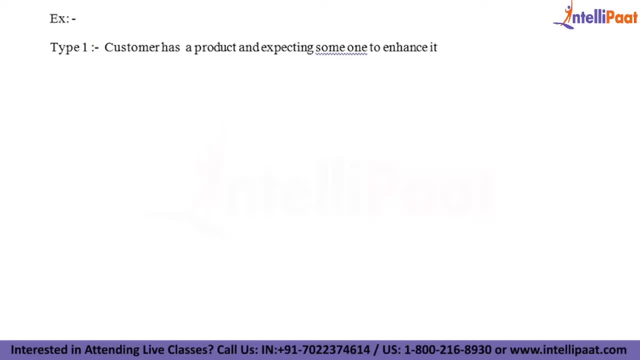 of all, you need to know about what customer wants to enhance and for what reason. customer has a product and expecting someone to enhance it to that- instead enhance it to the next level- it means it means they are expecting some features to add, right? this is the first type of thing, right? 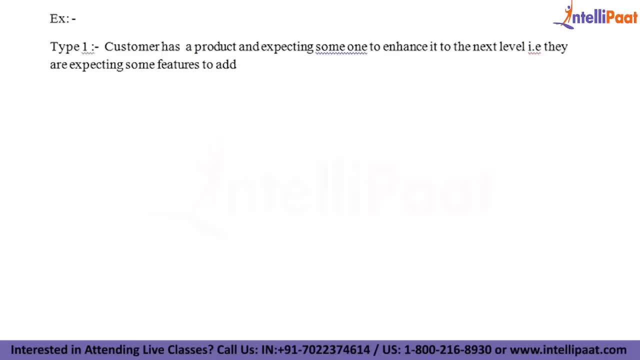 now the goal will be different. that's the reason i have told you because, when it comes to the goals, there will be a two different goals. one is about the business goal, second is a project goal. right, so, two different things we need to understand, because most of the people will have a confusion. 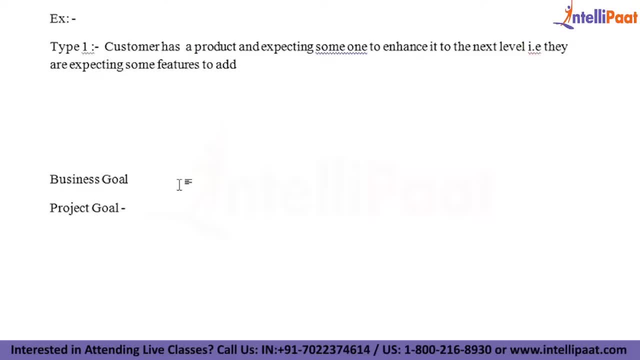 here. so one is business goal, second is a project goal. business goal is what client having right? so this is what generally business goal means. what they want to achieve in their business is what generally the business goal is. so, towards the business goal, if they want to invest some kind of money, to be invested to have some solution and all, obviously they'll be. 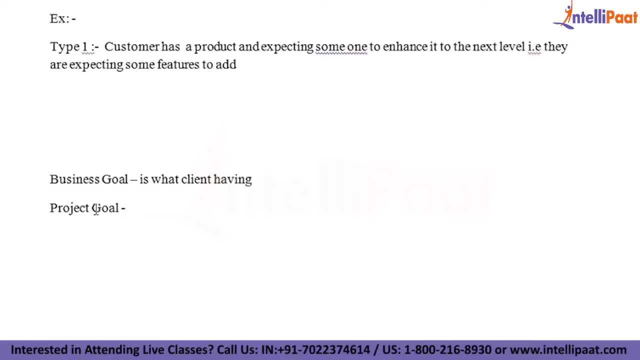 investing on the product. whatever the project or a product goal, whatever it is, this product goal must be understood and defined by the team who are implementing and all they should understand. so there must be a proper alignment, as well as the connectivity between the kind of business goal, what customer wants to achieve in connection to the product, what we are going to. 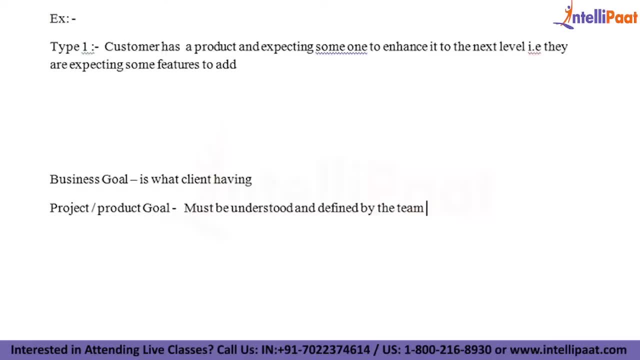 develop. if you don't have any connection between these two, obviously it leads to a failure of the. it leads to a failure of the product because customer is having a product. assume that in the first case or in the second type might be anything- customer is having some goal. 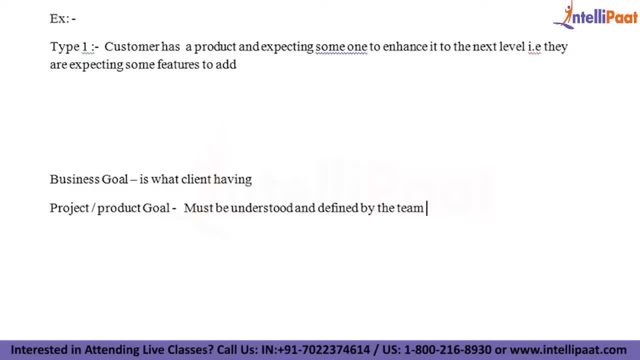 which they wants to achieve finally, right, so which? for that reason, he is investing some amount of money to develop some product for the future needs. so that must be the product goal. when someone is trying to develop the application, if those two have two different uh understandings, obviously it leads to the product failure. that's the reason. 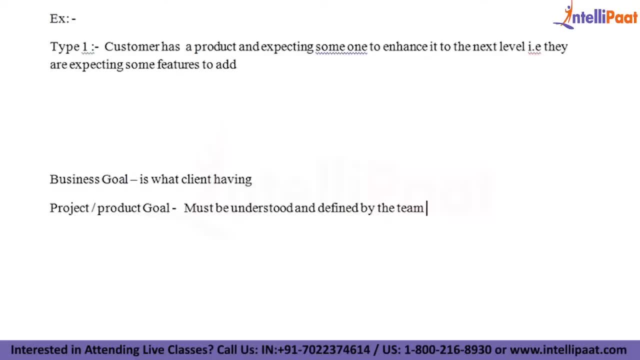 why there is a two different things. one is business goal from the customer perspective as well as the product goal from the implementation perspective. so do different things. so, being an implementation team who is trying to understand and who is trying to provide solutions for this kind of projects, products, all that stuff, they should understand the kind of business goal. 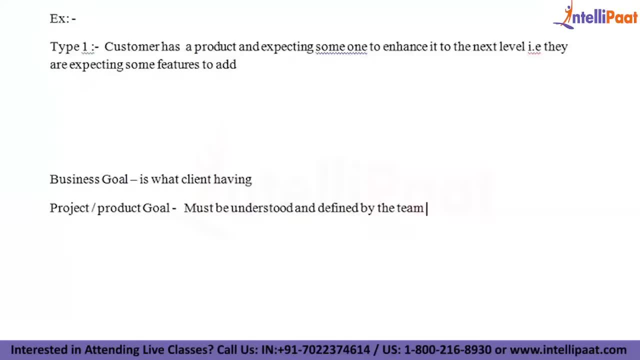 that the customer wants to achieve. finally, unless, until otherwise, developing a product and all according to the reads of the customer and all would be really difficult and challenging. so this is what the point is. so the first type is this second type to customer is expecting us to develop. 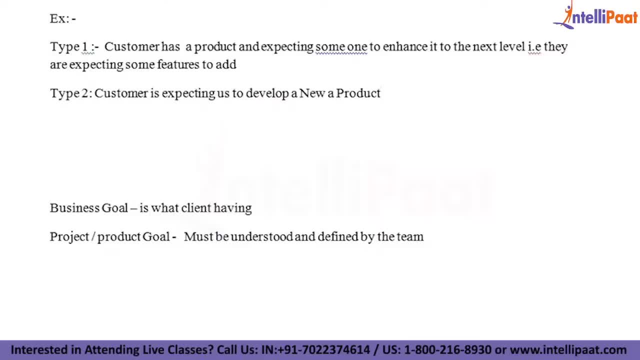 a new application. normally, this proposal we may get from the customer or we may be providing. i'll give you an example between two things. for example, there was an application called core banking being used by one of the bank for a very long time now. their business model was there, but still there. 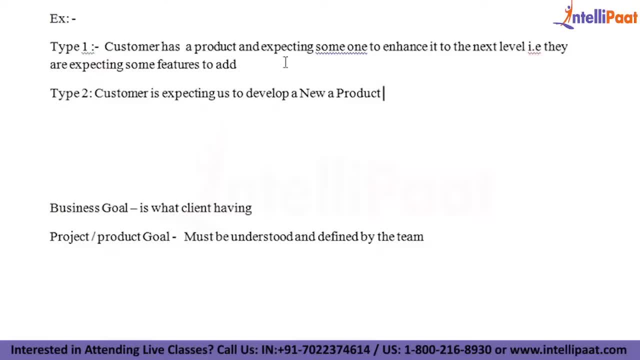 are some changes in terms of the lines of the services has added in recent times. due to that reason, they wants to add some new features and functionalities into the existing ones. whenever they wants to add some new features and functionalities, what is that they need to understand? they want someone to develop to new features and functionalities to the existing ones. 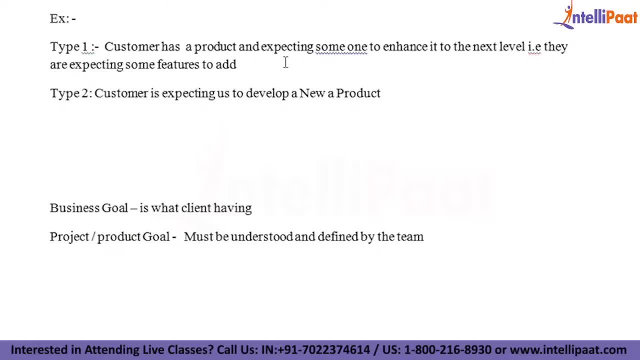 compatibility is the issue. this is where, generally, feasibility study comes into play. assume that you're all belongs to the development team. assume that i am the customer. i am expecting you to develop a core banking solution. there was an application called core banking where i'm expecting you to add some new features and functionalities. assume that now. if 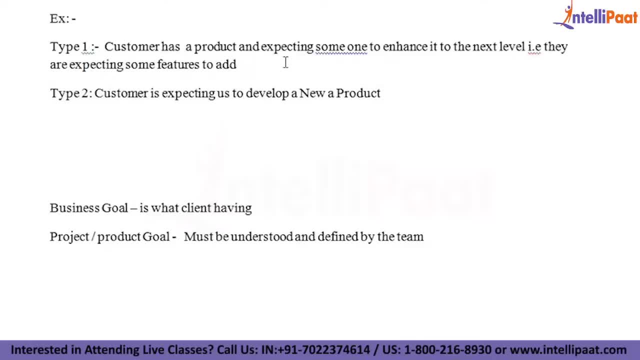 i came this, if i came with this proposal to you, you are into implementation, understand this very right. so it all belongs to the implementation team. what is the first thing you see, apart from the financials, apart from the remaining things, all that stuff? see, first of all, you tc the first. 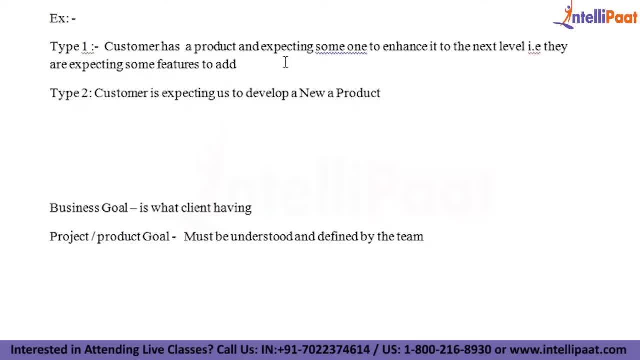 point is about the technical feasibility. financials, of course that's required, but keep your side for some time. technical feasibility is what normally you consider first. what is technical feasibility? assume that the application was developed on dotnet. i'm using this for from past 10 years now. i'm expecting you to add some new features and functionalities to. 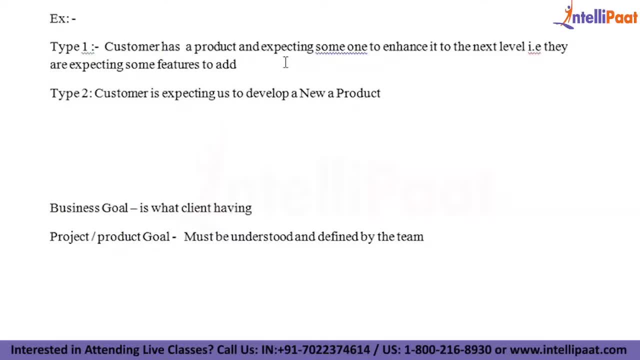 the existing one. the existing technology means either hardware or software. may or may not support new features and functionalities, because the system infrastructure was very old. may or may not support. this is point number one. so, in reference, by understanding this, what is the thing you you'll be saying? this is where generally technical feasibility comes into picture, whether 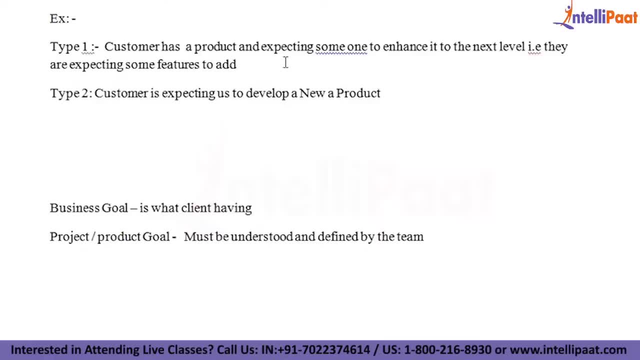 is it compatible or not? if it is not compatible, right. so what do you want to do? we have to propose to the customer that we are going to develop a new product for you as separate, because, rather than repairing the existing one, it is always easy for any team to develop a new application as fresh. 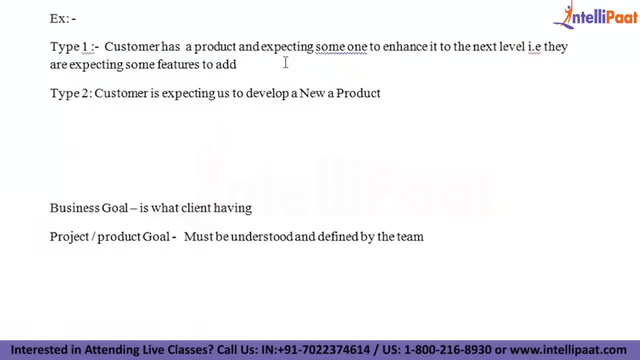 because requirements are very fresh from the beginning, so they could understand requirements well in advance so that they can develop and build the product easily, rather than understanding the architecture of the existing product, making changes out of it and all everything. normally it's a difficult and challenging task, but sometimes it happens that's a different story. 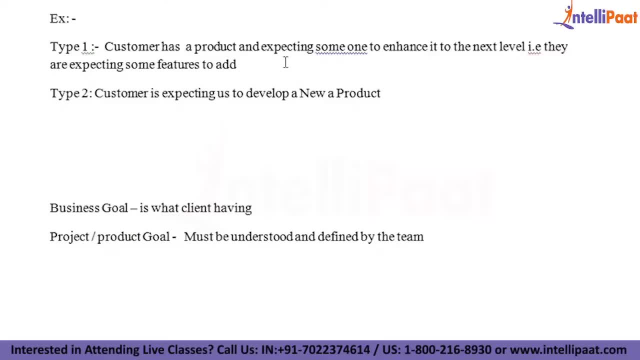 so being. you are a technical team, you are into the development team, wherein you guys are into the implementation side, where you always try to see in what way, technically, it is feasible for us to develop right. this is where, generally, feasibility study comes into picture. so if i am a customer, if i am expecting some sort of solution from you guys, what is that? first of 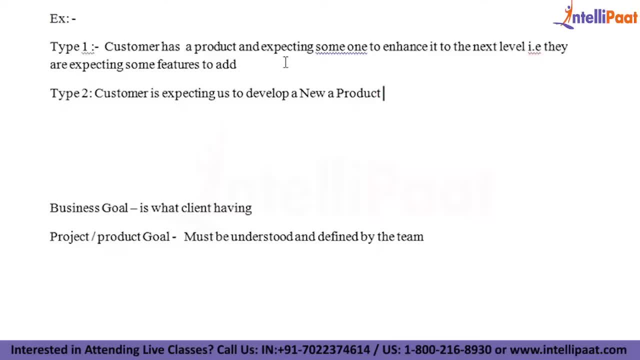 all i need to have, whether it's either- i'm expecting you to enhance the new features, i am expecting you to develop a new product test for whatever it could be. i need to have a clear understanding about the kind of business needs, followed by the goal, what i want to achieve. 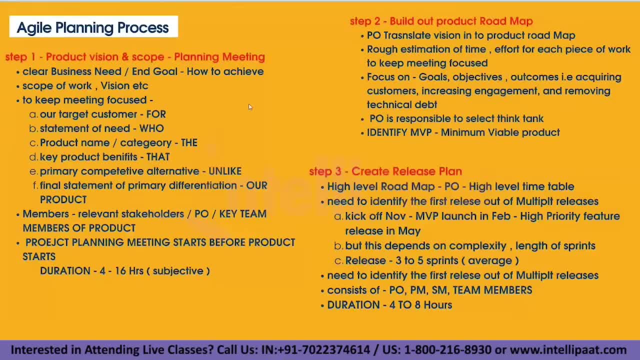 finally, this is what, first of all, i need to have a clear understanding. being a stakeholder- v i don't, don't say as individual, i can say: like we need to have a clear understanding about whether do we have clarity on this perspective or not, is what i need to know first. at the same time, i must be 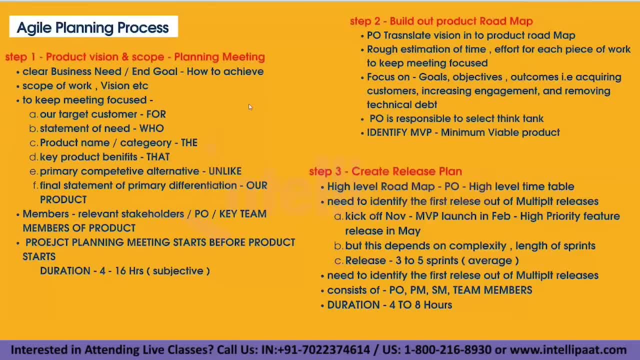 knowing about how to achieve it because, being a vm gain, expecting a solution from technical people, all that being a stakeholder or being a client, i must be knowing about how this could be achieved because, if any clarifications come across in near times in reference to the expectation of the 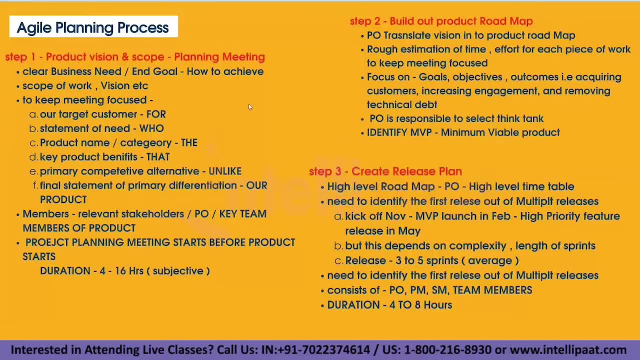 product itself is concerned, i was the first person to answer those questions. i may be an individual or a group of people, whoever they are, so we need to have a clear understanding about the need of the business. for what reason am i expecting someone to develop the product right? so business. 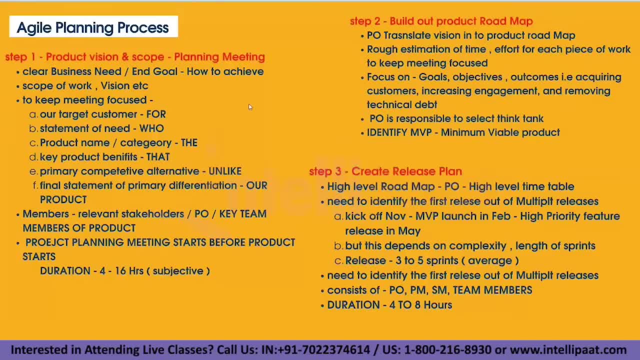 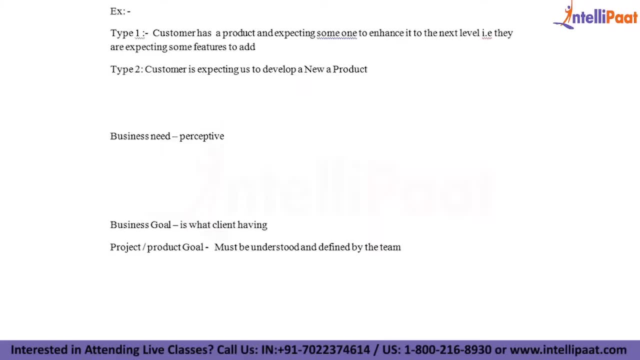 need. so when we talk about the business need, there are few things we need to understand when we talk about the business need from the perspective of perspective of the client, perspective of the client, i am saying this right. so, first point: what is the the need of me to make someone to develop a solution at this time? point number one to be 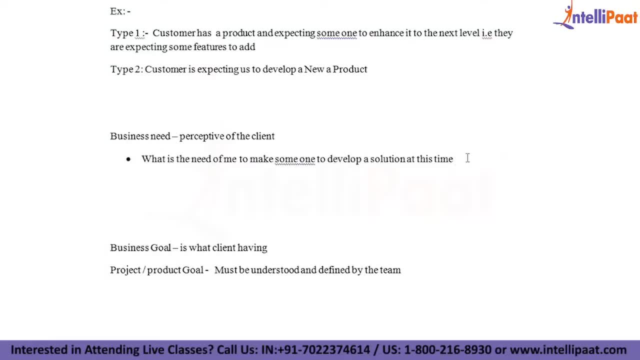 noted. so, being a stakeholder, being a client, i must be knowing about this. well, right, what is the need of me to make someone to develop the solution at this time? second point: how important for me to use this at the present condition, because i am endorsing someone to develop the product. 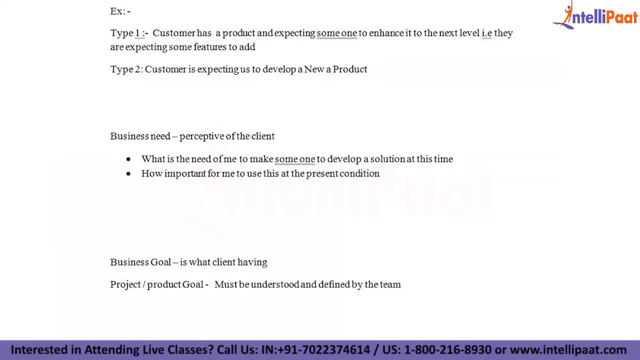 so how important for me, right? so how important for me. it's not only important how immediate, because depends on my immediate need and all everything we will be knowing, for example, if i am expecting a product to be developed as early as as possible, whatever the model they were choosing, and all. 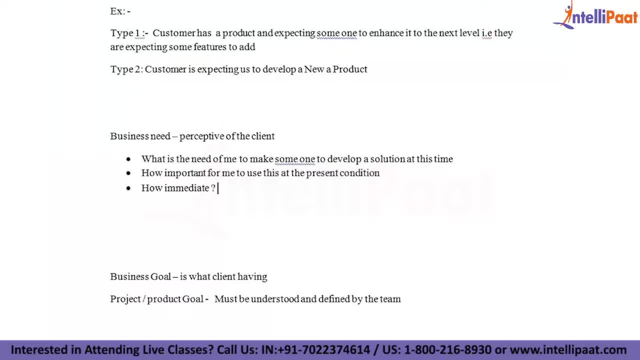 everything will be different. end of the day, we are using aj, so that is one thing. how immediate, right? so next, who are going to get benefit out of this? right means beneficiaries. right, we must be knowing about beneficiaries, etc. so when i am trying to understand about the need being a customer, being 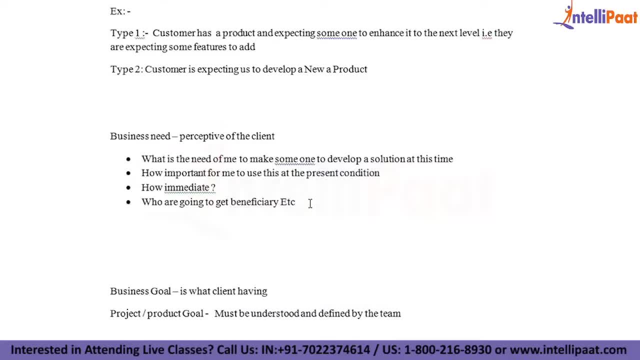 a client or being in person, who is whom expecting the product to be developed. so i must be having a clear understanding about for what reason am i developing. i am expecting someone to develop the product and how important it is to me, how immediate is it for me right, and who are going to get benefit. 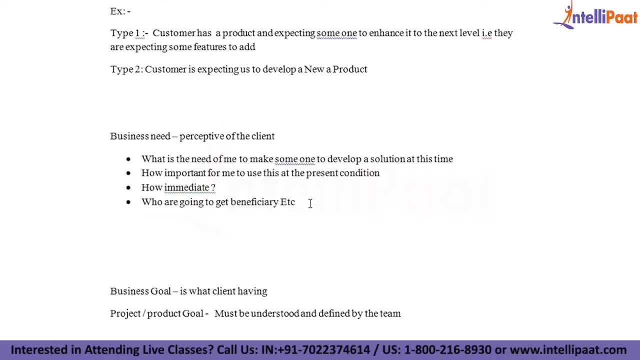 out of it. this is what generally, in business analysis terms, we call it as business case, because, again, i am comparing to me, like you are comparing. if someone is trying to develop a project for you, the traditional one, because there is a connect between traditional agile- will happen sometimes. 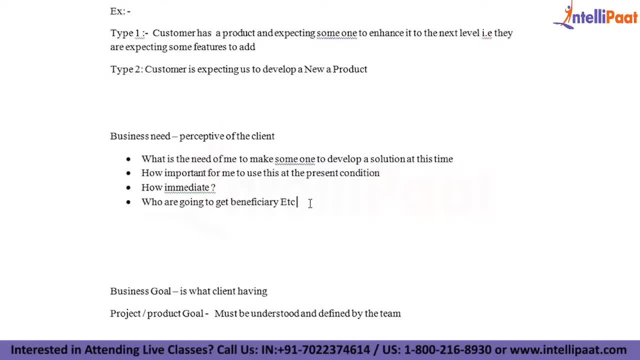 in between the reason i always i am trying to compare when it is required to the traditional one. also, this is where generally in business and other systems, we call it as business case, business case. we need to define the business case here, normally in regular models and all we call it. 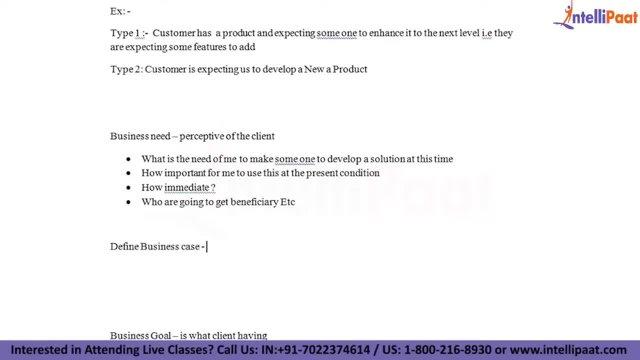 as business case, defining a business case right. so defining the business case is what generally we do, so when we want to define a business case, especially in reference to your business, because i am explaining about the business rate, so that hope it is helpful to you, so that i am explaining. 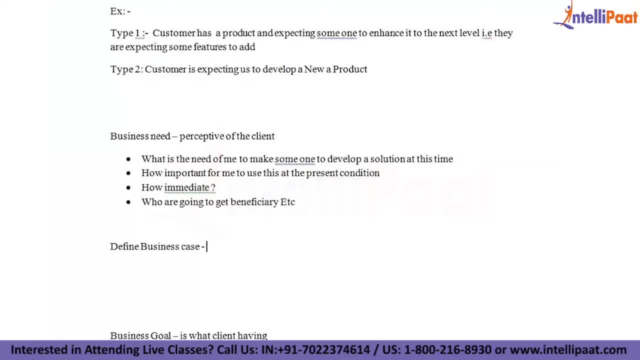 this point to you. it's not a deviation. but in addition to that, because it's a traditional way of approach we follow. whenever we follow a traditional way of approach, we need to define the business case first. so when you want to define a business case first, you need to understand. 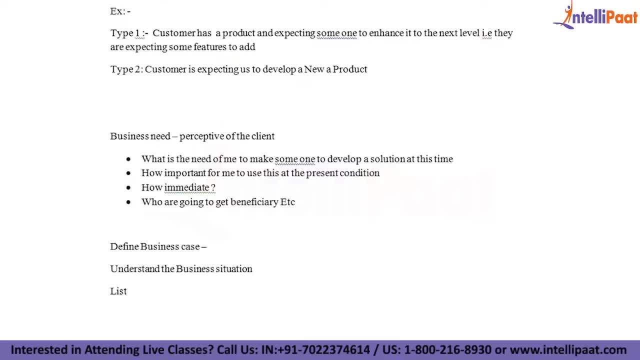 the business situation. understand the business situation. second list of problems: right next the same point. how important for us at this level, someone to develop the solution right. so this is one more thing we need to understand here now, how immediate. who are the beneficiaries? who are the beneficiaries going to benefit out of this right? what are the assumptions and dependencies? what? 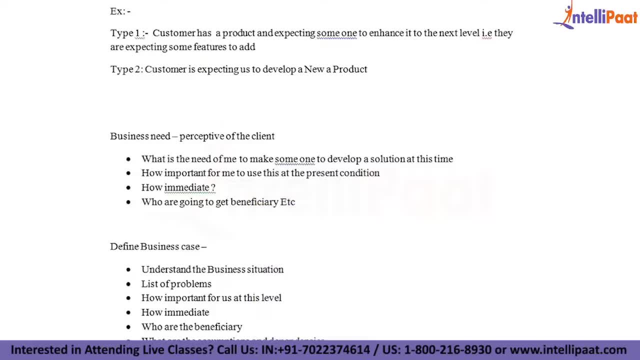 are the different, different designs, these assumptions and dependencies? we have to think from two different ones. one is from the client side, other second from the implementation team, vendor side, right. what are the assumptions, dependencies, these are all comes under the business case here. so very first thing is that when we want to understand the business need of 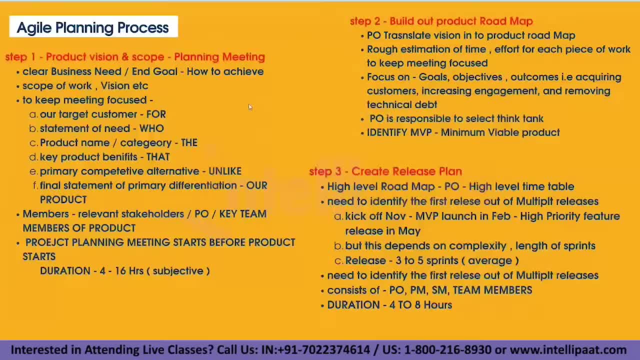 the customer. these are the points we have to focus more on. so understanding about the business need had to have how to achieve it and what is the final goal we want to achieve. there must be the goal. whatever you are going to achieve must be a business goal, obviously right. so the end goal has. 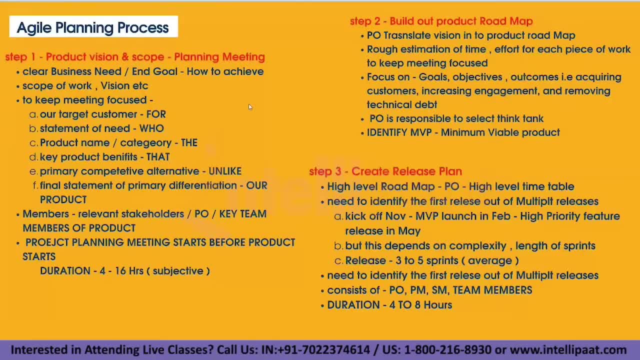 to be knowing. so that is what the first point is. the second point you need to know about the scope of work, followed by the vision. what is scope of work? scope means scope. we need to define nothing but scope, nothing but the possibility, possibilities of developing solution. is what we call it a scope? 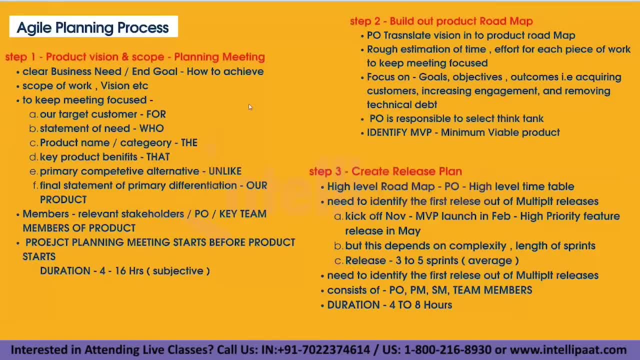 of the members. do we have that scope to develop the product or not? normally, when we talk about the scope, this scope we need to understand from two different ways. assume that i am the customer. right, i am the client, wherein you guys here all belongs to the development team. scope will be: 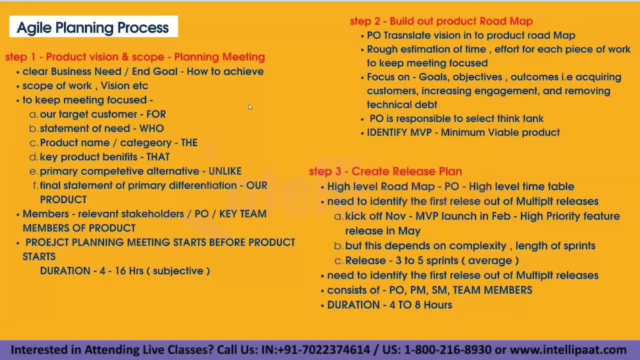 defined by me as well as by you as well, because scope means when i am giving some problem to you, to solve that, all that stuff. first of all i need to have a clear understanding about: do we have the possibility, someone to develop the product or not? so that sort of scope we need to. 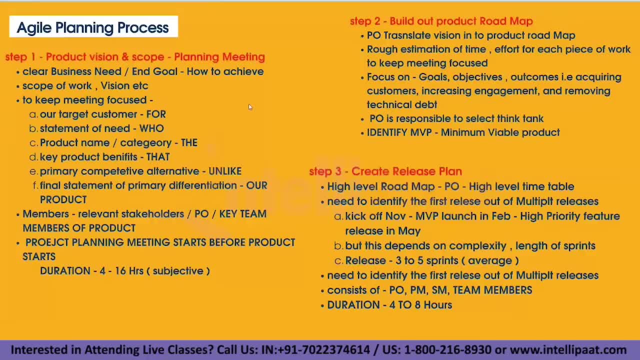 understand, because am i providing all the information to them? so do i have any kind of restrictions to provide any sort of information to them if i am not providing? if they have any kind of limitations in providing information and all that, how to go over about that? so that sort of 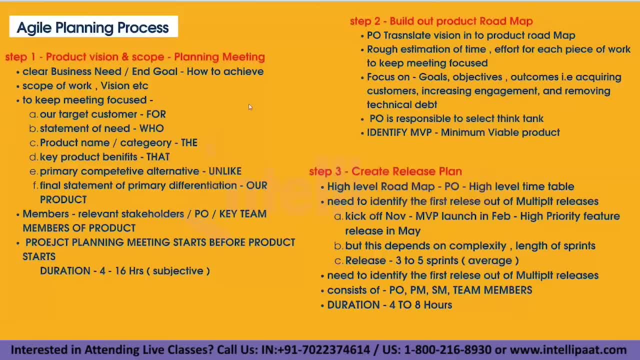 understanding, first of all, being a customer i need to have. at the same time, there are possibilities sometimes where i may be changing requirements in between, right. so these sort of understanding is all concerned the scope of the project from my perspective. so there are two perspectives, remember in case so. one is from the customer side. scope of the project from your side is different because 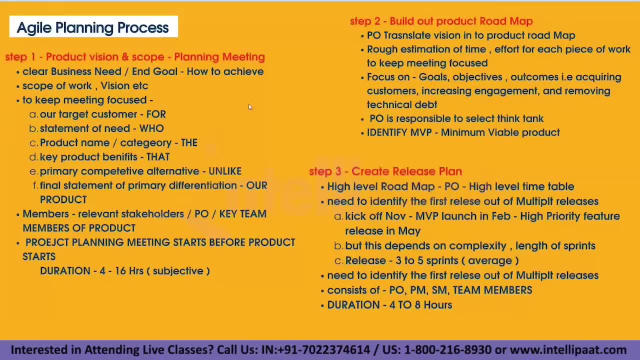 you are into implementation thing, you see the possibility right, how to make it successful because, for example, i am assigning a task to you guys to complete. so when i'm assigning a task, what is the first thing? you see? you see what are the possibilities, probability of success, so probability. 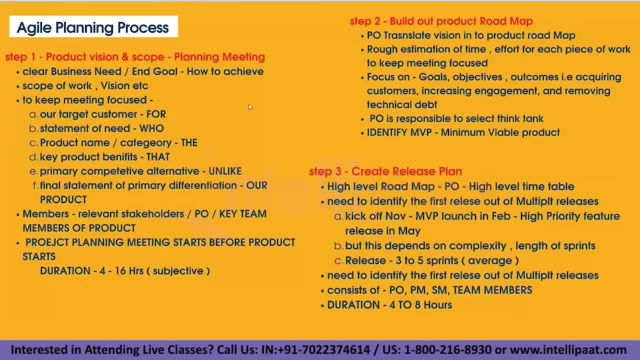 of success. success you will be dividing into two different things: which is in your hand, which is not in your hands. right, what is in your hand? how you are planning. right, have you understood what it is right? how you are planning? right, how your team is going in your hand, what is your? 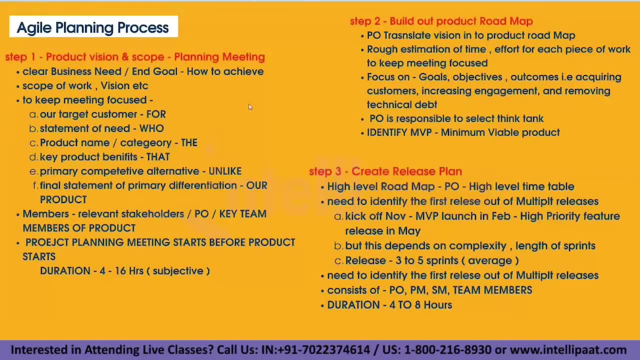 management capacity? what is the technical capacities or business capacities, how well you are organizing your time, your team, all that stuff. all these things comes under the capacities in terms of the internality, which is something relating to you. you are whole and soul responsible for that right. so i am now responsible, which is in your control, which is in your territory, but there 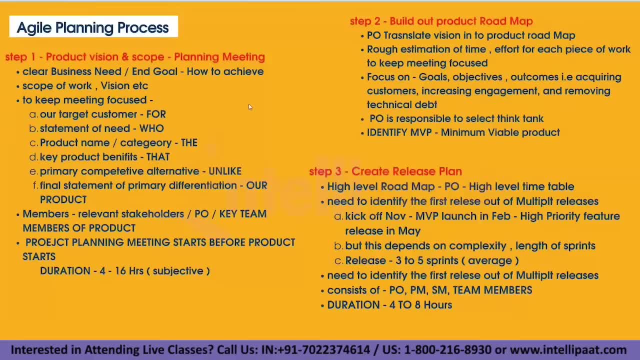 will be some situations which is not in your control. that's what normally we call it as out of scope. what was that? Assume that customer has changed requirements all of a sudden. What will happen? Whatever the scope we have defined and all everything will get deviated right. 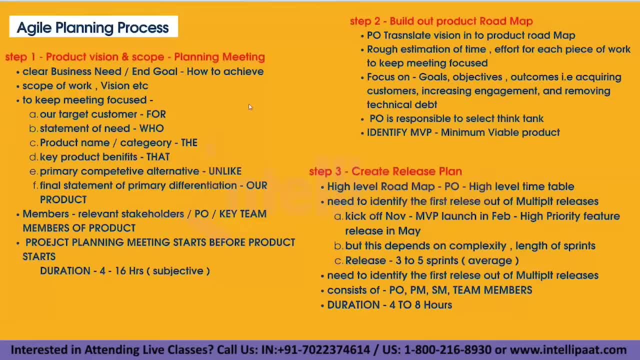 So, whatever we want to implement, something will get disturbed due to this right. So if this is the case, what should I do? How should we proceed? This is point number one. Second, in purpose of understanding the requirements: gathering the requirements before we are implementation or at the time of implementation. 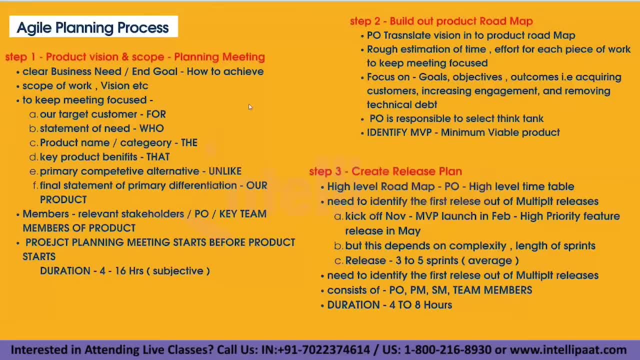 if any sort of additional information we want to provide, is that easy for you to access or do you have any kind of restriction? Because, especially if you see the best example, especially healthcare or finance related products when we deal- it's not easy to access their systems because they don't allow you to access their server systems. all that due to different security reasons. 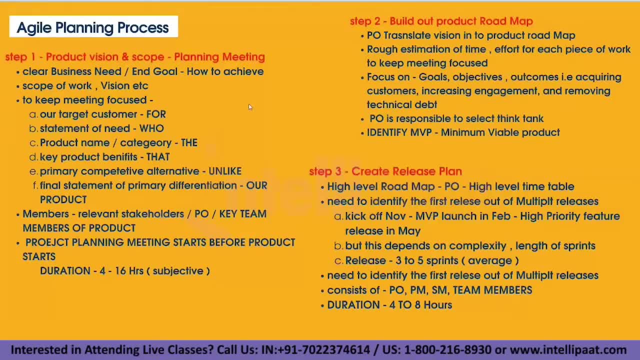 But sometimes there are. but especially for technical team I'm saying this- there will be some problem they come across like because they need to have a sample data, they need to connect to the server and they'd have to test in a process of implementing the project. 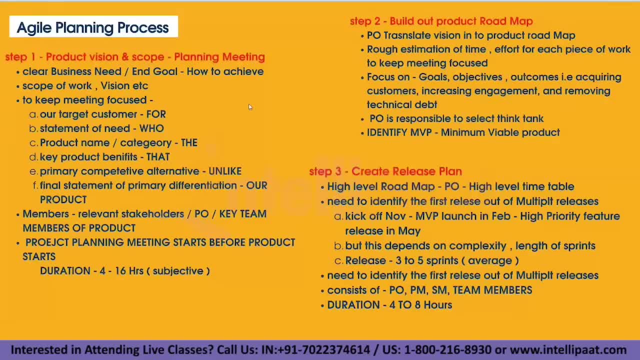 They want to do it right, Some sort of live data- But normally some customers were reluctant due to different reasons, as I told you. Normally those are genuine reasons, for sure, But they don't allow someone to access their system and all of the things for whatsoever reason. 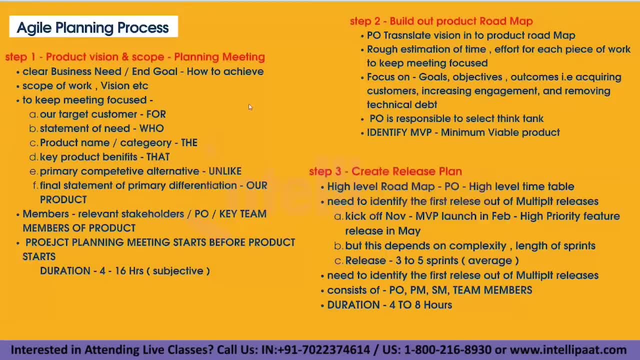 So when we are trying to implement the project, this is where most of the times, we get the problem here. This is what generally the kind of problem when we are facing when it comes to the out of scope, So scope of the project, when we are trying to understand, we have to understand two different. 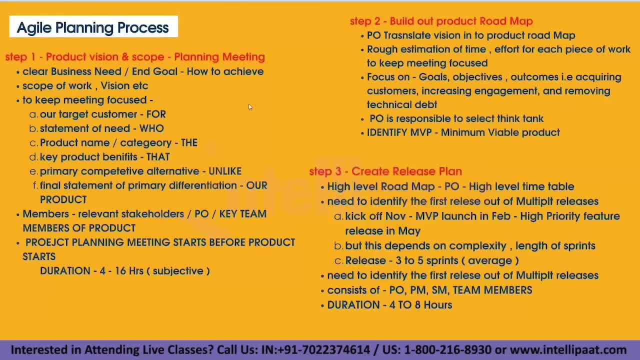 One is in scope, second is out scope. In scope means which is in your control. In your control, like project planning, your team, technical expertise, the kind of model you are using, right, So the kind of technical infrastructure, whatever the infrastructure, desired infrastructure to develop the project. do we have sufficient or not? 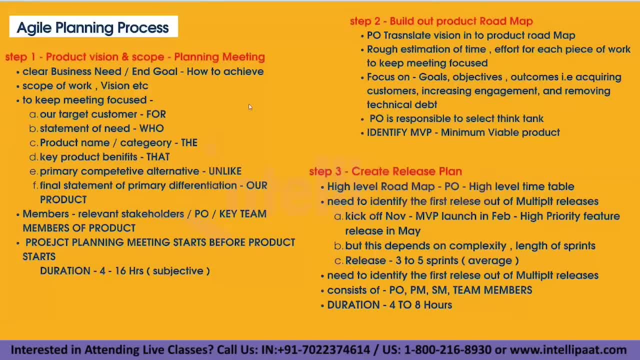 Is this. your technical team is well equipped to develop the product. All these things comes under your control, End of the day, So if you are failing in doing so, that is your responsibility. But when it comes to the out of scope and all, there will be some conditions, like changes in requirements. 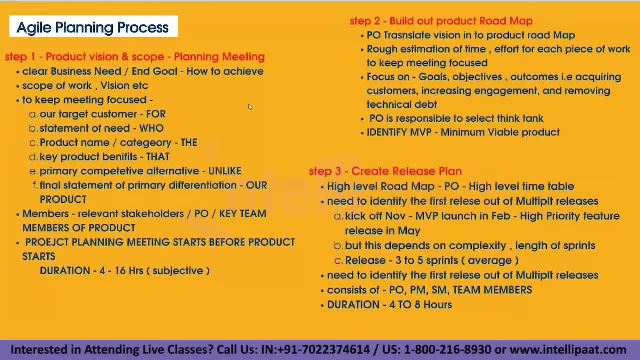 Volatility of requirements Might be taking place. sometimes Changes in requirements happens. Second, not only changes in requirements. sometimes there are possibilities that there is a possibility that sometimes what we call sometimes accessing of information, additional information, may not be so easy. 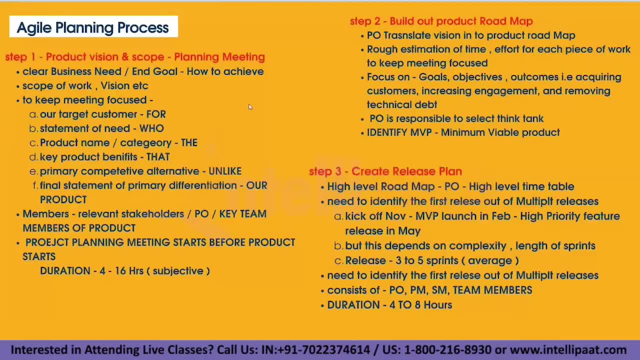 So this is what generally the scope of work from the customer perspective, Because whatever I have truly explained you so far from the client, from the development team perspective, as as for the first level I have explained about the customer perspective, This is what generally the scope, followed by the kind of vision. 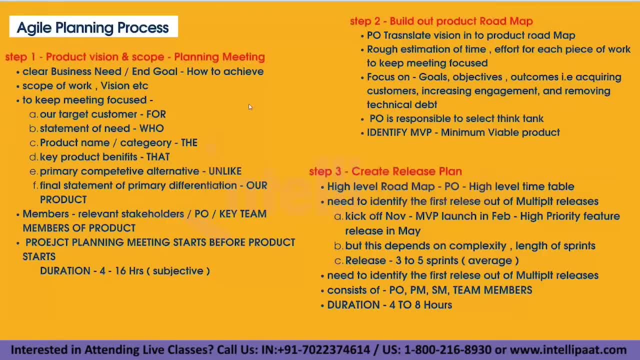 What they want to achieve is what, being a customer, we need to understand. This is. this is the second point. Now, whenever we are going to conduct the meeting, this is where generally planning meeting will be conducted. Of course, if you are in agile team and all, you are nowhere related. 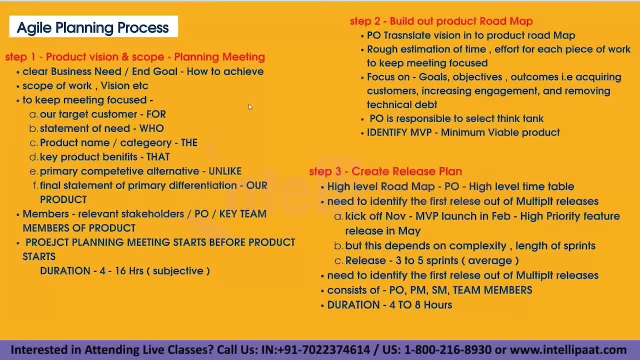 Point to be noted, Because if you are in an agile team, or if you, whenever you are in a team, right, you are part of scrum team or something of that sort- You have nothing to do with this, because understanding about the vision and scope is important. 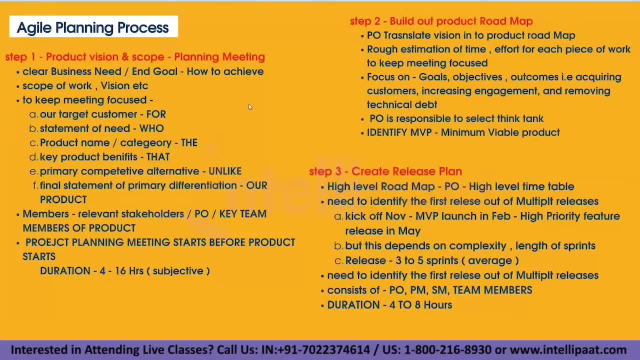 How they are going to conduct and all. it's nowhere relating to your, to you nearly matter, But when you are trying to understand about the agile planning process and all of the things, how it happens and all of the things should be known. That's the reason why we are discussing about these points. 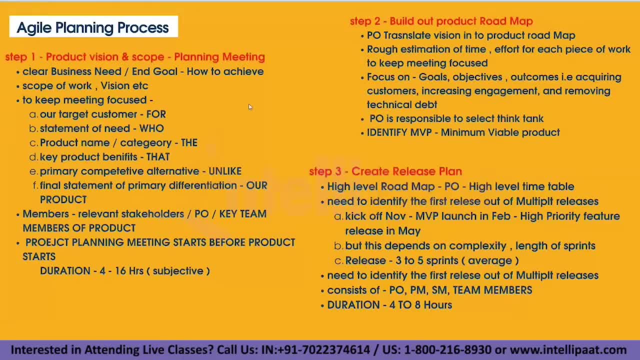 Otherwise it is not required for you. But if you are a product owner, yes, it is required, because we never know how tough people who are comes, who are going as a product owner or a scrum master or team member and all That's a different story. 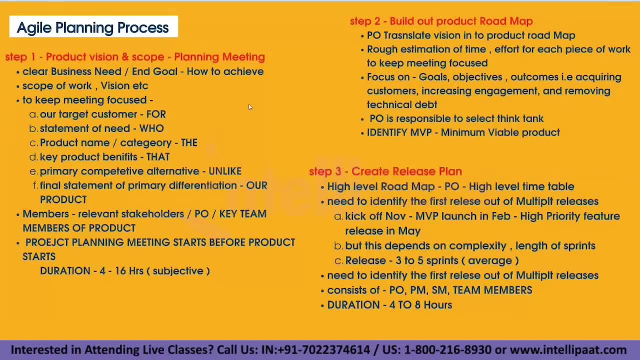 We don't know. So if you are a product owner, for example, maybe in future and all, you must be having a clear understanding about the vision and as well as the scope of the product. What we want, We want to achieve. 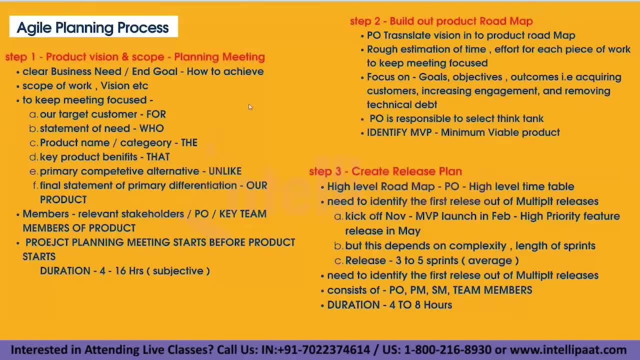 Hence, planning of meeting and all everything will be conducted here at the client location, where they have to focus on the target customers who are going to use the application. Let's say, let us take a core banking target customer. When we talk about target customer, let us understand from the business user, user perspective. 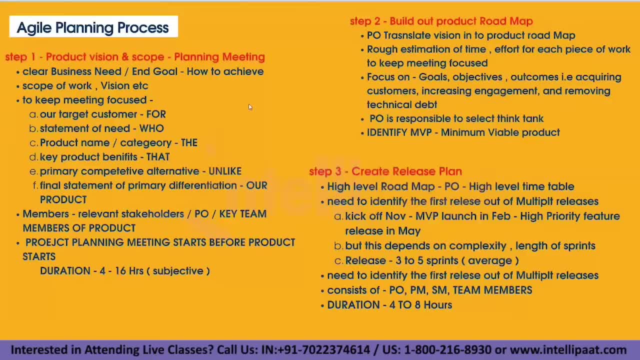 Normally, when you are developing a solution or whenever someone to develop you the solution, for any kind of product, we need to understand the user first, target customers, users. users will be of two different types: Users- People who are inside the organization. 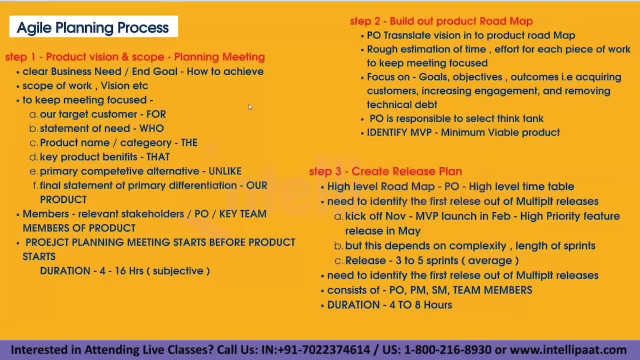 Second, we call it as business users. I'll give you two different examples to you in reference to the user part. If you are developing a core banking application, who will be the user? here? User will be a bank customer, bank employees. They are the users because core banking is an internal application used in the bank itself. 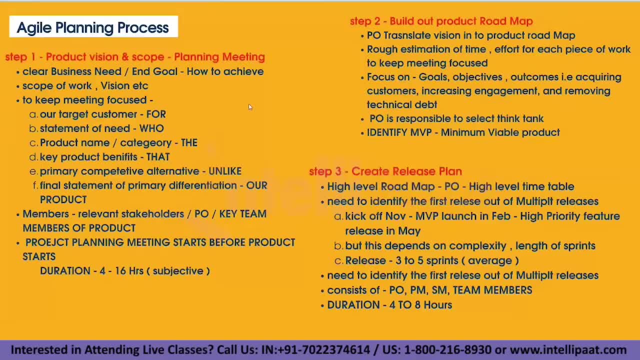 It is not for the external usage. It's only for the banking transactions in regular intervals They'll be using. This is what generally what we called core banking application is being used. So this is only for the internal purpose. Second, there will be some applications like something like e-commerce. 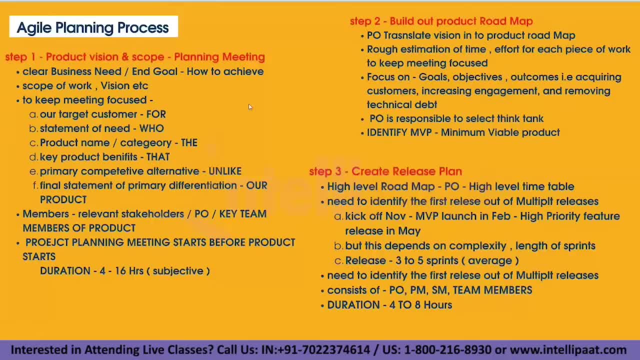 If you take online shopping portal, something of that sort, generally users will be, to one, employees of that portal because they are receiving the orders right. So what are the supply chain process and all of the thing has to be handled by them at the same time. 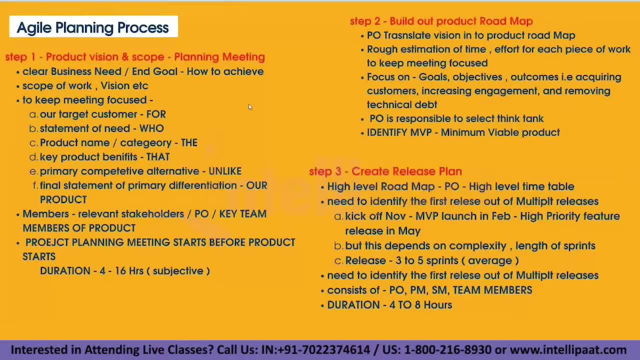 Business, user business uses nothing but customer. For example, if I am a person who is developing a solution for some of the customers, something like online shopping, all that- So what is that I have to do? sometimes Not only a solution provider. Sometimes I have to think from the user perspective. 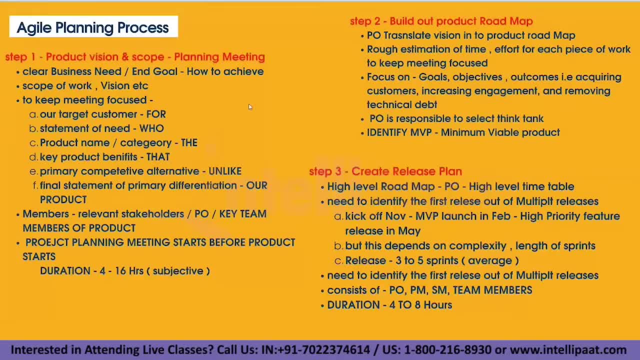 When we talk about user again, I have to think in two different ways. If I am the person who is receiving an order, what is that I am going to do? If I am the person who is placing the order, what is that? 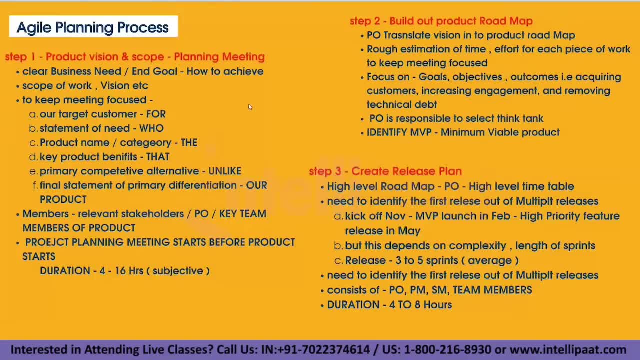 I want, I'm expecting someone should be on the screen right. So when you are developing some solution, when you are becoming a solution provider, it is not always helpful to you from to think from the solution provider perspective. We have to think from the end user perspective, right. 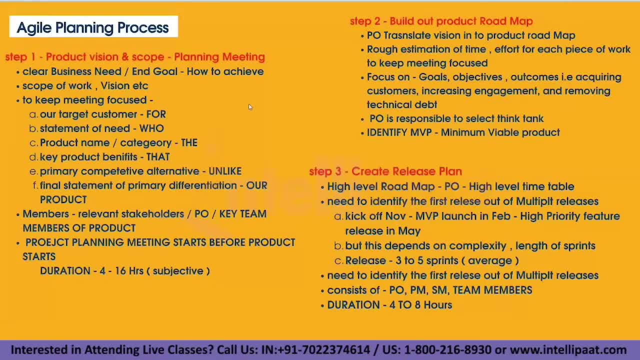 So we have to think from the end user. If I am the person who is going to use this e-commerce application, what is that I'm expecting someone to develop? right? So we need to understand: if I am a person who is developing someone, I'm expecting someone to develop the product. 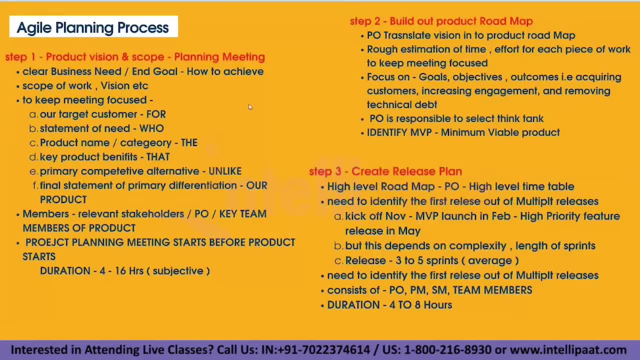 So, first of all, I need to have a clear understanding about the target customers, followed by the need at the same time. What was the name of the product category? What kind of product I'm expecting someone to develop right? Which car under which category falls into? at the same time, 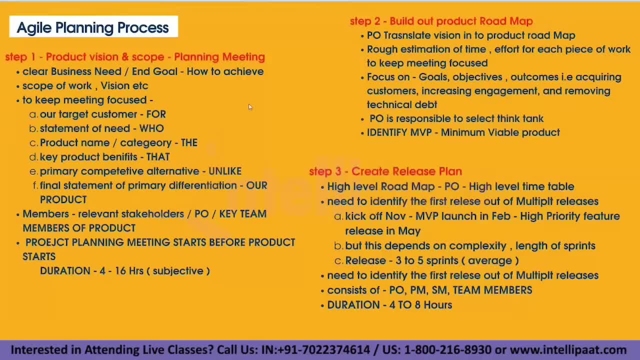 What kind of benefits I'm expecting from the product. because if I'm developing some, if I'm expecting someone to develop the product, for sure there will be some benefits. right, I'm expecting some sort of benefits and all of it. So what are those benefits could be next? at the same time, 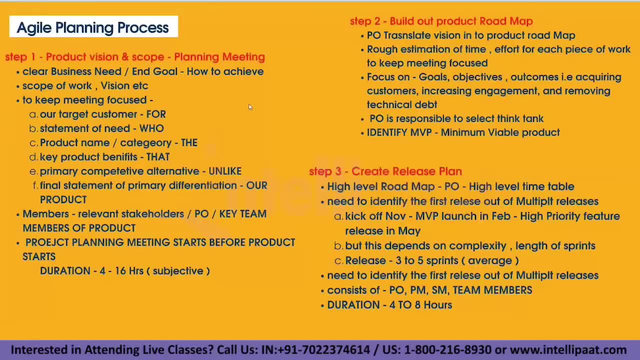 We need to understand the primary competitive alternative. Is there any kind of alternatives? We need to understand when we are developing some kind of solution in future. at the same time, What kind of who are the relevant people who are finally participating in the meeting? 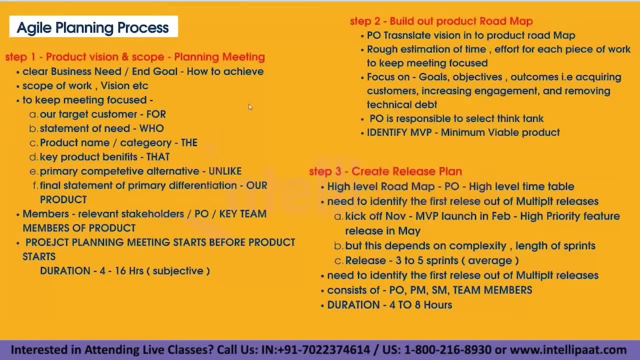 Planning, meeting and all that. who are the people? because if I'm a business owner, I'm not only the one participating. right along with that, There will be some relevant stakeholders, like other functional heads, and all everybody will be attending at the same time. Key team members will be attending of the product at the same time. 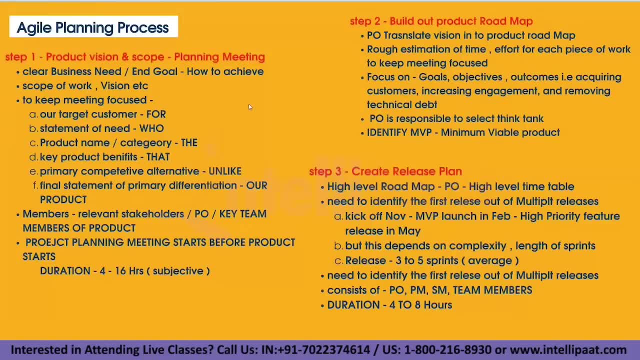 There will be a role called Pivo. in the last time also have told you about the Pivo role itself. Pivo: nothing but the product owner role. So this product owner will also be attended. So, understanding about creating understanding about the vision and as well as the scope of the product. 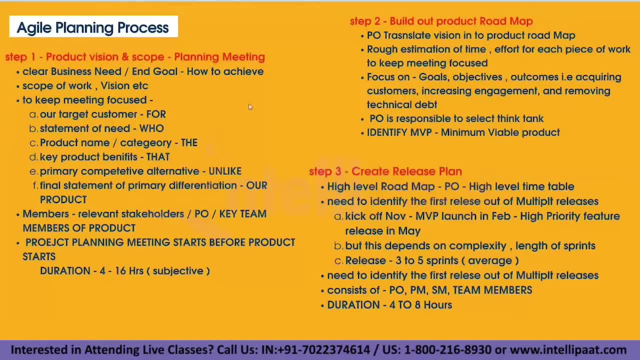 What one must be knowing. So, before you are going to do the project, before we are going to develop any kind of product, and all that, one must be conducting this meeting so that they'll be having a clear understanding about what they are expecting and what they're up. 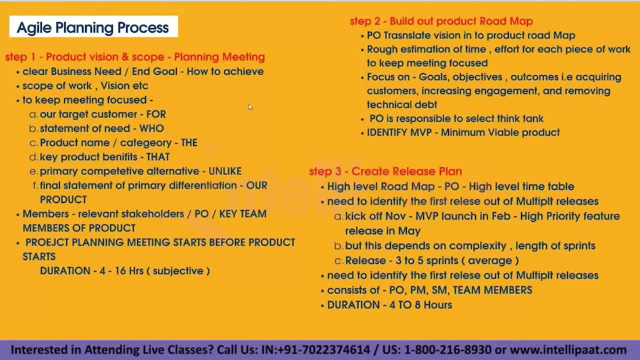 They're expecting, the product must be finally right. So that sort of clarity is required. So, in agile planning process, the first step will be this point Number two: based on this, based on the clear understanding, based on the meeting, based on the inputs, what we have discussed, 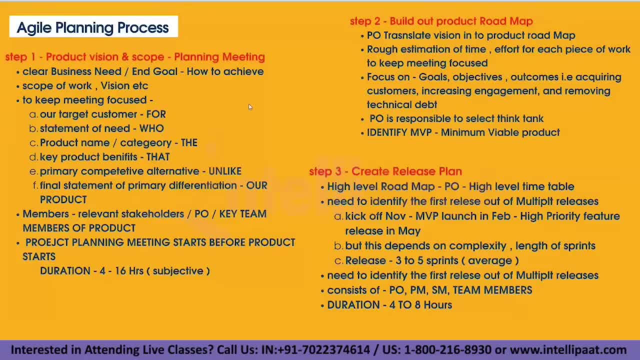 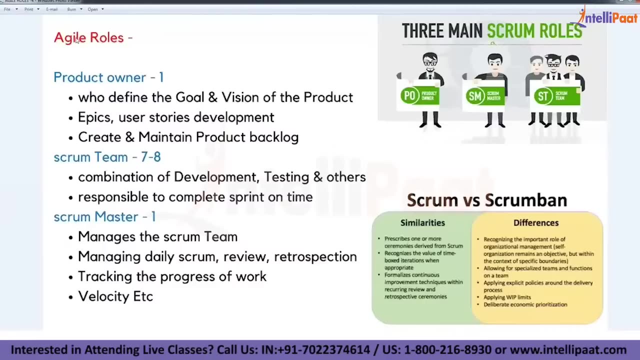 So far, based on the final conclusions, What we have made in out of this meeting. from here onwards, the responsibility of a Pivo starts because, if you remember, I have explained you about the roles of a product owner right. So here I've told you right to define the goal and vision of the product, all that I have discussed in the earlier session. 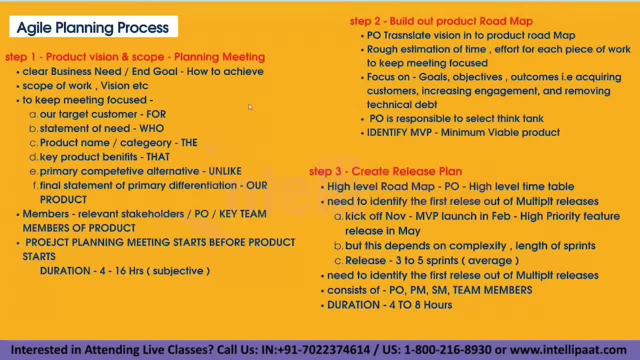 If you remember, this is where generally a product owner do means if I am a product owner, reason that if I am a product owner. as I have attended the meeting, I got to know what is requirement, right. So what? what is their Expectation? everything known to me well. 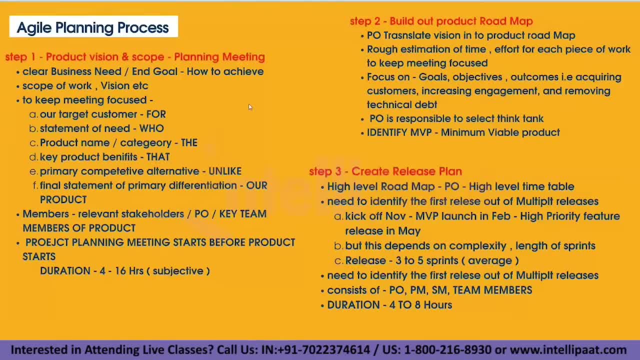 So, being a product owner, what I have to do, whatever the vision- and what vision means? what is that they want to? they want to see near times. right, That is what generally we want to have a vision. So I want to make that vision into a visual representation. 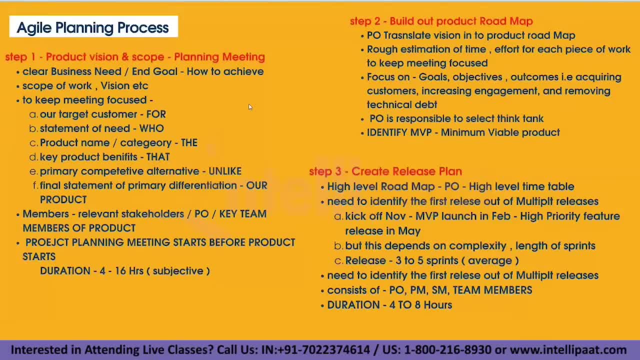 This is where generally, reality comes into. picture means I want to make it real. if I want to make it real, What is that I need to have? I need to make it visual. This is where generally we call it as product roadmap. I'll give you an example. 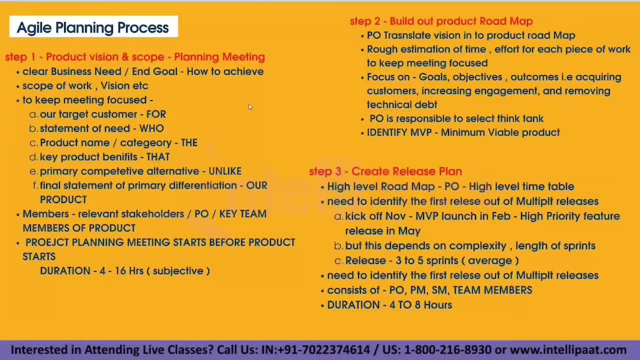 To you because I'm not explaining Jira here. I'll explain Jira in some time, Maybe once it is done, and all of the thing I'll be showing, because there is an application in between. Anyway, I'm just explaining about the this part. 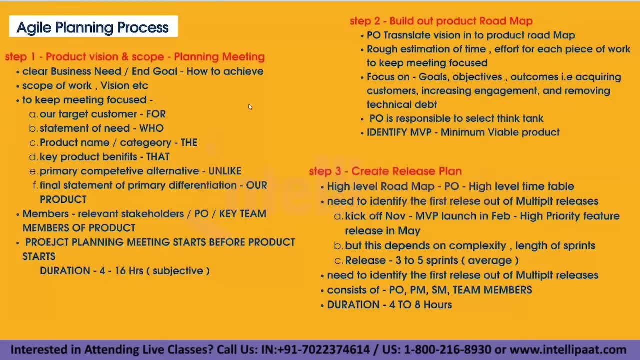 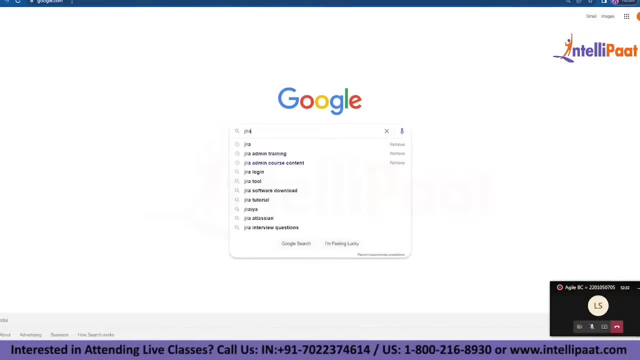 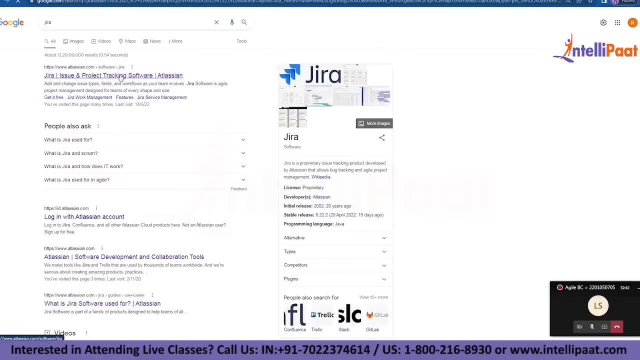 I'm explaining about product roadmap to you. Let me introduce this Jira part. There is an application called Jira. Usually it's kind of project management tool- compact tracking- which is widely used across Industries for managing the project, all that stuff. When you see a product, for example, this is in high level explanation. 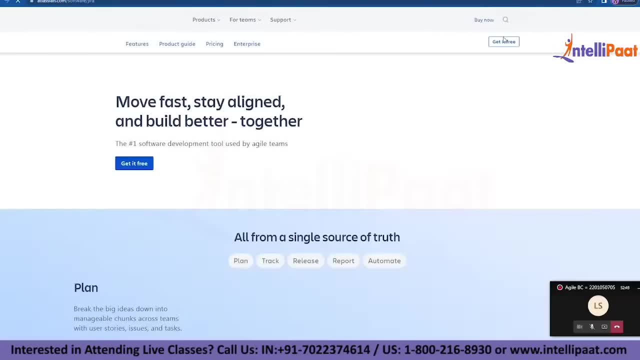 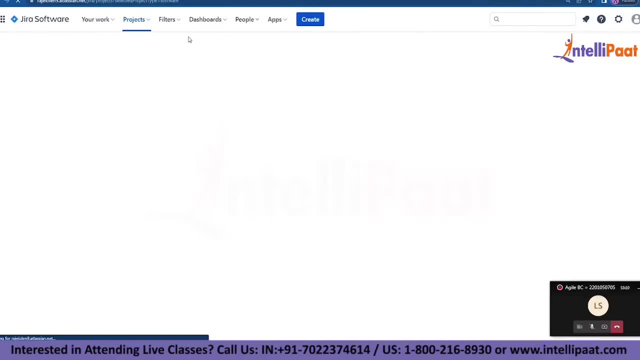 I'm giving so because I'm explaining about the project planning. I'm just showing you here, right? So if we can go to the projects, how to create project, and all I'll show you means, once this is everything is done, Finally we go to that right, how to create project and how to. I'll show you that later. 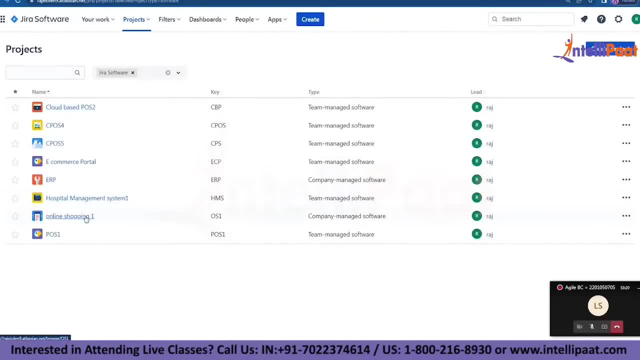 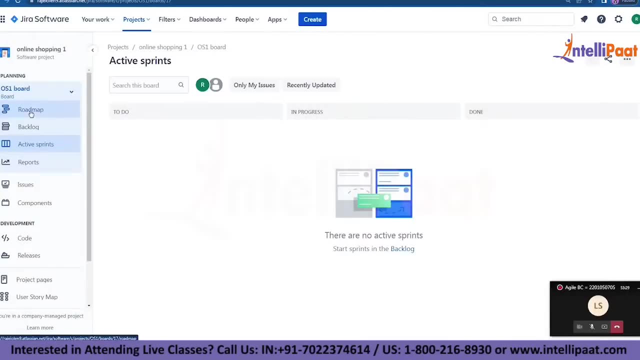 Let me show you if there is an existing application called, for example, online shopping, This is one application. So this is where, generally, a roadmap has to be created. First of all, we have to create a roadmap. roadmap means what are all? because based on the, this is what, whatever the epics you can see here, all that stuff. 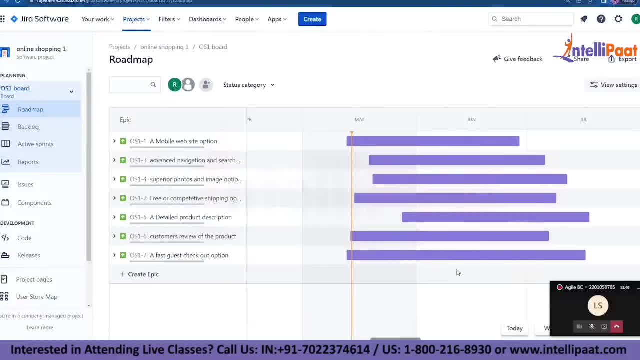 This is what generally the roadmap, This is what generally a roadmap stands for. this roadmap has to be created by the product owner. How the roadmap? this roadmap has been created by the product owner based on the kind of meetings They had earlier means. this is where, generally, this creation of product vision goal. 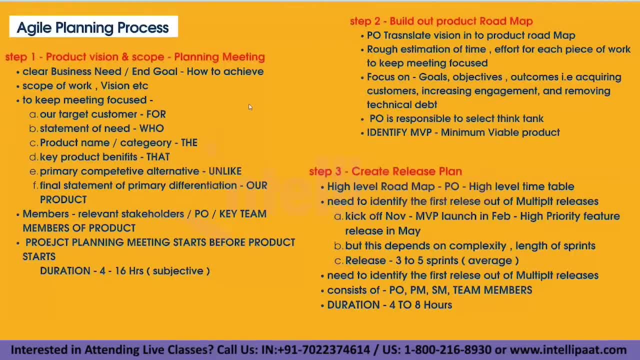 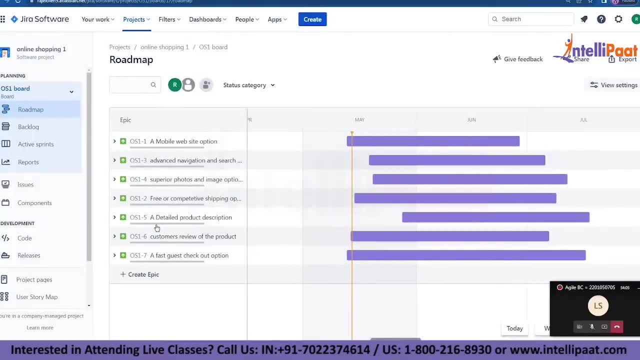 All that stuff happens. based on that, a product owner is the person who is responsible To build a product roadmap. This is how generally a product roadmap looks like. means there are epics, user stories, all that stuff. I'll explain one by one later, right? 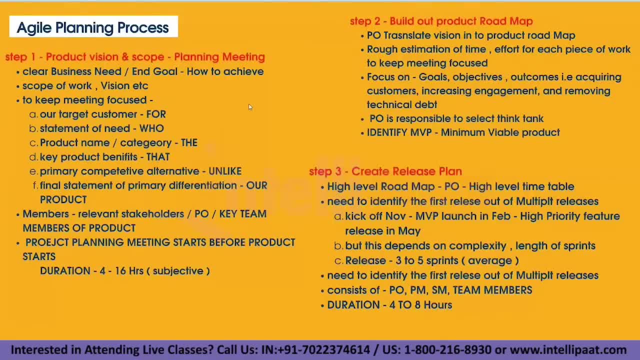 So this is where, generally, the product roadmap. So, whatever the vision and whatever being a product owner, I have something in my mind. means in my mind is that I want someone to. I am expecting an online shopping portal to be developed Now, being a product owner, 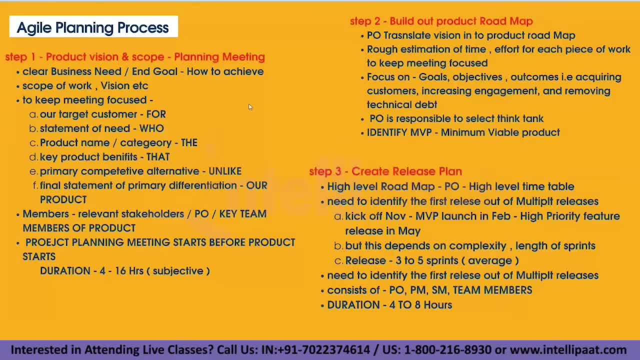 What is that I have to do? I have to make it into reality means I want, I have to create a product roadmap First. product roadmap means what are all the features should be there in each and every product. For example, website option of mobile is required. 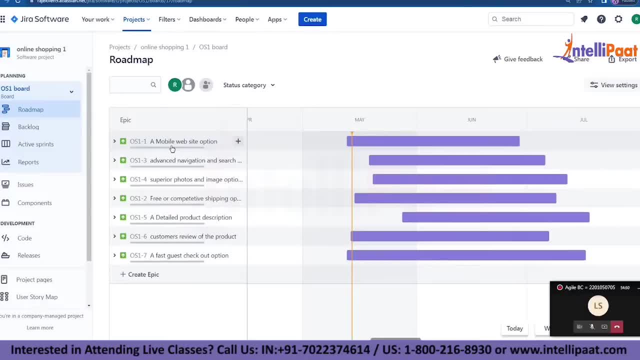 Mobile website option is one kind of epic is required, Advanced navigation, and such is one more epic. I require superiors. photos and image options is one thing. at the same time, Product descriptions are customer reviews right, She cost option. So these are the different, different epics which, based on the interaction, 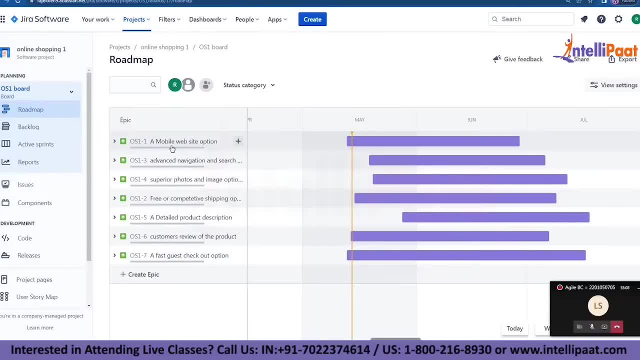 As well as the discussion we had with the team. Finally, being a product owner, I have decided that these are the epics. majorly, My customer means myself. being a product owner, I am expectation that I am the owner of the product issue. that right. 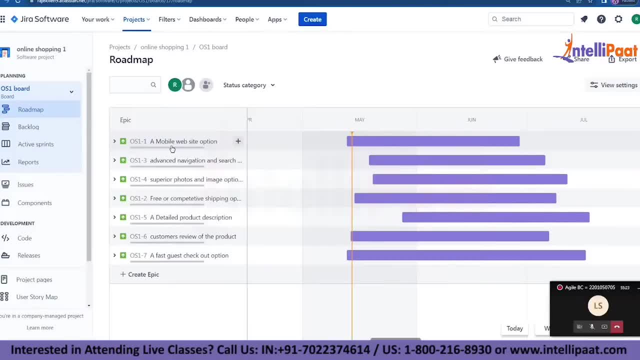 So, if I am the product owner, this is what I am expecting. So assume that you're all belongs to the technical team, wherein, if you want to understand and to implement the product successfully, being a PO, I have to create this epic first. First of all, I have to create a big at the same. 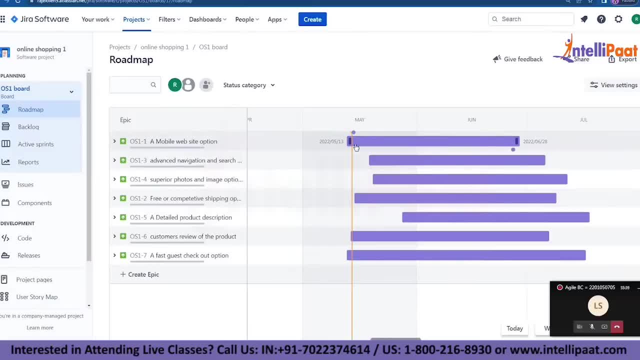 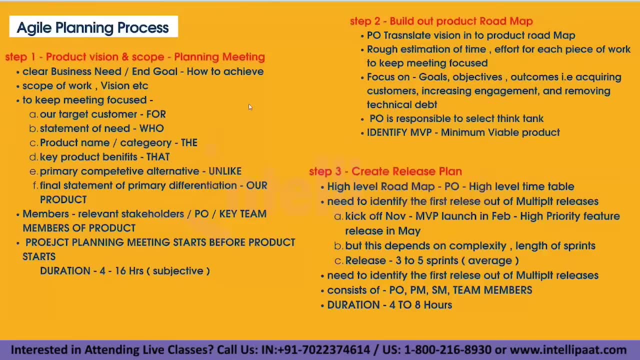 Time, not only creation of the pics. I have to give some timelines Also. these timelines, remember, were nothing but the estimation timelines because, being a BO PO, I must be knowing about the rough estimation Now how much of the time it will be taken for the team members to develop right. 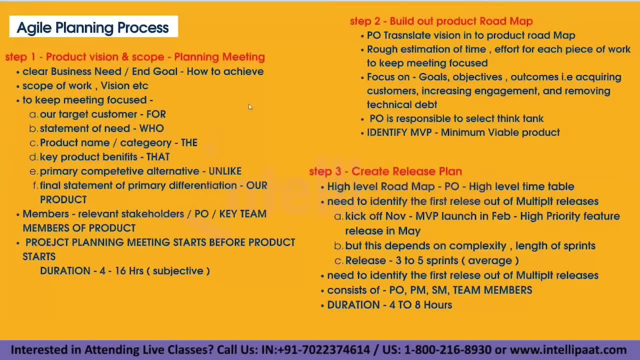 So what is the amount of time it will be taken for us to implement? right, for you guys to implement, because, end of the day, implementation and all everything will be done by you, accepted, But even though you are implementing the product, first of all being a product owner. 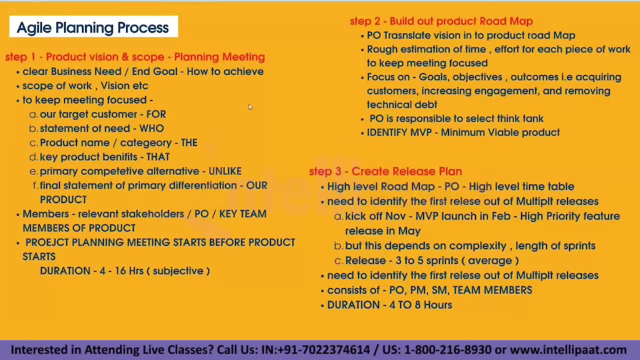 I need to have a clear understanding about the kind of effort estimation. How much, how much effort estimation it will be taken for me to implement. That is what generally you must be having. This is what generally call it as rough- rough effort estimation- months. 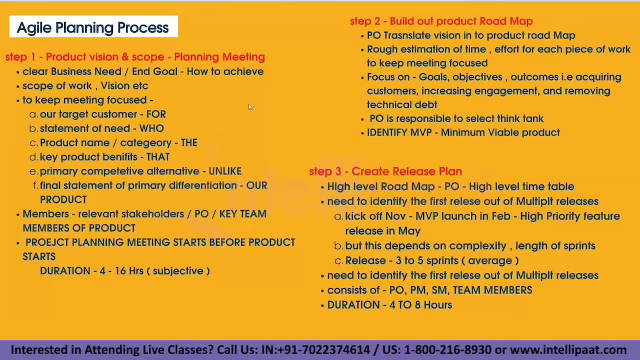 How much, approximately, it will be taken for a team members to develop the product, the whole product, right. How much time it will be taken for them to develop the project is what generally, the rough estimation time, all that. So the rough estimation time is what generally. 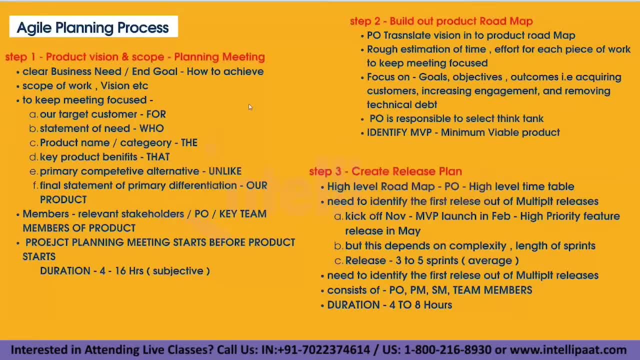 We must be knowing this is what generally happens in the second level means being a product owner. What is the first to have done? I have understood the goal and as well as the vision of the product, followed by this, I need to understand rough estimation time. 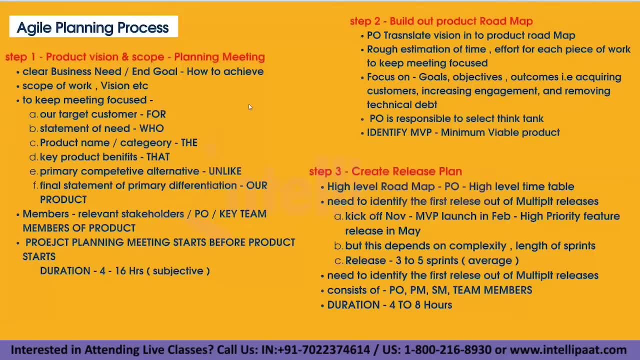 right. How much amount of time it will be taken for me to complete the product. at the same time, How much effort it will be taken for someone to develop the product, is what, first of all, I need to have. I need to know first, now, based on this, 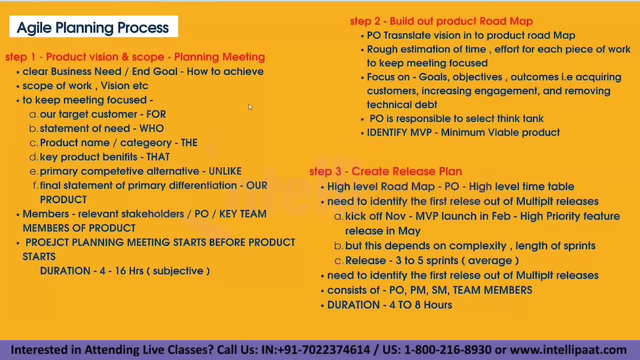 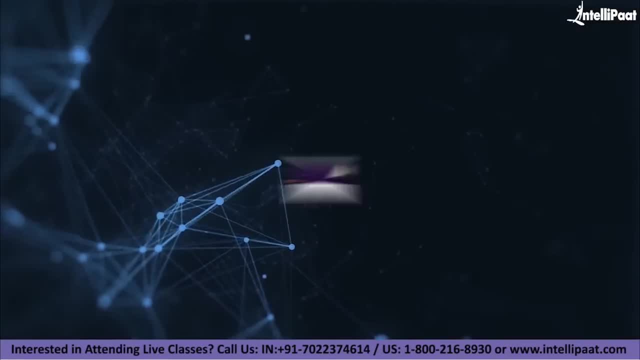 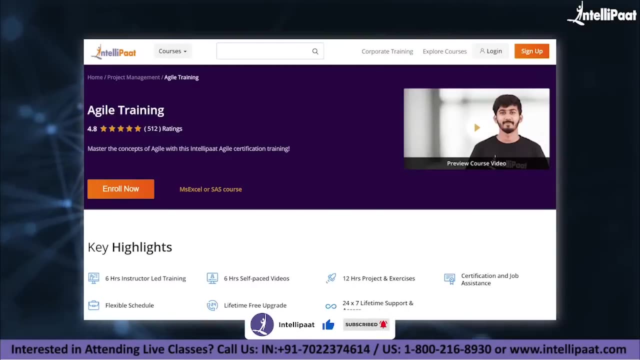 I should also keep something in mind about the kind of goals and objectives means. again, These goals- objectives- will be two different types, as I told you. just a quick info, guys. Intellipaat provides agile trading mentored by industry experts, The course link of which is given in the description below. 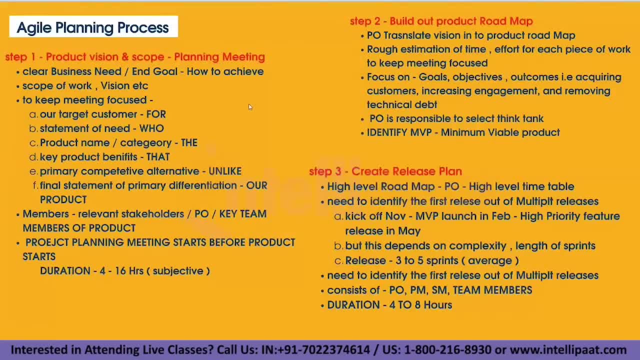 Now let's continue with the session. Whatever we discussed in the planning meeting is all under under the business goal. Now, whatever the goals we are discussing here and all everything comes under Project goal means based upon the business goals and all that. 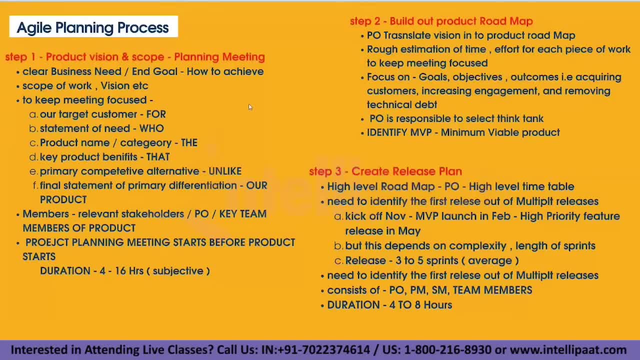 So what is the project goal and all everything that we have to see. So the goals must be knowing. at the same time, We must be knowing about the objectives. Any project is been connecting with few things. first, objectives and goals. second, need, followed by the scope. 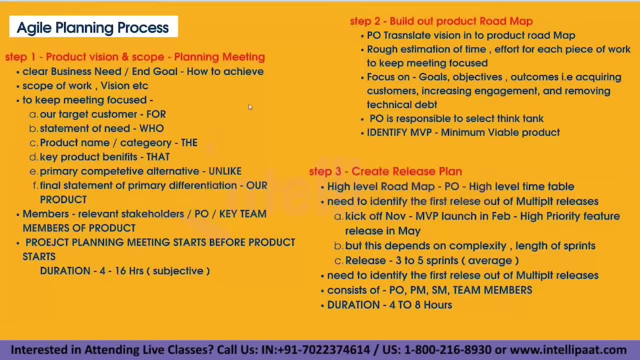 These are the three major aspects. will be there for any of the project, If you want to develop any kind of product, if you want to develop any product to be successful in long run. So we have to focus on three different things. One is objectives and goals. second is need, third, followed by scope. 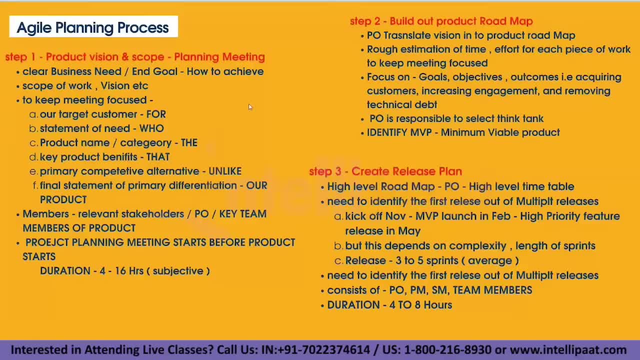 If there is any kind of clarity, which is missing in these three things, The product will be. even though product is developed, end of the day It is not surviving the actual purpose what customer is expecting. That's the reason why I need to have a clear understanding about the kind of business goals in connection to that. 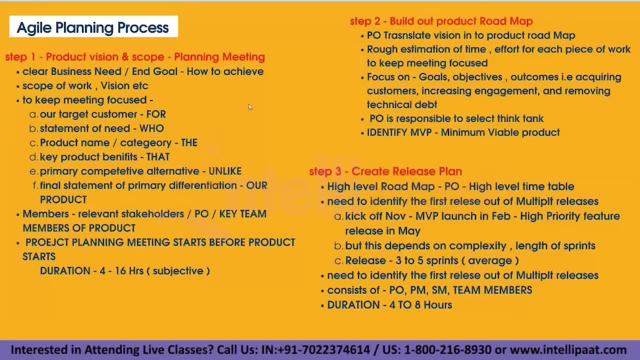 What kind of product you are developing. that product goal must be connecting to this. at the same time, What kind of objectives we want to achieve. finally, is what we must be knowing about in this second step comes under the product roadmap, Which is being done by the product owner, for sure, at the same time. 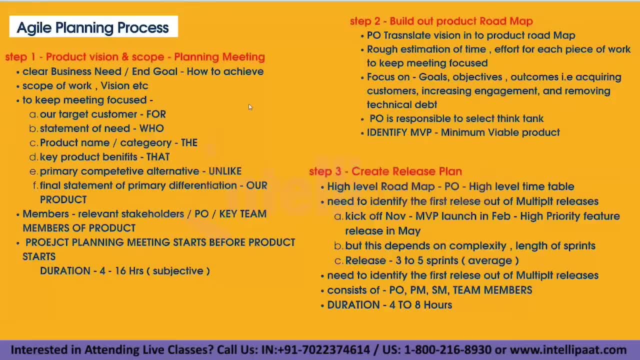 This product owner should have responsibility to create a product backlog. This is where generally product backlog and all everything comes into picture. Normally, before we are going for a product backlog and all a product owner should have to and should, should prepare or else Should have an idea about the MVP part. 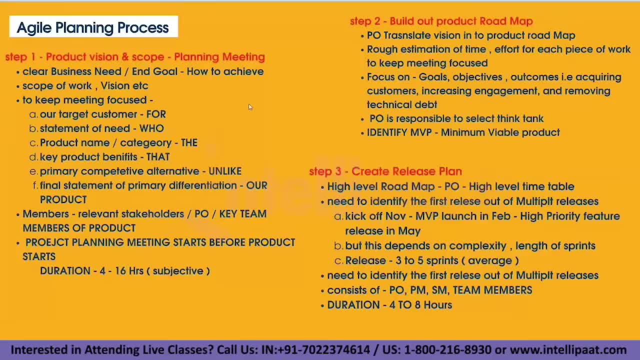 This is where MVP. what is MVP? MVP, nothing but minimum viable product. in other sense I can say like: because in agile normally we call it as MVP, all that, normally we call it as minimum viable product, Minimum viable product, nothing. but it's something like a prototype. 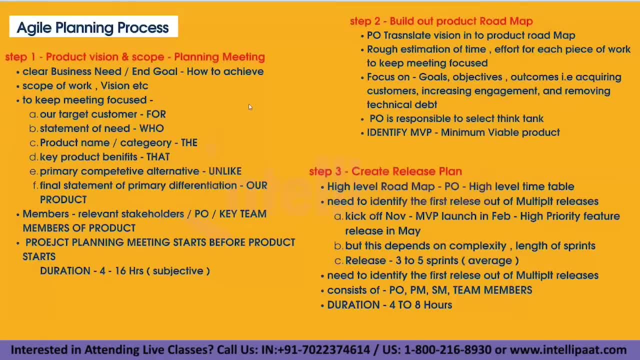 For example, someone wants to develop an e-commerce portal, right, something, website or something, Normally for a general, general understanding, and I'm giving this explanation to you. For example, someone is expect, Expecting you to develop a website now, before you are going into a website or before you are going to develop the actual website. 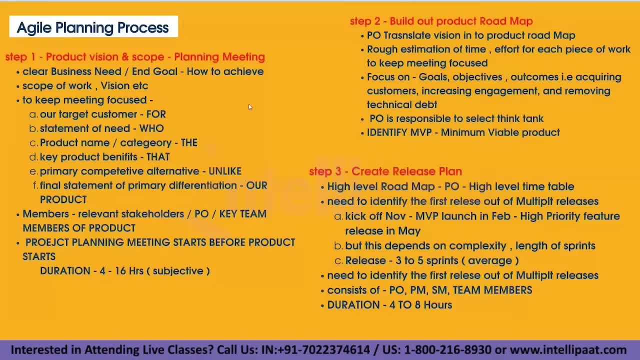 What is that? normally happens sometimes? because, if you are, anybody come from that segment will be knowing that well, you are developing a website to one of your customer. So when there is a negotiation taken place, whenever there is an interaction happened before, you are going for a full-time website implementation. 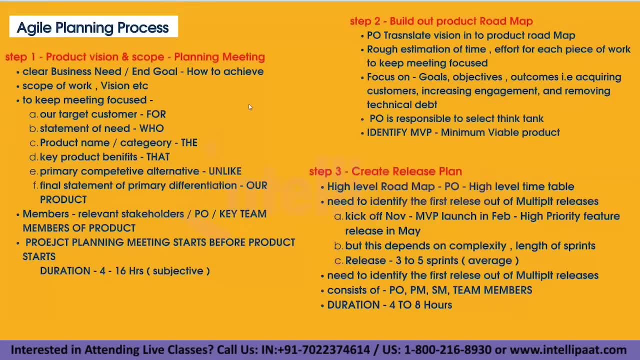 What is that first thing they'll ask you? first thing they'll ask you to develop some prototype, isn't it right? So demo kind of thing, prototype They'll ask you to develop first, So that prototype may not be the real one. Assume that right and there is no guaranteed that program will be going on the next level, because this prototype will give you and clear understanding about how it looks like. 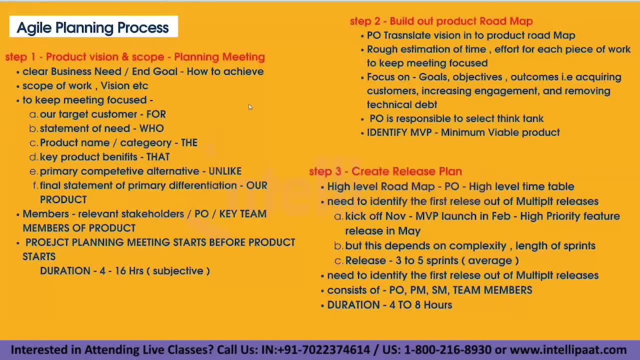 Right. So how it works from an external point of view is what generally prototype. so, based on that prototype and all, what is that customer say? customer has given you the signal: Yes, next level will be implemented. the same prototype will be Turned as a product, right, so turned as a website and we complete the whole thing. 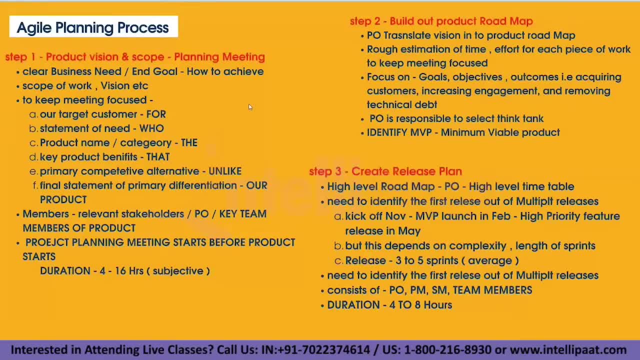 This is how generally happen. the same thing happens even in agile environment, but we call it as identifying the MVP like minimum viable product. What is the minimum viable product which customer is expecting at this level means being a product owner. I have to understand. creating an MVP first. 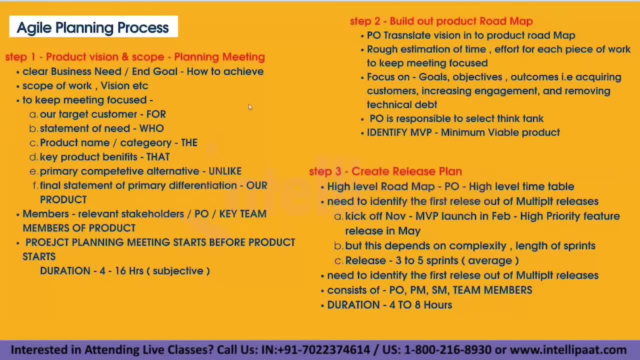 I need to identify the MVP. this identification of MVP and all everything may not be the real one. right, Because there is no guarantee in agile that MVP implemented hundred percent. as as as a as this because there may be some sort of changes and all happens in between. right because, but to have a clear understanding about this first of all, 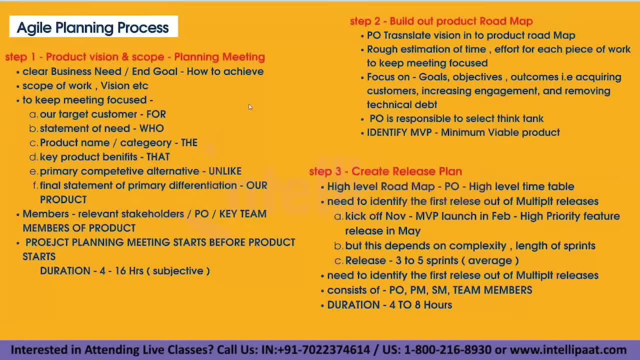 we need to identify the MVP- This is what we call it as minimum viable product. So if you are a product owner, based upon the understanding, what we have, first of all you need to translate whatever the inputs you have taken and whatever the final conclusions. 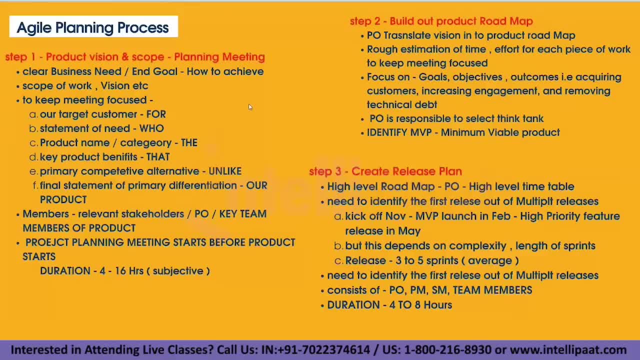 You have identified So far, those you have to translate into product roadmap. So, once you are creating product roadmap, if you want to create a roadmap of the product, you need to have few different things. One: you need to understand the epic, followed by the pic and all that. 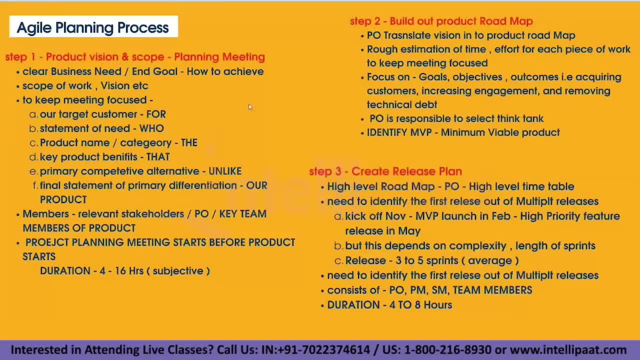 So you have to write down the user stories, user stories. If you want to write down the user stories and epics and all everything, first of all you need to understand the actual solution which you are expecting someone to develop. So, based on that epic, epic, nothing. 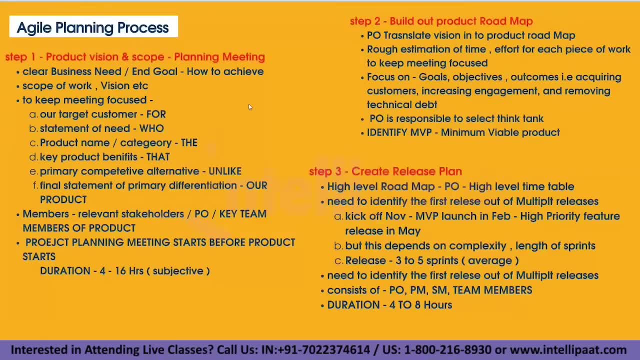 but I can, simply, I can call you epic, nothing but a feature. epic, nothing but a feature. So again in feature, there are different, different functional and non-functional requirements will be there. Those functional and non-functional requirements will be called as user stories, right? So all these things and all comes under the product roadmap. 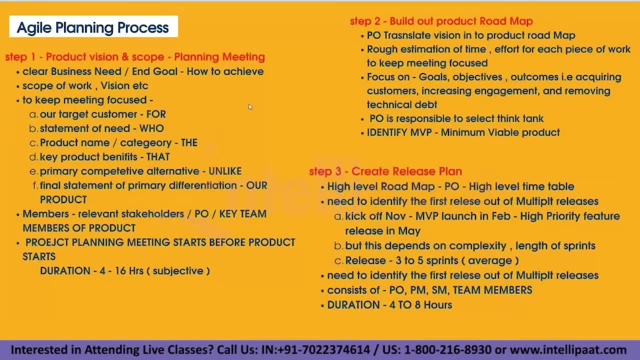 So, once the product roadmap has been created, we need to have rough estimation of timelines is required. at the same time, What is the goal of objectives and, as well as the goals, What we want to achieve? Finally, at the same time, a product owner is the person who is trying to identify the minimum viable product. 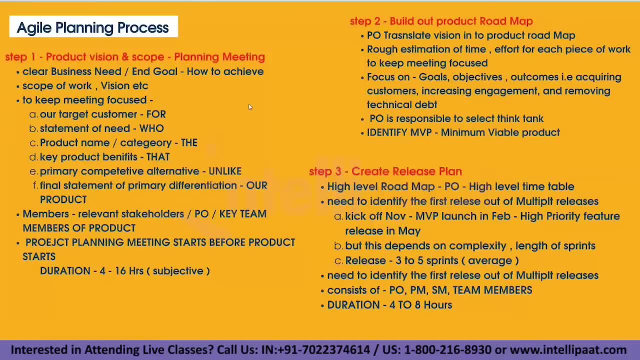 which is to be developed first. So, based on the minimum viable product, next level product implementation will be taken place because this is the base level to move on to the product, to the next level, because this is the minimum thing which customer is required at this level at this stage. 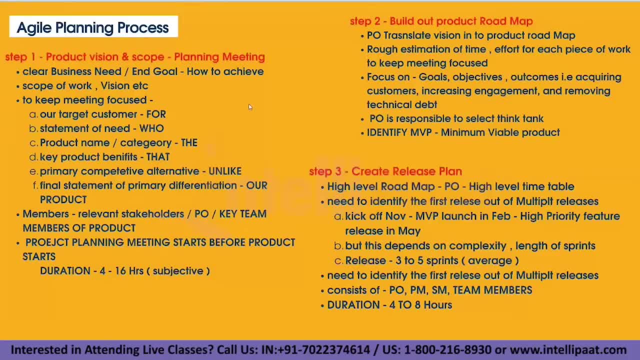 It doesn't mean that it will stop, to the extent it will go to the next level, but this is the minimum available product which gives a clear understanding about the high-level view and high-level understanding about the product. all that, This is what generally- the second- we call it as product roadmap. 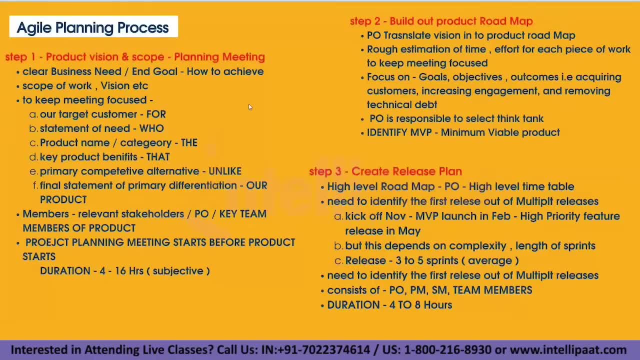 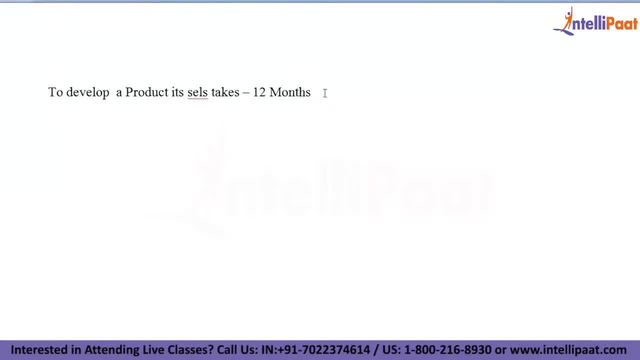 Is it clear to everyone. any doubts in these two points? any questions now? for example, let us understand release planning process here. For example, to develop a product itself taking 12 months. Okay, I'm making it simple so that you'll be understood by 12 months now. 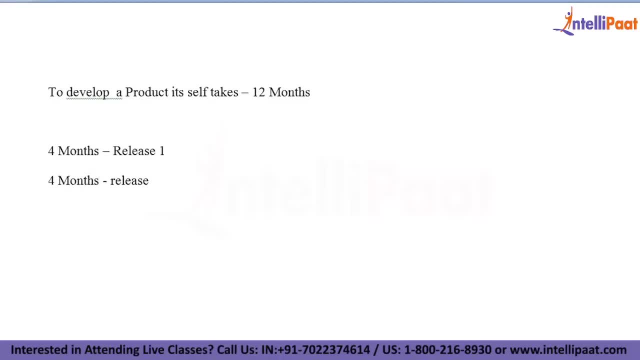 release one in four months. There is release two in another four months. There is release release three. right, There is release one, release two, release three. Now, if you are completing the whole product, it is itself is taking 12 months. 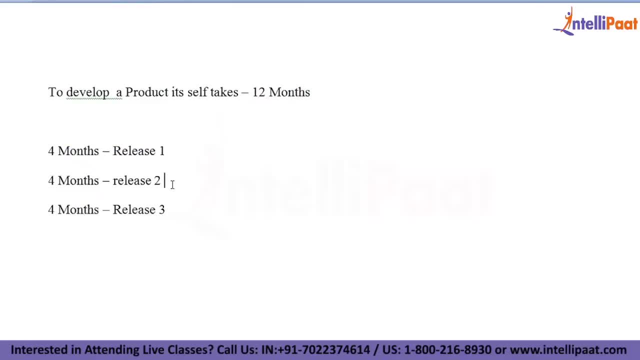 But whereas when we are doing agile implementation, whenever we are working in agile implementation, the planning process and all everything happens through release, part release, one release, two release Now in the first release. assume that right in the first Release, product owner wants few epics to complete. product owner wants few epics to complete it. 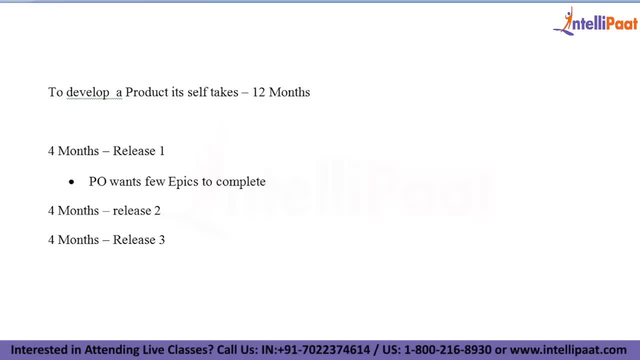 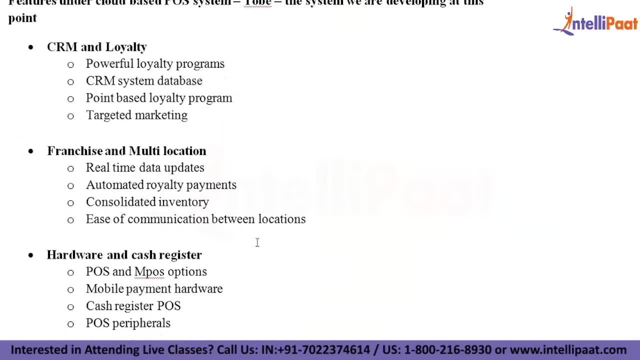 You can take any of the product. Let's say, for example: let us take our point-of-sale system as an example. I'll show you, for example. Yeah, so, for example, this is a cloud-based point-of-sale system. Assume that these are the different, different features. 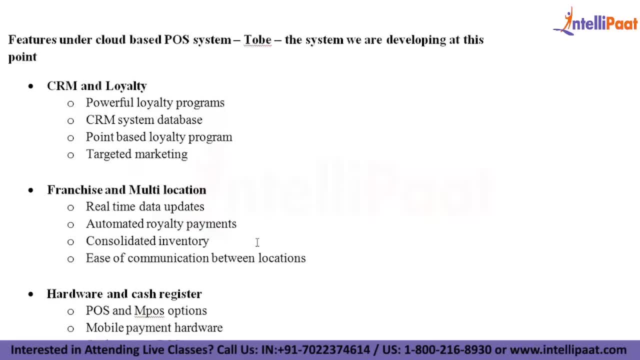 We have different, different features We have now. customer is expecting a CRM is one thing may not be required. All the user stories can to develop on the first level. right may not be now. For example, customer is expecting few epics here. For example, CRM, loyalty, hardware in cash registers. 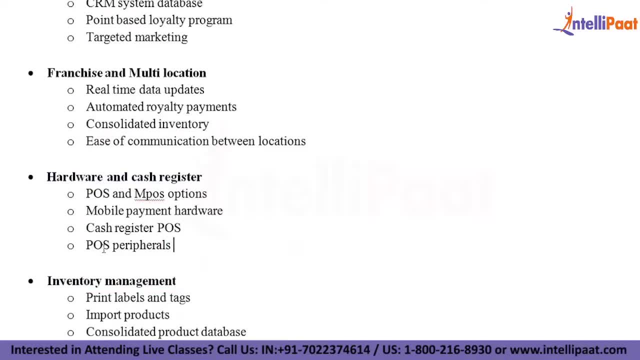 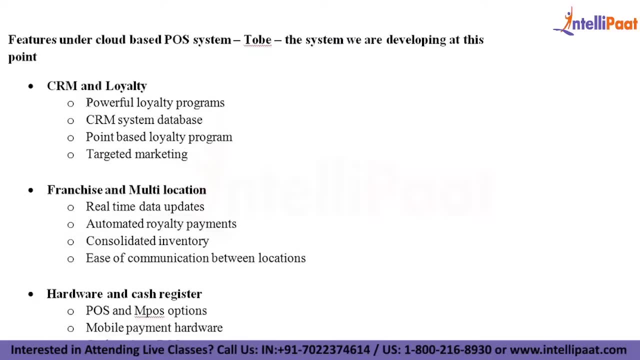 maybe inventory management system. So these are the three epics required by the product owner at this level. So if you are taking three epics into consideration, how many user stories we have, we have four user stories here. Remember, again, I'm repeating, if you are taking about, 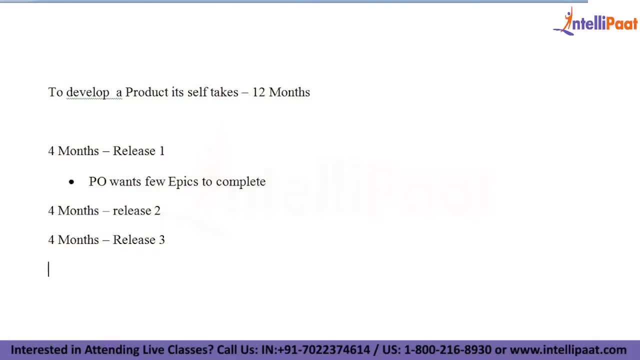 product backlog into consideration because next time, next thing got me what I'm explaining about product backlog. because product backlog nothing bad. It's a repository to store all the user stories. to store all the user stories. Normally product backlog starts. If you're talking about product backlog, user story is nothing. 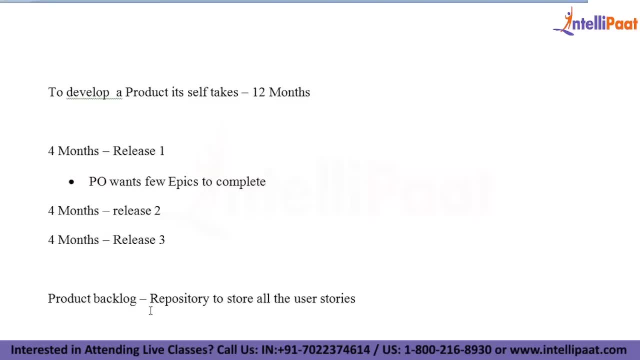 but only functional requirements, even technical dates, even technical requirements, bugs, everything will be there. in that that, I believe that I'll be explained it later. Okay, Now what is that we want here? For example, customer is expecting CRM loyalty is what wants to develop in the first level. second, 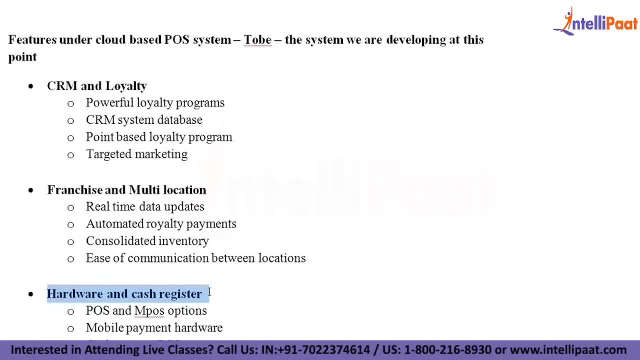 They want inventory management system. third, hardware in cash register. These are the three different epics which customer is expecting us to complete now. How many user stories we have assume that functionality? nothing but the user story for 4 plus 4, 8, 8 plus 4, 12, right. 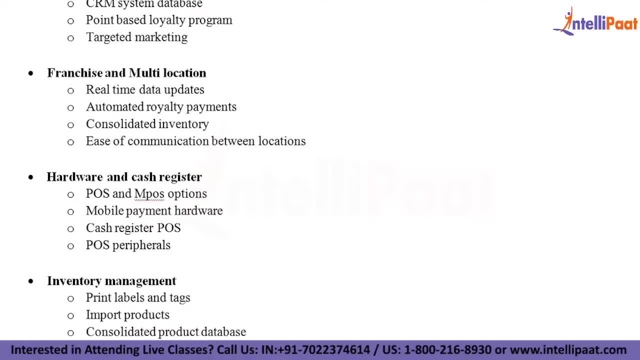 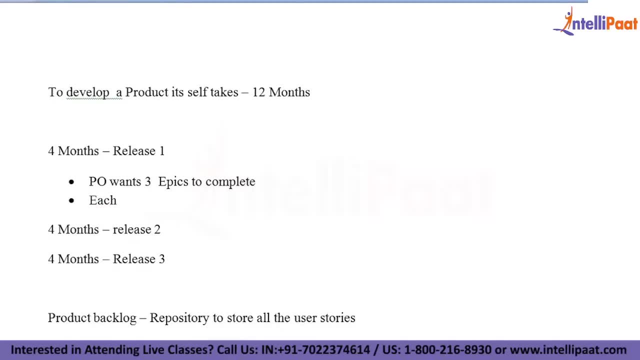 So 12 user stories. So how many user stories? there are three epics, three epics to complete. Okay, each epic, as per the case today, have shown you, I'm writing you as an example: each in epic total. epic total, three epics- consists of 12 user stories, nothing but 12 functionalities. 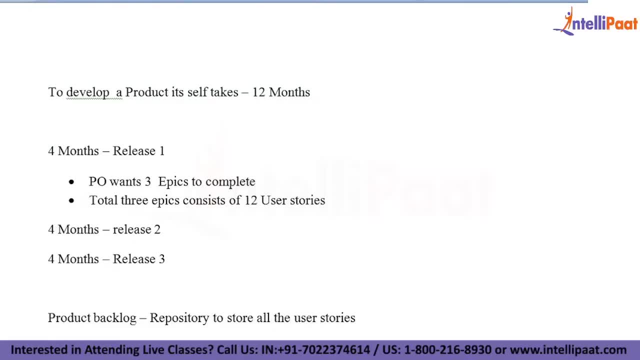 Okay, forget about technical requirements. all that aside, I'm talking about only requirement, functional requirement. I'm talking three epics to complete total. three epics. total consists of 12 user stories because one epic may be having four, one more having four, one more having four, four into three: 12 user stories to complete. 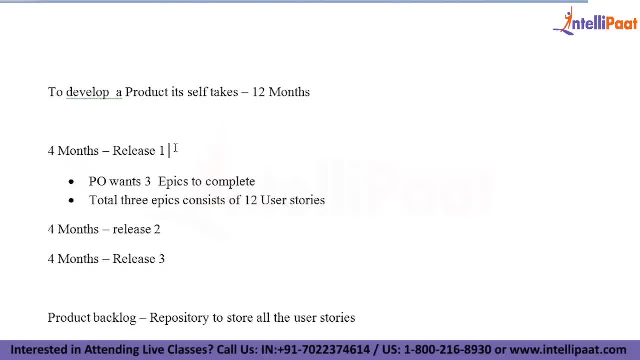 This is the first release. now, when you talk about four Months, when you talk about four months, how many weeks it is? four weeks into four months means 16 weeks, right? 16 weeks is what the time we have. 16 weeks is what the time we have. But when it comes to working days- because this is where generally print, planning and all everything comes here, When we talk about this in your converting into working days, how many? usually five days per week into how many weeks? 16?. Five days in a week into 16.. 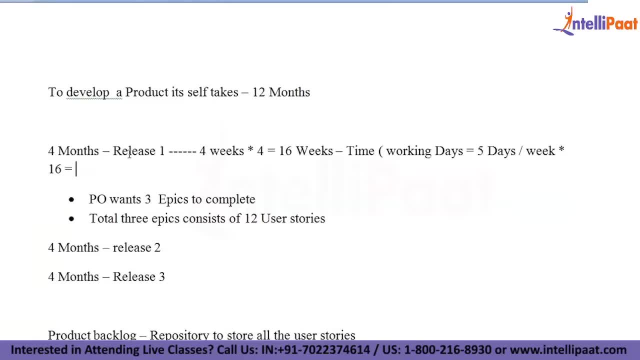 So five days in a week into 16.. So which is coming around 80 working days because, especially in agile, whenever we are going for spring planning and all normally whenever we are doing the release part and all, we have to take working days into consideration. 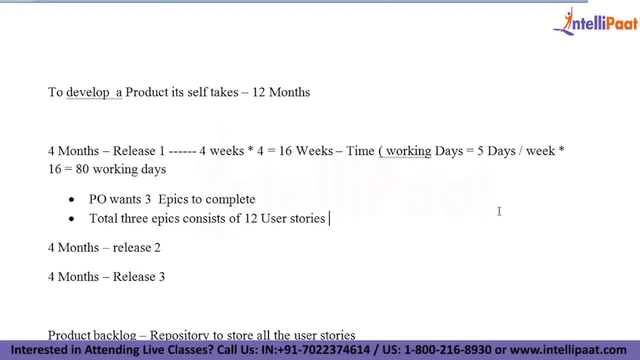 Now you could ask me one thing: why, Raj? why you have taken five days a week? because Monday to Friday is the working time, So Saturday, Sunday is the holiday. Hence we have taken five days in a week, right, five days per week into 16, 16 weeks. 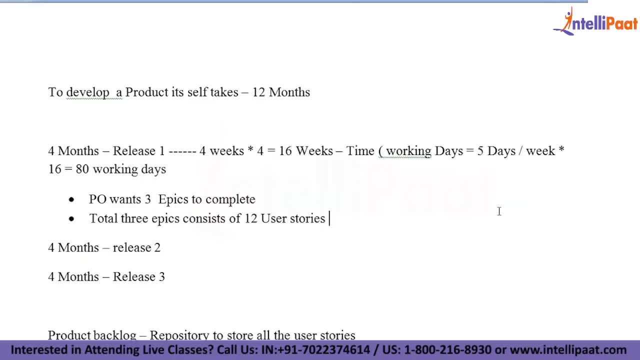 Means for four months. I'm talking about one release. I'm talking about one release release planning. release planning happens in every release. They said the same process we follow but whatever the user stories we have taken, whatever they picks we have taken, might be different from one to another. 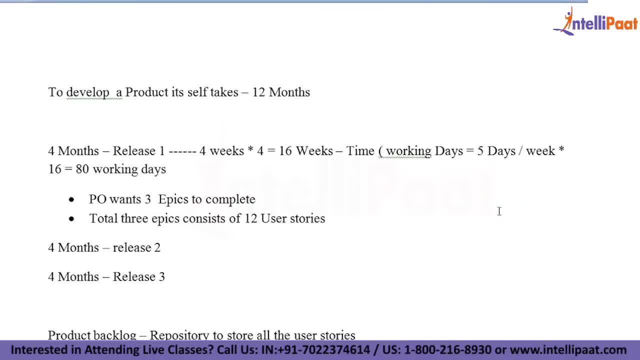 It will not remain constant and same all the time. So, roughly speaking, five days in a week into 16, 80 working days in this, 80 working days excluding any excluding holidays, any government holidays or festivals. all that comes, we have to exclude it. 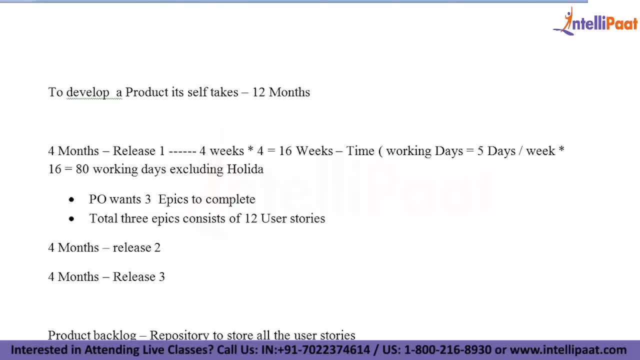 Then only we have to consider otherwise, because we cannot include all that right excluding holidays, because if there is any government holidays or some other days and all that, so that has to be deducted. Finally, working days comes into picture Now in this four months time. four months, nothing but four weeks into four: 16 weeks. five days in a week into 16: 80 working days excluding holidays. 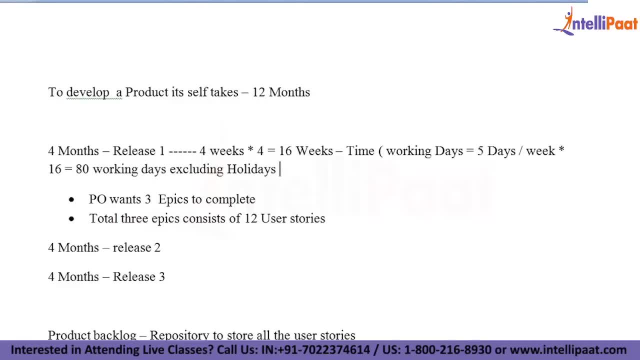 Assume that there was no working. there is no holidays except Saturday, Sunday. Assume that there is no holiday right: 80 working days in 80 working days. product owner wants three epic To complete. total consists of full user story. This is where generally the release planning process will be initiated. 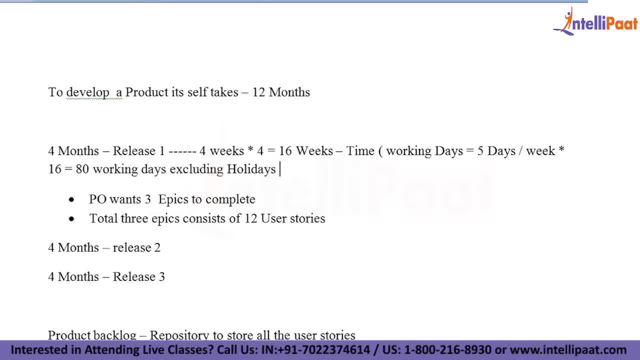 Now, if you want to discuss about the release planning process and all that, who has to involve here? product owner has to involve, point number one. second, a scrum master has to involve, because scrum master is the person who is to manage the scrum team and all they have to involve here at the same time. 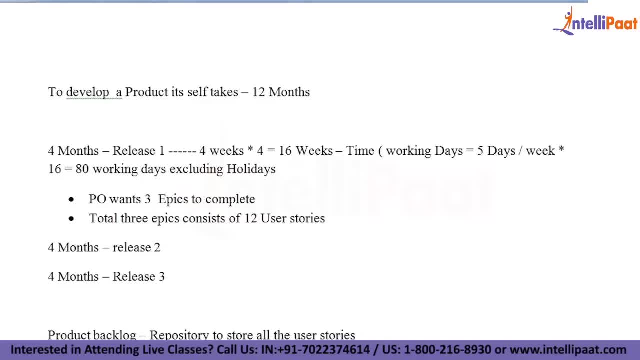 Team members should also be involved. scrum team members on that. Why? because, especially in agile, whatever the decision in reference to the implementation itself Is concerned, everything will be taken care of by the development team, not by the product owner, nor by the scrum master. scrum team members has to take in a decision on how much time it will be taken. complexity- all that stuff will be taken care of by the people itself. 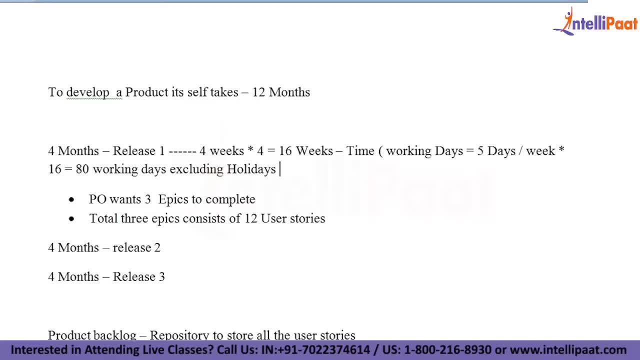 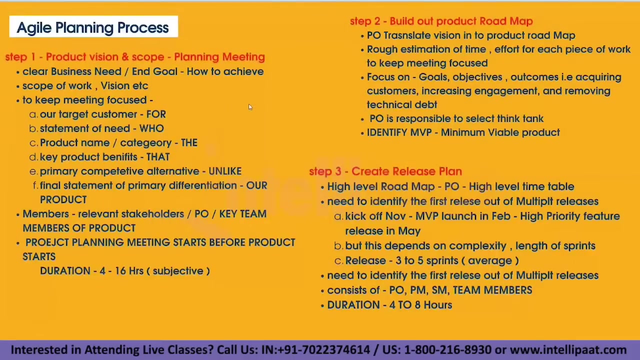 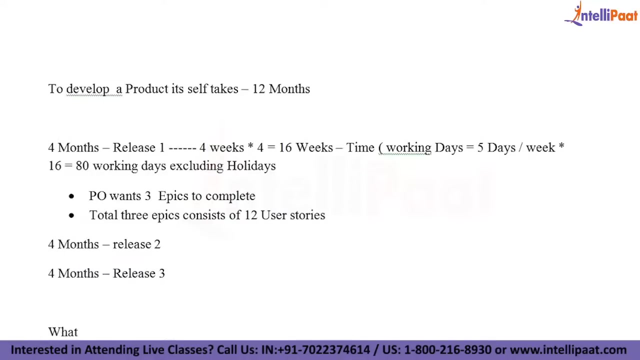 This is where, generally, the release planning process and all everything will happen means, if you're talking about four months, is the first release, roughly speaking, to complete a product wherein four months, product owner will give you the guideline to you. product owner will tell you In the first release: this is what I want. these are the three different topics which I am expecting you to complete. this, whatever the three, whatever the four months release, and all that, if you're talking about three epics, these user stories may be different. right, so the sprints and all everything will be different, because there are a few things we need to understand here. first point: what is product backlog? few answers, few questions. you need to understand what is user story. if you know about this, you'll be knowing what is user story, what is epic? first, what is product backlog? 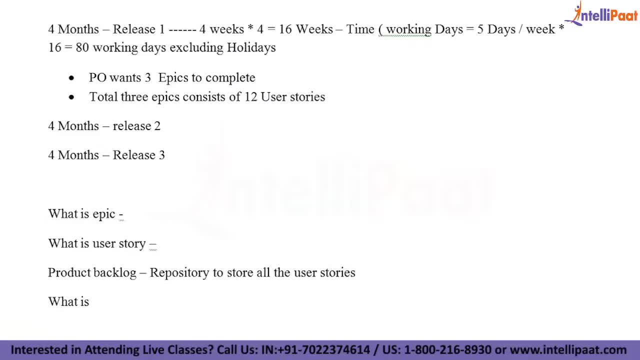 What is product backlog? next, what is right? these are the four things: epic, epic- nothing but large scale of solution. is what we call this epic right? what is user story? short description of requirement is called as user story. what is product backlog? there are different, different user stories. we are writing. for example, we have one user stories in three epics. where to store all these? there must be some repository to store all that. this is where generally product backlog comes. 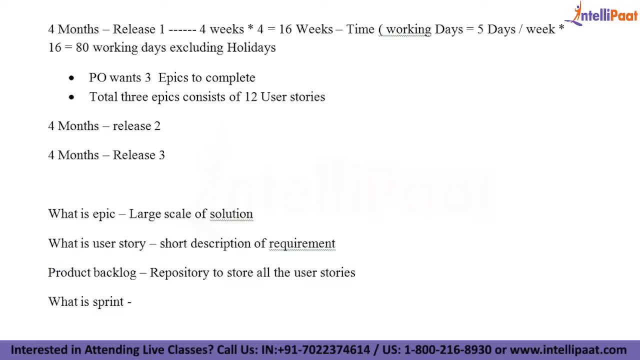 Now, what is sprint? sprint, nothing but collection of user stories which are we developing based on that. this is what we call it a sprint sprint. in simple terms, you can consider it as module. I don't compare that sprint with module. normally it won't, but assume that right, for example, this sprints may be anyone right. for example, if you have four weeks, for example, four into four, sixteen weeks, in sixteen weeks, normally sprints will be calculated. 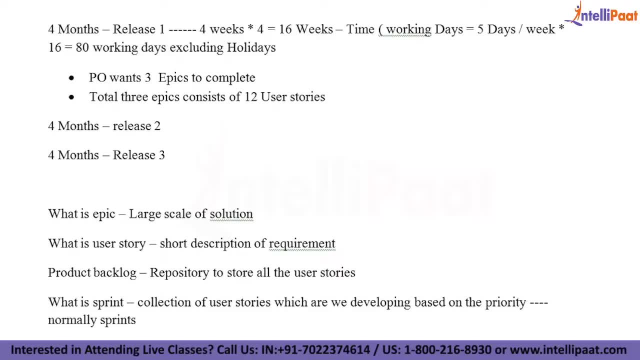 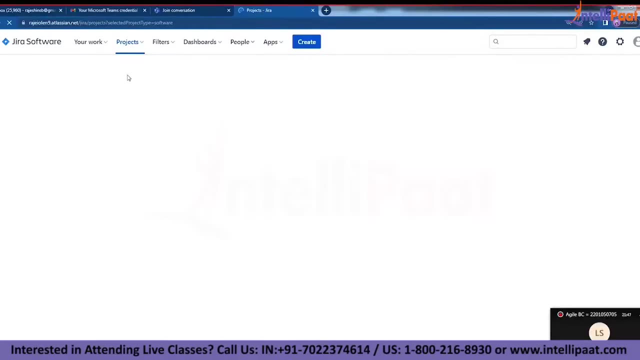 Sprints will be calculated, implementation of speed will be calculated into the weeks, into weeks, like, for example, this project. we have taken, for example, some project. let us take some project here. let's say, for example, Hospital management system. I have taken, okay, for example, right now there were different, different epics. we have written, followed the epics and all we have written the user stories also. 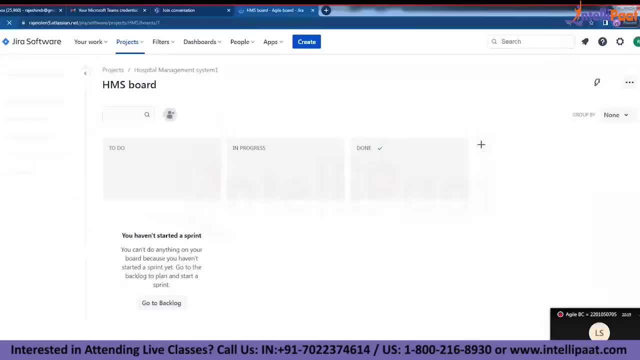 So whenever we write user stories, what is that we have to do, right? So here is where generally backlog is. backlog means what are the user stories and all everything will be there in this right. so this is the. this is all. whatever the user stories we have and all leftover. 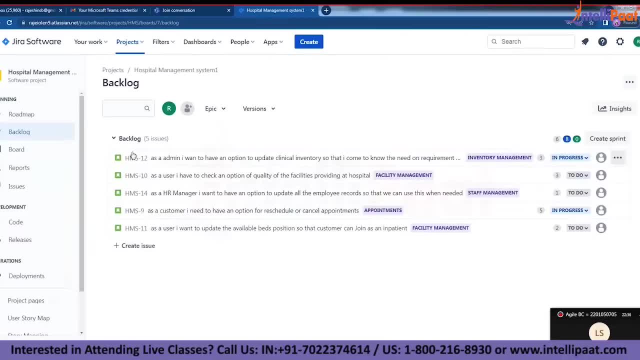 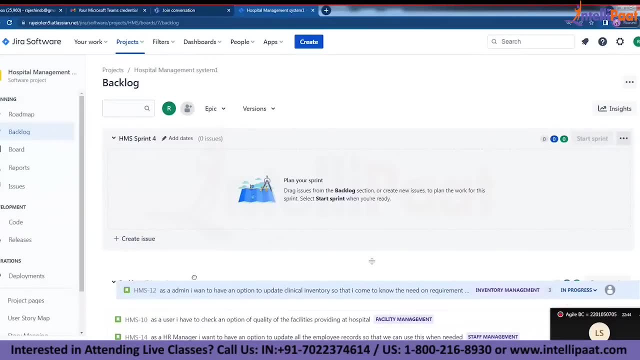 user stories will be there on the sprint, in the backlog. from here, what we have to do, we have to create a sprint, whatever the sprint we want to develop. so these we have to push here, we have to push here. push here means this is again based upon the priority, based upon the priority and all. 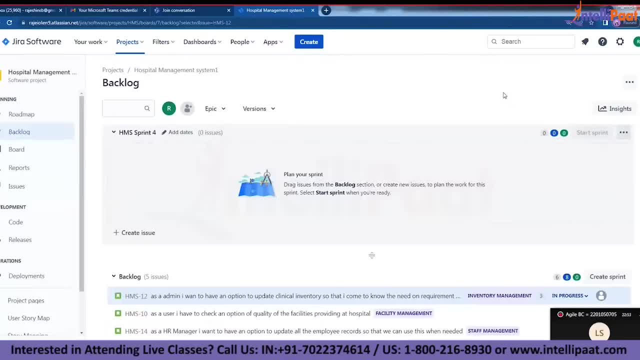 everything, so sprint nothing. but whatever the implementation based upon the time frame or time boxing thing, we are following, for that the thing is, which is called a spring means. if you are taking this into consideration, for example, if you want to complete four user stories, 12 user stories. 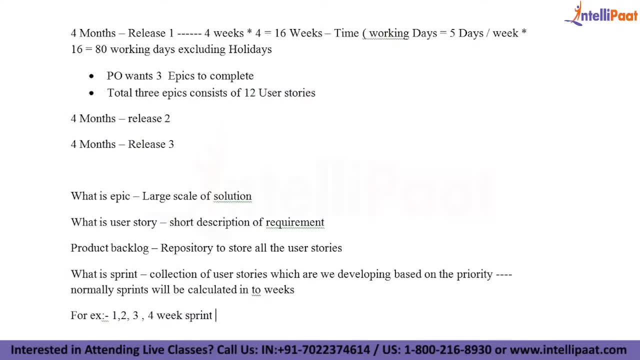 in three epics will be formed in different, different sprints. sprint will be form of one, two, three, four weeks and all. for example, sprint one out of twelve. right three user stories. right next sprint two, sprint two. for example, customer is expecting you to develop four user stories. 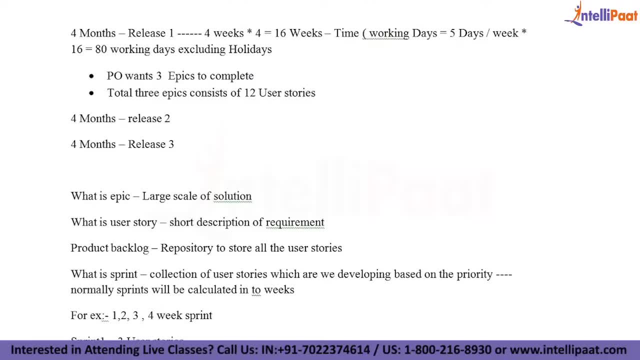 right, and maybe sprint: three, uh, four plus three. twelve, four plus three, twelve, yes, uh, four plus three. seven, right, purpose is seven. for example, two user stories. we have taken print. so sprints: there is no guarantee like these many sprints, it will be taken. so if you are taking sprint and all, 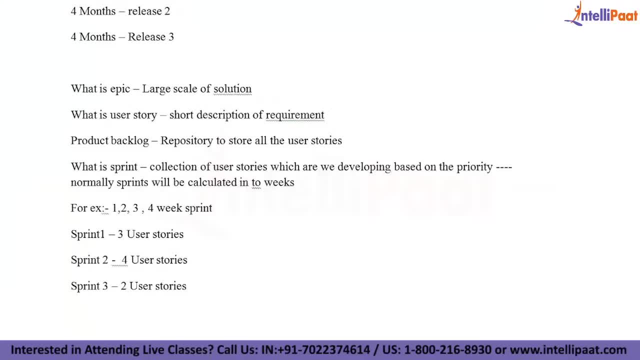 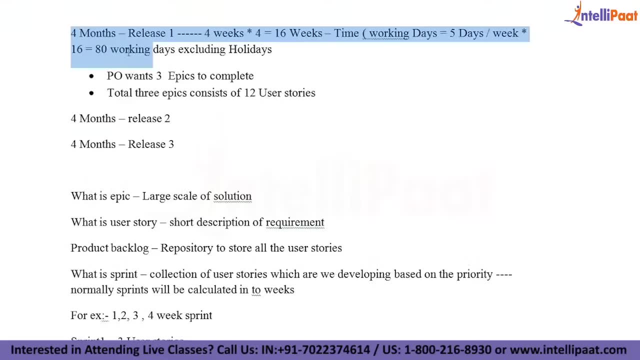 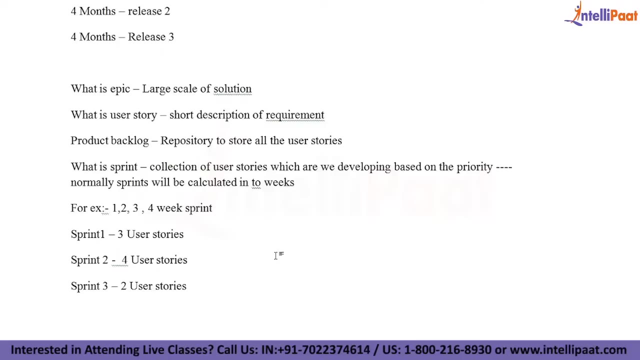 it depends on how many user stories we have taken and how much effort it will be taken all that into consideration. so, whenever we are doing the release planning- release planning process and all everything is depending on how many sprints we are developing- these prints normally will be converted in a form of weeks: one week, two weeks, three weeks, four weeks and so on. right so? 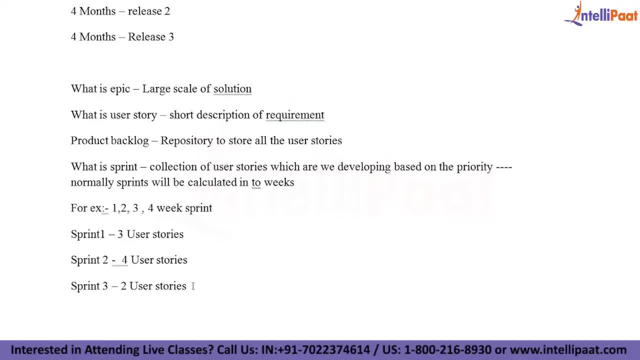 normally, for example, if you are taking 12 user stories, it can be like this: sprint one may be having three user stories. sprint two may be having four user stories. sprint three will be having two user stories, four plus three, seven, seven plus two, nine- for example nine, print four may be having 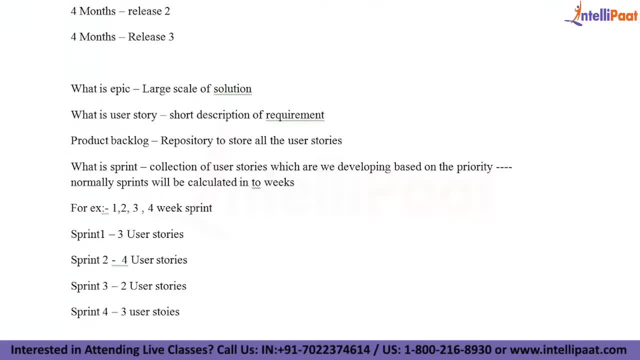 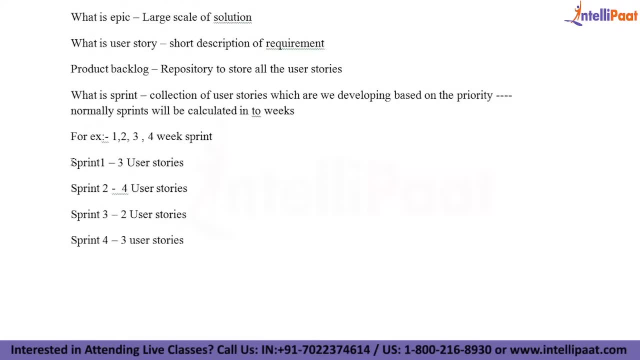 three users, right, so three users to this. so to complete, if you can see roughly, if you want to complete this, 12 user stories out of three epics in the first release. how many sprints we have planned? we have planned four user stories, four sprints. it may not be four sprints, sometimes it may be six. 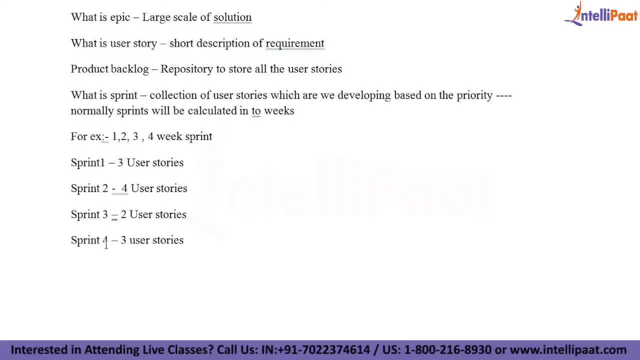 it may be two, it may be three, it may be four, even why? because it's purely depends on how many user stories we have taken at the same time. what is the complexity which is involved to implement that? because particular user story, nothing but the functionality. if you want to implement the 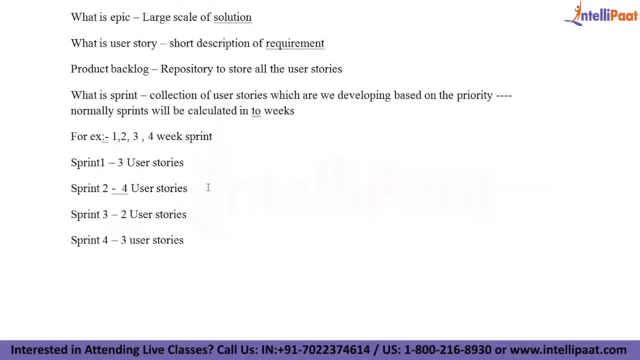 functionality. what is that you require? there is an amount of complexity which is involved in it's depends on so. for example, three user stories may be taking two weeks. for example, four user stories may be taking three weeks, four weeks time for you to come two user stories. sometimes it may. 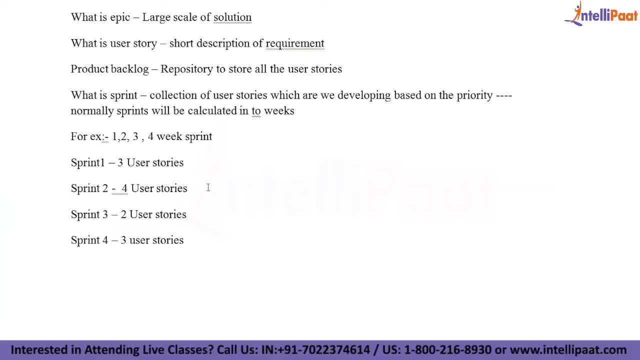 be taken one week for you to come. maybe the three user stories may be taken four weeks time for you to come, right, so, which is not something guaranteed, right? it's really because this planning, whatever the sprint planning and all everything this will be decided by the team members, but when we are 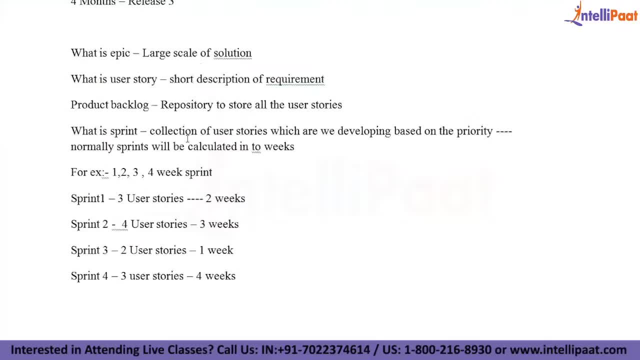 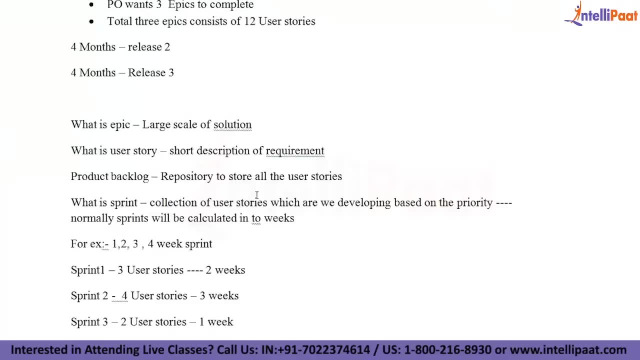 planning about the first release means, whatever the release we are planning, and all being a product, a reason why product owner is being involved here. why? because product on is the person is expecting you. this is what i want you to complete now, when it comes to the implementation part, who has to? 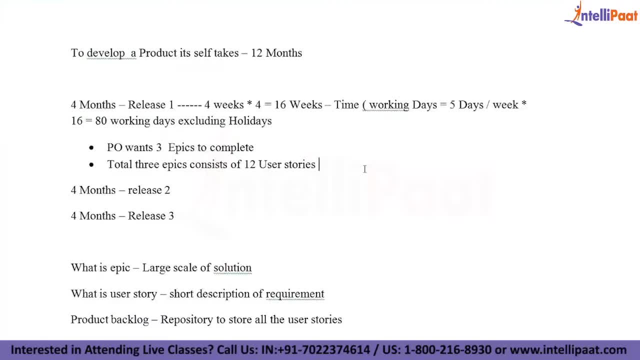 take any decision on this. this decision has to taken by the team members, so team members should also be knowing about the release planning process in advance, whether how many user stories they are developing, how many sprints they are developing in first sprint, second, third, fourth and all everything. 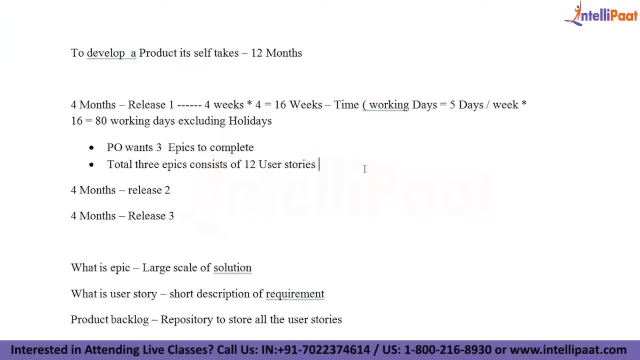 is done at the time of sprint plan. so before that, whenever they are completing the release planning process, product owner will give you the clear understanding about what is that is they are expecting in how many days this has to be completed. assume that if it is taking four months sprint for 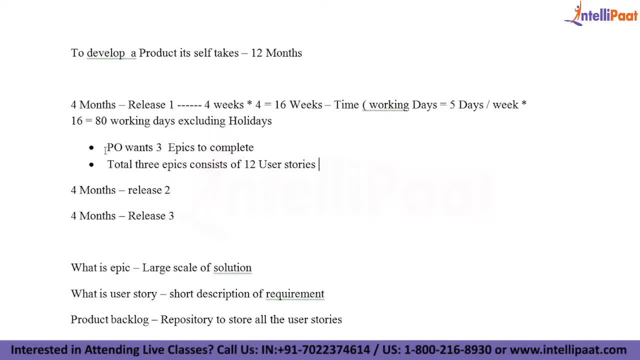 example, in 80 working days, i want these three epics to be completed, which is a combination of 12 user stories. now you could ask me one thing, raj: is it only confined to 12 user stories? don't you think sometimes, more than 12 user stories will also be there sometimes? yes, there is a possibility. 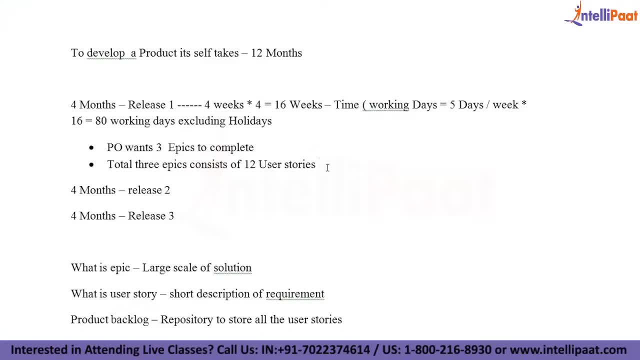 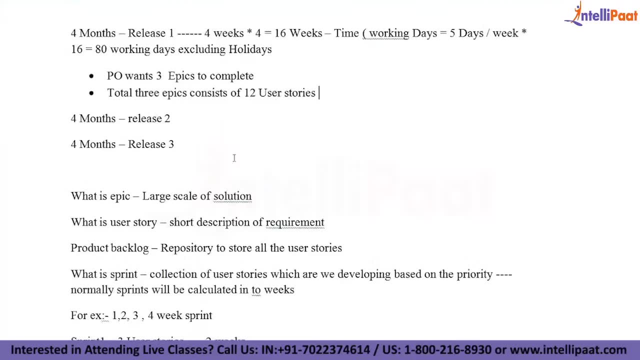 that's the reason why, whenever we are implementing in agile implementation and all, there are two different things: some user stories and all everything will be in the sprint, some user stories in real environment. normally what we say that there are out of sprint means there are no no in the sprint, in the initially sprint, whenever the sprint planning and all everything we do. 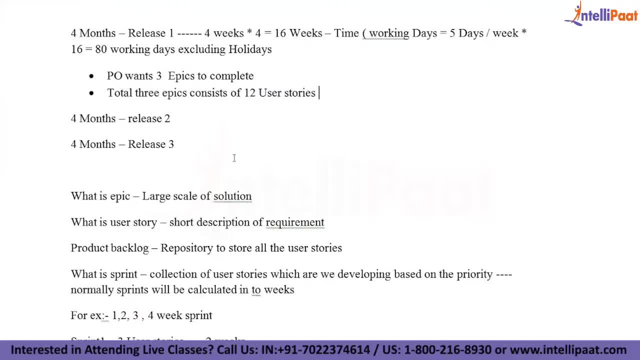 these user stories won't be there. after that these user stories will come and add in. between. that kind we arise means there is possibility. i don't say it's a problem, there is a possibility it may be arise to you. so that's the reason why, whenever we are doing the release planning process, 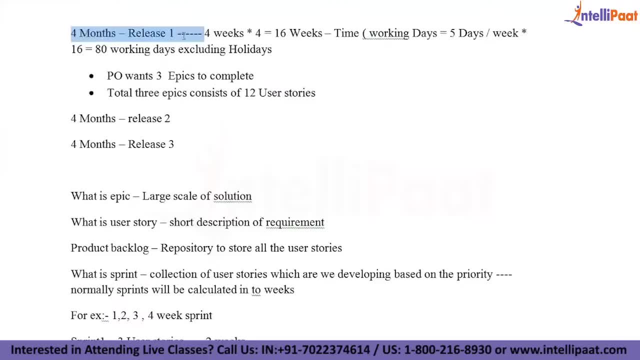 in the release planning process. how many epics should be completed, irrespective of the user stories, of course. i have taken 12 user stories here. it may be 20, 30, 40, 50 and so on. right, so forget about that. how many epics to be completed in the first release? that decision will be given. 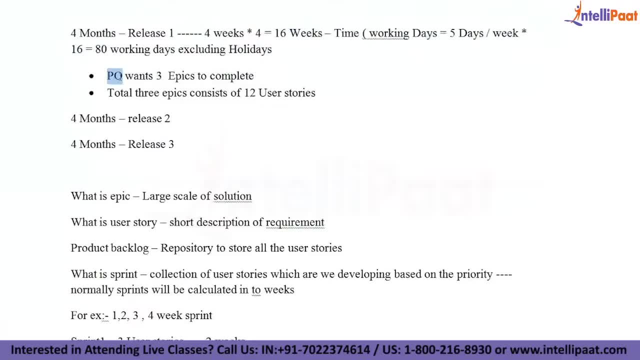 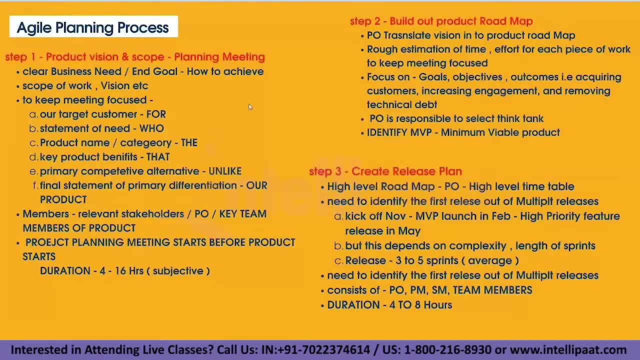 by the periodic toner, where this understanding and all should be there to the team members who are attending in the release planning process means either by scrum masters or scrum team, and all these people should understand how many epics to be completed, irrespective of user stories, because how many sprints we want to develop, each and every sprint. 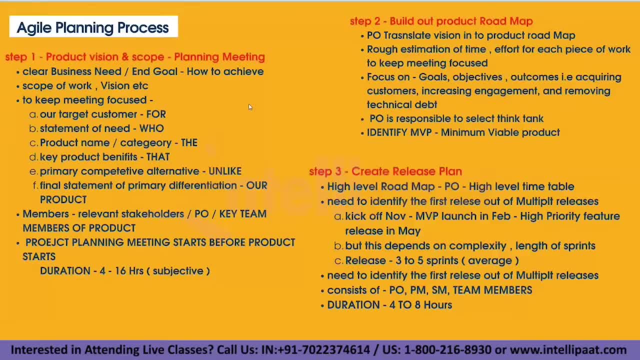 how many user stories, and all again that is depends on the complexity of the particular user story, because that complexity is different. right, for example, even though there will be some simple requirements, something like login page creation itself looks very simple, but when starts implementation and all complexity might be increased day by day. because we have started for 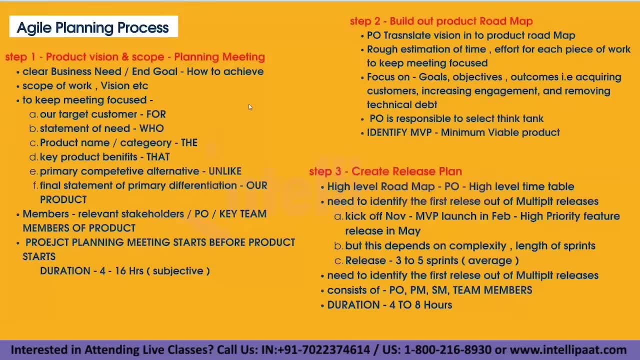 example, right, because login page, we don't feel much difficulty. but what will happen in practical, difficult, practical possibility is that you could ask me, raj, what, what complexity you can see in login page creation, because it looks very simple. so why? why it will be complex in future? because 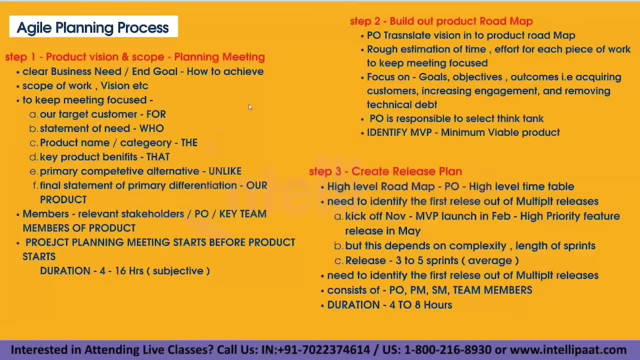 what will happen whenever we have started, maybe the complexity might be less, but afterwards keep on. some sort of requirements and some sort of changes happened in between, might happen, might be taken place. so what will happen? obviously, as there is a lot of changes are involved in the existing functionality, what we are developing automatically, complexity also. 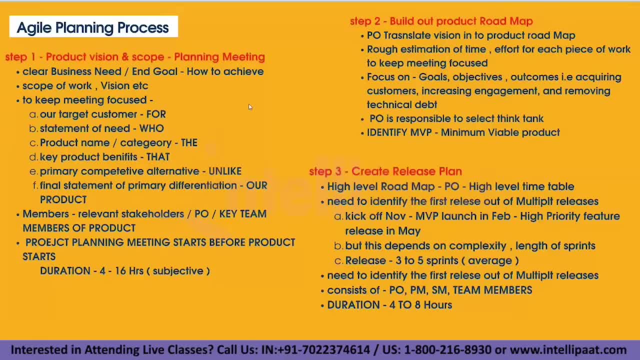 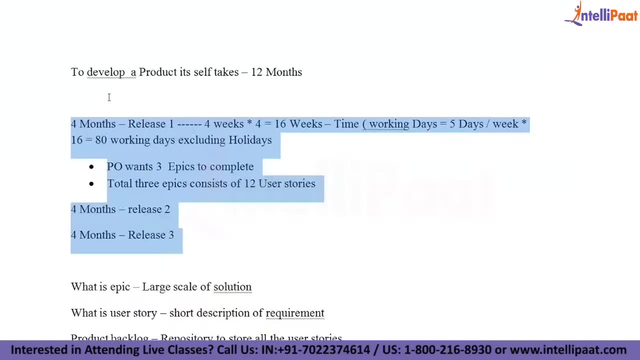 increased when there is a complex increase, the effort, how much time people were spending to complete, and all will also be increased, obviously when duration is increasing. obviously the timelines will also becoming very short, understood, clear everyone. is it clear to everyone, or not normally in traditional model, what we do? 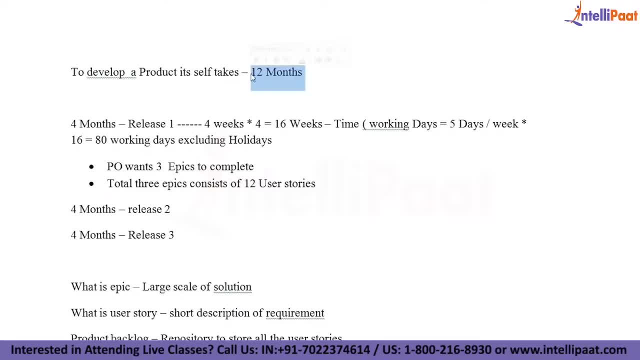 once the product is completed. finally, after the duration, after 12 months or so, normally, finally we, finally we deliver the product to the client, normally speaking, in regular models, all that stuff, but whereas when it comes to the agile and all everything we are doing, releases by point number. 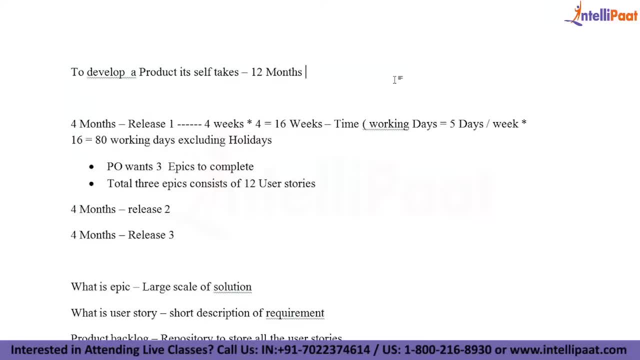 one point. number two, not only on the releases, if there is any kind of things to be added in between, there is a flexibility of doing the changes. here there is a flexibility of doing changes. why there is a flexibility of doing changes? because whatever the flexibility of doing changes, because whatever the 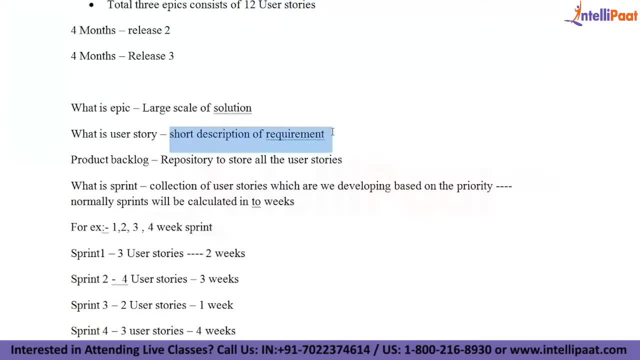 user stories. whatever the requirements we are writing, all these requirements are writing in a form of user story. user story is individual, user story is individual. so you, there is no connect with user story with other user story, right? if i am writing a user story, this user story is no way. 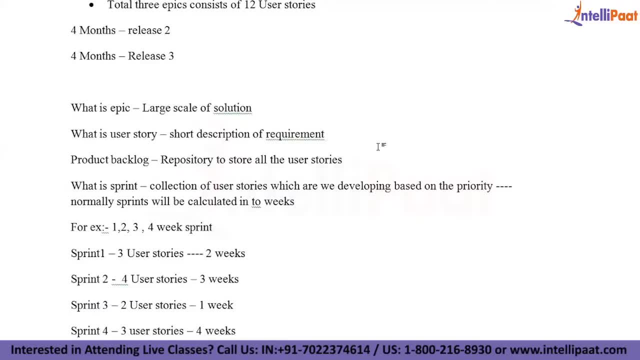 connecting to other one. there is no connect. that user story is individual on its nature. so when there is an individuality, what will happen automatically? there are possibilities that that can be changed at any point in time. of course, effort is taking more, but there is a possibility. 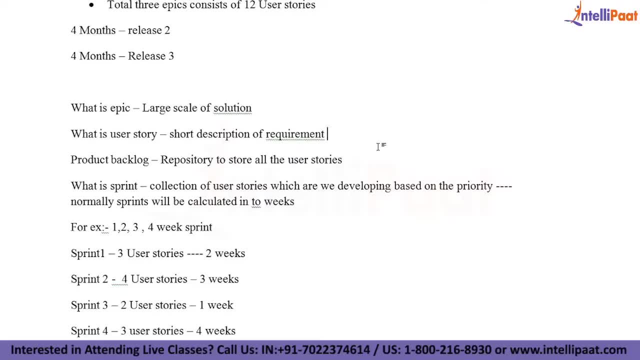 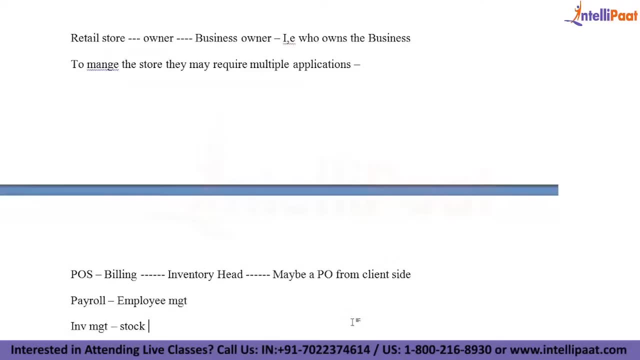 that we can start doing changes by point and that we place facilities in a particular, that we can change n number of times, subject to terms and conditions, if it is being accepted by the team. yeah, this is what generally the release planning process is, so release planning has to be done. 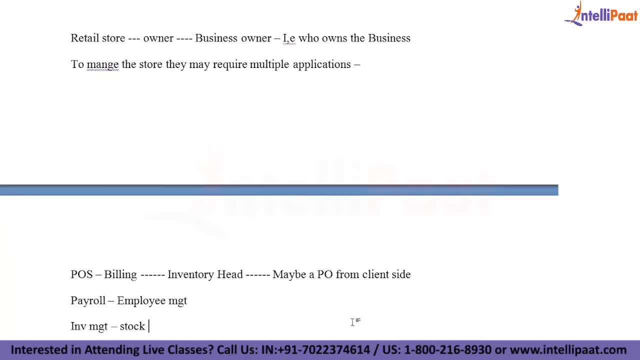 so release planning, whatever the release planning process i have explained you so far, the same process happens in each and every release. even it may be first release, second release, third, fourth and so on, the release planning remain constant every time. whenever there is a really there is a release, the planning process is something inevitable. okay, because there. 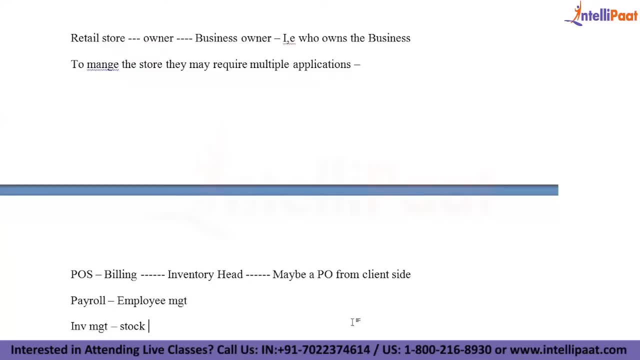 is no one release plan. how many releases we have, those many release planning processes has to be made. yeah, in this release plan, release plan for the particular release either. it may be one, two, three, so whatever the part of creating a release plan- and all this is a repetition- one first: 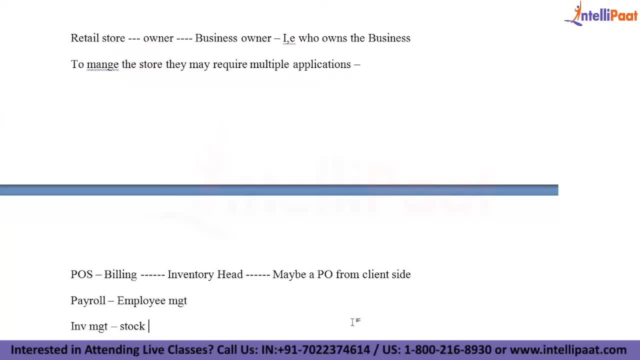 release, that happens the same, maybe for the second release, maybe for the third release, and so on. whenever, whenever, whenever, how many releases we have, release planning will be continued the same, the same way. i have just given you the rough idea here, right, for example, if you're taking one release, so based on that, 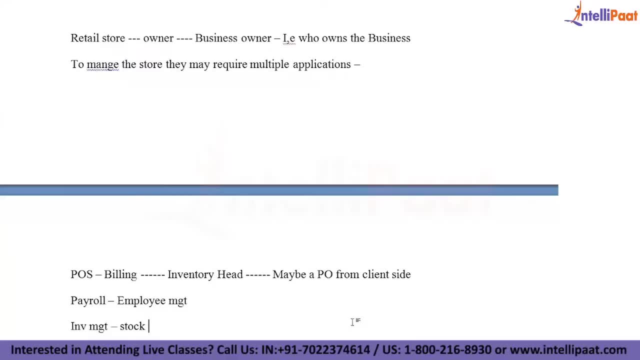 because how many epics and all everything. there is a dependency, right. so how many releases and all everything. so this is what generally release planning process is all about. once the release planning process is completed- yeah, once the release planning is completed- the next part is that fourth is sprint planning. for this sprint planning, right? so the release planning part and all of 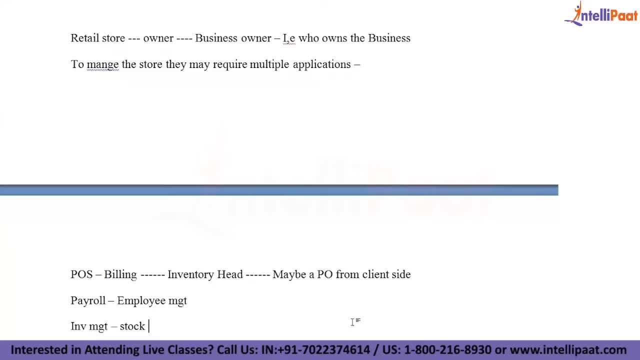 the things. what is the sprint planning part? so, whenever we are going to sprint planning, first of all, what we have to do, whenever the first part- like providing creating this product roadmap right, so creating release plan, all that- normally there is a concept called product back. this is where we have discussed here, but of course not in detail, product backlog. so what is product backlog? for example, there is a product called payroll. now task. what is task? 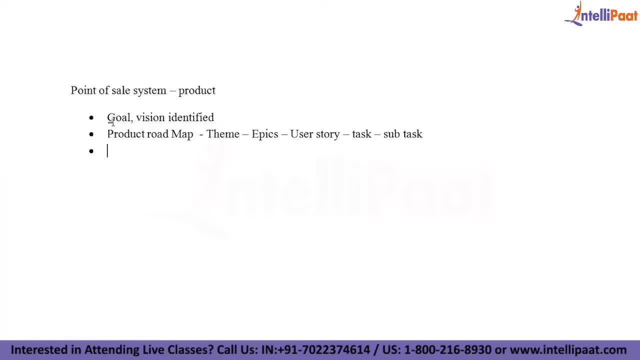 task, task. simplifying user story is nothing but task. again, simplifying the task into sub task, because this is all to reduce the complexity. you are doing this, right, simplifying the task. this is what we call it a sub task. right, this is what, generally, the roadmap is. once the roadmap is created, what 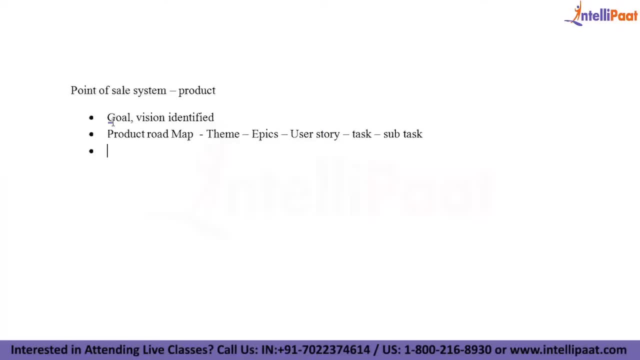 is that you are doing? you are writing down the user story where you have to put is we have to put to product back. what is product backlog? it's a repository to store all the user stories, not only user stories. we can store anything, right. so this is what generally, the product backlog is. 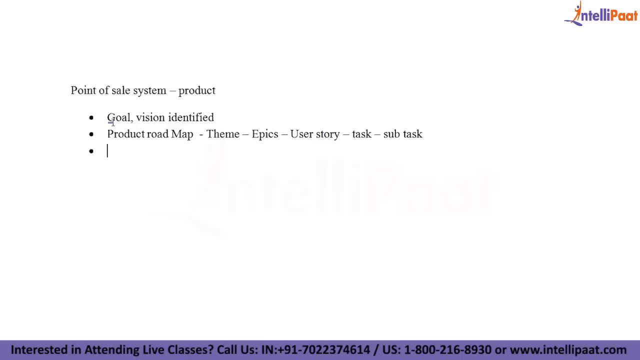 so product backlog creation is what we have to discuss before you are going for sprint planning. product backlog is there, so this is what the product is. for example, you are taking hospital management system. there are different epics. epics have user stories. what is that we are doing? 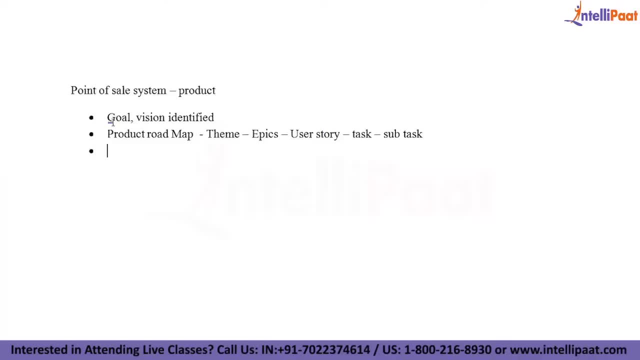 whatever the product is, we are putting to product backlog. so this is what the product is, where user stories, everything will be there, all these these things you can see in the product backlog. this is what your product backlog means. it's a repository to store all the user stories. 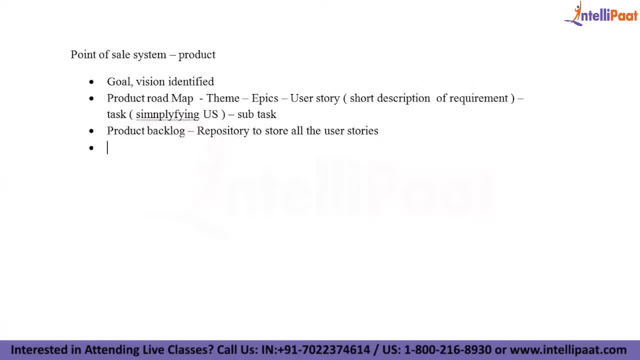 whatever the user stories and all everything will be done under product background, right, so from product backlog, what is that we are doing from here onwards? whatever the scrum ceremonies i have told you, right sprint planning, daily scrum sprint review and retrospection will be taken place. understood, everyone right, understood or not. following right goal and vision, followed by 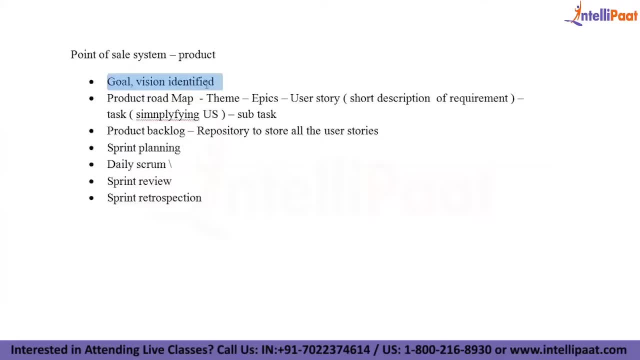 this product roadmap you have created. in this product roadmap you have epics, user stories, all that as i shown you on jira just know, sometime back next from there what you are doing: you are creating a product backlog in the same user story, in the jira itself. we are storing all the user. 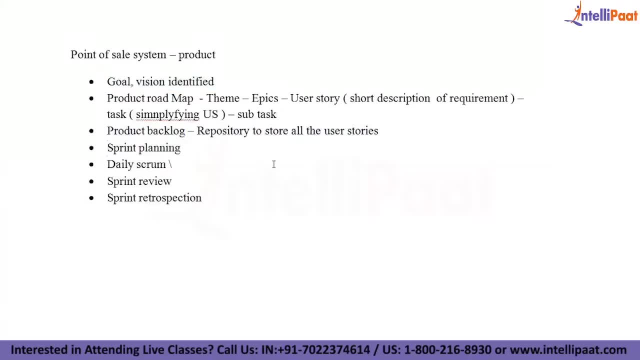 stories in the product. from there what you are doing, again from the product backlog. we are taking few user stories and we have to do sprint planning and all, of course, sprint planning. i have not started yet, because what is product backlog? why do we do product backlog? for what reason product backlog is to be done, i have to discuss now. so for that there. 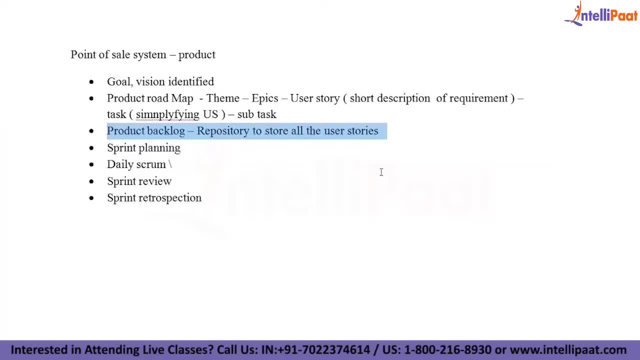 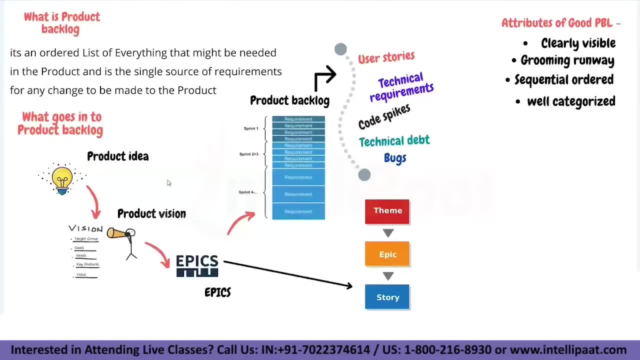 is a presentation for product backlog which i am showing you. let me explain that. first, confirm me whether you can see this or yeah. can you see this product backlog? right? so this is yeah. so this is what generate product backlog consists of. what is product backlog? just don't have told you product backlog- nothing. but whatever the user story is. 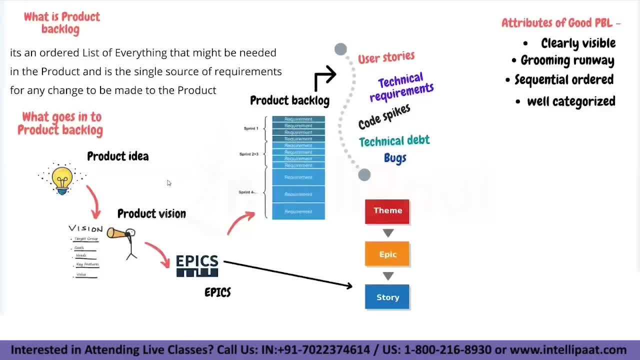 are we writing to store all the user stories? we require a product backlog. it's a repository to store all the user stories, but product owner is. product backlog is not only for user stories, because user stories are nothing but functional requirements, isn't it? that's what i have told you. 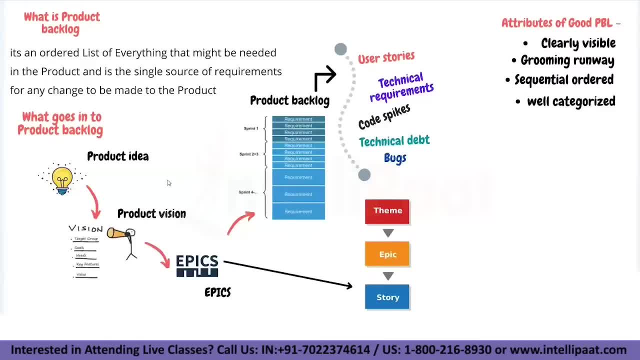 in the beginning. but there may be some technical requirements also. right, some technical requirements will be there, so technical requirements will also be there in the product. back, for example, code spikes. code spikes means, for example, some demo kind of work has been done by the team, so where? 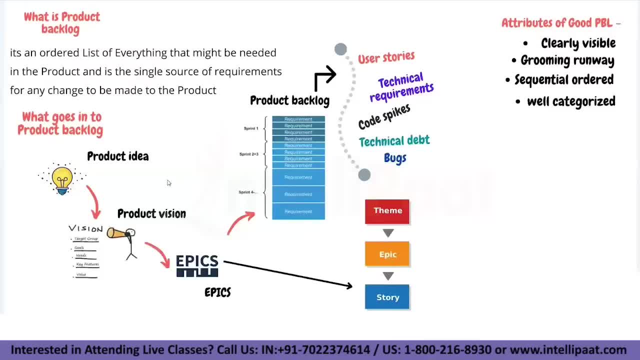 are we that putting that information? for that information also, we put it on the product backlog. for example, there is some technical doubts, technical debts, all these that also will be there in the product backlog. so product backlog means this is what generally product backlog is. so product backlog means where in this product backlog, whatever the user stories we are writing. 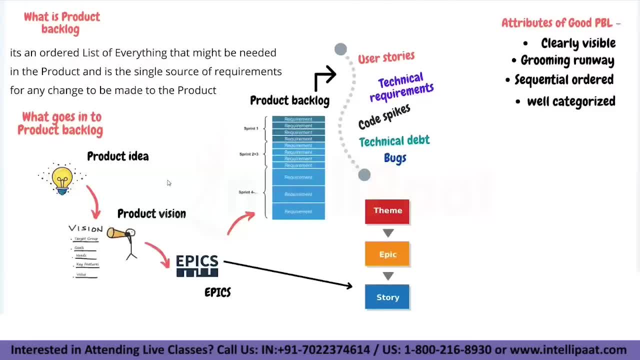 whatever the technical requirements, whatever the code spikes we have, whatever the user stories we are writing, whatever the technical requirements, whatever the code spikes, whatever the user stories we are writing, whatever the code spikes we have, whatever the code spikes we have, whatever the technical gets debts, whatever the bugs. bugs may be may not be immediate, maybe once. 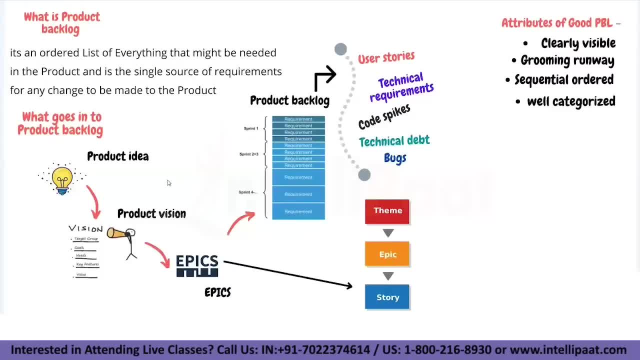 the implementation has been taken place, whatever the bugs we have identified. all this can be stored in this product backlog. so product backlog refinement process, creation of product backlog, maintaining it, backlog refinement process- all that we'll be looking after by the product owner in normal. but if you want to put something in the product backlog- what are all product backlog goes. 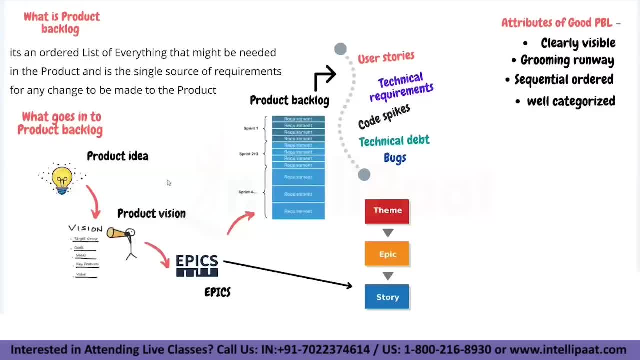 and all this is how generally the product backlog goes and this is how generally the product backlog goes and this is how generally the product backlog goes and this is how generally the product backlog is. structured product idea: we have discussed earlier product was structured product idea we have discussed here. product Ukrain- his 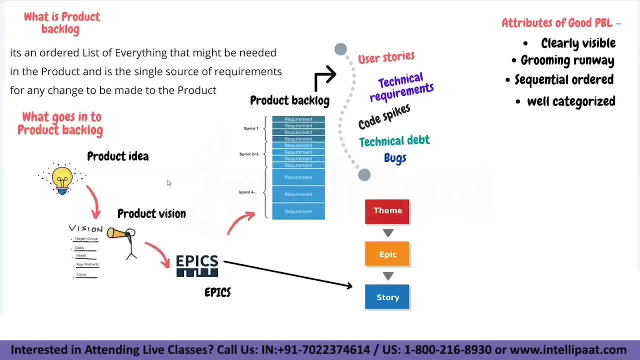 repository between means. once the product roadmap is being created. once the product roadmap is being created, at the time of the thing, product backlog has to be created. we have to create a product backlog, product roadmap, based on that release planning process. after that sprint plan, sprint planning in its development: what to develop? how to develop? how much time do we have, how much manpower? 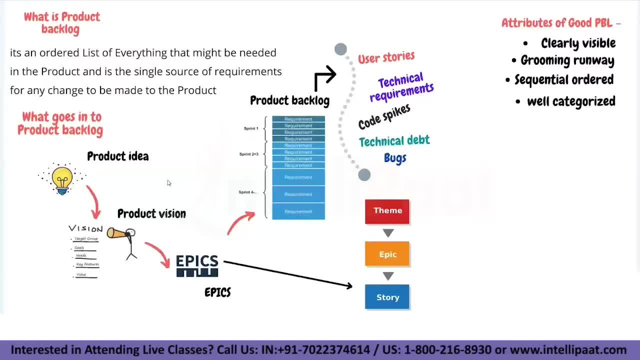 do we have? how much manpower? how much time do they have to complete? will there be any possibility for them to complete within the timelines or not? how much time it will be taken for the particular user story to complete and for that how many story points to be given. and all everything comes under. 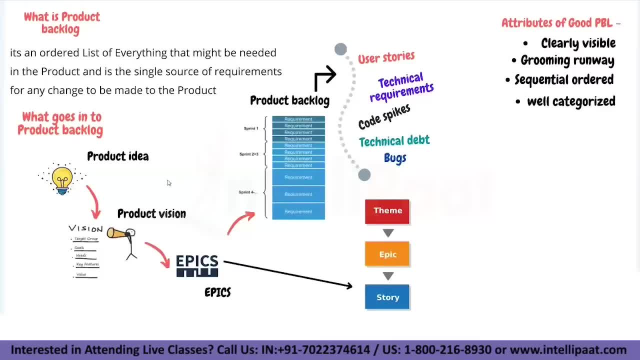 the sprint planning. so we have not even started sprint planning yet. remember right, we have not started sprint planning. actual sprint planning will be started after, not now. what is that we have done so far? is that only about till release? planning is what we have completed, you so creation and vision on scope of the product is what we have created first. 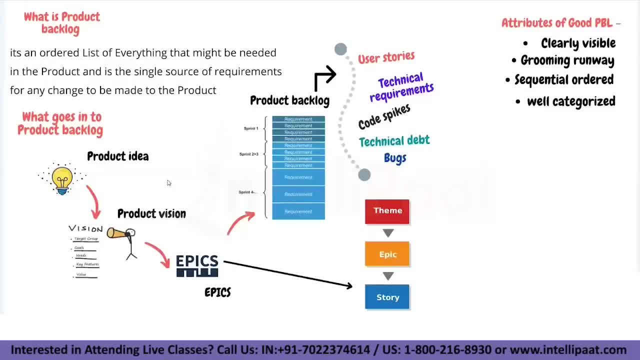 next, we have to create a roadmap. based on the roadmap, product backlog creations and everything will be done here. based on that, release planning will be made here. once the release planning, everything is done, okay, fine, we understood clearly that in another four months, this is what we want.